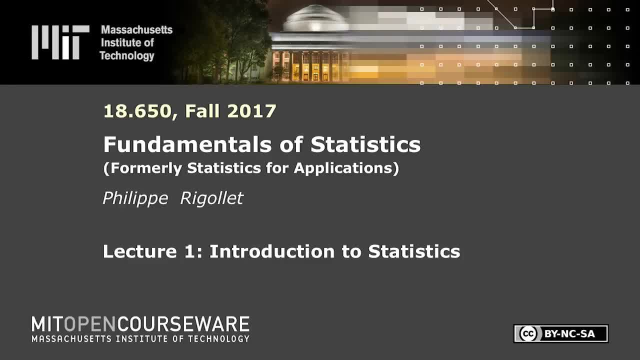 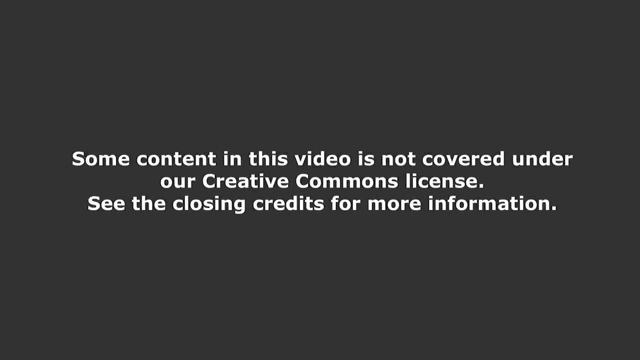 The following content is provided under a Creative Commons license. Your support will help MIT OpenCourseWare continue to offer high-quality educational resources for free. To make a donation or to view additional materials from hundreds of MIT courses, visit MIT OpenCourseWare at ocwmitedu. 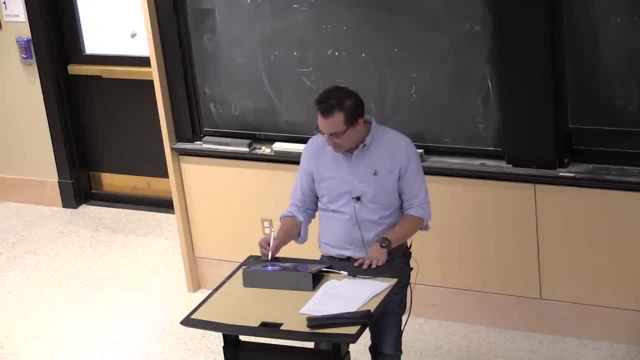 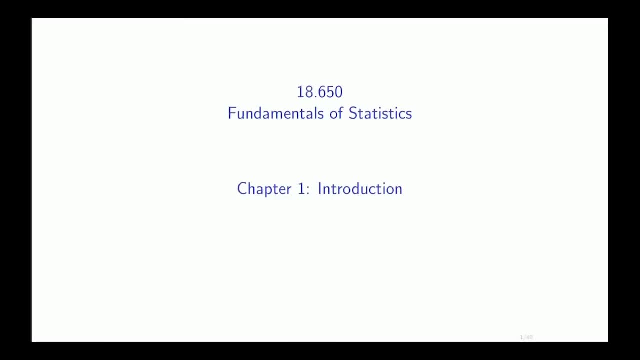 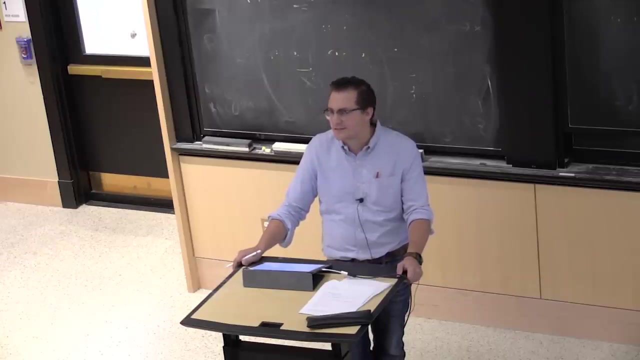 Okay, so the course you're currently sitting in is 18650, and it's called Fundamentals of Statistics, And until last spring it was still called Statistics for Applications, and it turned out that really, based on the content, Fundamentals of Statistics was a more. 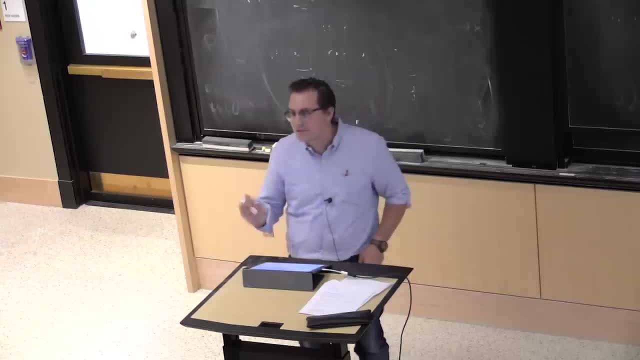 appropriate title, So I'll tell you a little bit about what we're going to be covering in class, what this class is about, what it's not about. I realize there's several offerings in statistics on campus, so I want to make sure that you've chosen the right one. I also 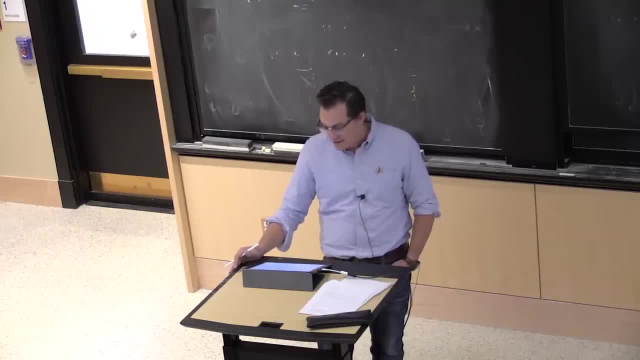 understand that for some of you it's a matter of time, It's a matter of scheduling. I need to actually throw out a disclaimer. I tend to speak too fast. I'm aware of that. You know someone in the back. just do it like that when you. 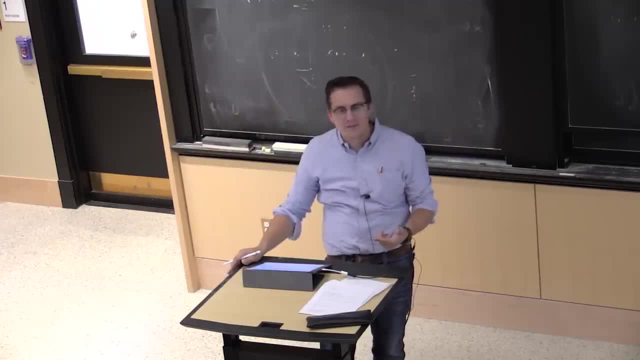 have no idea what I'm saying. Hopefully I will repeat myself many times. so if you average over time, you will see that statistics will tell you that you will get the right message that I was actually trying to send. All right, so what are the goals of this class? So the first one is basically to give you 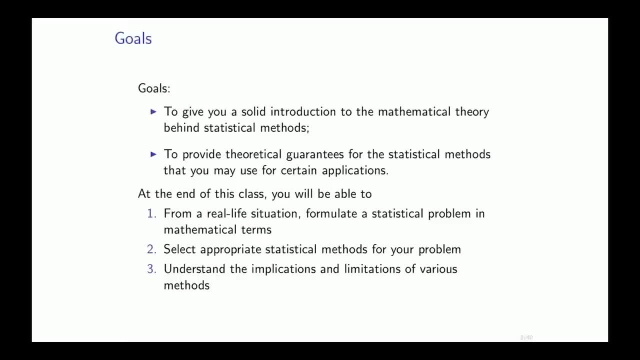 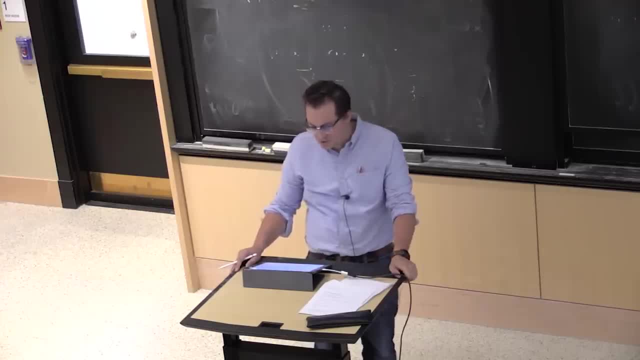 an introduction, No one here is expected to have seen statistics before but, as you will see, you're expected to have seen probability and usually you do see some statistics in a probability course. so I'm sure some of you have some ideas, but I won't expect anything And we'll be using 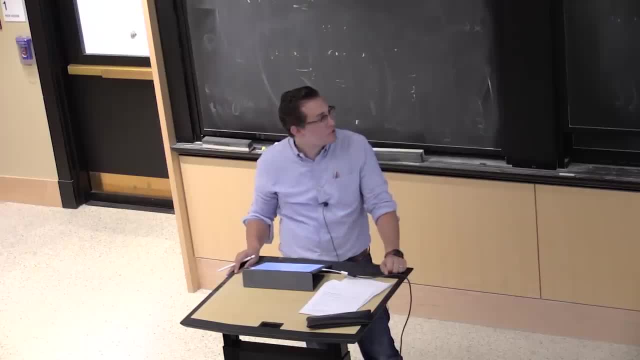 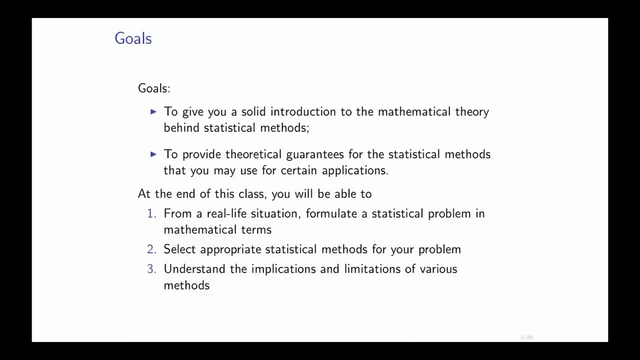 mathematics. right, It's a math class, so there's going to be a bunch of equations, not so much real data and statistical thinking. We're going to try to provide theoretical guarantees. We have two estimators that are available for me. 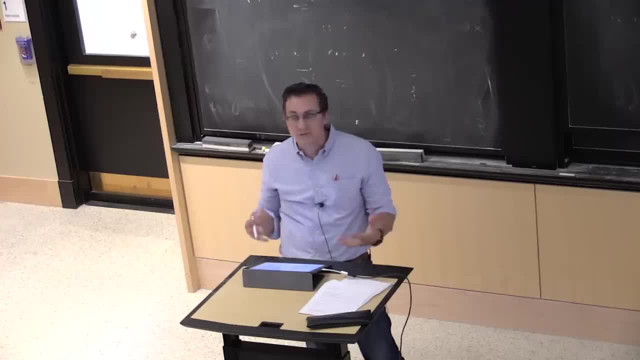 The theory guides me to choose between the best of them. How certain can I be of my guarantees or prediction? It's one thing to just spit out a number, It's another thing to put some error bars around them. so we'll see how to build error bars, for example, And you will. 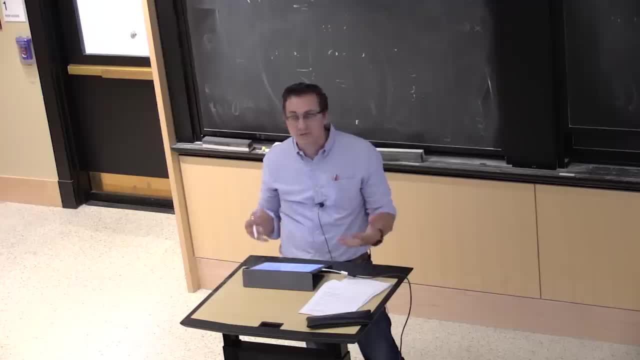 And so you know, I think that's the goal of this class. And then you know, the theory guides me to choose between the best of them. how certain can I be of my guarantees or prediction? It's one thing to just spit out a number, It's 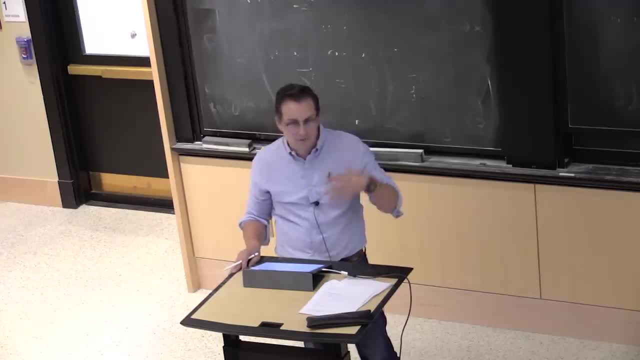 another thing to put some error bars around them. so we'll see how to build error bars, for example, And you know you will have your own applications. I'm happy to answer questions about specific applications, but rather than trying to tailor applications to an entire institute, I think 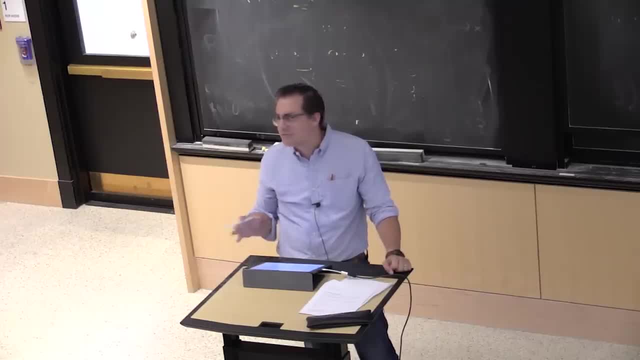 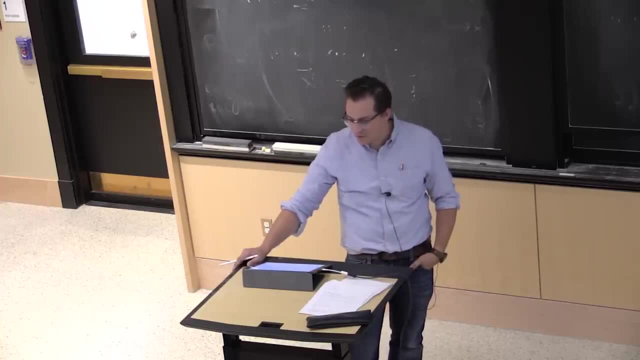 we're going to work with pretty standard applications mostly. you know you're going to have a lot of people that are going to be, you know, not very serious ones, And hopefully you'll be able to take the main principles back with you and apply them to your particular problem. 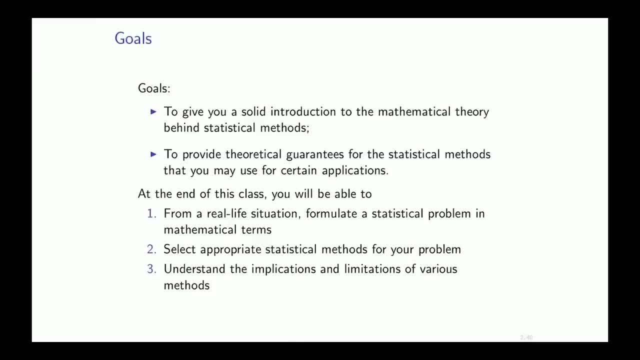 So what I'm hoping that you will get out of this class is that when you have a real life situation- and by real life I mean mostly at MIT, so some people probably would not call that real life- the goal is to formulate a statistical problem in mathematical terms. 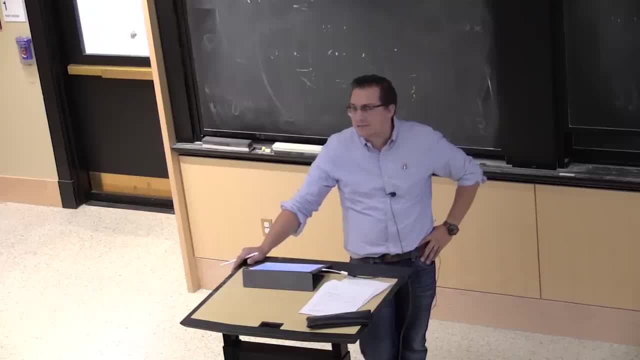 If I want to say, is a drug effective? that's not in mathematical terms. I have to find out which measure I want to have to call it effective. I want to. maybe it's over a certain period of time, Maybe it's over. so there's a lot of things that 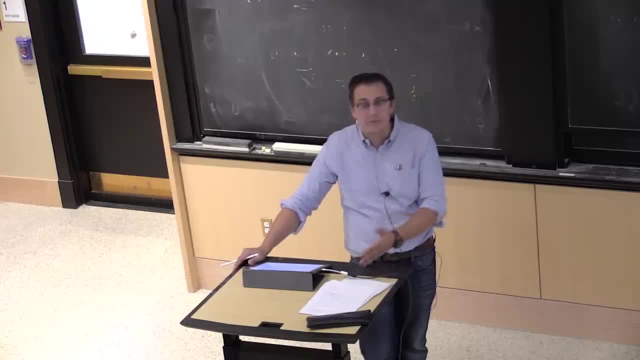 you actually need, And I'm not really going to tell you how to go from the application to the point you need to be, but I will certainly describe to you what point you need to be at. if you want to start applying statistical methodology, Then, once you understand what, 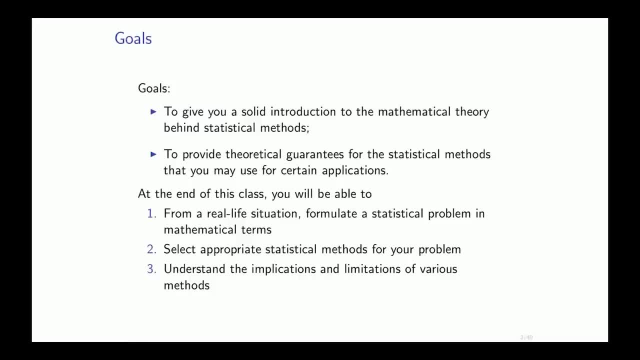 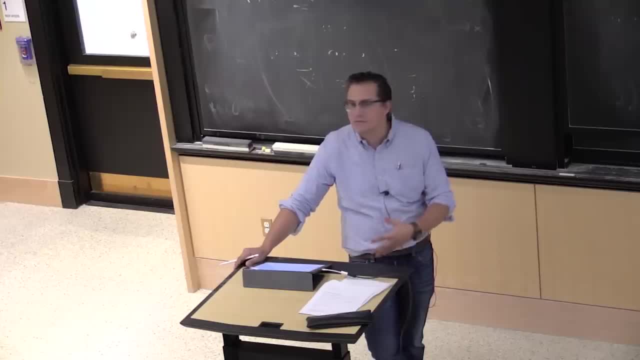 kind of question you want to answer. do I want a yes- no answer? Do I want a number? Do I want error bars? Do I want to make predictions five years in the future? Do I have sighted information or do I not have sighted information? All these things. based on that, hopefully you 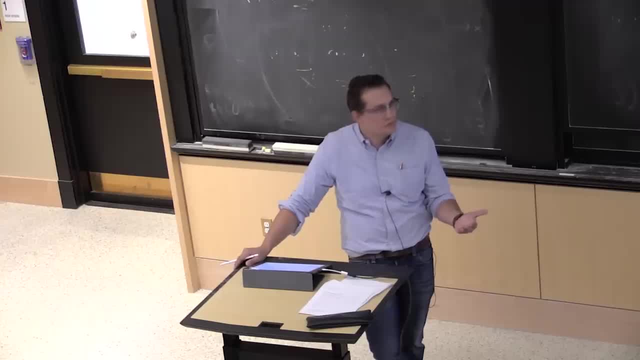 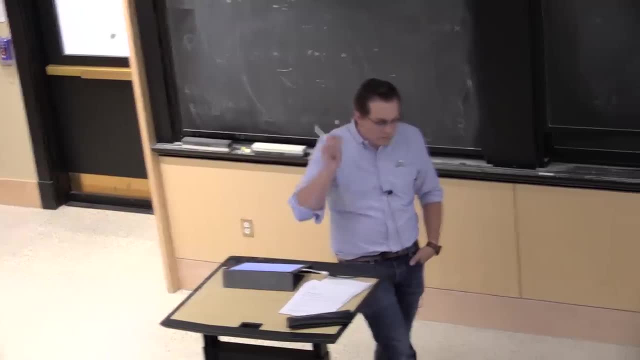 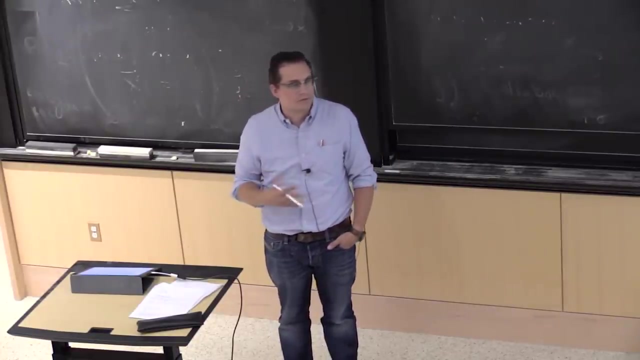 will have a catalog of statistical methods that you're going to be able to use and apply in the while. And also, no statistical method is perfect. Some of them people have agreed upon over the years and people understand that this is the standard, But I want you to be able. 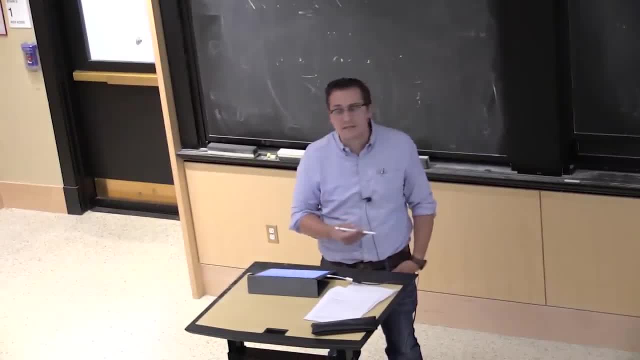 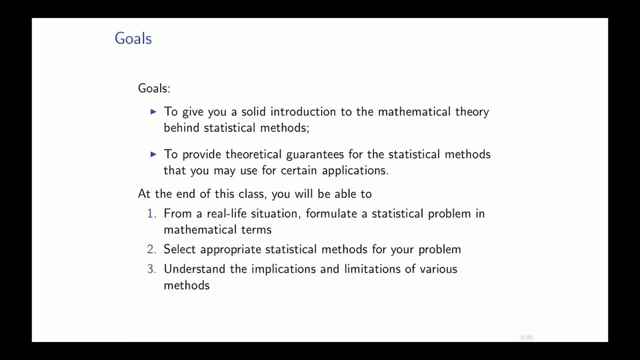 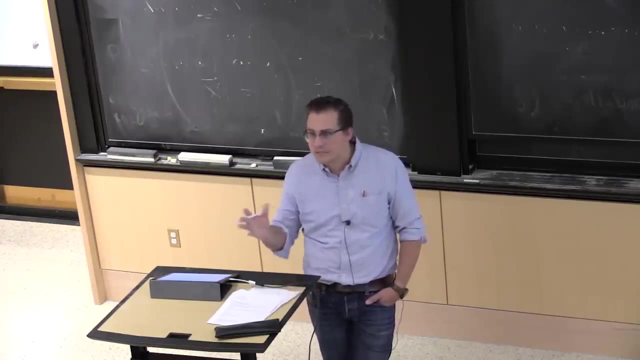 to understand what the limitations are And, when you make conclusions based on data, that those conclusions might be erroneous, for example. More practically, my goal here is to have you ready. So who has taken, for example, a machine learning class here? So many of you, actually Maybe a third, have taken a. 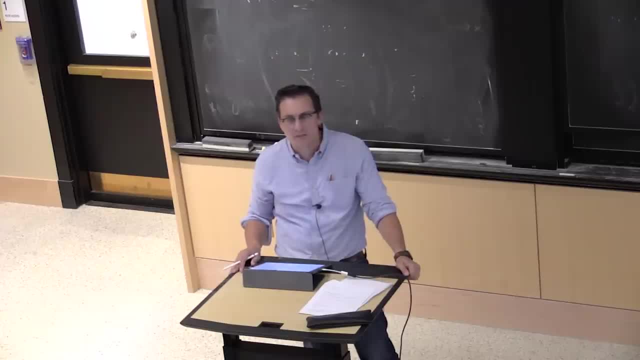 have your own applications. I'm happy to answer questions about specific applications, but rather than trying to tailor applications to an entire institute, I think we're going to work with pretty standard applications. Okay, So I'm going to start with the basic ones, which are the ones that are really not very 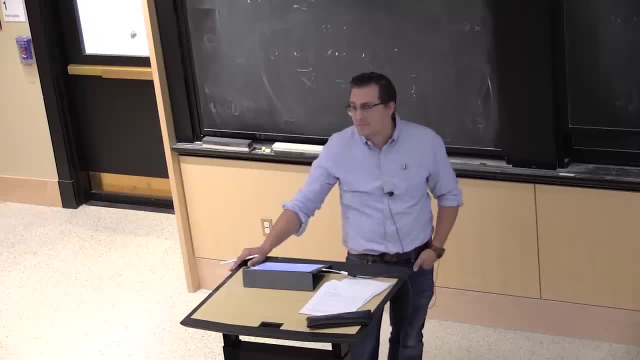 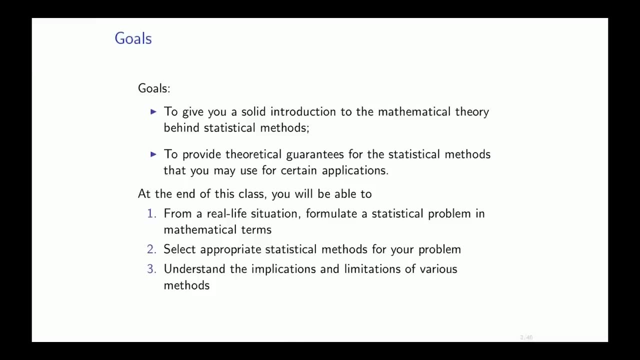 serious ones, and hopefully you'll be able to take the main principles back with you and apply them to your particular problem. So what I'm hoping that you will get out of this class is that when you have a real life situation- and by real life I mean mostly- 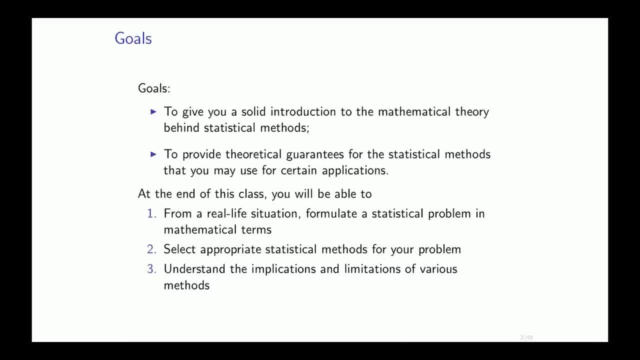 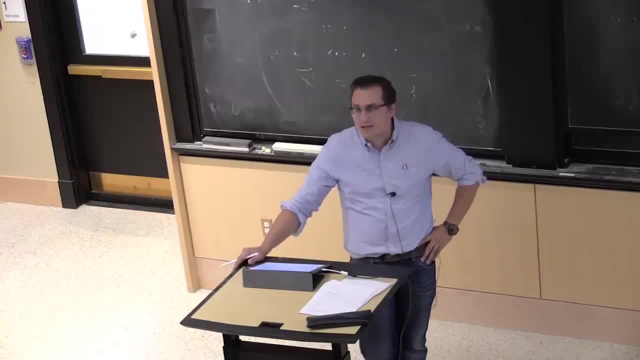 at MIT, so some people probably would not call that real life. the goal is to formulate a statistical problem in mathematical terms. If I want to say, is a drug effective, that's not in mathematical terms. I have to find out which measure I want to have to call it effective. Maybe it's over. 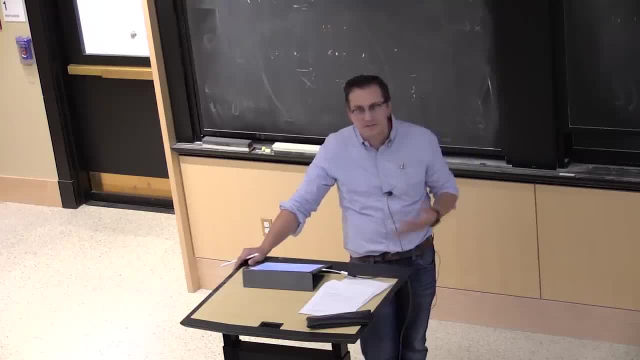 a certain period of time. So there's a lot of things that you actually need, and I'm not really going to tell you how to go from the application to the point you need to be, but I will certainly describe to you what point you need to be at if you want to start. 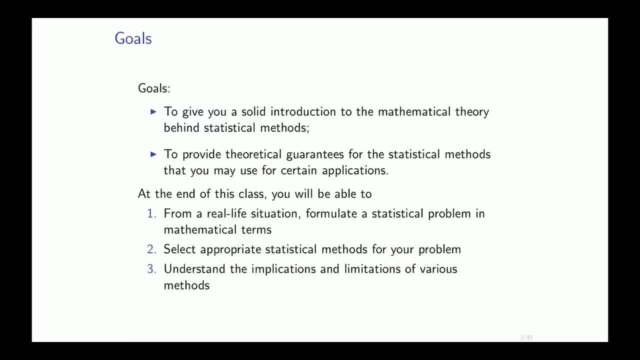 applying statistical methodology. Then, once you understand what kind of question you want to answer, do I want a yes- no answer? Do I want a number? Do I want error bars? Do I want to make predictions five years in the future? Do I have side information or do I? 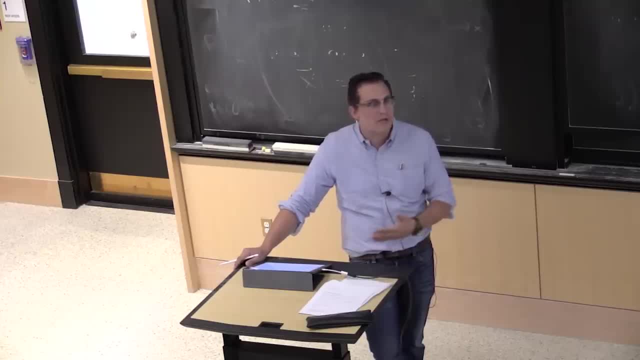 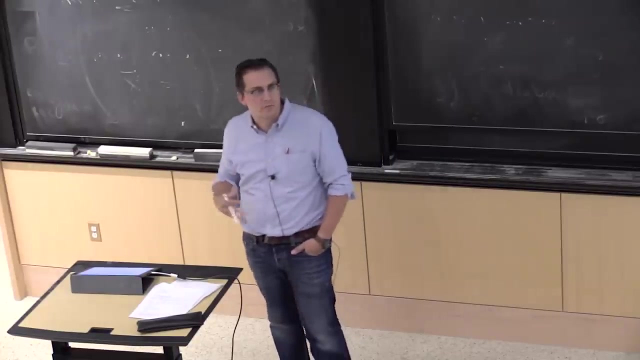 not have side information, All these things. based on that, hopefully, you will have a catalog of statistical methods that you're going to be able to use and apply in the while. And also, no statistical method is perfect. Some of them people have agreed upon over. 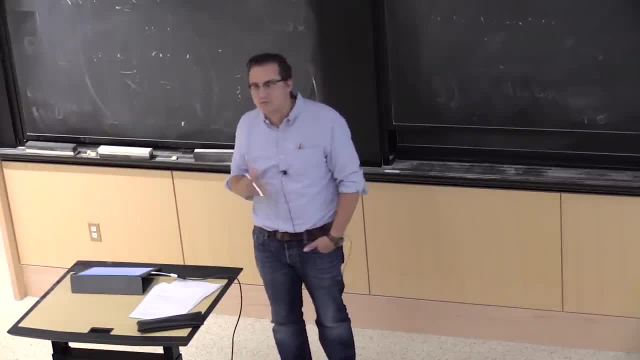 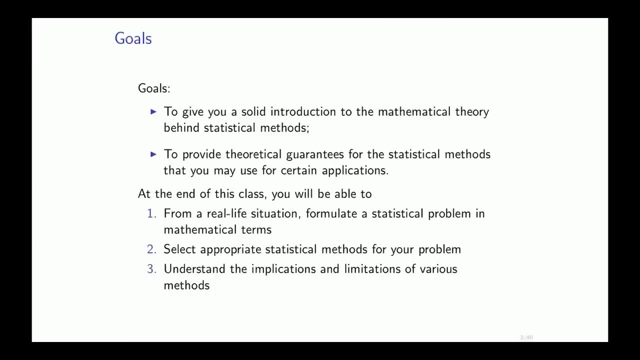 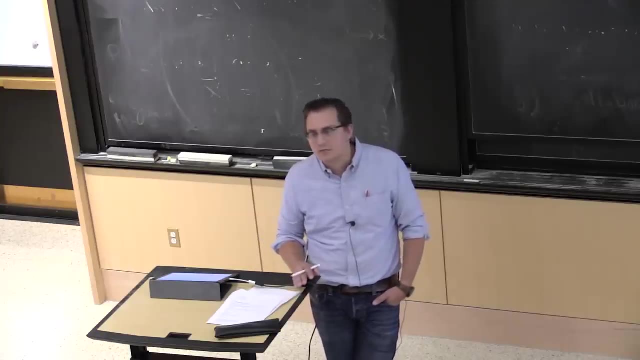 the years and people understand that this is the standard, but I want you to be able to understand what the limitations are And, when you make conclusions based on data, that those conclusions might be erroneous, for example. All right, More practically, my goal here is to have you ready. So who? 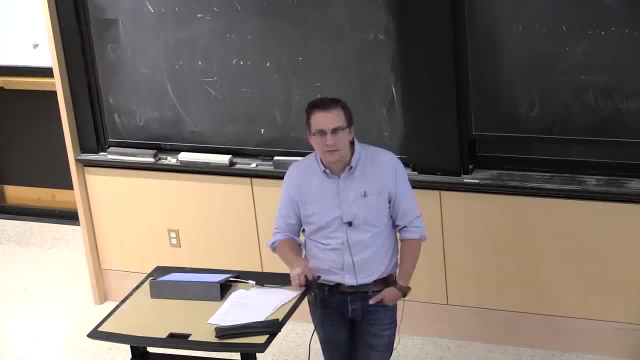 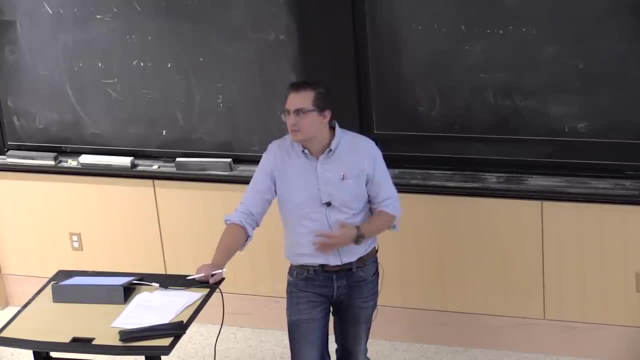 has taken, for example, a machine learning class here. All right, so many of you, actually Maybe a third, have taken a machine learning class. The goal here will be to take you. So statistics have somewhat evolved into machine learning in recent years and my goal is to 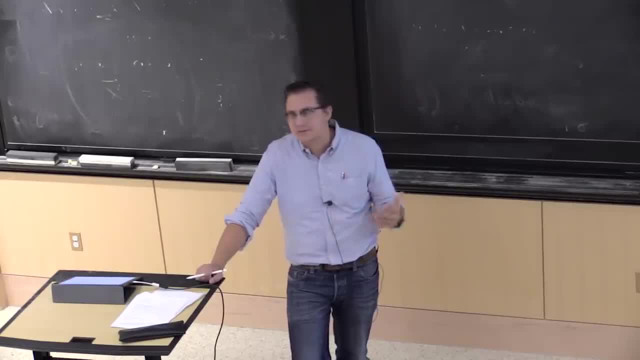 machine learning class. The goal here will be to take you. So statistics have somewhat evolved into machine learning in recent years and my goal is to take you there. So machine learning has a strong algorithmic component. I've taken a machine learning class that displays mostly the algorithmic component, but there's 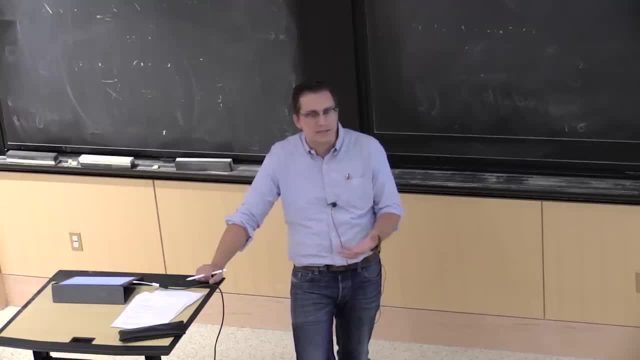 also a statistical component. right, The machine learns from data, And hopefully so this statistical track and there's some statistical learning, which are statistical machine learning classes that you can take here, So they're offered at the graduate level, I believe. 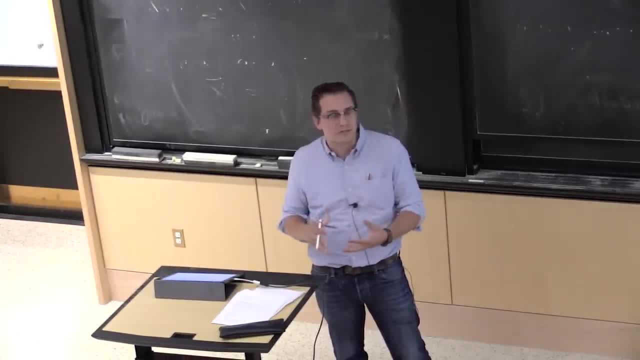 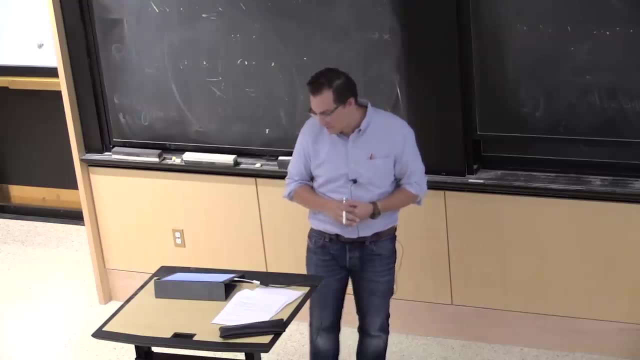 But once you take those classes, I want you to be ready to be able to take those classes, having the statistical fundamentals to understand what you're doing, and then you're going to be able to expand to broader data. So if you're not yet in this universe, you don't know what you're doing. You can use. 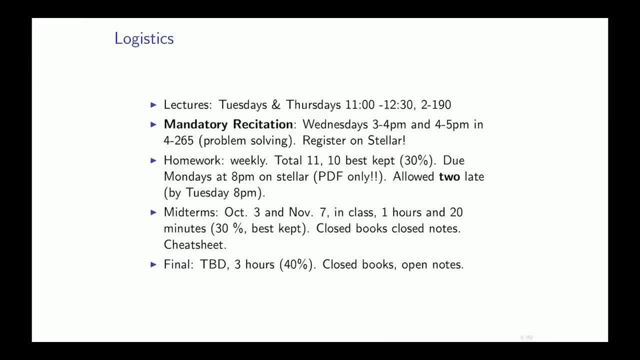 some introduce more of the methods and more sophisticated methods. So lectures are here from 11 to 12.. 30 is on Tuesday and Thursday. Victor Emmanuel will also be- and you can call him Victor- will also be holding mandatory recitation, So please go on, Stellar, and pick. 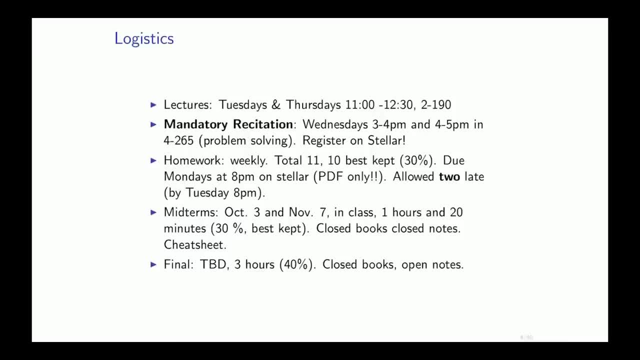 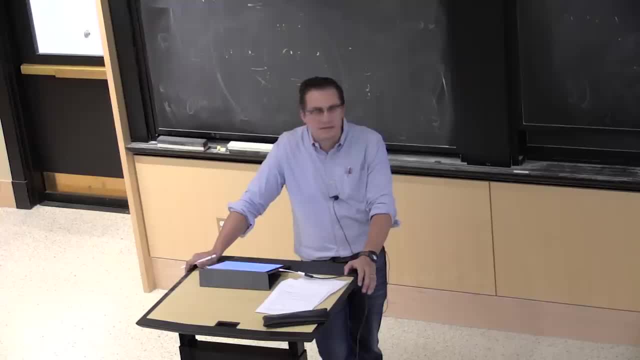 your recitation. It's either three to four or four to five on Wednesdays, and it's going to be mostly focused on problem solving. They're mandatory in the sense that, well, we're all smart, We have a lot of good things, We have a lot of good things and we're going to be 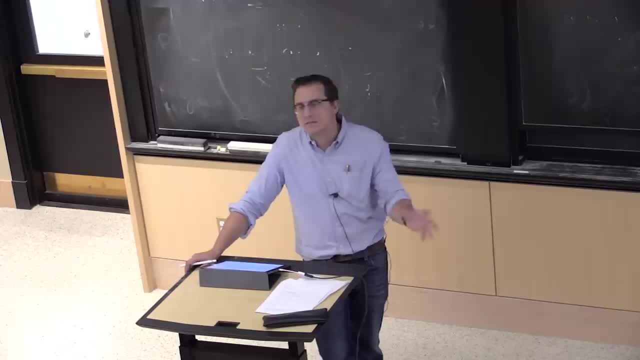 We're allowed to do this. but they're not going to cover entirely new material, but they might cover some techniques that might save you some time when it comes to the exam, So you might get by. so attendance is not going to be taken or anything like this. 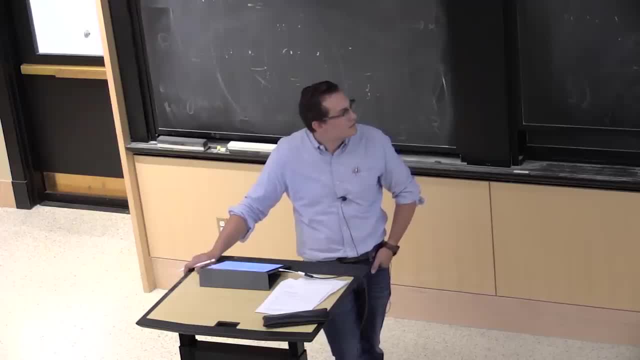 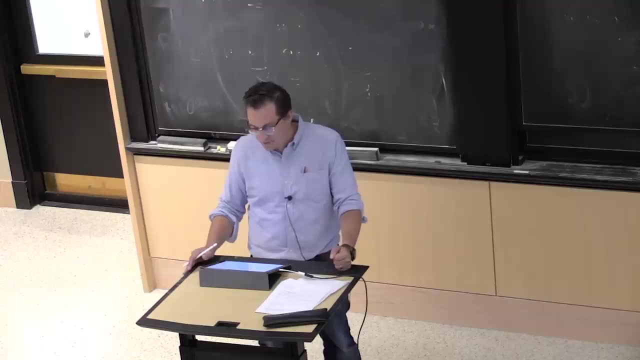 But I highly recommend that you go because, well, they're mandatory, so you cannot really complain that something was taught only in recitation. So please register on Stellar for which of the two recitations you would like to be in. They're capped at 40, so first come, first serve. 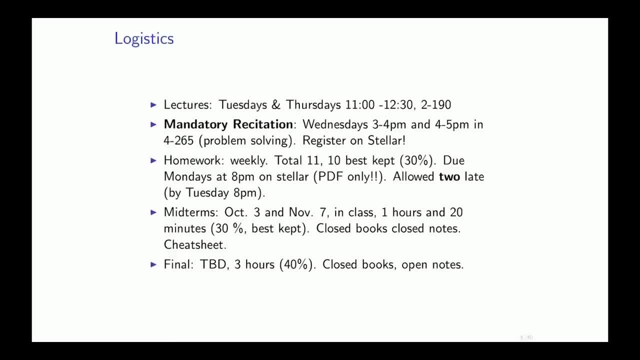 So homework will be due weekly. There's a total of 11 problem sets. I realize this is a lot. Hopefully we'll keep them light. I just want you to not rush too much. The 10 best will be kept, and this: 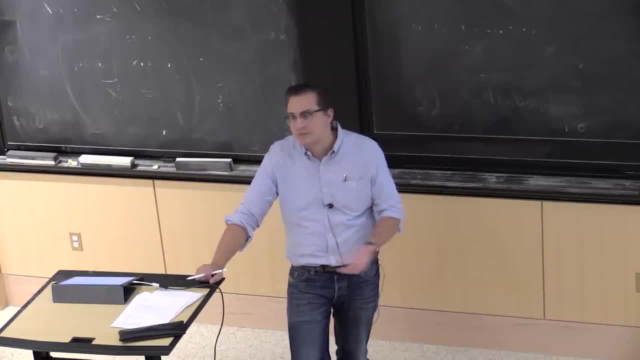 take you there. So machine learning has a strong algorithmic component, so maybe some of you have taken it. Maybe you've taken a machine learning class that displays mostly the algorithmic component, but there's also a statistical component, right, The machine learns from data and hopefully, 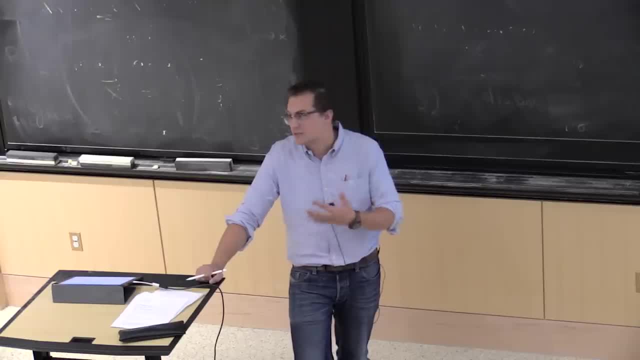 this statistical track and there's some statistical learning, which are statistical machine learning classes that you can take here. so they're offered at the graduate level, I believe. But once you take those classes, I want you to be ready to be able to take those classes. 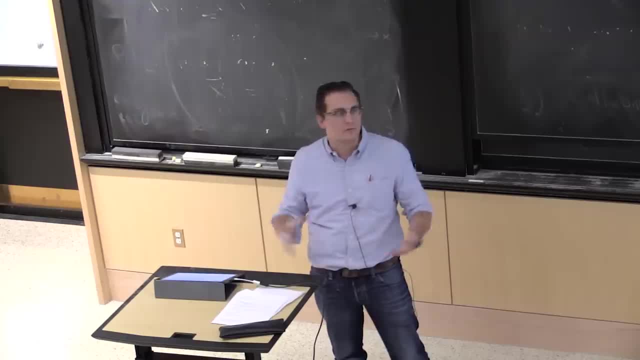 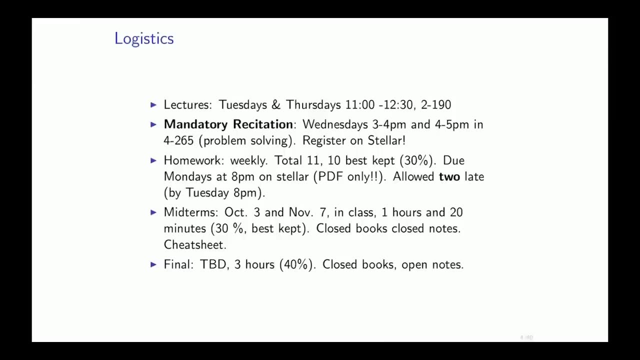 having the statistical fundamentals to understand what you're doing, and then you're going to be able to expand to broader and broader goals, Thank you, and more sophisticated methods. So lectures are here from 11 to 12.30 on Tuesday and Thursday. 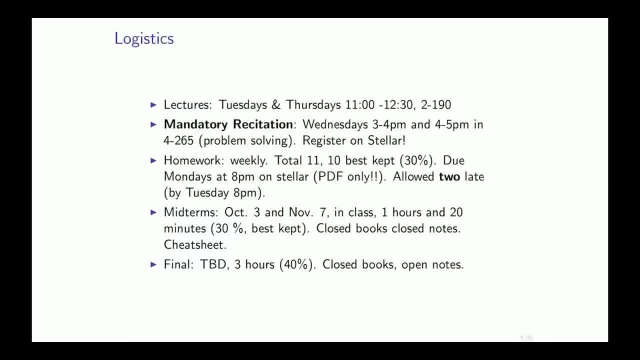 Victor Emmanuel will also be- and you can call him Victor- will also be holding mandatory recitation. So please go on, Stellar, and pick your recitation. It's either 3 to 4 or 4 to 5 on Wednesdays. 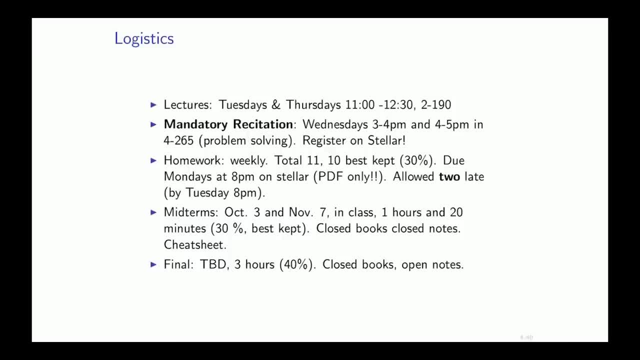 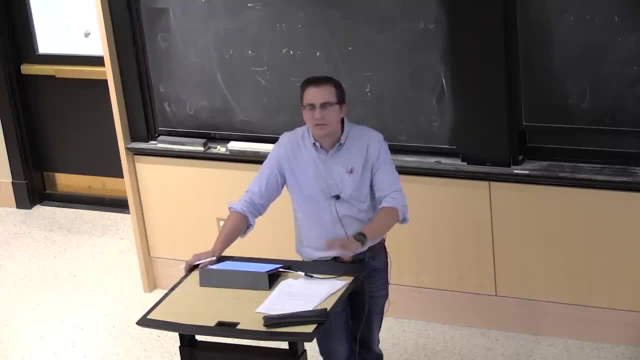 And it's going to be mostly focused on problem solving. They're mandatory in the sense that, well, we're allowed to do this, But they're not going to cover entirely new material, But they might cover some techniques that might save you some time when it comes to the exam. 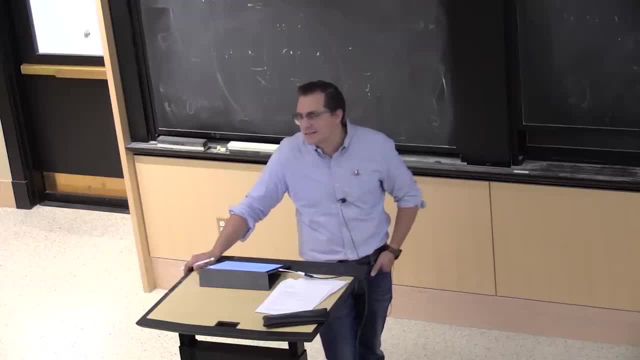 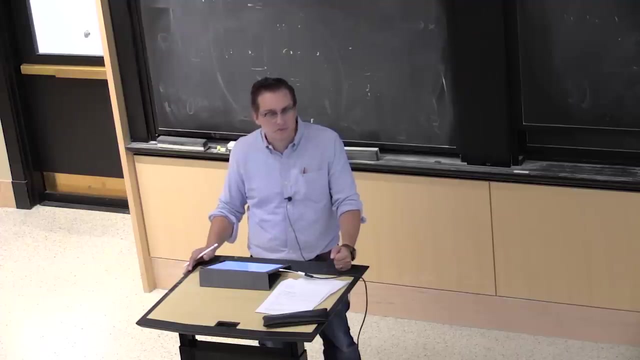 So you might get by. So attendance is not going to be taken or anything like this, But I highly recommend that you go because, well, they're mandatory, So you cannot really complain that something was taught only in recitation. So please register on, Stellar, for which of the two recitations? 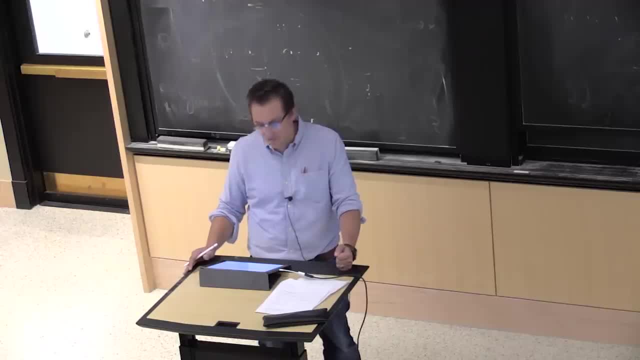 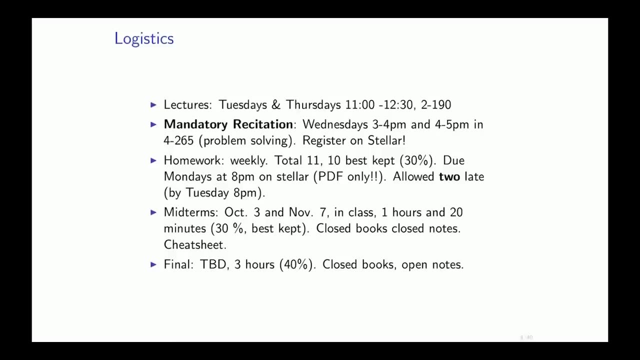 you would like to be in. They're capped at 40, so first come, first serve. So homework will be due weekly. There's a total of 11 problem sets. I realize this is a lot. Hopefully we'll keep them light. 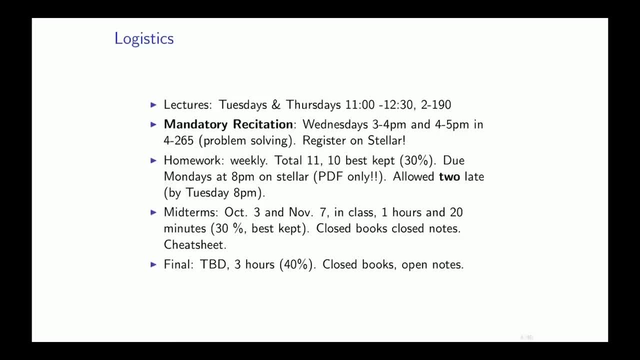 I just want you to not rush too much. The 10 best will be kept, And this will account for a total of 30% of the final grade. They're due Mondays at 8 PM on Stellar, And so this is a new thing. 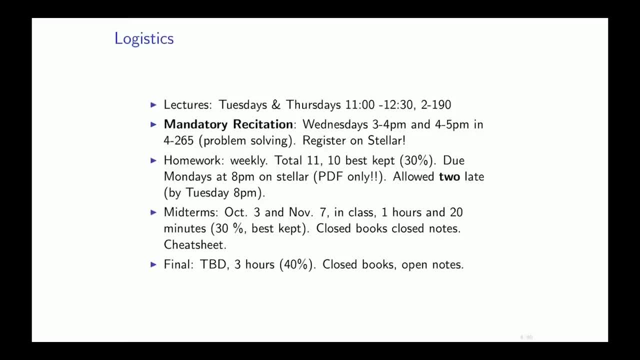 will account for a total of 30% of the final grade. They're due Mondays at 8 PM on Stellar, And so- This is a new thing- We're not going to use the boxes outside of the math department. We're going to use only PDF files. 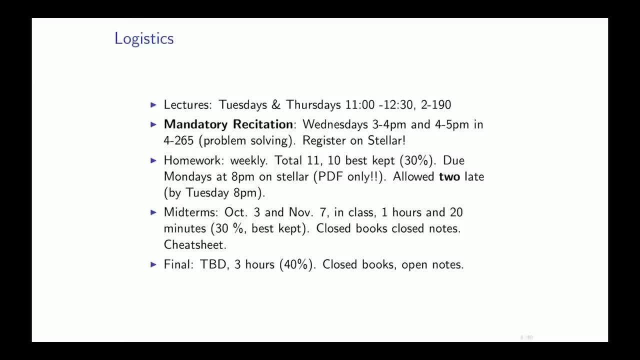 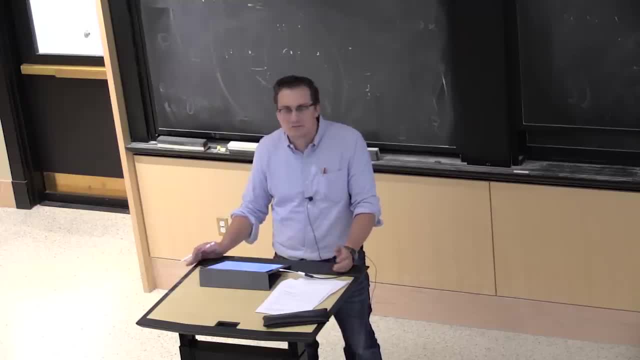 So well. you're always welcome to type them and practice your LaTeX or Word typing. I also understand that this can be a bit of a strain, So just write them down on a piece of paper, Use your iPhone and take a picture of it. 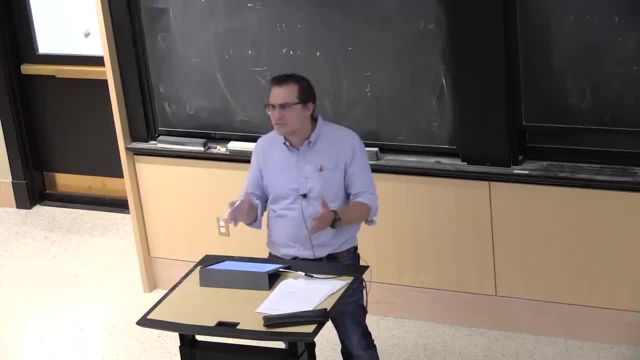 Dropbox has a nice new, So try to find something that puts a lot of contrast, especially if you use pencil, Because we're going to check if they're readable, OK, So this is your responsibility: to have a readable file In particular. so I've had over the years 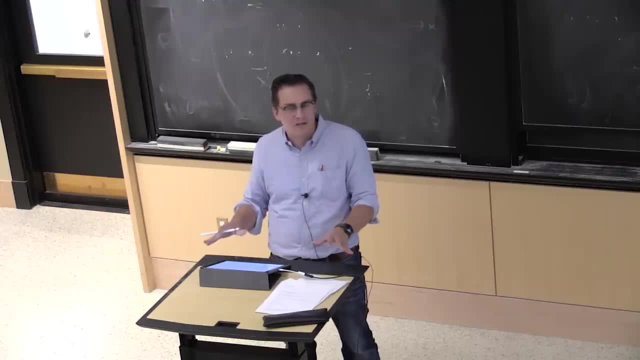 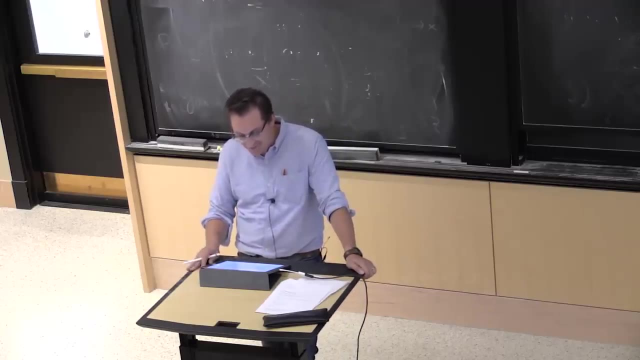 OK, not at MIT, I must admit, But I've had students who actually write a doc file and think that converting it to a PDF consists in erasing the extension DOC and replacing it by PDF. This is not how it works, And so I'm sure you will figure it out. 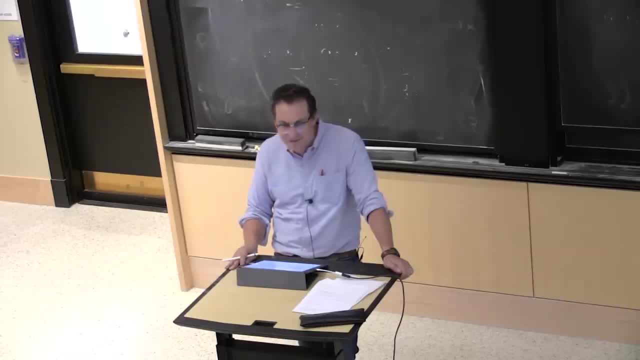 Please try to keep them letter sized. This is not a strict requirement, but I don't want to see thumbnails either. You're allowed to have two late homeworks, And by late I mean 24 hours late. OK, No questions asked. 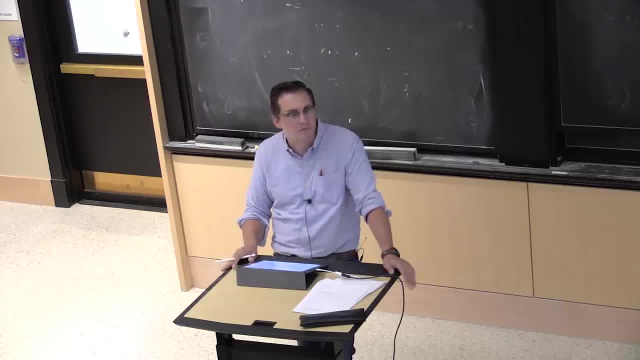 You submit them, This will be counted. You don't have to send an email to warn us or anything like this. Beyond that, it's going to be given that you have one slack for one zero grade and slack for two late homeworks. 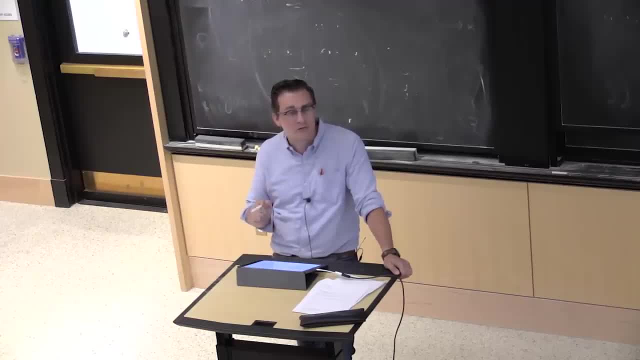 you're going to have to come up with very good explanation why you need actually more extensions than that, if you ever do. In particular, you're going to have to keep track about why you've used your three options. So you have to keep track of what you've used in the last two. 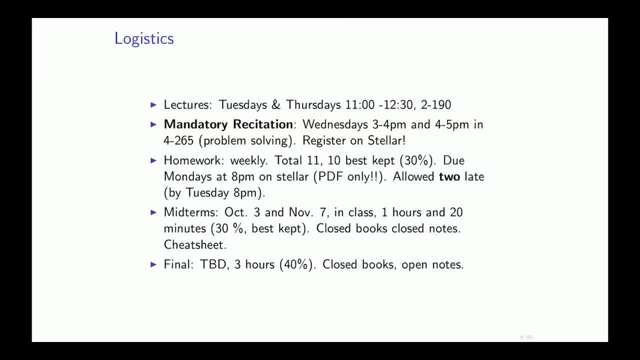 or three months before. There's going to be two midterms: One is October 3rd and one is November 7.. They're both going to be in class for the duration of the lecture, When I say they last for an hour and 20 minutes. 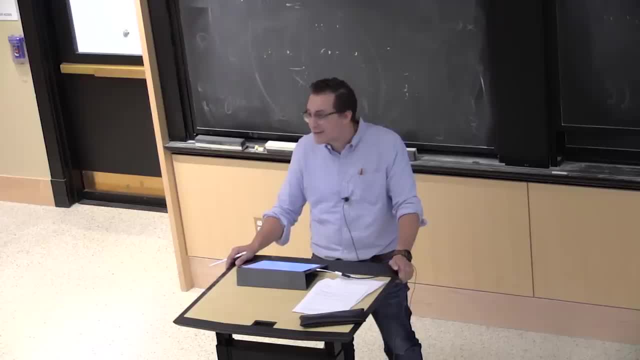 it does not mean that if you arrive 10 minutes before the end of lecture, you still get an hour and 20 minutes. It will end at the end of lecture time. For this as well, no pressure. Only the best of the two will be kept. 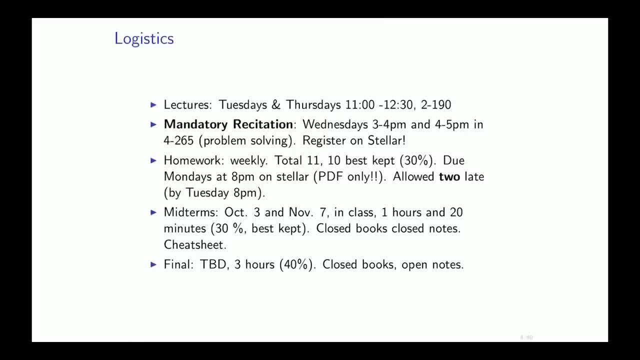 We're not going to use the boxes outside of the math department. We're going to use only PDF files, So you're always welcome to type them and practice your LaTeX or Word typing. I also understand that this can be a bit of a strain. 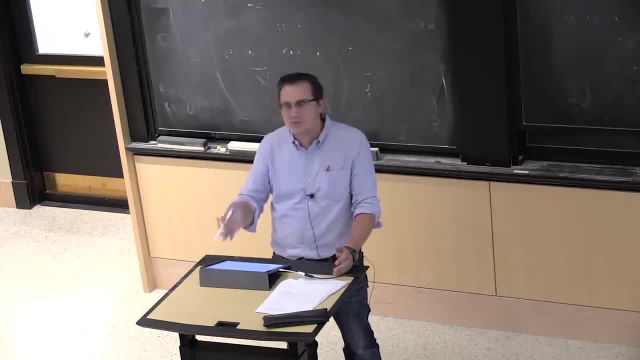 So just write them down on a piece of paper, Use your iPhone and take a picture of it. Dropbox has a nice new, So try to find something that puts a lot of contrast, especially if you use pencil, Because we're going to check if they're readable. 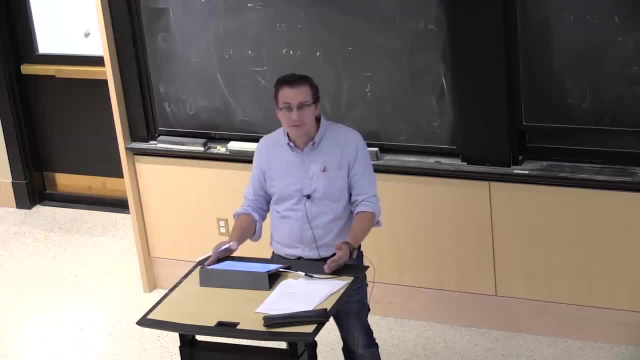 And this is your responsibility. It's your responsibility to have a readable file In particular. so I've had over the years- OK, not at MIT, I must admit, but I've had students who actually write a doc file and think that converting it to a PDF. 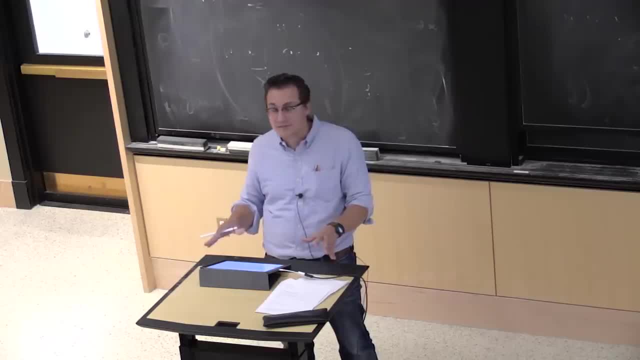 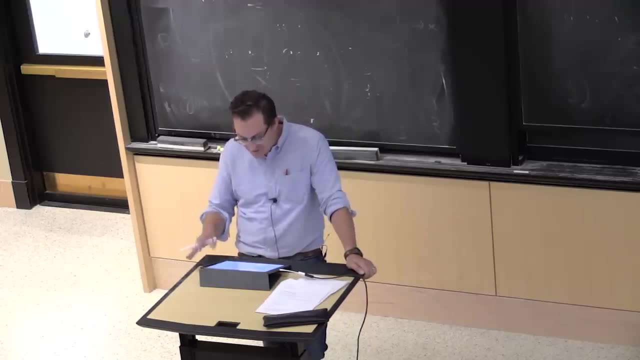 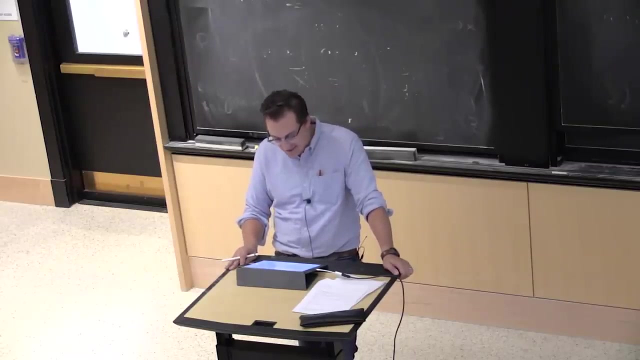 consists in erasing the extension DOC and replacing it by PDF. This is not how it works, And so I'm sure you will figure it out. Please try to keep them letter sized. This is not a strict requirement, but I don't want to see thumbnails either. 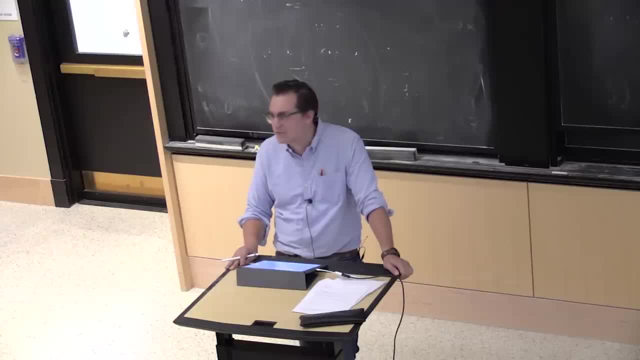 You are allowed to have two, Two late homeworks, And by late I mean 24 hours late. OK, No questions asked. You submit them, This will be counted. You don't have to send an email to warn us or anything like this. 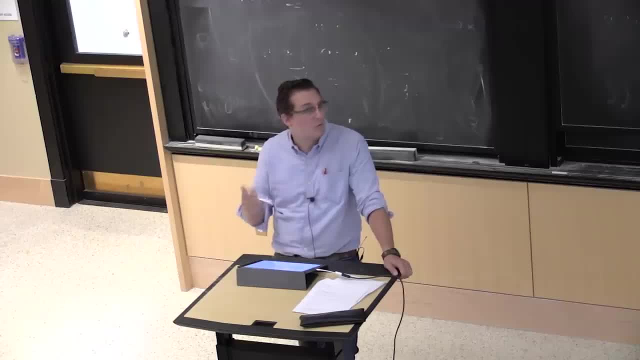 Beyond that, it's going to be given that you have one slack for one zero grade and slack for two late homeworks. you're going to have to come up with very good explanation why you need actually more extensions than that, if you ever do. 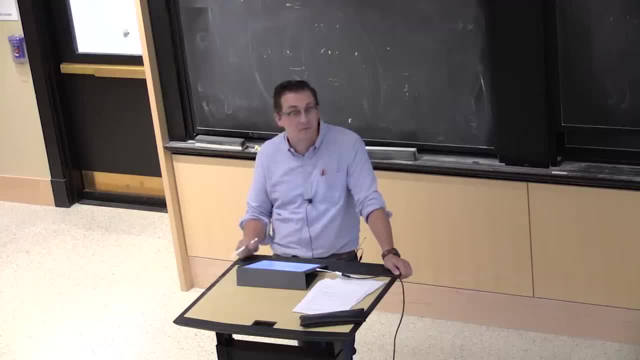 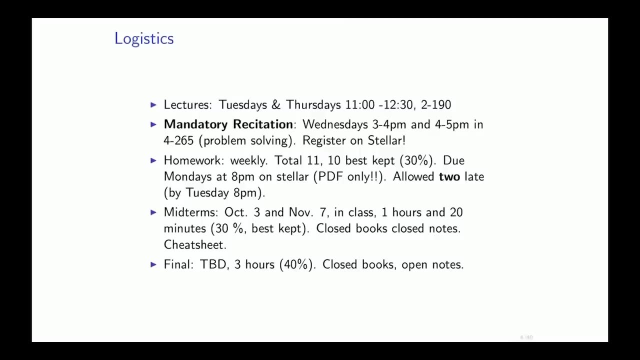 In particular, you're going to have to keep track about why you've used your three options before. There's going to be two midterms: One is October 3rd and one is November 7.. They're both going to be in class for duration of the lecture. 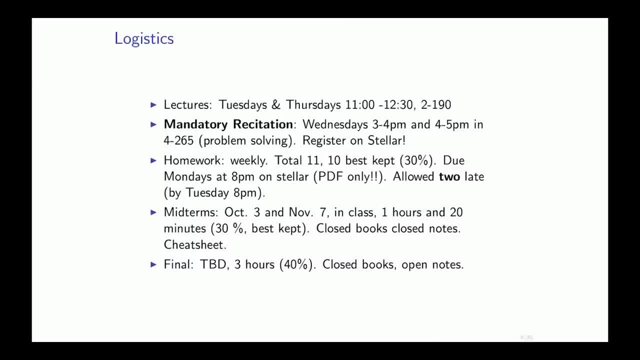 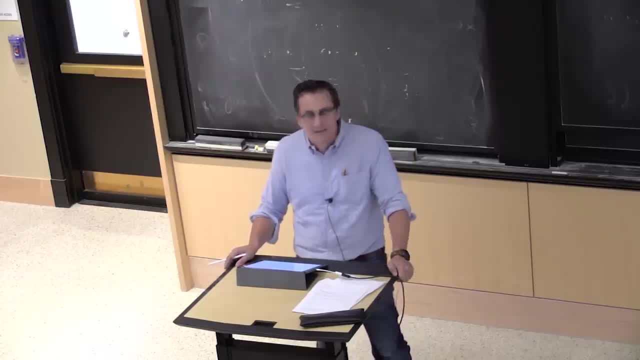 When I say they last for an hour and 20 minutes, it does not mean that if you arrive 10 minutes before the end of lecture, you still get an hour and 20 minutes. It will end at the end of lecture time For this as well, no pressure. 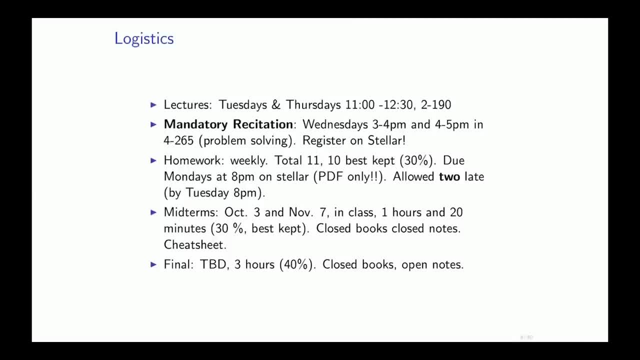 Only the best of the two will be kept And this grade will count for 30% of the grade. This will be closed books And closed notes. So the purpose is for you to Yes, How many midterms did you say there are? 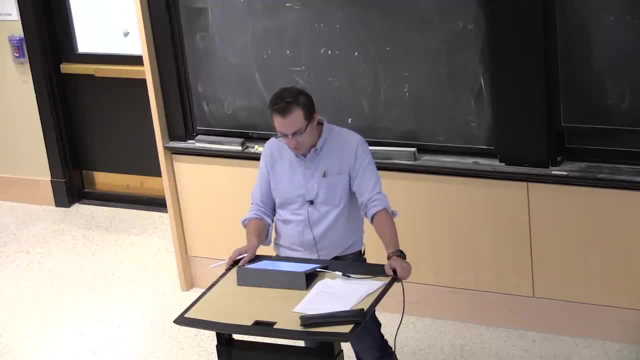 PHILIPPE RIGOLLET- Two: You said the best of the two will be kept. PHILIPPE RIGOLLET- I said the best of the two will be kept. yes, Suppose the midterms will be kept. 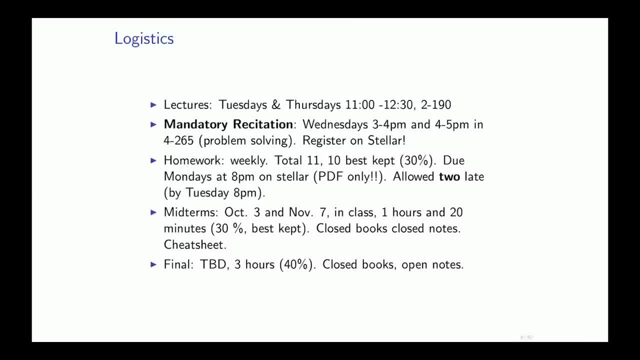 And this grade will count for 30% of the grade. There will be closed books and closed notes. So the purpose is for you to yes. How many midterms did you say there are? PHILIPPE RIGOLLET- Two. 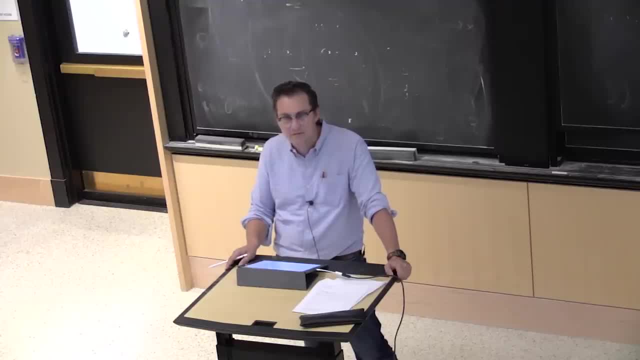 You said the best of the two will be kept. PHILIPPE RIGOLLET- I said the best of the two will be kept. yes, Suppose the midterms will be kept. PHILIPPE RIGOLLET- The best of the two, not the best two. 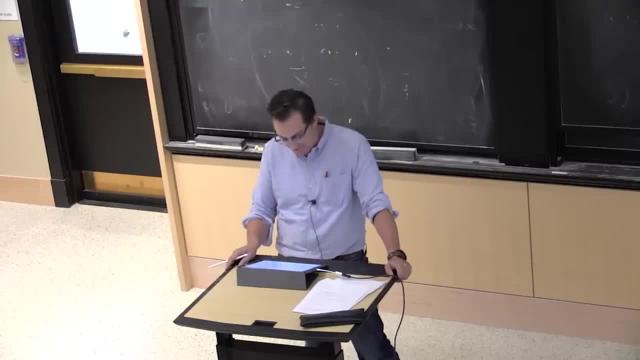 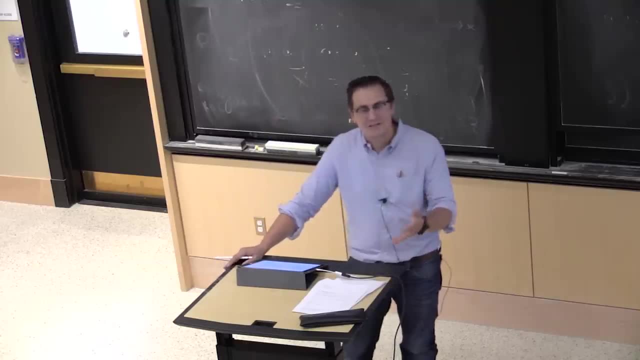 All right, We will add them. multiply the number by 9, and that will be your grade. So I am trying to be nice. There is just a limit to what I can do, All right. so the goal is for you to learn things. 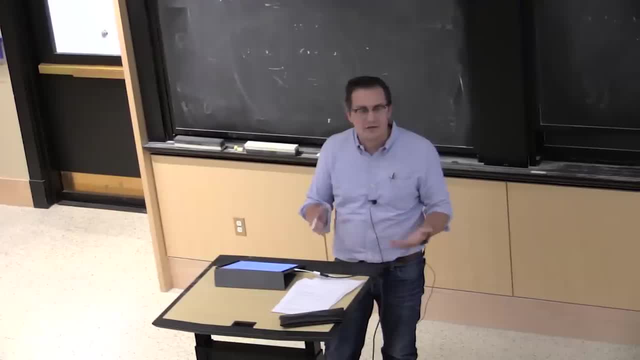 and to be familiar with them. In the final, you will be allowed to have your notes with you, But the midterms are also a way for you to develop some mechanisms so that you don't actually waste too much time on things that you should be able to do. 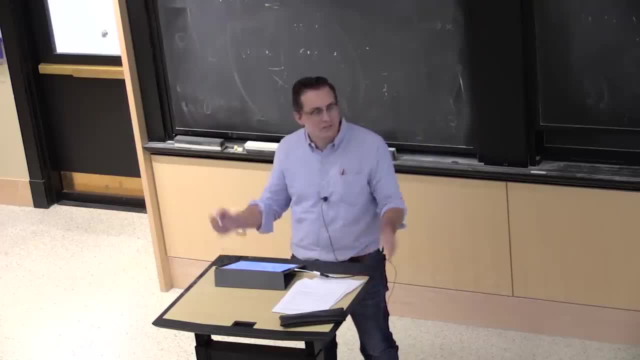 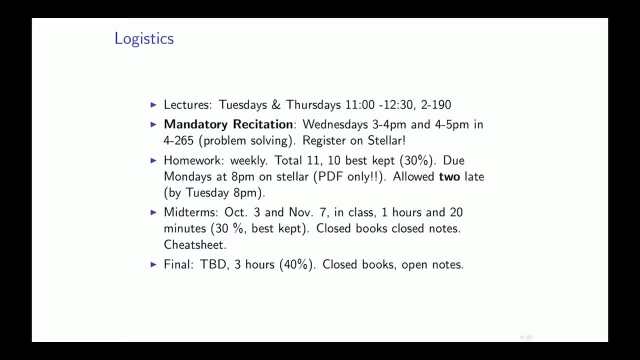 without thinking too much. You will be allowed a cheat sheet- because, well, you can always forget something, And there will be a two-sided letter sheet and you can practice yourself as writing as small as you want, And you can put whatever you want on this cheat sheet. 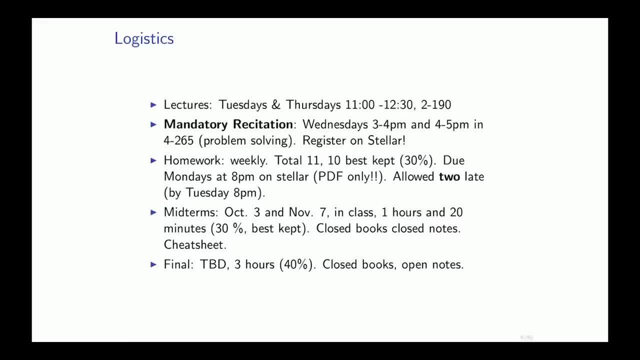 All right, the final will be decided by the register. It's going to be three hours and it's going to count for 40%. You cannot bring books, but you can bring your notes. Yes, I noticed that the midterms today. 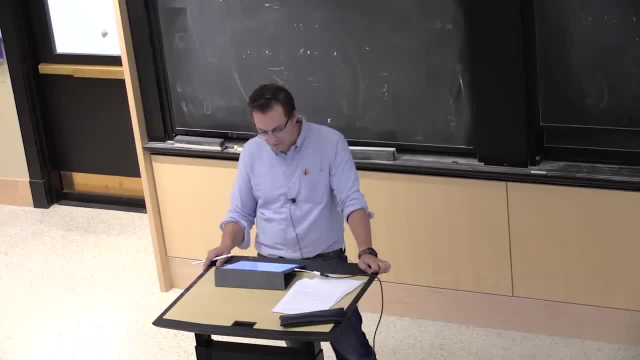 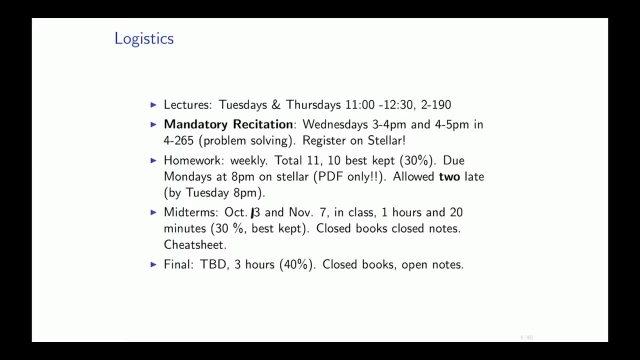 have a syllabus. PHILIPPE RIGOLLET- They're not. Yeah. PHILIPPE RIGOLLET- Oh yeah, there's one that's missing on both of them, isn't there? You're a bust. 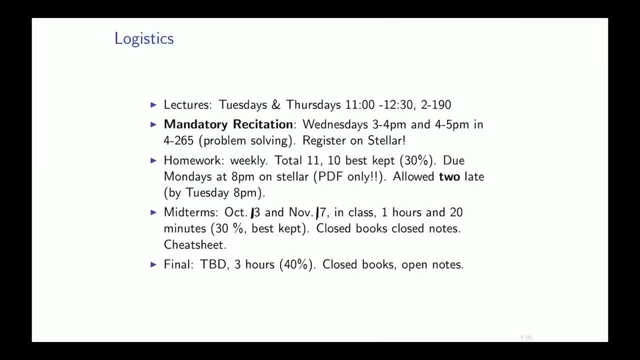 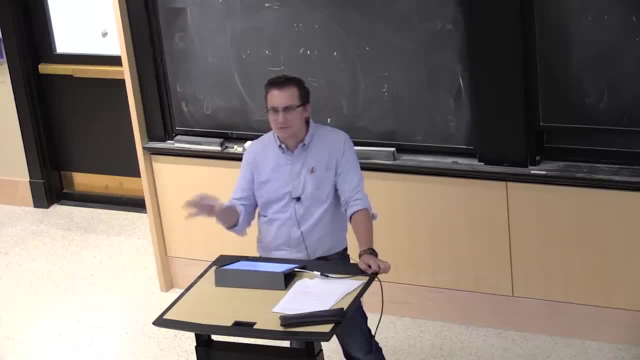 PHILIPPE RIGOLLET- Yeah, Let's figure that out. The syllabus is the true one. The slides are so that we can discuss, But the ones that's on the syllabus is the one that counts, And I think they're also posted on the calendar on Stellar. 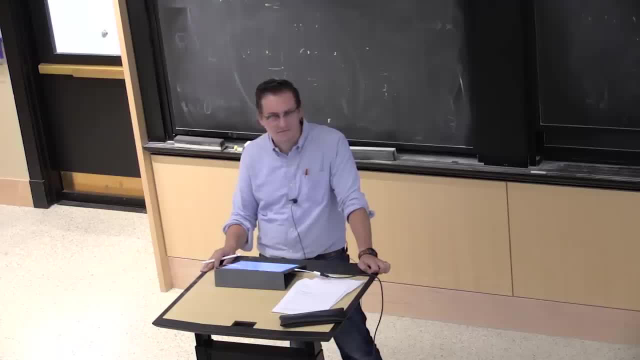 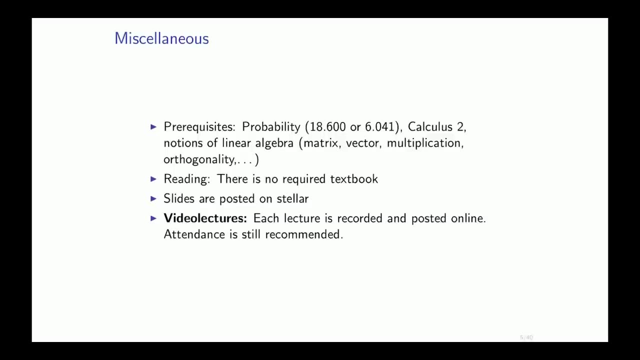 as well. Any other question? OK, so the prereqs here and who has looked at the first problem set already. So those hands that are raised realize that there is a true prerequisite of probability for this class. It can be at the level of 1,800,, 600, or 6041. 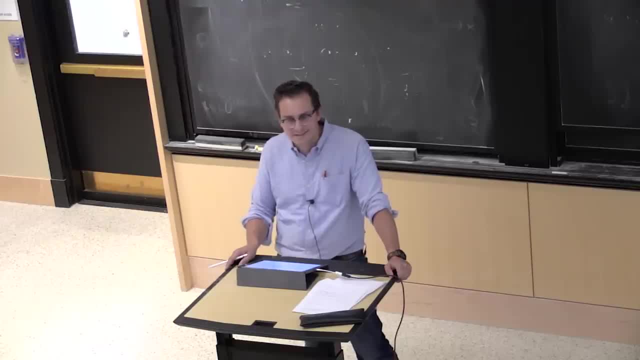 PHILIPPE RIGOLLET- The best of the two, not the best two. We will add them. multiply the number by 9, and that will be your grade. So I am trying to be nice, There's just a limit. 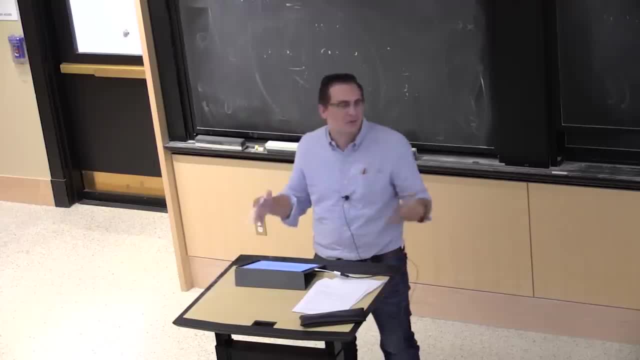 PHILIPPE RIGOLLET- Yeah, there's a limit to what I can do. The goal is for you to learn things and to be familiar with them. In the final, you will be allowed to have your notes with you. 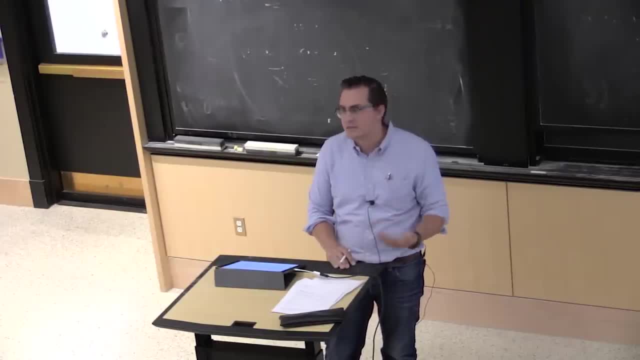 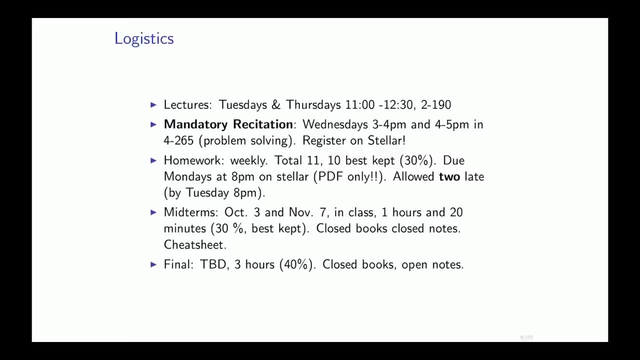 But the midterms are also a way for you to develop some mechanisms so that you don't actually waste too much time on things that you should be able to do without thinking too much. You will be allowed a cheat sheet, because you can always forget something. 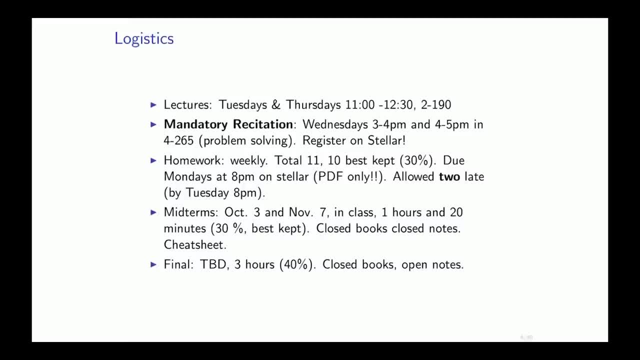 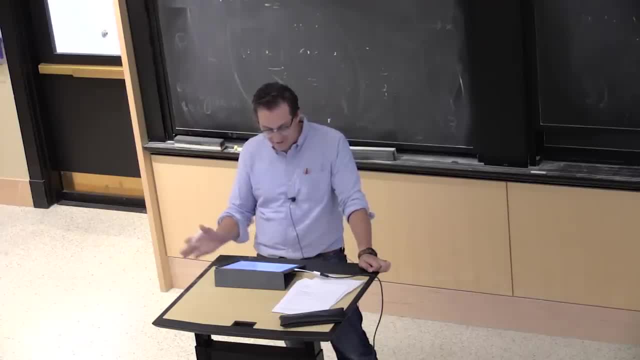 And there will be a two-sided letter sheet And you can practice yourself as writing as small as you want, And you can put whatever you want on this cheat sheet. All right, the final will be decided by the register. It's going to be three hours and it's going to count for 40%. 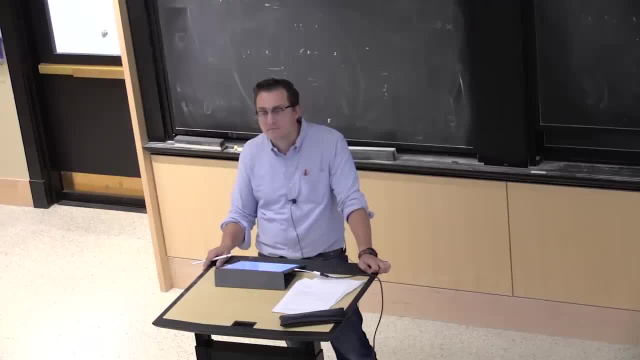 You cannot bring books, but you can bring your notes. Yes, I noticed that the midterms don't have a syllabus. PHILIPPE RIGOLLET- They're not. Yeah, PHILIPPE RIGOLLET- Oh yeah, there's. 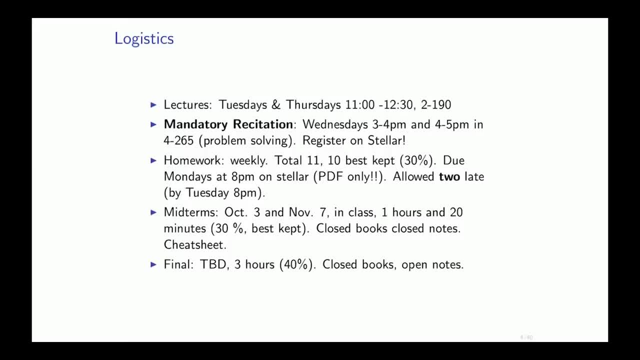 one that's missing on both of them isn't there. That's too bad. I think it was a good idea to not do it. PHILIPPE RIGOLLET- Yeah, OK, PHILIPPE RIGOLLET- Yeah. 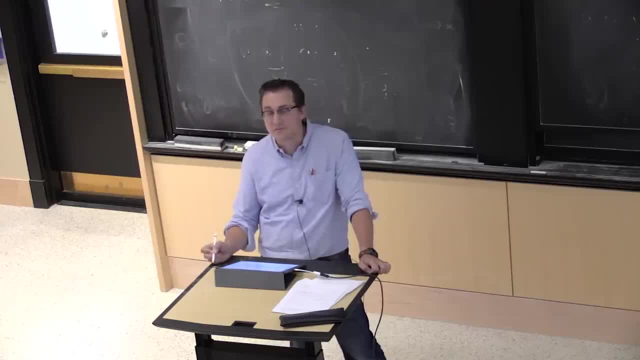 Let's figure that out. The syllabus is the true one. The slides are so that we can discuss, But the ones that's on the syllabus is the one that counts, And I think they're also posted on the calendar on Stellar as well. 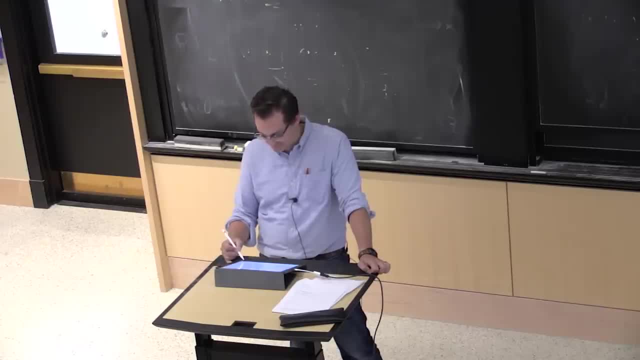 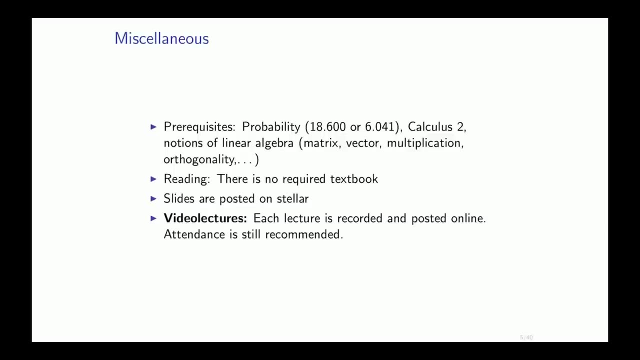 Any other question? OK, so the prereqs here, And who has looked at the first problem set already. OK, so those hands that are raised realize that there is a true prerequisite of probability for this class. It can be at the level of 1,800,, 600, or 6041. 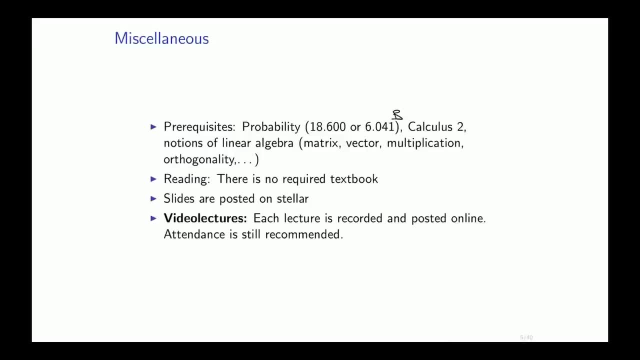 I should say B, Now it's two classes. I will require you to know some calculus and have some notions of linear algebra, such as what is a matrix, what is a vector, how do you multiply those things together, and some notion of what orthogonal vectors are. 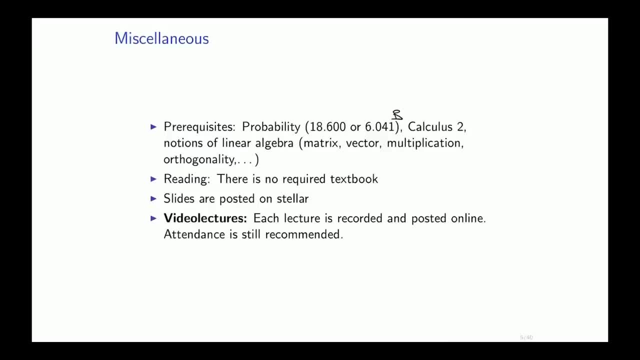 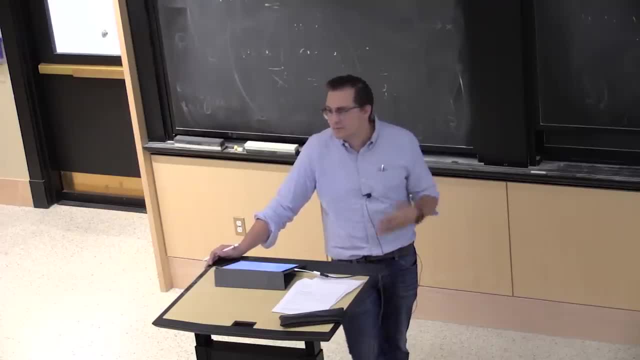 And I'll remind you about. so we'll talk about eigenvectors and eigenvalues, but I'll remind you all of that. So this is not a strict prereq, But if you've taken it for example, doesn't hurt to go back to your notes. 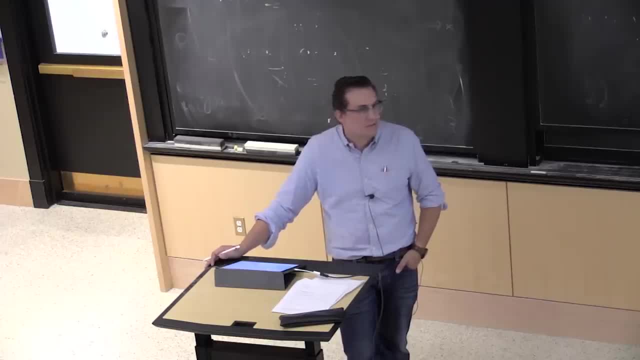 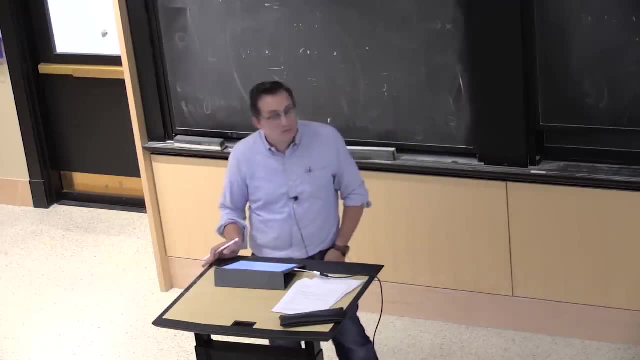 when we get closer to this chapter on principal component analysis. And the chapters as they're listed in the syllabus are in order, So you will see when it actually comes. So there's no required textbook, And I know this is a bit of a I mean. 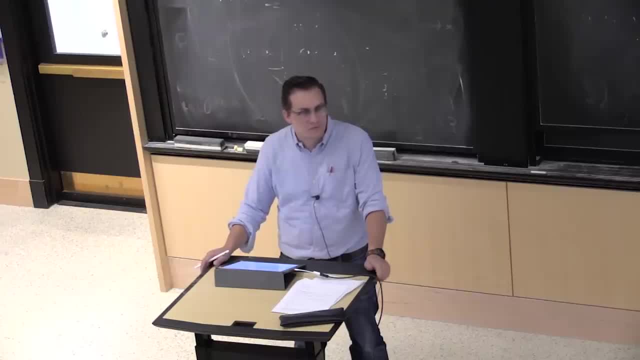 I know you tend to not like that. You like to have your textbook to know where you're going and what we're doing. I'm sorry it's just this class. Either I would have to go to a mathematical statistics textbook, which is just too much. 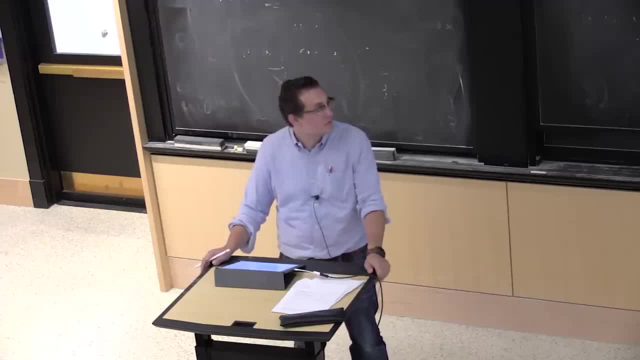 or to go to a more engineering type statistics class, which is just too little. So hopefully the problems that will be enough for you to practice the recitations will have some problems to solve as well, and the material will be posted on the slides. 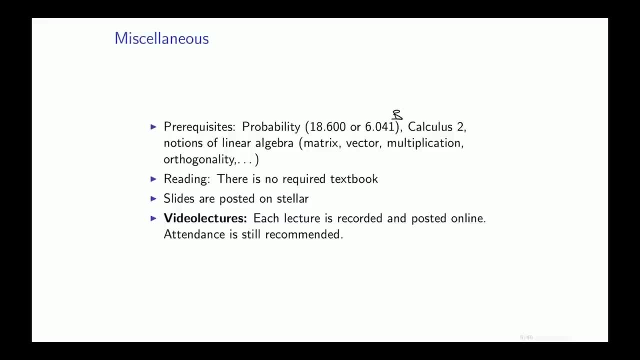 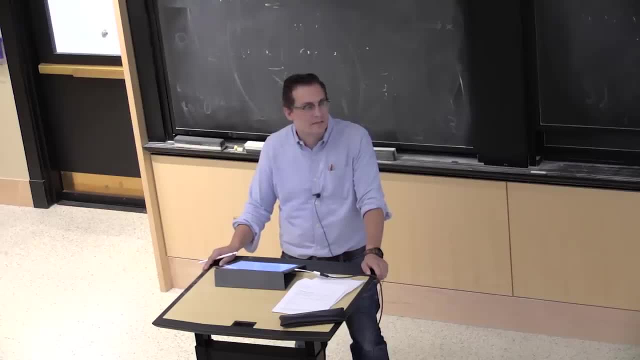 So you should have everything you need. There's plenty of resources online if you want to expand on a particular topic or read it said by somebody else. The book that I recommend in the syllabus is this book called All of Statistics by Wasserman. 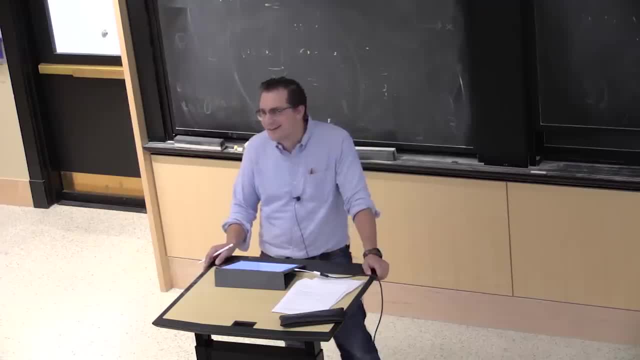 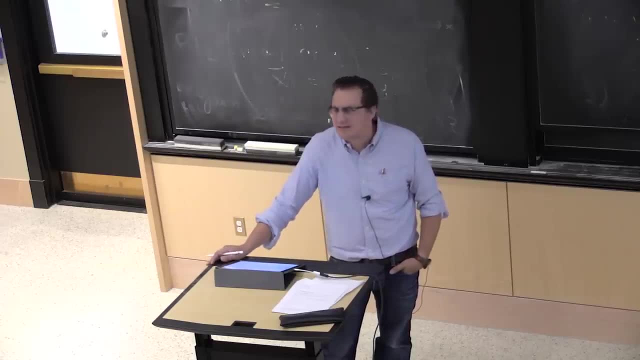 mainly because of the title. I'm guessing it has all of it in it. It's pretty broad. There's actually not that many. It's more of an intro-grad level, but it's. it's not very deep, but you see a lot of the overview. 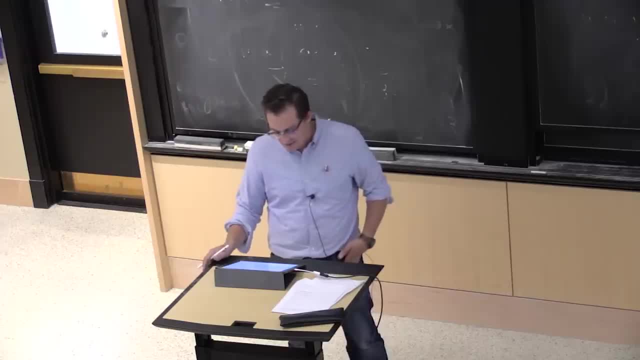 Certainly, what we're going to cover will be a subset of what's in there, So the slides will be posted on Stellar before lectures, before we start a new chapter and after we're done with the chapter, with the annotations and also with typos corrected, like for the exam. 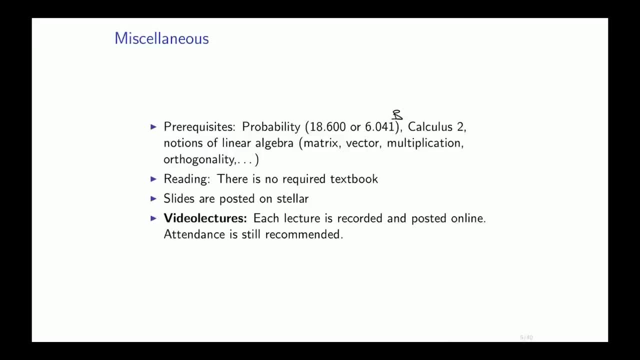 I should say B. Now it's two classes. I will require you to know some calculus and have some notions of linear algebra, such as: what is a matrix? what is a vector? how do you multiply those things together? some notion of what are there. 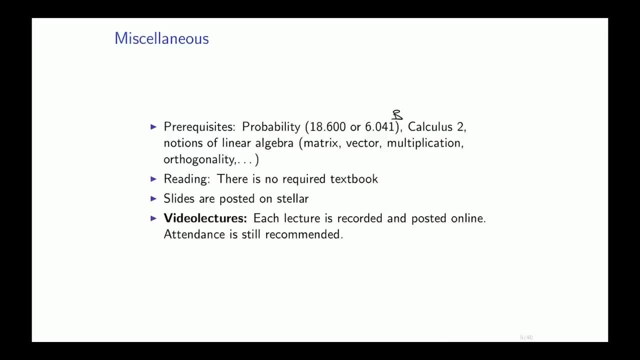 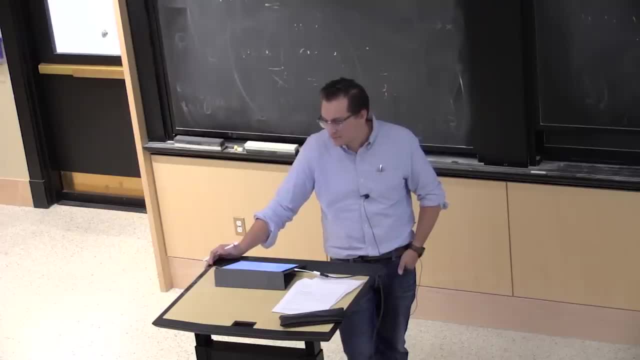 PHILIPPE RIGOLLET- Yeah, And then I'll remind you of the general vectors And I'll remind you about- so we'll talk about- eigenvectors and eigenvalues, But I'll remind you all of that. So this is not a strict prereq. 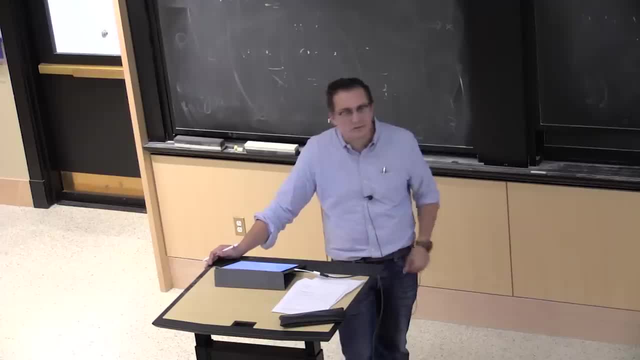 But if you've taken it for example, doesn't hurt to go back to your notes when we get closer to this chapter. on principal component analysis. The chapters as they're listed in the syllabus are in order, So you will see when it actually comes. 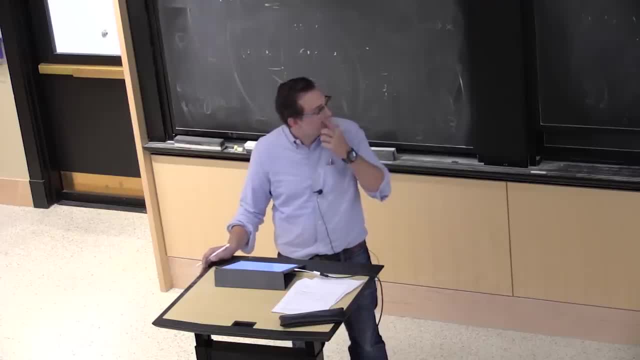 So there's no required textbook- And I know this is a bit of a- I mean, I know you tend to not like that. You like to have your textbook to know where you're going and what we're doing. I'm sorry, it's just this class. 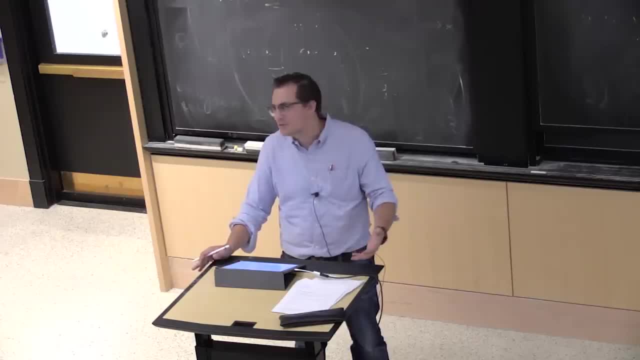 Either I would have to go to a mathematical statistics textbook, which is just too much, or to go to a more engineering type statistics class, which is just too little. So hopefully the problems that will be enough for you to practice. the recitations will have some problems to solve. 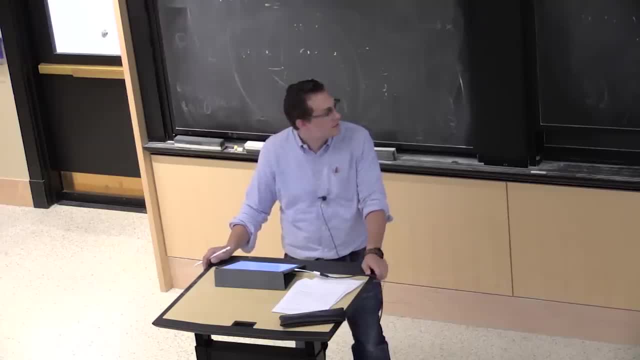 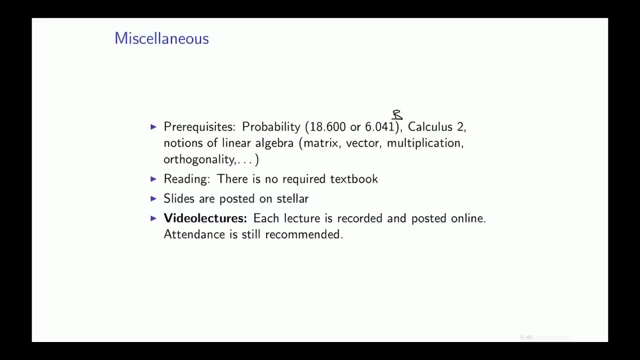 as well, And the material will be posted on the slides, So you should have everything you need. There's plenty of resources online if you want to expand on a particular topic or read it said by somebody else. The book that I recommend in the syllabus: 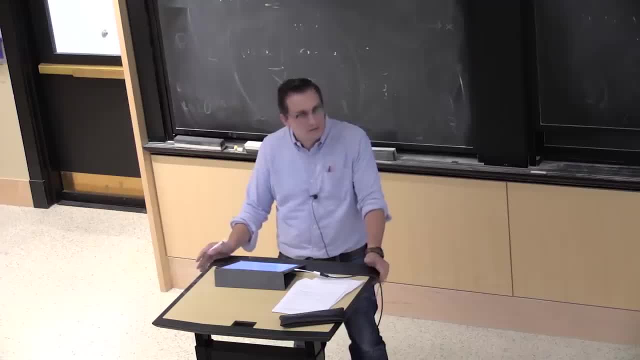 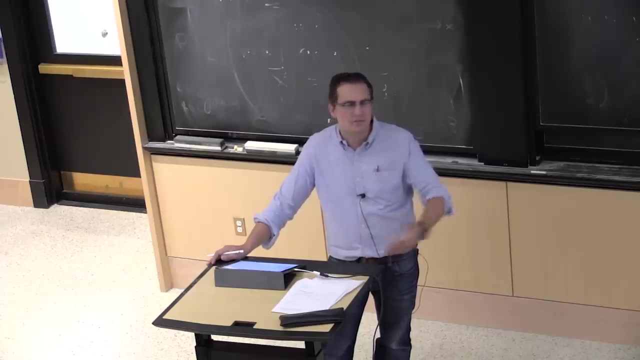 is this book called All of Statistics by Wasserman? mainly because of the title, I'm guessing it has all of it in it. It's pretty broad. There's actually not that many, It's more of an intro grad level But it's not very deep. but you see a lot of the overview. 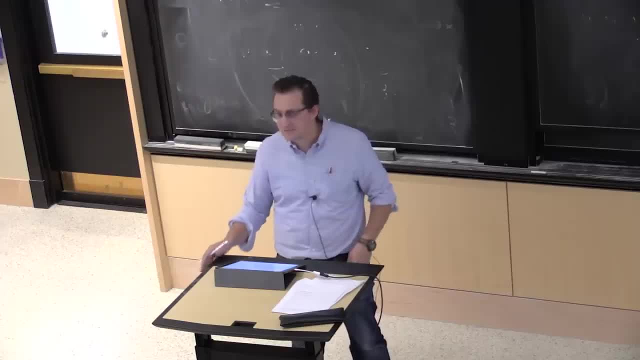 And certainly what we're going to cover will be a subset of what's in there. So the slides will be posted on Stellar before lectures, before we start a new chapter and after we're done with the chapter, with the annotations and also with typos corrected, like for the exam. 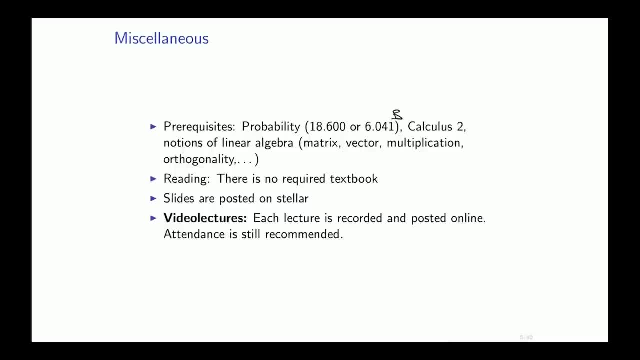 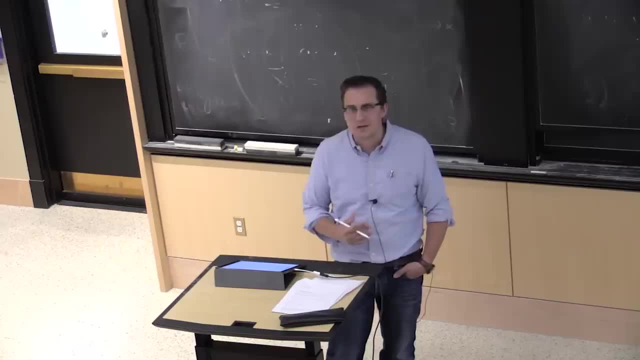 So there will be some video lectures Again. the first one will be posted on OCW from last year, but all of them will be available And Stellar, of course modulo technical problems, But hopefully this is an automated system And hopefully it won't work out well for us. 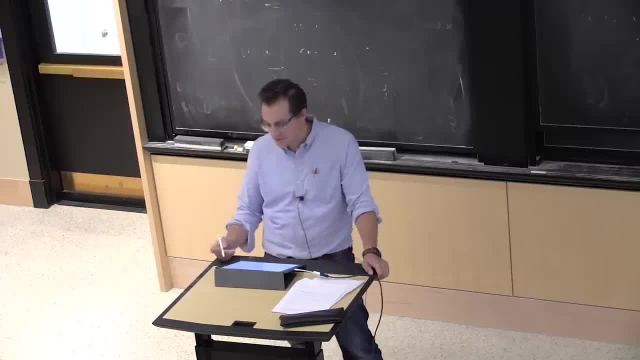 So if you somehow have to miss a lecture, you can always catch it up by watching it. You can also play it at speed 0.75, in case I end up speaking too fast. But I think I've managed myself so far, All right. so just last warning. 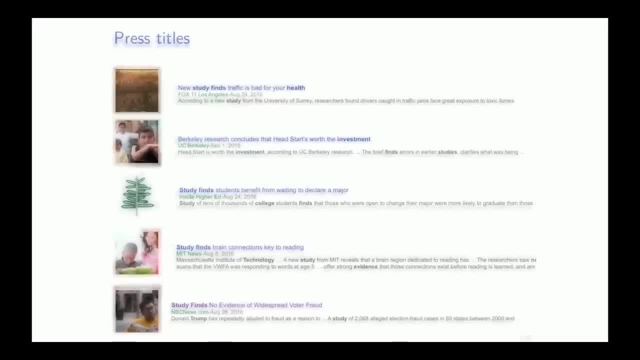 All right. so why should you study statistics? Well, If you read the news, you will see a lot of statistics. I mentioned machine learning. It's built on a lot of statistics. Statistics is now. if I were to teach this class 10 years ago. 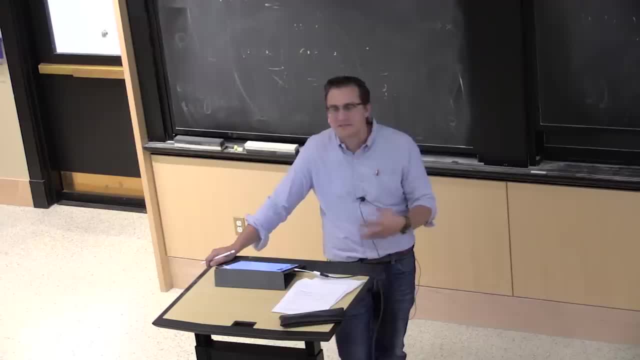 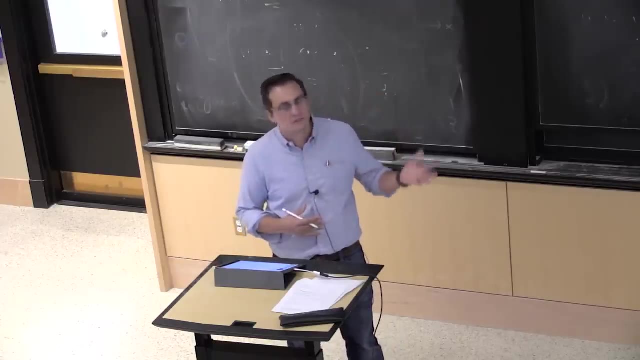 I would have to explain to you that data collection and making decisions based on data was something that made sense, But now it's almost in our life. We're used to this idea that data helps making decisions, And so people use data to conduct studies. 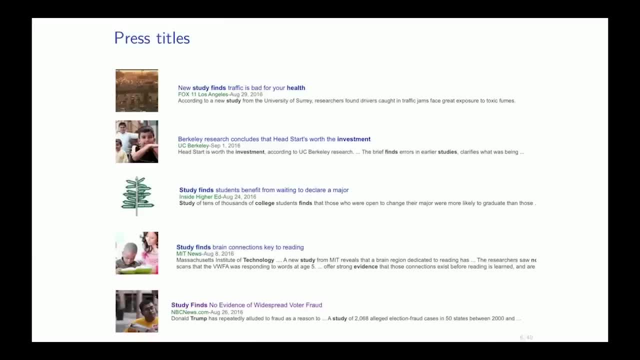 So here I found a bunch of press titles that I think the keyword I was looking for was study finds. if I want to do this, So this. I actually did not bother doing it again This year. this is all: 2016,, 2016,, 2016.. 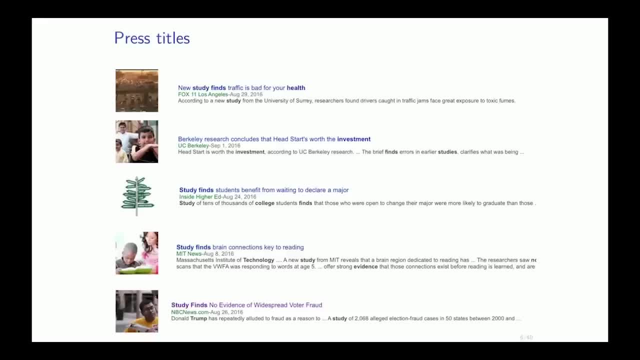 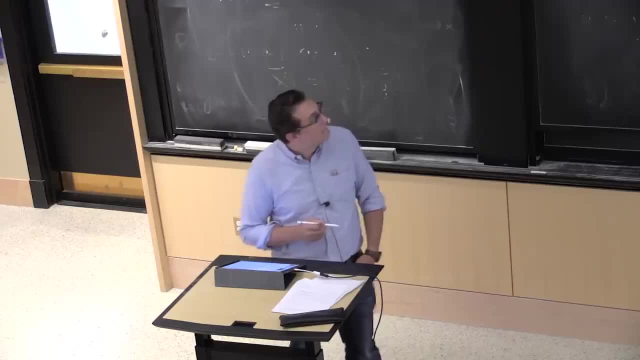 But the keyword that I look for is usually study finds. So a new study find: traffic is bad for your health. So we had to wait 2016 for data to tell us that, And there's a bunch of other more, slightly more. 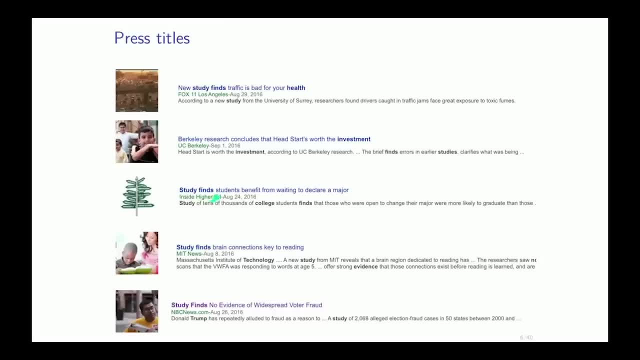 interesting ones. For example, one that you might find interesting is that the study finds that students benefiting benefit from you know waiting to declare a major. Now there's a bunch of press titles, one that studies, you know one in the MIT News that studies. 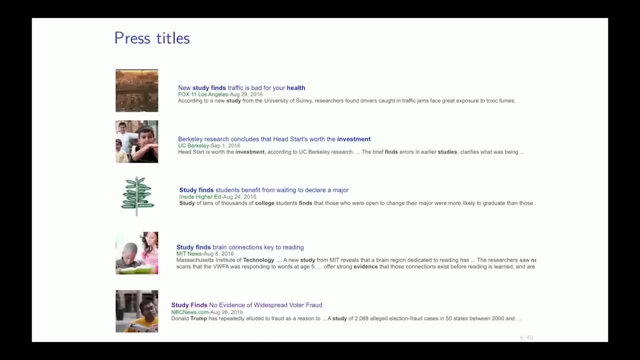 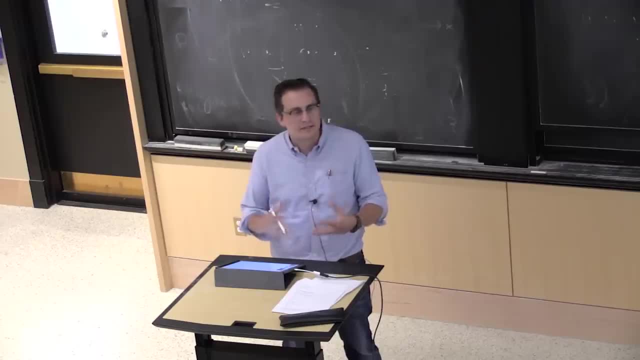 finds brain connections key to reading. And so here we sort of have an idea of what happened there. Some data was collected, Some scientific hypothesis was formulated, And then the data was here to try to prove or disprove the scientific hypothesis. That's the usual scientific process. 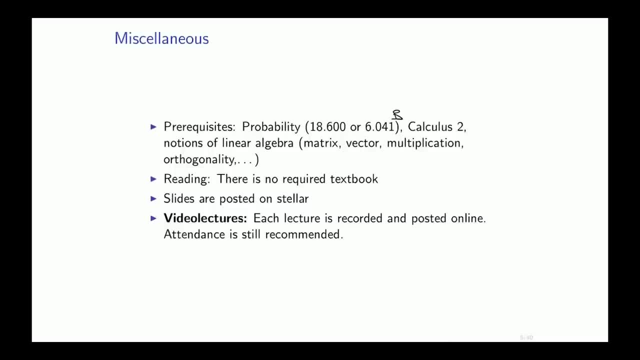 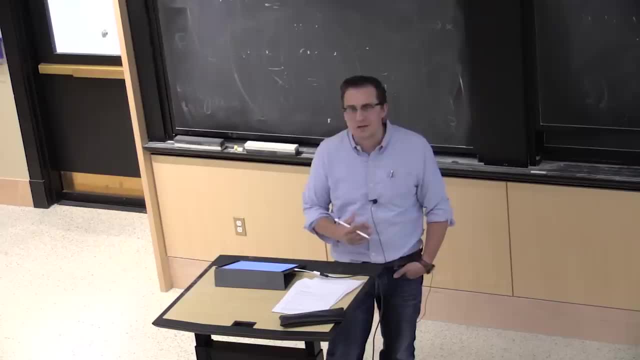 So there will be some video lectures Again. the first one will be posted on OCW from last year, But all of them will be available on Stellar. of course, Modulo. There will be some technical problems, But hopefully this is an automated system. 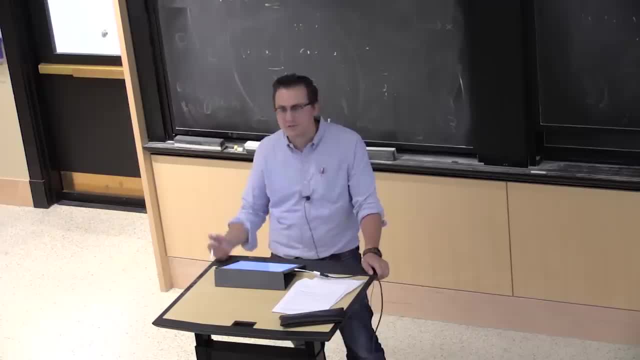 And hopefully it won't work out well for us. So if you somehow have to miss a lecture, you can always catch it up by watching it. You can also play it at speed 0.75 in case I end up speaking too fast. 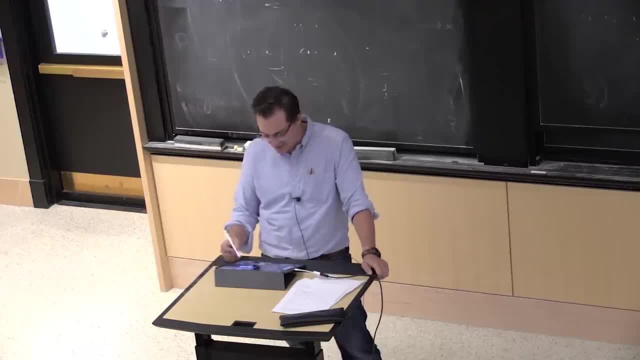 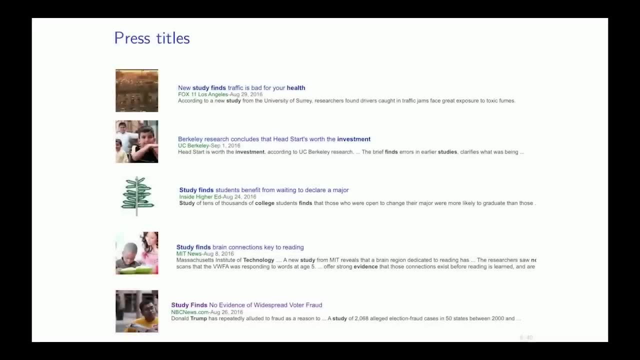 But I think I've managed myself so far, All right. so just last warning, All right, so why should you study statistics? Well, if you read the news, you will see a lot of statistics. So why? Why should you study statistics? 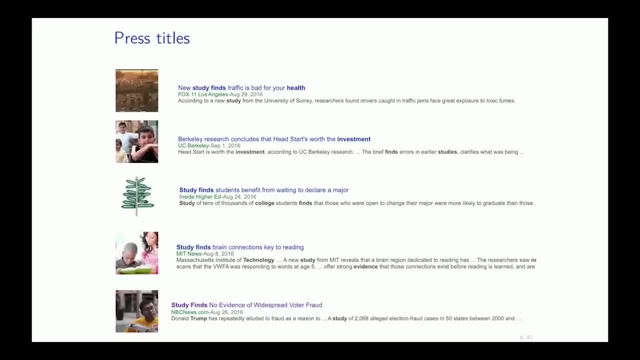 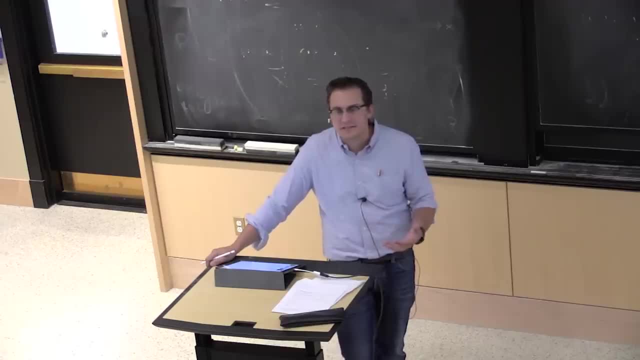 I mentioned machine learning. It's built on a lot of statistics. Statistics is now. if I were to teach this class 10 years ago, I would have to explain to you that data collection and making decisions based on data was something that made sense. 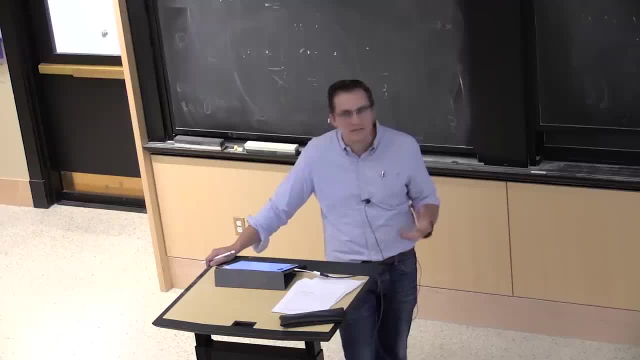 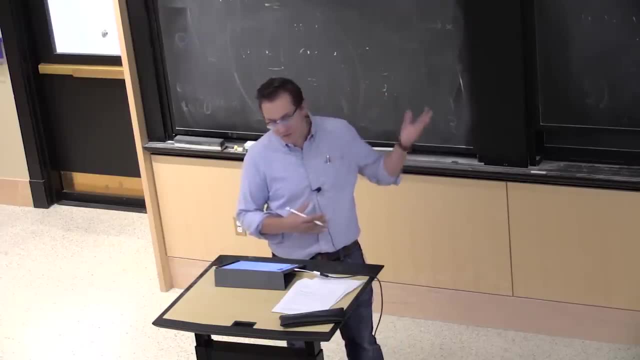 But now it's almost in our life. We're used to this idea that data helps making decisions, And so people use data to conduct studies. So here I found a bunch of press titles that I think I was looking for was study finds. if I want to do this, 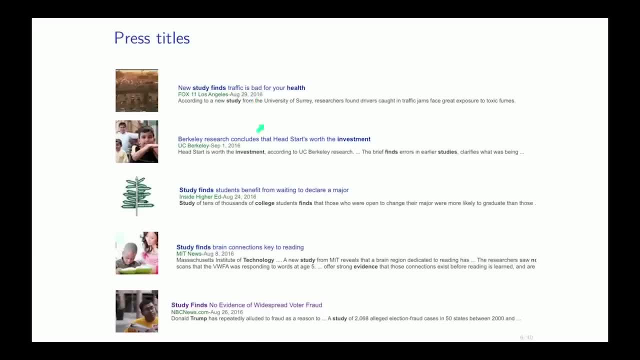 So this I actually did not bother doing it again This year. this is all 2016,, 2016,, 2016.. But the keyword that I look for is usually study finds. So a new study find: traffic is bad for your health. 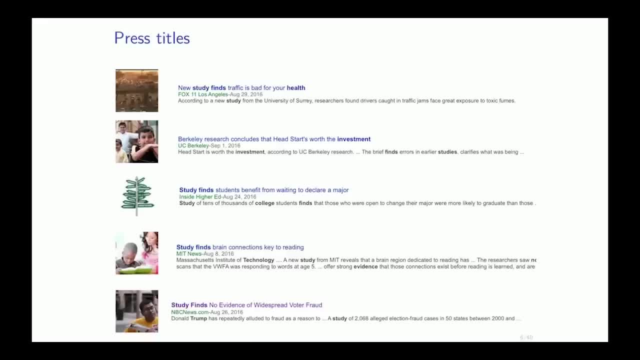 So we had to wait 2016 for data to tell us that, And there's a bunch of other slightly more interesting ones. For example, one that you might find interesting is that a study finds that students benefit from waiting to declare a major. 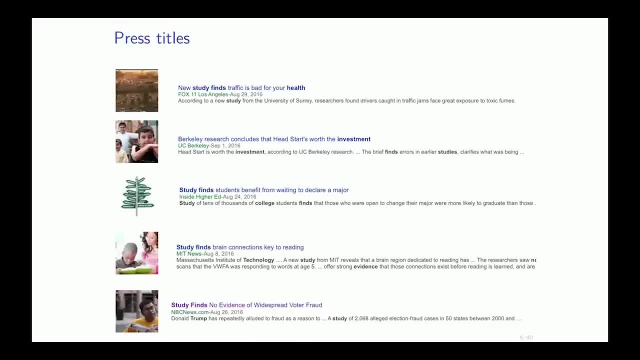 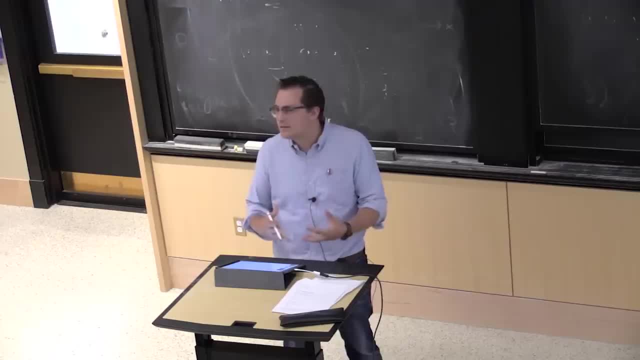 Some data was collected, Some scientific hypothesis was formulated, And then the data was here to try to prove or disprove the scientific hypothesis. That's the usual scientific process And we need to understand how the scientific process comes, because some of the data that we're 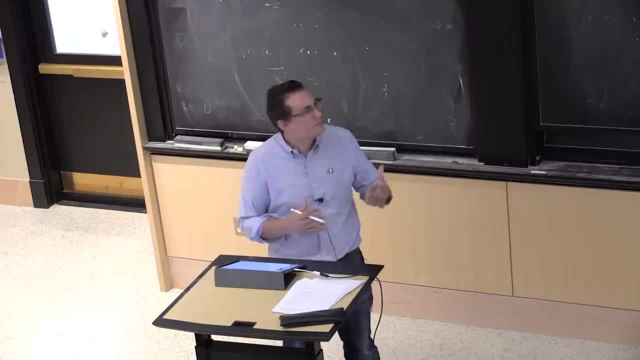 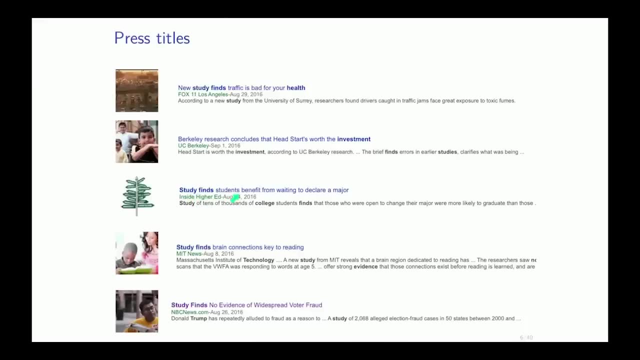 And we need to understand. We need to understand how the scientific process comes, Because some of those things might be actually questionable. Who is 100% sure that study finds that students do you think that you benefit from waiting to declare a major right? 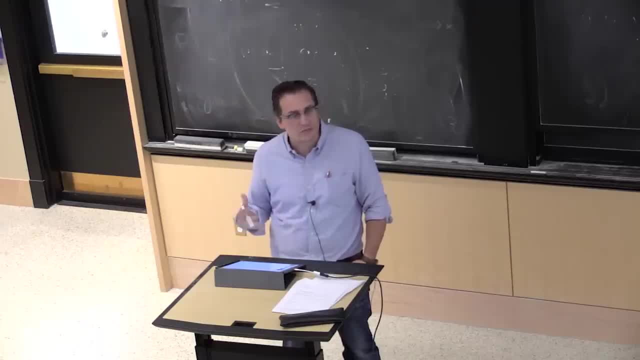 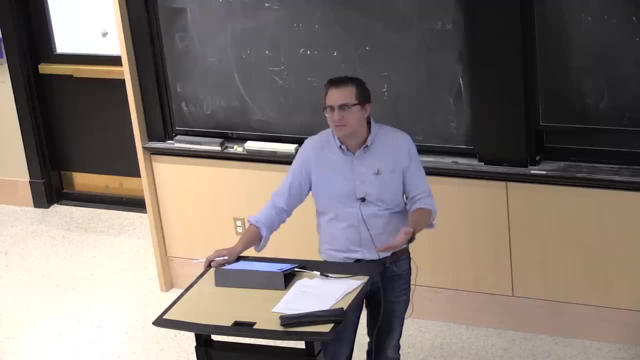 Maybe some of you, I mean, I would be skeptical about this, right, I would be like I don't want to wait to declare a major. Maybe this study. so what kind of thing can we bring? Well, maybe this study studied somebody people. 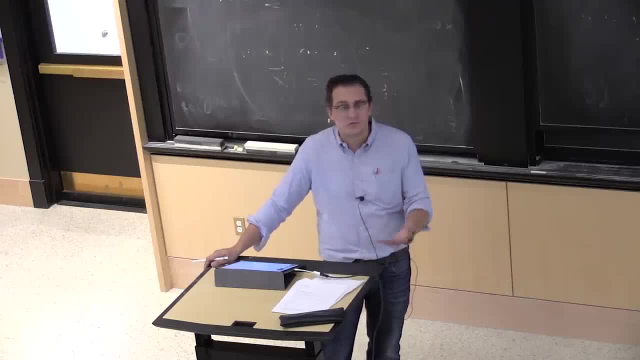 that were different from me, Or maybe this study, find that a majority that this is beneficial for majority of people. I'm not a majority, I'm just one person. There's a bunch of things that we need to understand what those things actually mean. 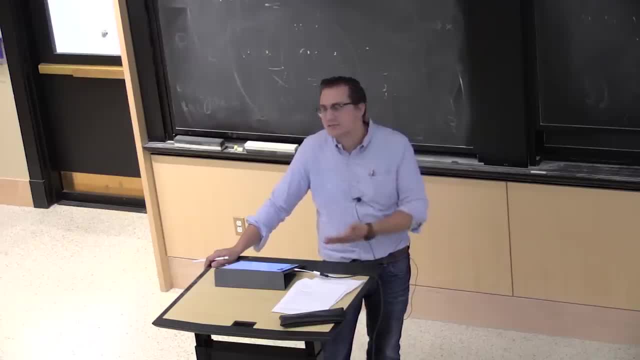 And we'll see that those are actually not statements about individuals. They're not even statement about the cohort of people they've actually looked at. They're statements about a parameter of a distribution that was used to model the benefit of waiting right. So there's a lot of questions and there 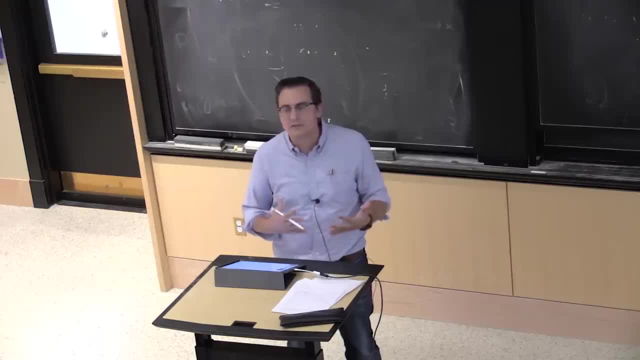 are a lot of layers that come into this And we're going to want to understand what was going on in there and try to peel it off and understand what assumptions, Assumptions, have been put in there, Even though it looks like a totally legit study. 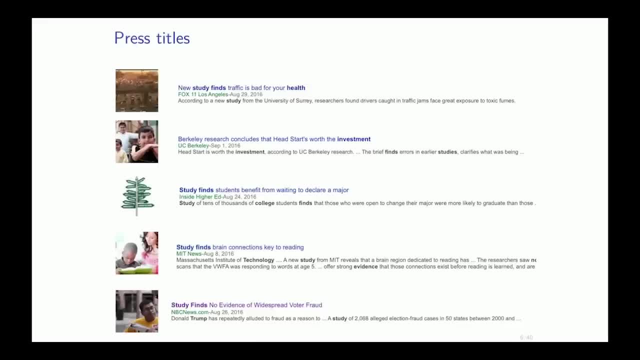 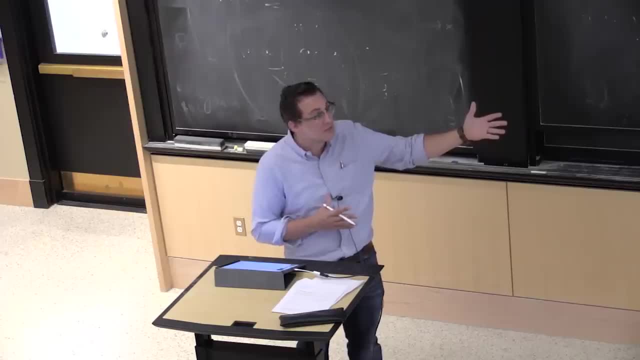 out of those studies, statistically, I think there's going to be one that's going to be wrong. Well, maybe not one, But if I put a long list of those, there would be a few that would actually be wrong. If I put 20,, there would definitely be one that's wrong. 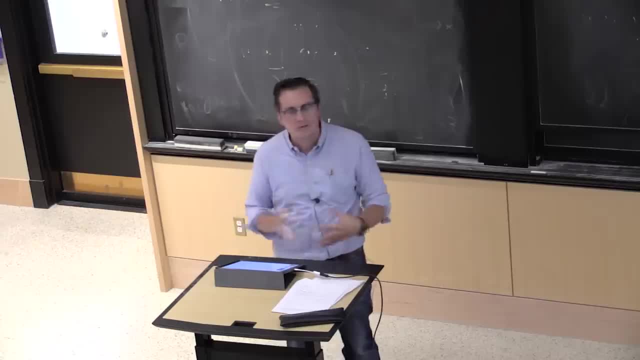 So you have to see that Every time you see 20 studies, one is probably wrong. When there are studies about drug effects, it would be out of the list of 100, one would be wrong. So we'll see what that means. 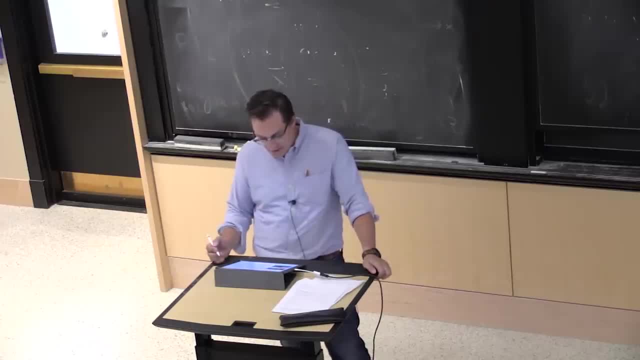 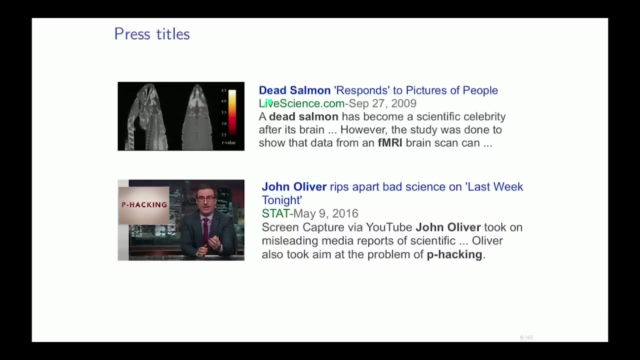 And what I mean by that. OK, So of course, not only studies that make these discoveries are actually making the press titles. there's also the press that talks about things that make no sense. So I love this first experiment: the dead salmon experiment. 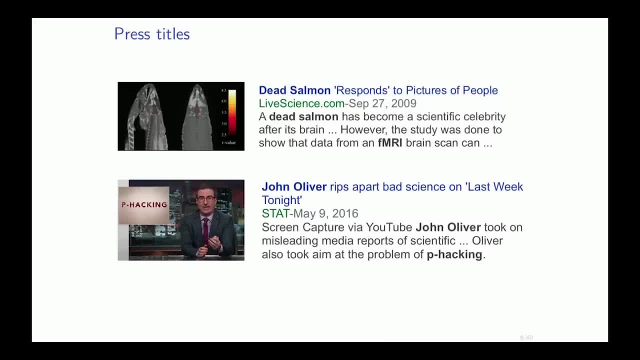 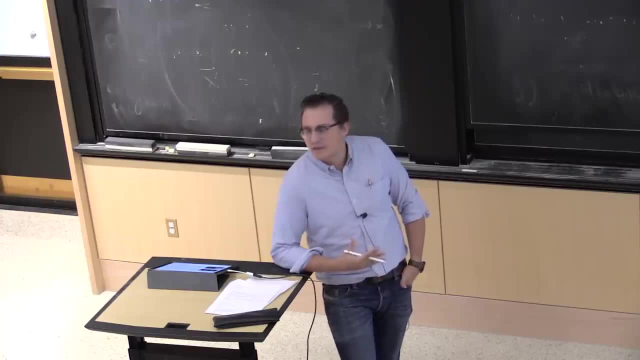 So actually it was a graduate student- came to a neuroscience poster session, pulled out this poster and explained the scientific experiment that it was conducting, Which consisted in taking a previously frozen and thawed salmon, putting it in an MRI, showing it pictures of violent images and recording its brain activity. 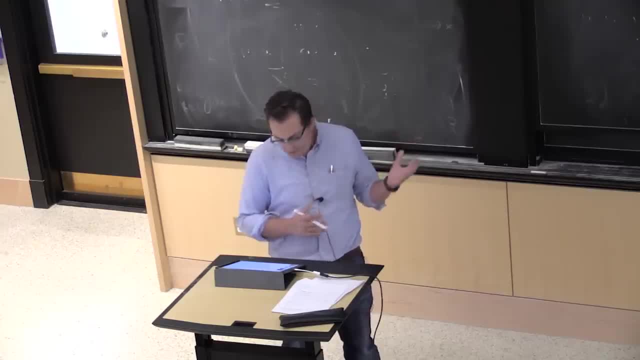 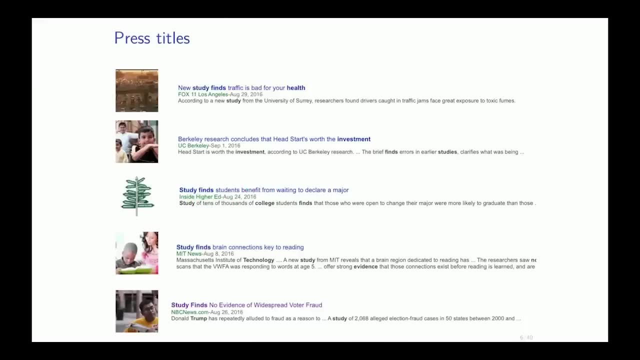 going to use some of those things might be actually questionable. Who is 100% sure that study finds that students do you think that you benefit from waiting to declare a major right? Maybe some of you, I mean, I would be skeptical about this. 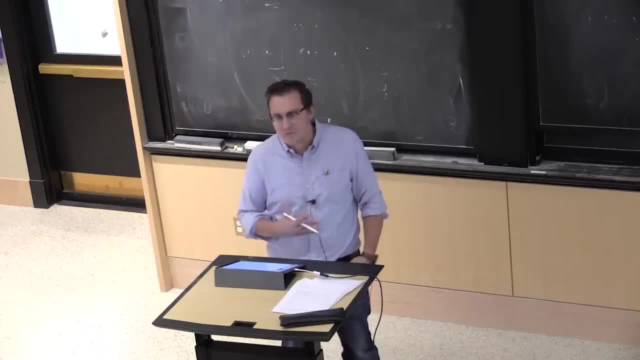 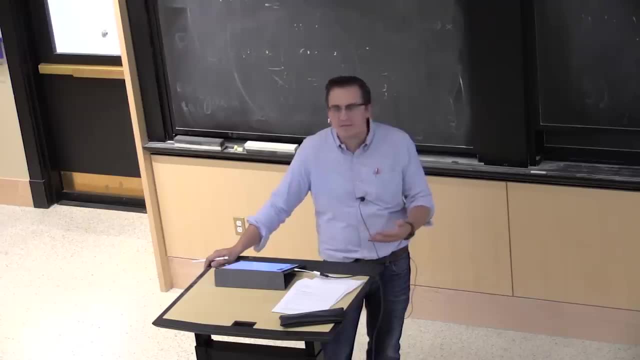 right, I would be like I don't want to wait to declare a major. Maybe this study. so what kind of thing can we bring? Well, maybe this study studied somebody, people that were different from me, Or maybe the study find that a majority. 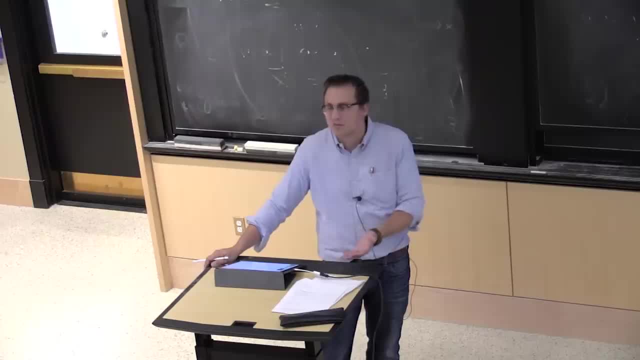 that this is beneficial for majority of people. I'm not a majority, I'm just one person. There's a bunch of things that we need to understand what those things actually mean, And we'll see that those are actually not statements about individuals. 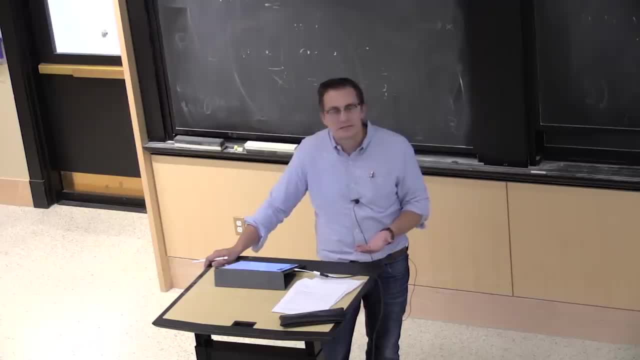 They're not even statements about the cohort of people they've actually looked at. They're statements about a parameter of a distribution that was used to model the benefit of waiting right. So there's a lot of questions and there are a lot of layers that come into this. 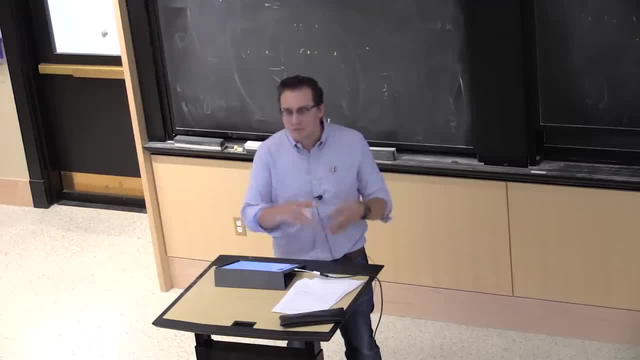 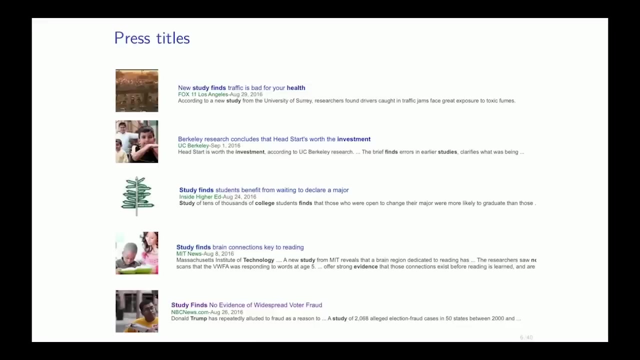 And we're going to want to understand what was going on in there and try to peel it off and understand what assumptions have been put in there, even though it looks like a totally legit study. Out of those studies, statistically I think there's going to be one that's going to be wrong. 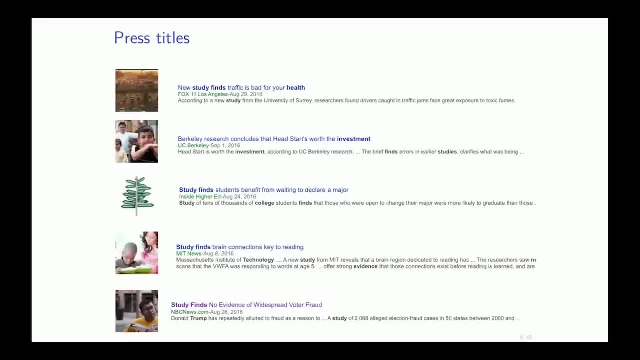 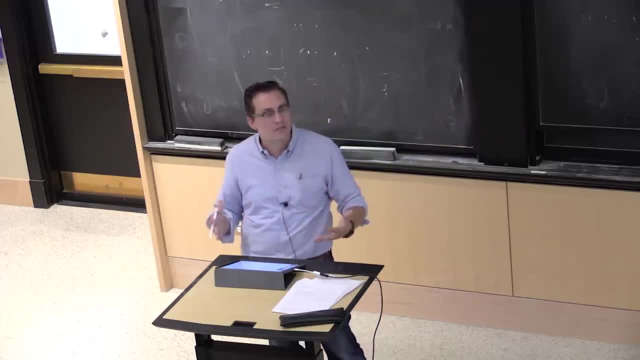 Well, maybe not one, But if I put a long list of those, there would be a few that would actually be wrong. If I put 20, there would definitely be one that's wrong. So you have to see that Every time you see 20 studies, one is probably wrong. 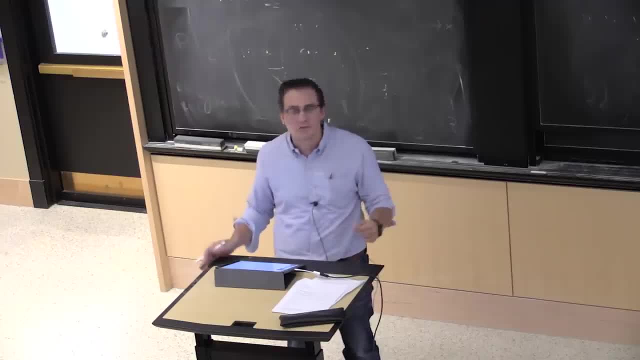 When there are studies about drug effects, it would be out of the list of 100, one would be wrong. So we'll see what that means and what I mean by that. OK, So of course, not only studies that make discoveries are actually making the press titles. 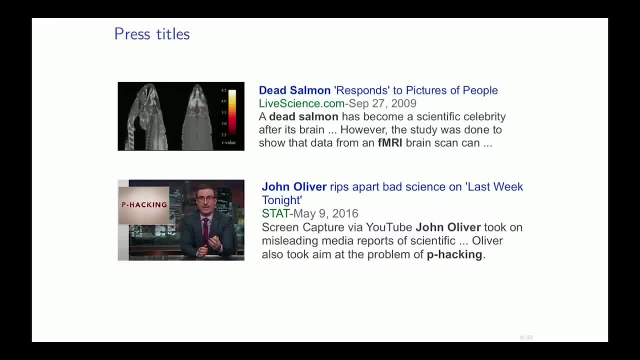 there's also the press that talks about things that make no sense. So I love this first experiment, the dead salmon experiment. So actually it was. a graduate student came to a neuroscience poster session, pulled out this poster and explained the scientific experiment that he was conducting, which. 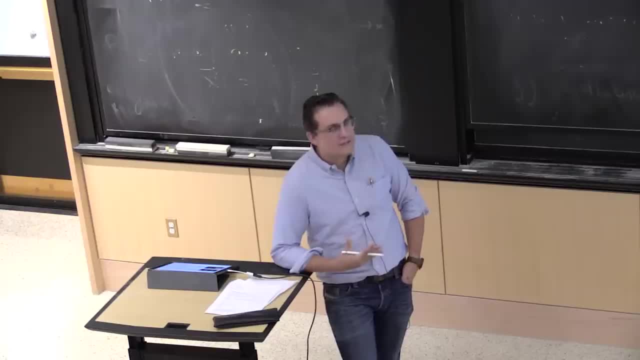 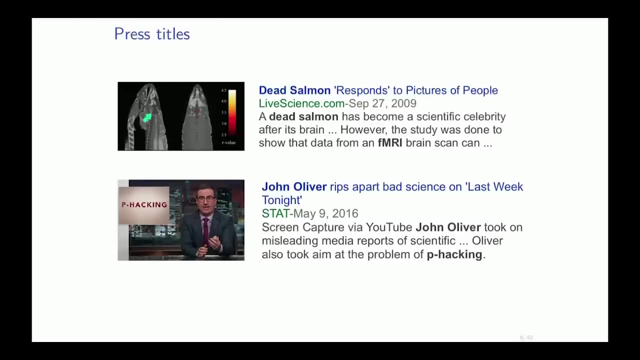 consisted in: He was taking a previously frozen and thawed salmon, putting it in an MRI, showing it pictures of violent images and recording its brain activity, And he was able to discover a few voxels that were activated by those violent images. 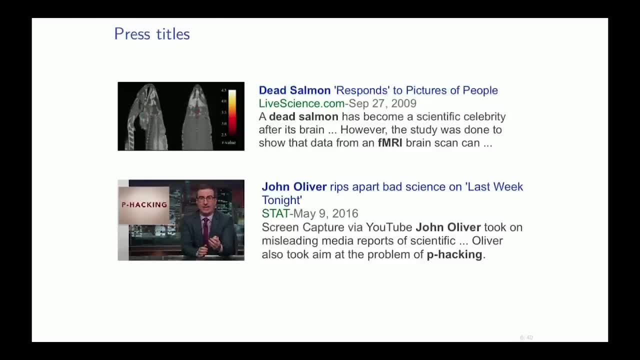 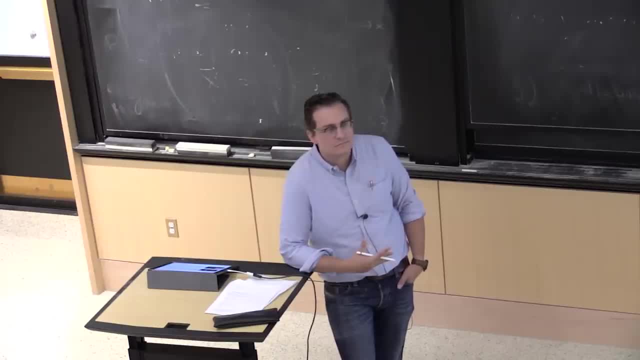 And he was able to discover a few voxels that were activated by those violent images. And can somebody tell me what happened here? Was the salmon responding to the violent activity? So basically, this is just the statistical fluke, right? That's just randomness at play. 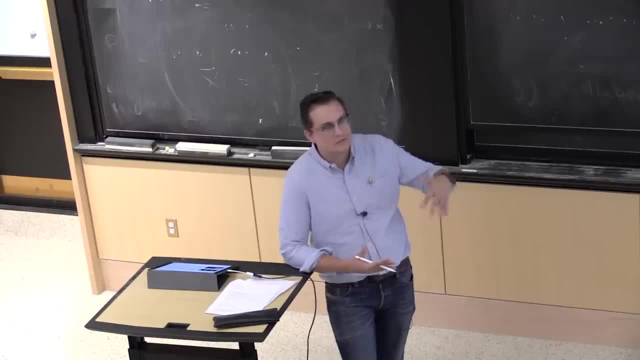 There's so many voxels that are recorded and there's so many fluctuations- right- There's always a little bit of noise when you run those things- that some of them just by chance got lit up, And so we need to understand how to correct for that. 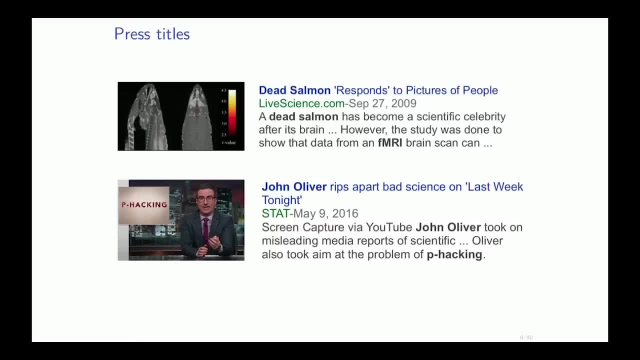 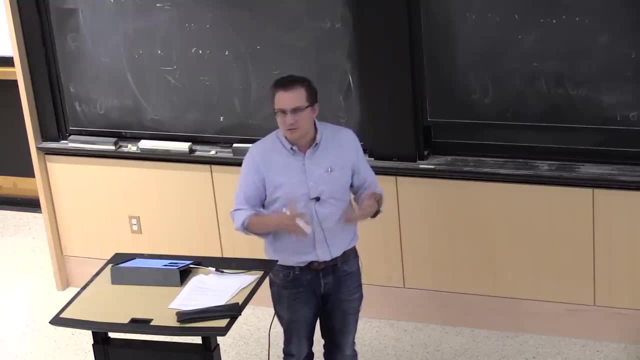 In this particular instance, we need to have tools that tell us that. well, finding three voxels that are activated- for that many voxels that you can find in the salmon's brain- is just too small of a number. Maybe we need to find a clump of 20 of them, for example. 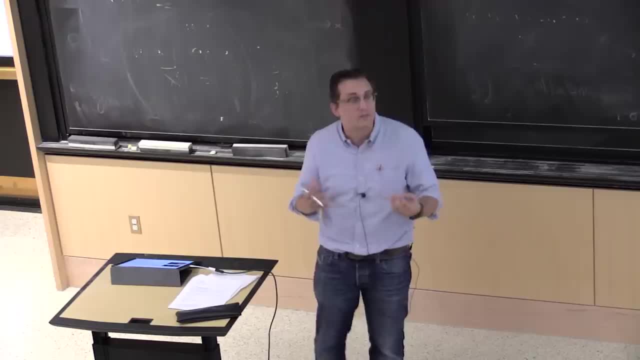 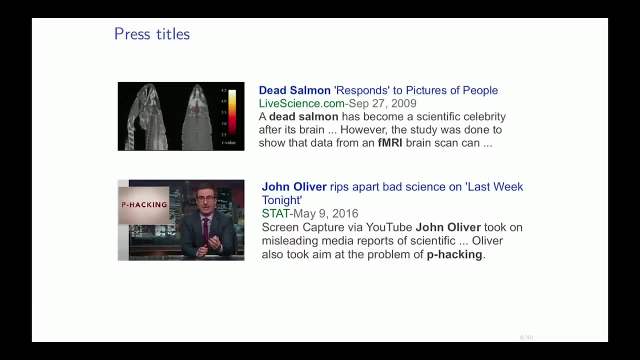 So we're going to have mathematical tools that help us find those particular numbers. I don't know if you saw this one by John Oliver about facking, Or actually it said p-hacking, And so basically what John Oliver is saying is actually a full length. like there's long segments on this. 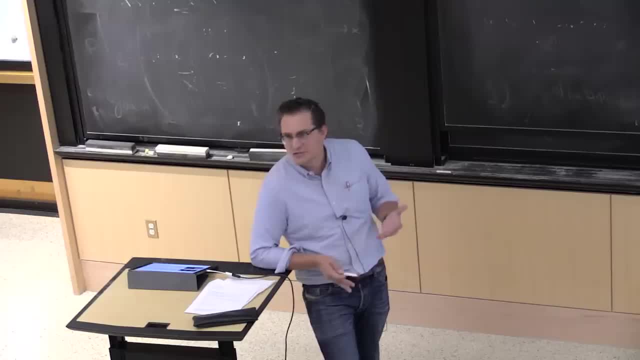 And he was explaining how there's a sociology question here, about how there's a huge incentive for scientists to publish results. right, You're not going to say you know what? This year I found nothing, And so people are trying to find things. 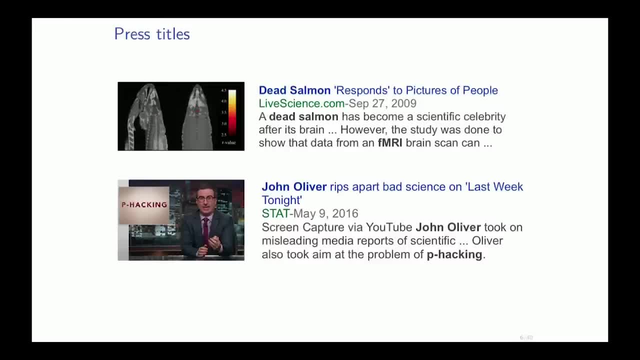 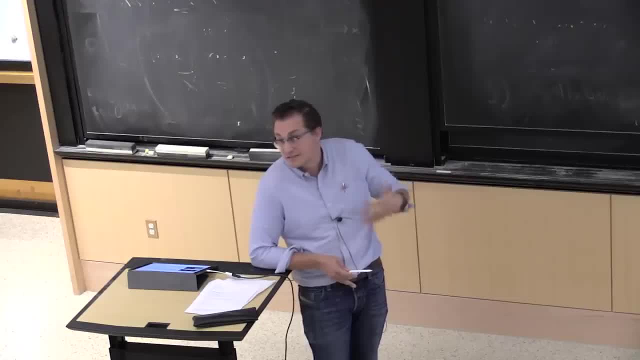 And just by searching. it's as if they were searching for all the voxels in a brain until they find one that was just lit up by chance. And so they just run all these studies And at some point one will be right, just out of chance. 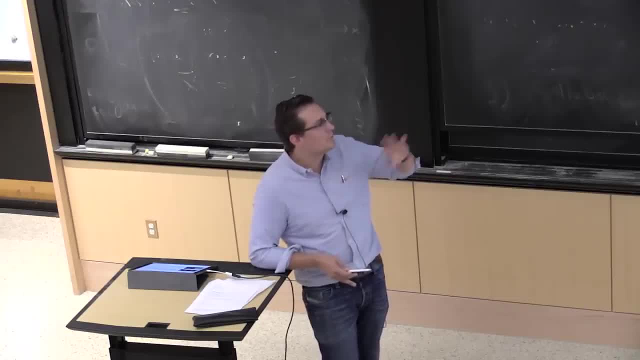 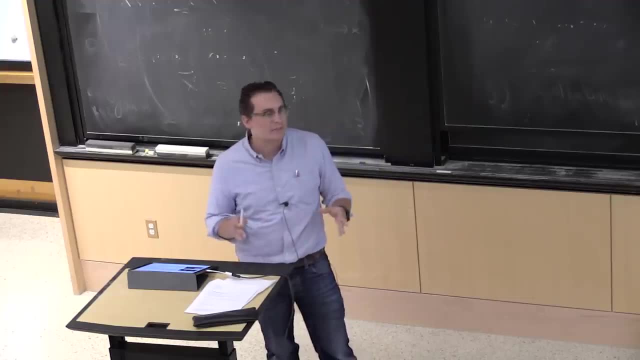 And so we have to be very careful about doing this. There's much more complicated problems associated to what's called p-hacking, which consists in violating the basic assumptions, in particular, looking at the data and then formulating your scientific assumption based on the data. 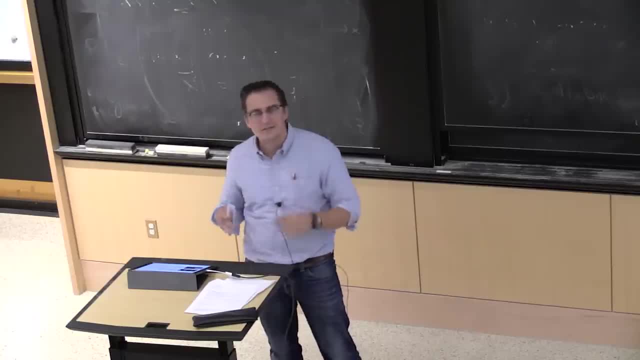 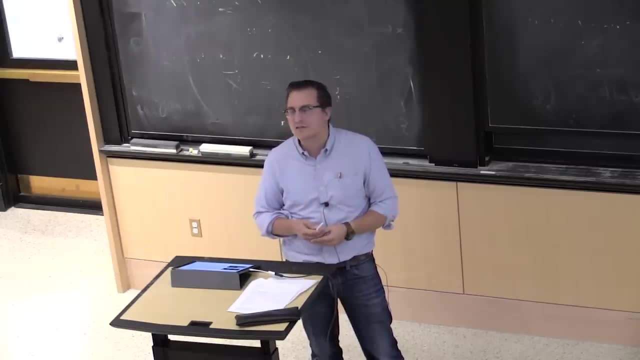 And then going back to it. it doesn't work. Let's just formulate another one, And if you start doing this, all bets are off. So actually, the statistics. the theory that we're going to develop is actually for very clean use of data, which 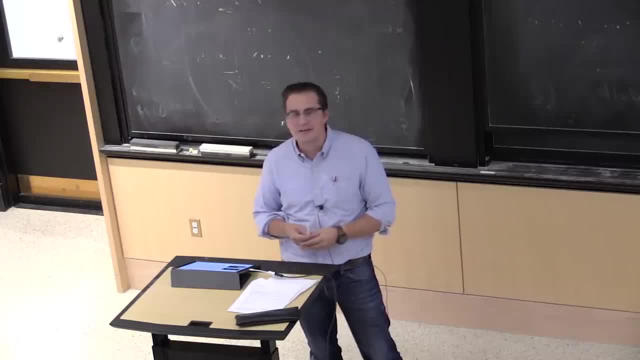 might be a little unpleasant if you've had an army of graduate students collecting genomic data for a year, for example. Maybe you don't want to say: well, I had one hypothesis, Didn't work, Let's throw all the data to the trash. 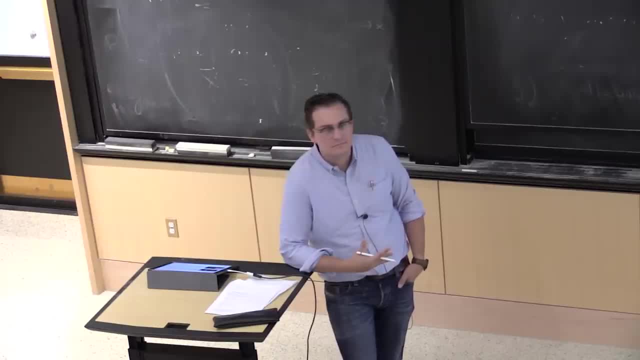 And can somebody tell me what happened here? Was the salmon responding to the violent activity? So basically, this is just the statistical fluke. That's just randomness at play. There's so many voxels that are recorded and there's so many fluctuations. 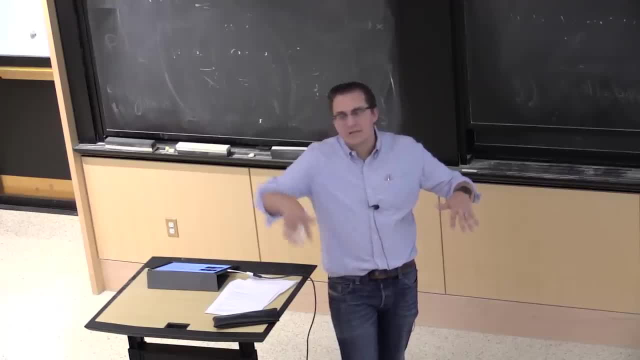 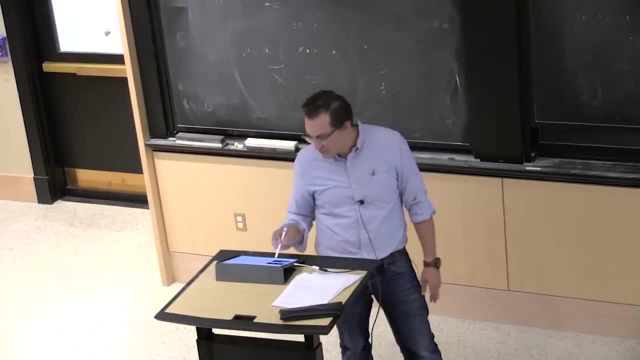 There's always a little bit of noise when you run those things, that some of them just by chance got lit up, And so we need to understand how to correct for that. In this particular instance, we need to have tools that tell us that. well, finding three voxels that. 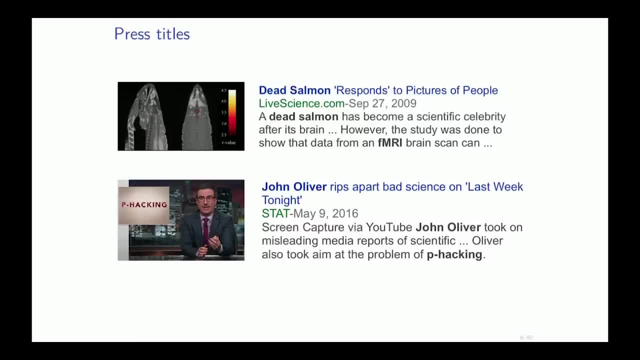 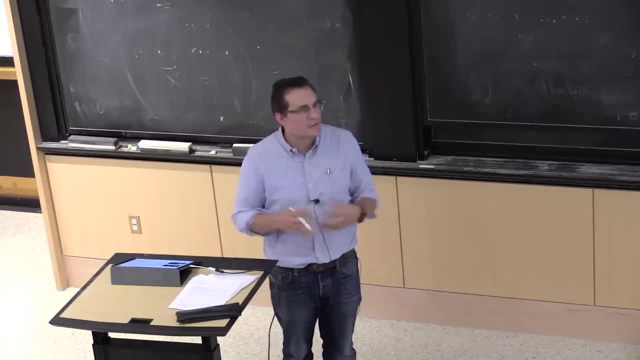 are activated, for that many voxels that you can find in the salmon's brain is just too small of a number. Maybe we need to find a clump of 20 of them, for example. All right, So we're going to have mathematical tools that help. 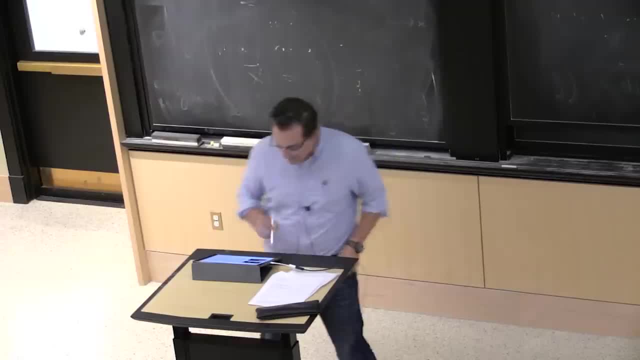 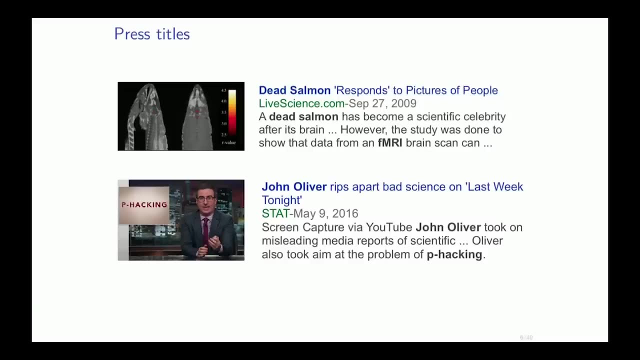 us find those particular numbers. I don't know if you saw this one by John Oliver about facking, Or actually it said p-hacking, And so basically what John Oliver is saying is actually a full length. There's these long segments on this. 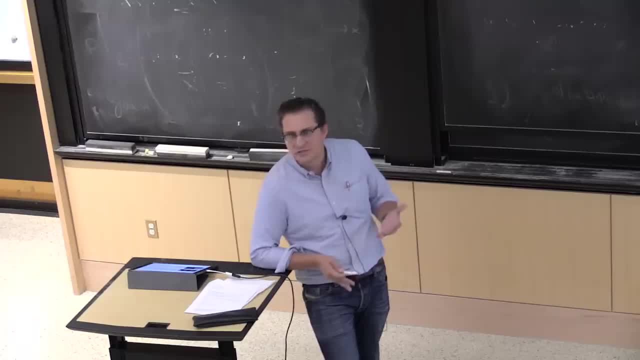 And he was explaining how there's a huge- I mean, OK, there's a sociology question here about how there's a huge incentive for scientists to publish results. right, You're not going to say you know what? This year I found nothing. 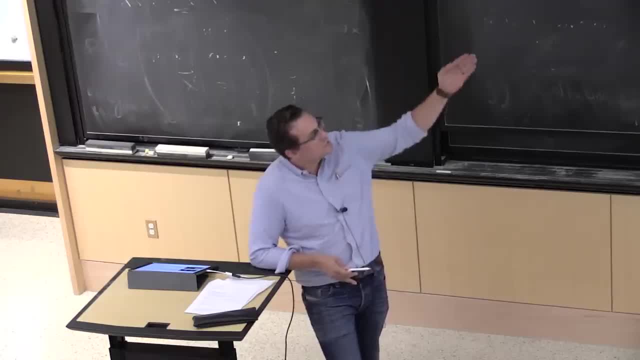 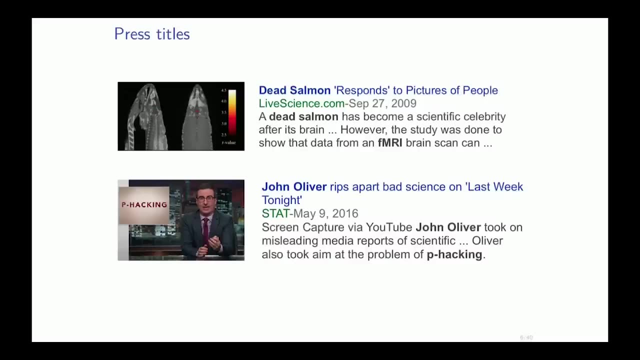 And so people are trying to find things, And just by searching it's as if they were searching for all the voxels in a brain until they find one that was just lit up by chance. And so they just run all these studies And at some point one will be right, just out of chance. 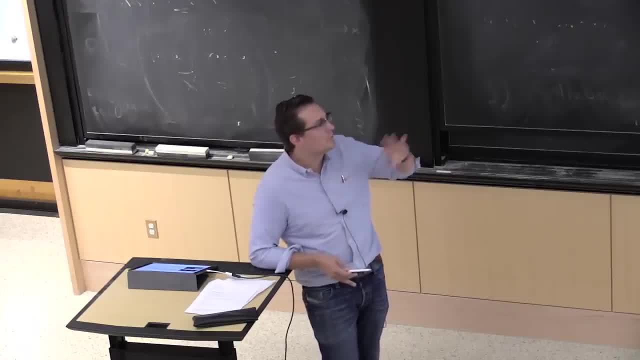 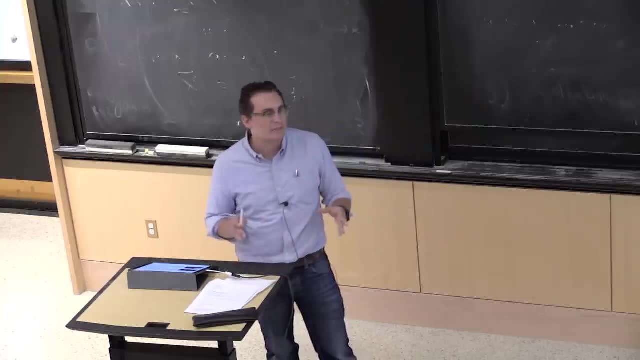 And so we have to be very careful about doing this. There's much more complicated problems associated to what's called p-hacking, which consists in violating the basic assumptions, in particular, looking at the data and then formulating your scientific assumption based on the data. 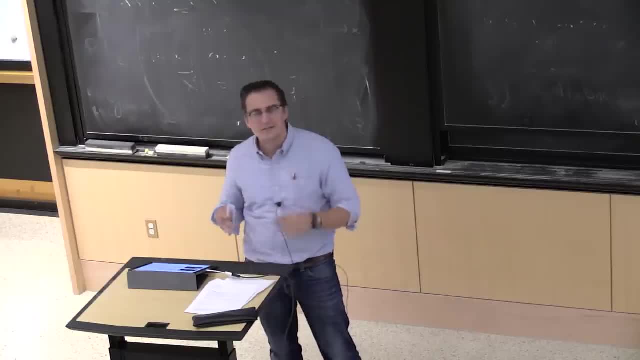 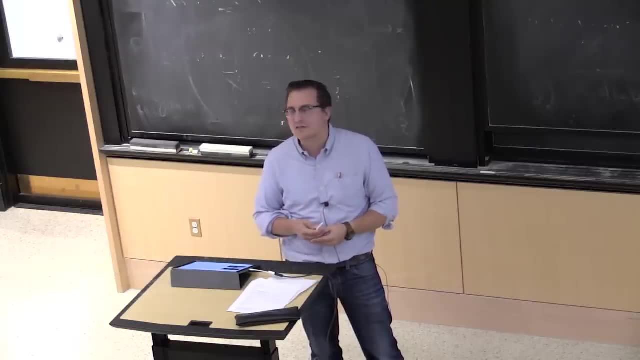 And then going back to it. it doesn't work. Let's just formulate another one, And if you start doing this, all bets are off. So actually, the statistics. the theory that we're going to develop is actually for very clean use of data, which 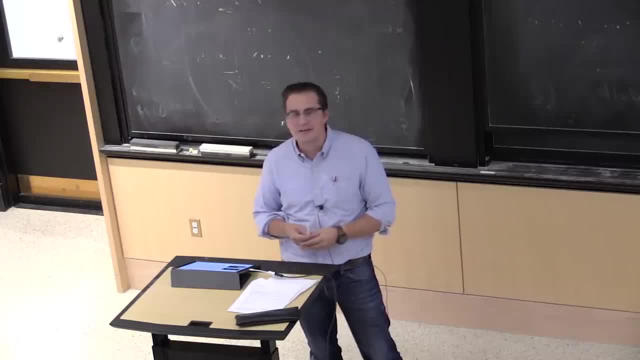 might be a little unpleasant. if you've had an army of graduate students collecting genomic data for a year, for example, Maybe you don't want to say: well, I had one, My hypothesis didn't work, Let's throw all the data to the trash. 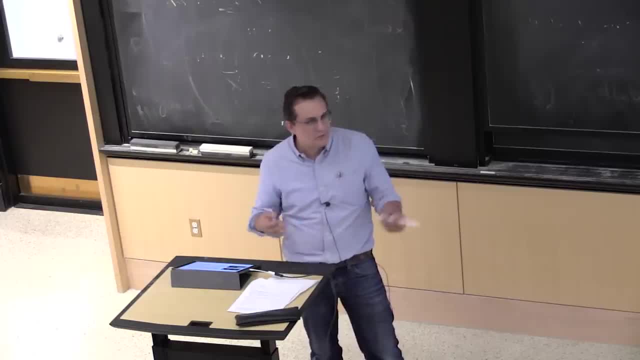 And so we need to find ways to be able to do this, And there's actually a course being taught at BU- I mean, it's still in its early stages- but something called adaptive data analysis that will allow you to do these kind of things. 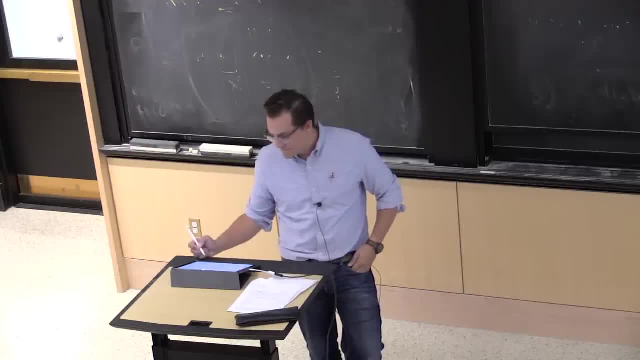 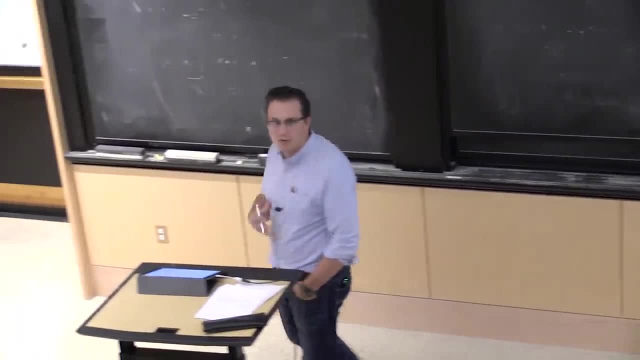 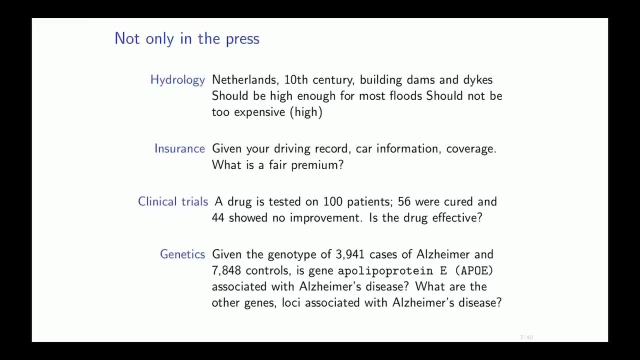 Questions. So, of course, statistics is not just for you to be able to read the press. Statistics will probably be used. It's going to be used in whatever career path you choose for yourself. So it started in the 10th century in Netherlands. 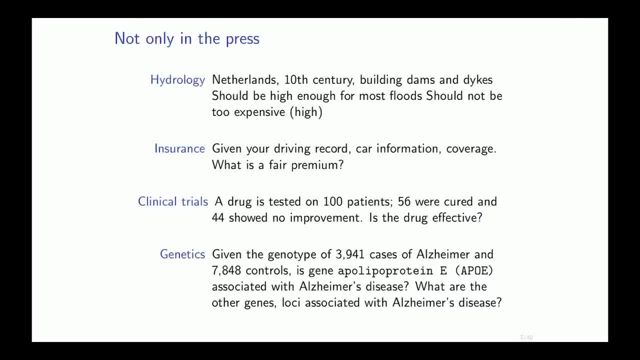 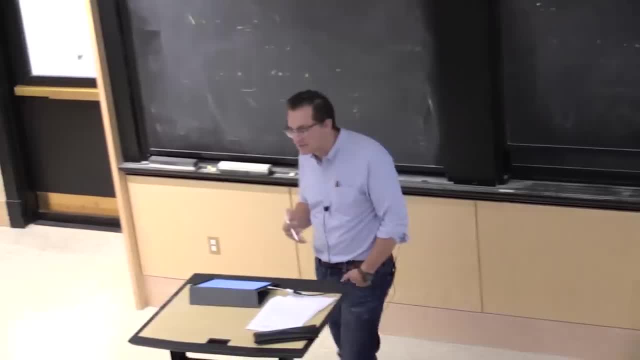 for hydrology right. Netherlands is basically in the water and the sea level, And so they wanted to build some dikes. But once you're going to build a dike, you want to make sure that it's going to sustain some tides and some floods. 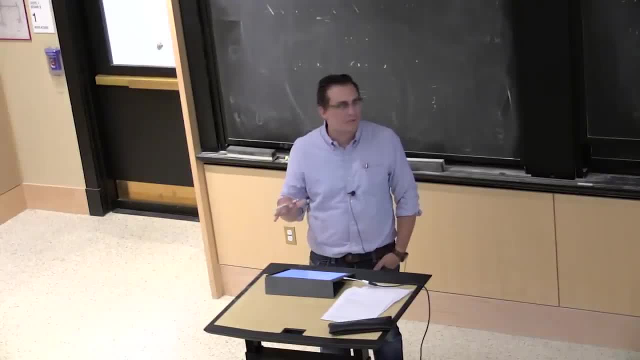 And so, in particular, they wanted to build dikes that were high enough, but not too high. You could always say, well, I'm going to build a 500-meter dike and I'm going to be safe. You want something that's based on data, right? 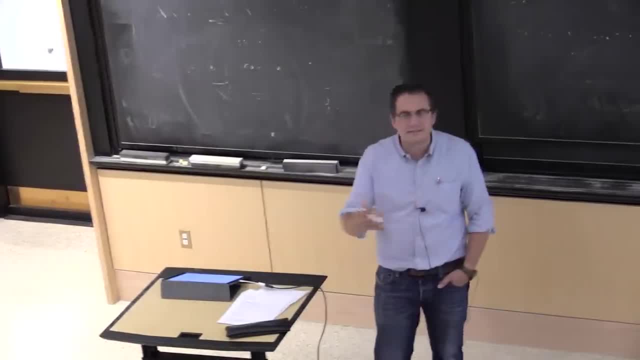 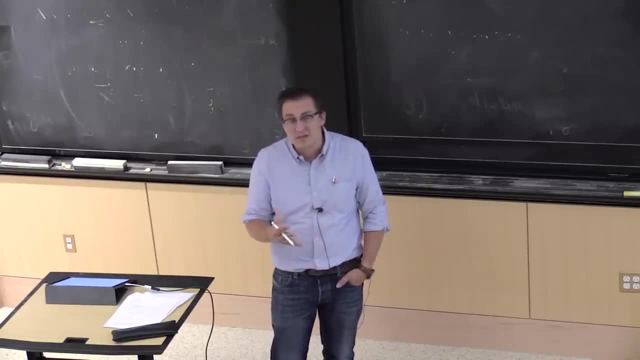 You want to make sure, And so, in particular, what did they do? Well, they collected data for previous floods, and then they just found a dike that was going to cover all these things. Now, if you look at the data, they probably had. 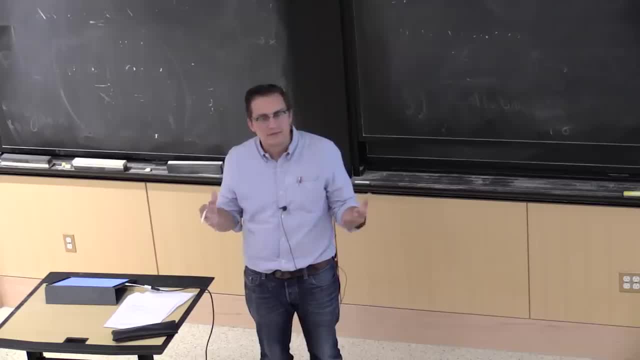 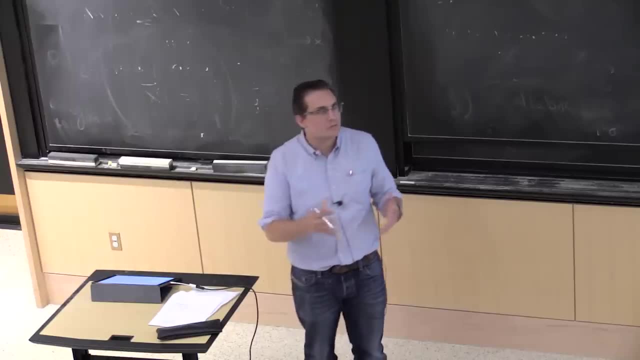 maybe it was scarce, right? Maybe they had 10 data points, And so, for these data points, maybe they wanted to sort of interpolate between those points, maybe extrapolate for the larger one. Based on what they've seen, maybe they have chances of seeing something which is even. 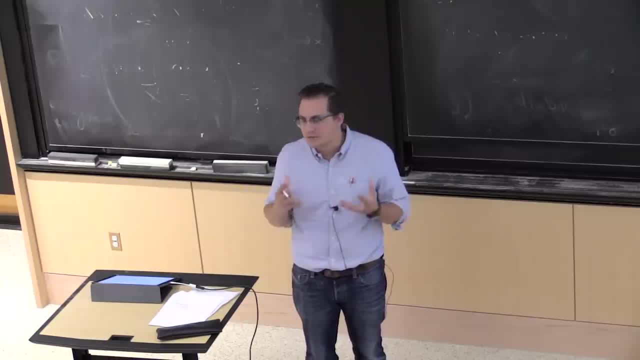 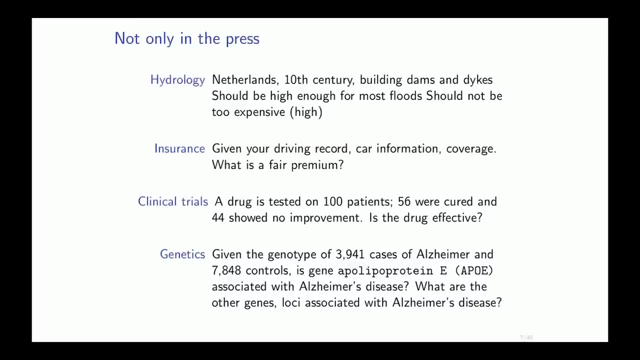 larger than everything they've seen before. And that's exactly the goal of statistical modeling: being able to extrapolate beyond the data that you have Guessing what you have not seen yet might happen When you buy insurance for your car or your apartment. or your phone. there's a premium that you have to pay And this premium has been determined based on how much you're in expectation going to cost the insurance. right, It says, OK, This person has, say, a 10% chance of breaking their iPhone. 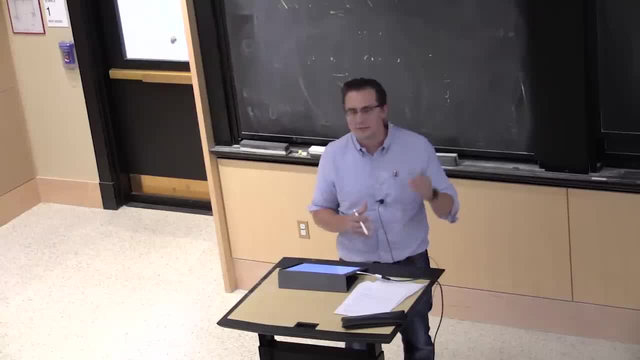 An iPhone costs that much to repair, so I'm going to charge them that much, And then I'm going to add an extra dollar for my time. So that's basically how those things are determined, And so this is using statistics. This is basically where statistics 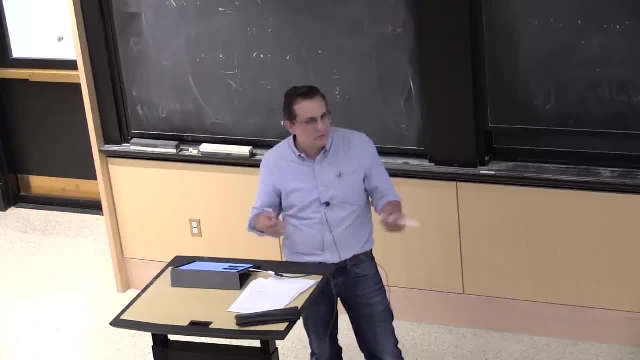 And so we need to find ways to be able to do this, And there's actually a course being taught at BU. It's still in its early stages, but something called adaptive data analysis that will allow you to do these kind of things. Questions: 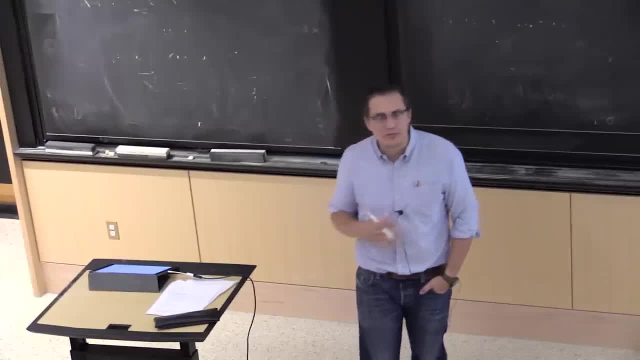 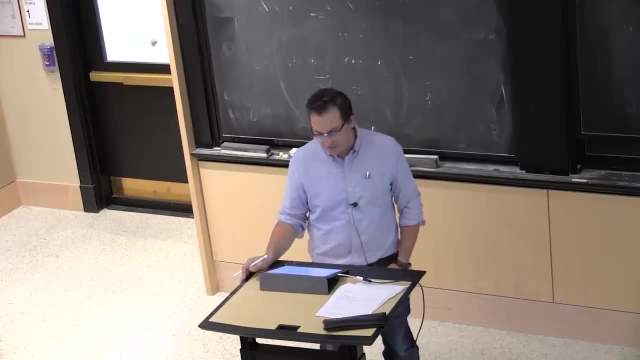 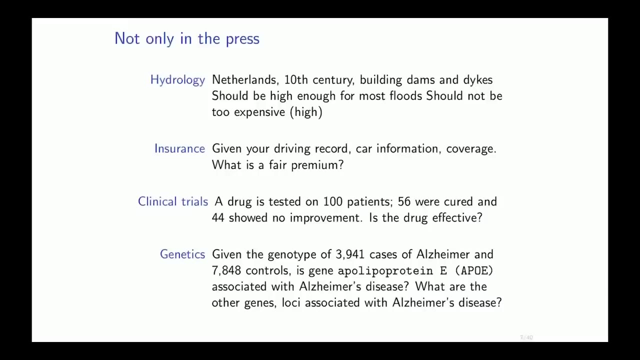 So, of course, statistics is not just for you to be able to read the press. Statistics will probably be used in whatever career path you choose for yourself. So it started in the 10th century in Netherlands for hydrology. Netherlands is basically in the water and the sea level. 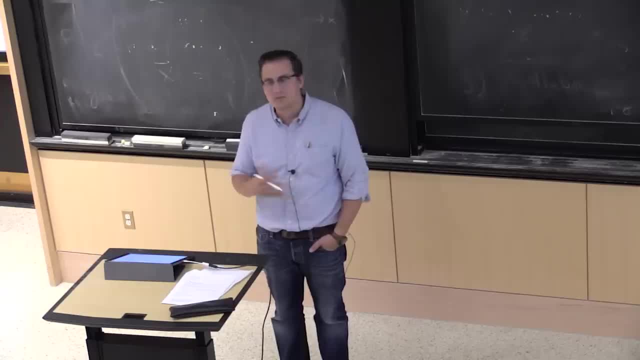 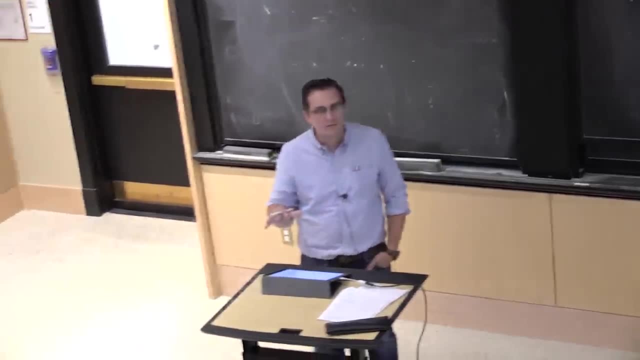 And so they wanted to build some dikes. But once you're going to build a dike, you want to make sure that it's going to sustain some tides and some floods, And so, in particular, they wanted to build dikes that were high enough, but not too high. 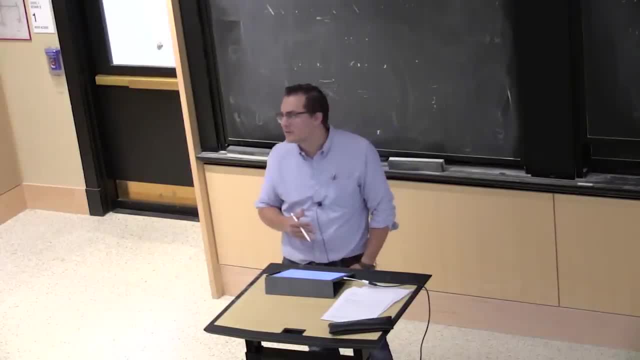 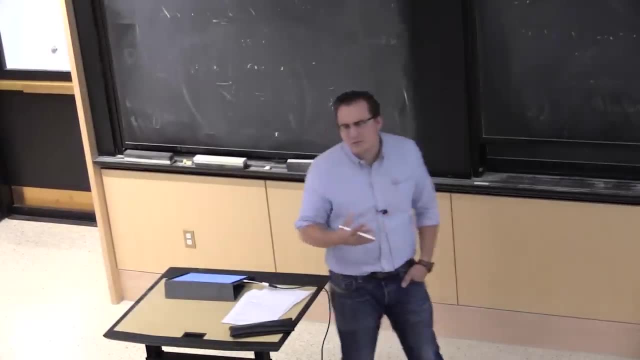 You could always say: well, I'm going to build a 500-meter dike and then I'm going to be safe. You want something that's based on data, You want to make sure, And so, in particular, what did they do? 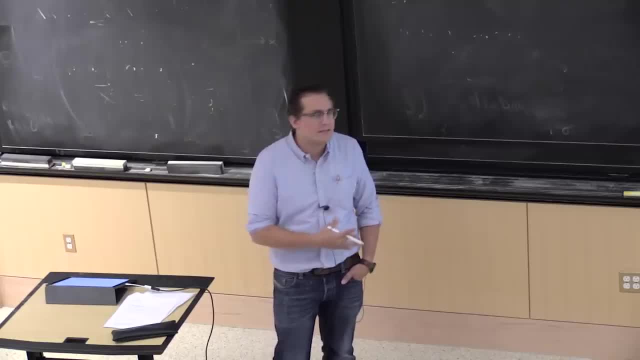 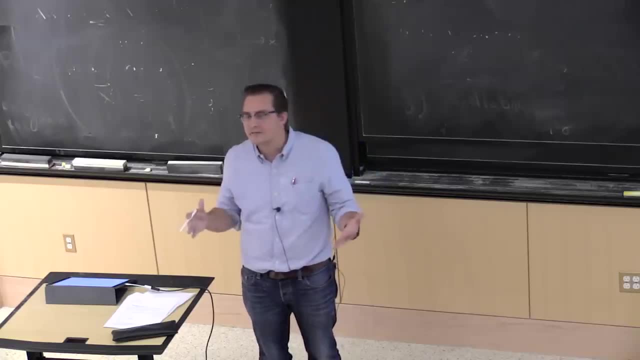 Well, they collected data for previous floods and then they just found a dike that was going to cover all these things. Now, if you look at the data they probably had- maybe it was scarce, Maybe they had 10 data points- 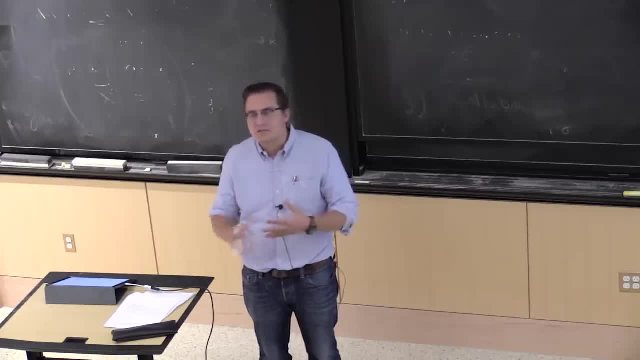 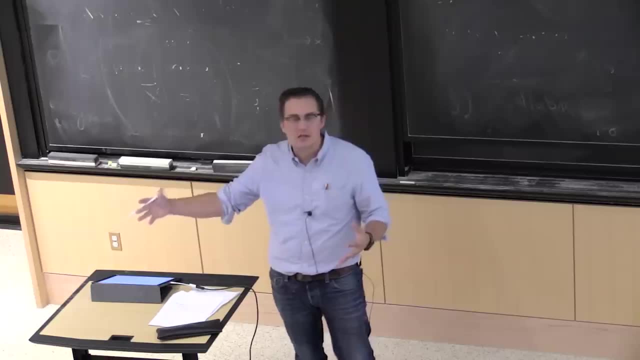 And so for these data points, then maybe they wanted to sort of interpolate between those points, maybe extrapolate for the larger one. Based on what they've seen, maybe they have chances of seeing something which is even larger than everything they've seen before. 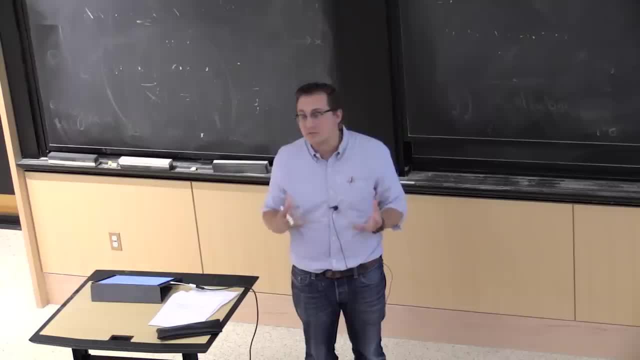 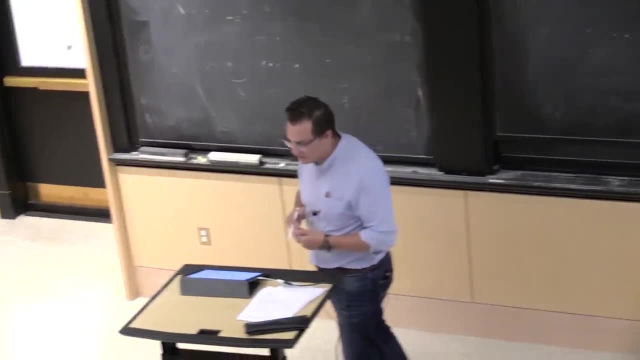 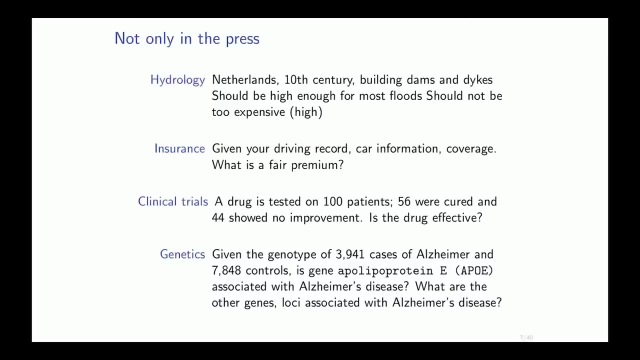 And that's exactly the goal of statistical modeling: being able to extrapolate beyond the data that you have guessing what you have not seen yet might happen. When you buy insurance for your car or your apartment or your phone, there's a premium that you have to pay. 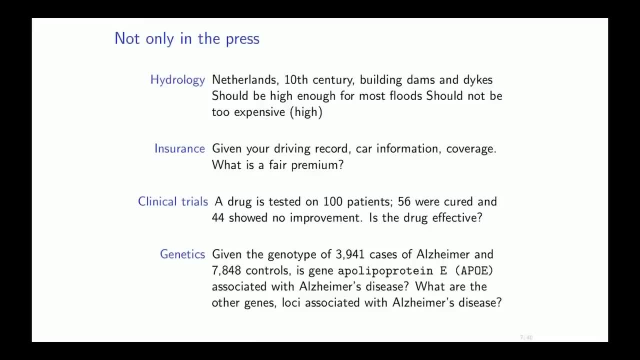 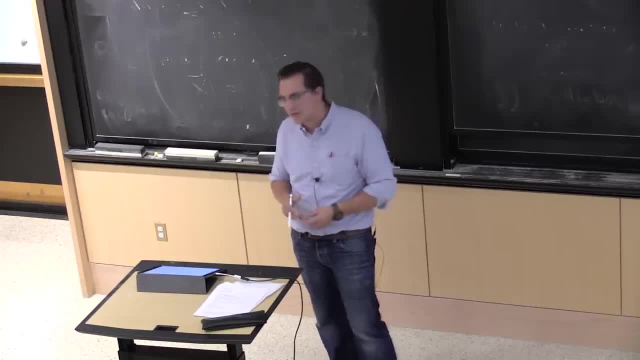 And this premium has been determined based on how much you're in expectation going to cost the insurance. It says, OK, this person has, say, a 10% chance of breaking their iPhone. An iPhone costs that much to repair. 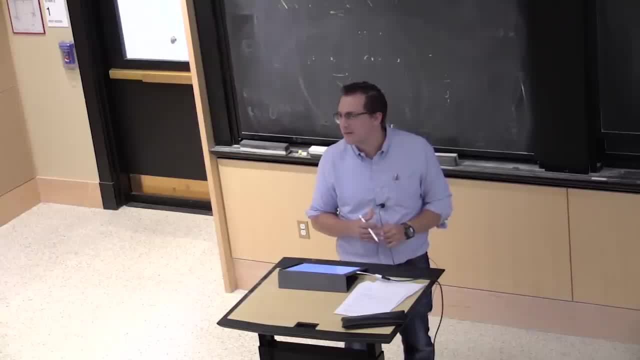 so I'm going to charge them that much and then I'm going to add an extra dollar for my time. So that's basically how those things are determined, And so this is using statistics. This is basically where statistics is probably mostly used. 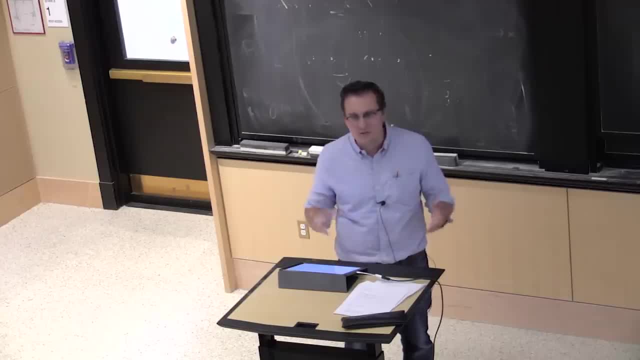 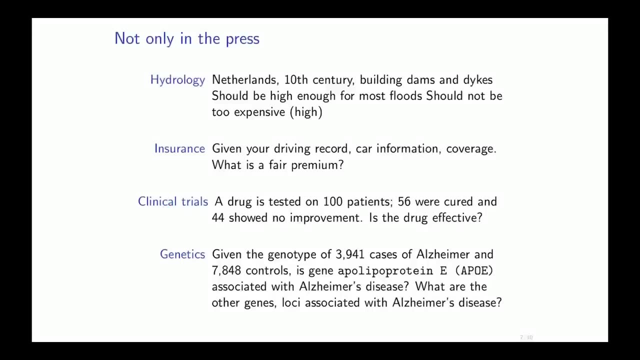 is probably mostly used. I was personally trained as an actuary and that's me being a statistician in an insurance company: Clinical trials- this is also one of the earliest success stories of statistics, So it's actually now widespread. Every time a new drug is approved for market by the FDA. 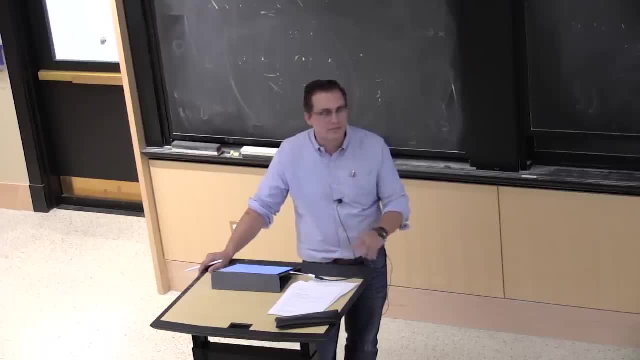 it requires a very strict regimen of testing with data and control group and treatment group and how many people you need in there and what kind of significance you need for those things. So in particular, those things look like this: So now it's more 5,000 patients. 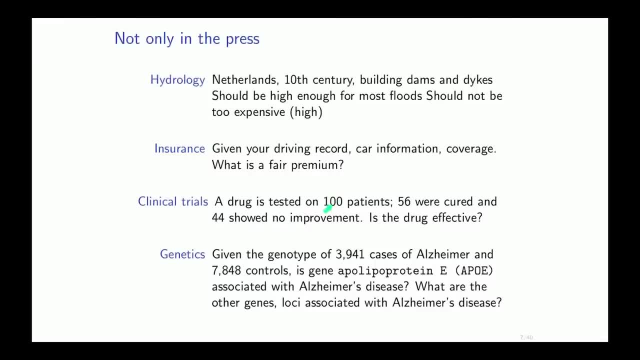 I mean, it depends on what kind of drug it is, But for, say, 100 patients, 56 were cured and 44 showed no improvement. Does the FDA consider that this is a good number? Does it have a table for how many patients were cured? 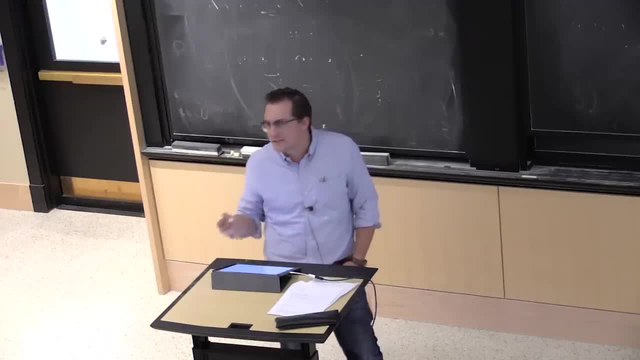 Is there a placebo effect? Do I need a control group of people that are actually getting a placebo? It's not clear, all these things, And so there's a lot of things to put into place and there's a lot of floating parameters. 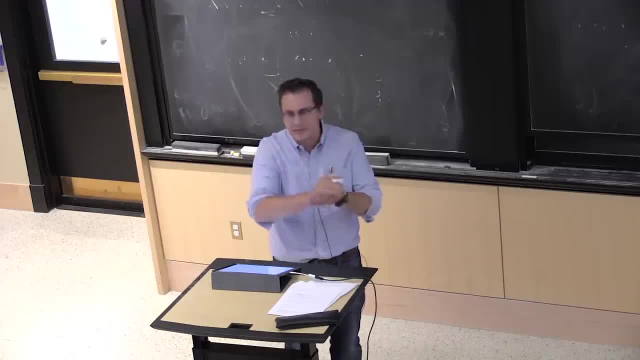 So hopefully we're going to be able to use statistical modeling to shrink it down to a specific number, Small number of parameters to be able to ask very simple questions: Is a drug effective? is not a mathematical equation, but is p larger than 0.5 is a mathematical question. 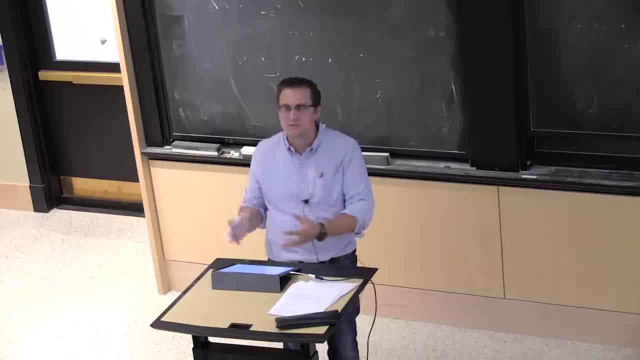 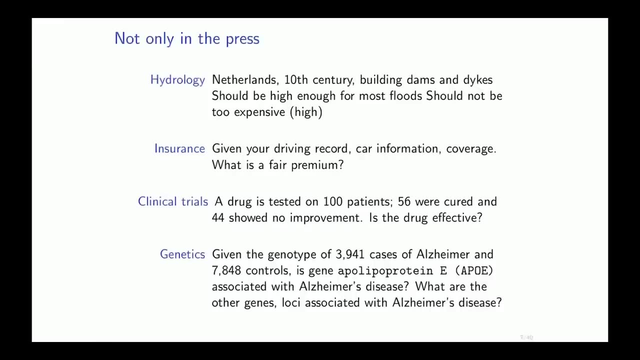 And that's essentially what we're going to be doing. We're going to take this is a drug effective to reducing to is a variable larger than 0.5. Now, of course, genetics are using that, So that's typically actually the same type of size of data. 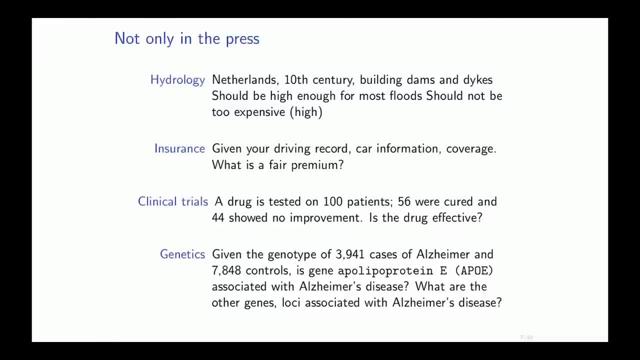 that you would see for fMRI data. So, given the genotype of a patient, we're going to be able to do a lot of things with it. So this is actually a study that I found. So you have about 4,000 cases of Alzheimer's and 8,000 controls. 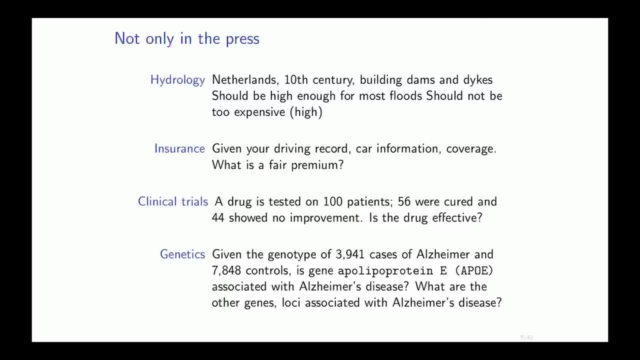 So people without Alzheimer's, that's what's called a control. That's something just to make sure that you can see the difference with the people that are not affected by either a drug or a disease. Is the gene APOE associated with Alzheimer's disease? 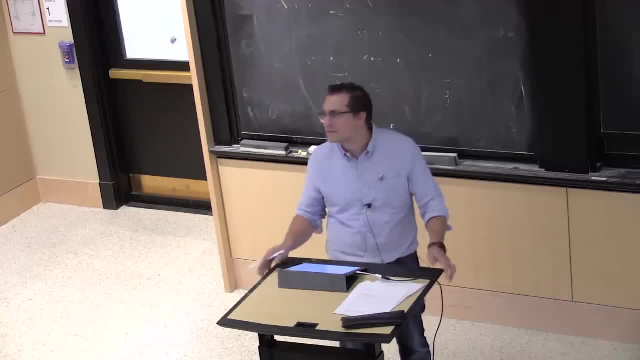 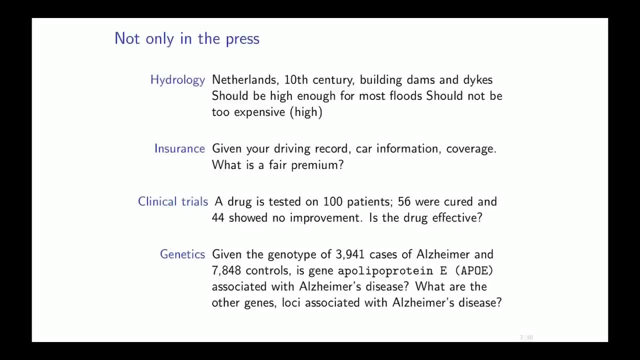 I was personally trained as an actuary, and that's me being a statistician in an insurance company: Clinical trials. This is also one of the earliest success stories of statistics, So it's actually now widespread. Every time a new drug is approved for market by the FDA. 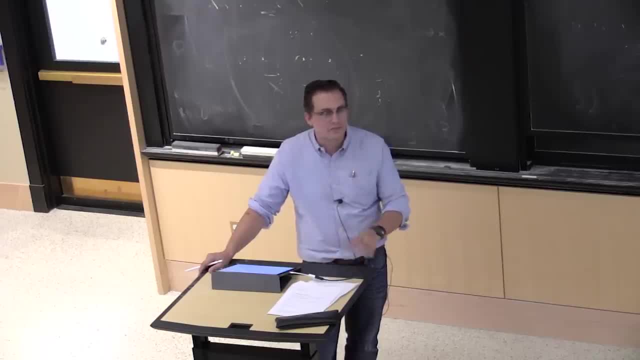 it requires a very strict regimen of testing with data and control group and treatment group and how many people you need in there and what kind of significance you need for those things. So in particular, those things look like this: So now it's more five: 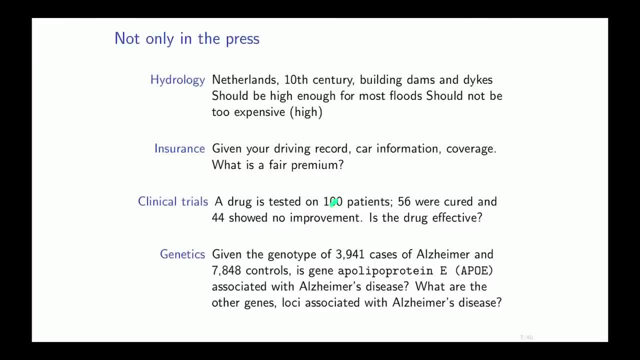 I mean, it depends on what kind of drug it is, But for, say, 100 patients, 56 were cured and 44 showed no improvement. Does the FDA consider that this is a good number? Does it have a table for how many patients were cured? 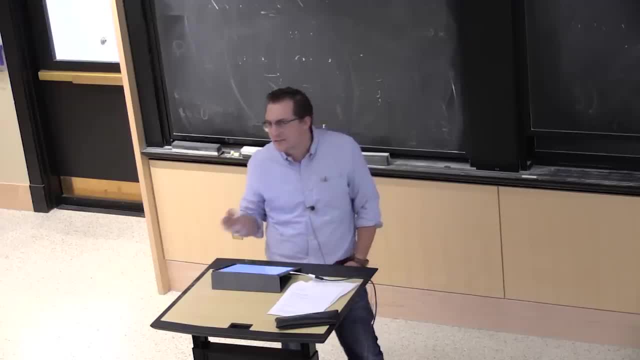 Is there a placebo effect? Do I need a control group of people that are actually getting a placebo? It's not clear, all these things, And so there's a lot of things to put into place and there's a lot of floating parameters. 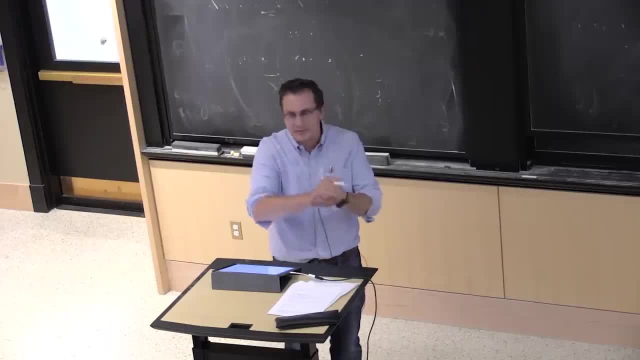 So hopefully we're going to be able to use statistical modeling to shrink it down to a small number of parameters to be able to ask very simple questions: Is a drug effective is not a mathematical equation, but is p larger than 0.5 is a mathematical question. 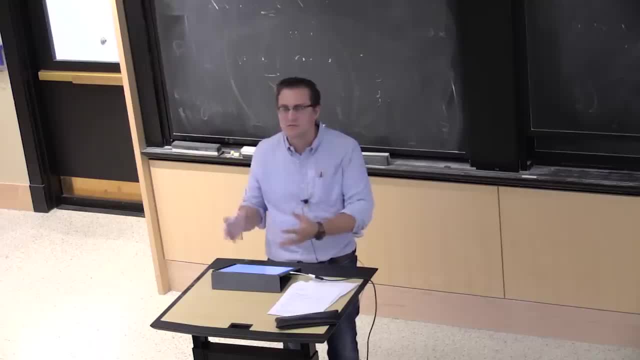 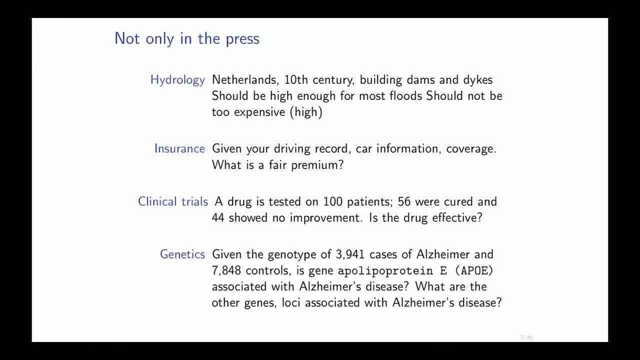 And that's essentially what we're going to be doing. We're going to take this is a drug effective to reducing to is a variable larger than 0.5. Now, of course, genetics are using that, So that's typically actually the same type of size of data. 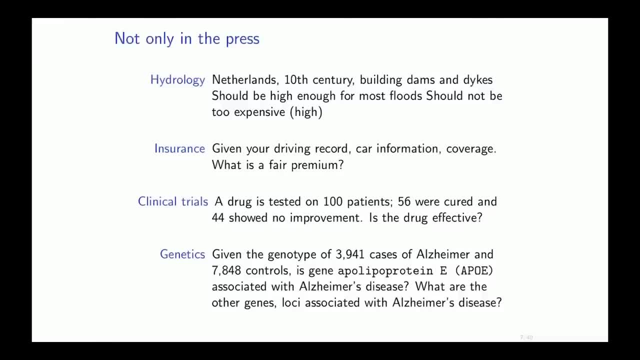 that you would see for fMRI data. So, given the genotype of, so this is actually a study that I found. So you have about 4,000 cases of Alzheimer's and 8,000 controls, So people without Alzheimer's that's. 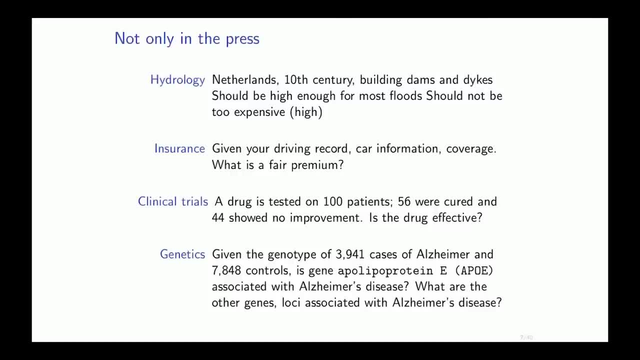 what's called a control. That's something just to make sure that you can see the difference with the people that are not affected by either a drug or a disease. Is the gene APOE associated with Alzheimer's disease? I mean everybody can see why this. 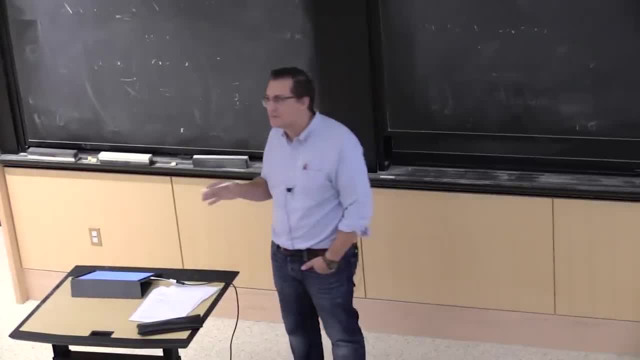 would be an important question. We now have CRISPR. It's targeted. It's targeted to very specific genes. If we could edit it or knock it down, or knock it up or boost it, maybe we could actually have an impact on that. 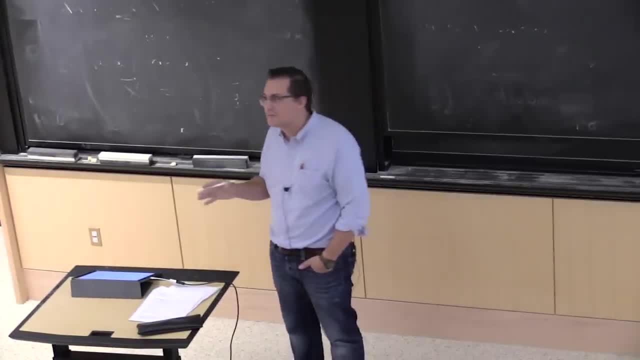 Everybody can see why this would be an important question. We now have CRISPR. It's targeted to very specific genes. If we can edit it or knock it down, or knock it up or boost it, maybe we could actually have an impact on that. 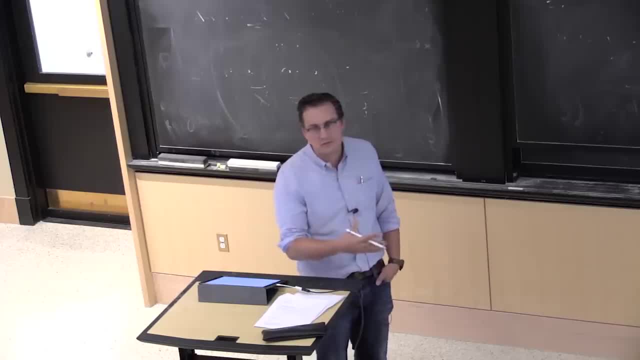 So those are very important questions because we have the technology to target those things, but we need the answers about what those things are. And so there's a bunch of other questions that the minute you're going to talk to a biologist about, say, I can do this, they're going to say OK. 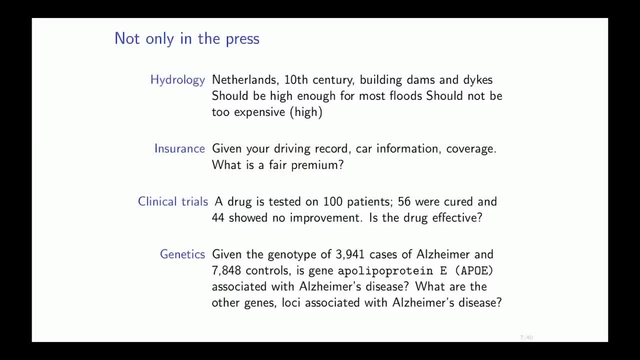 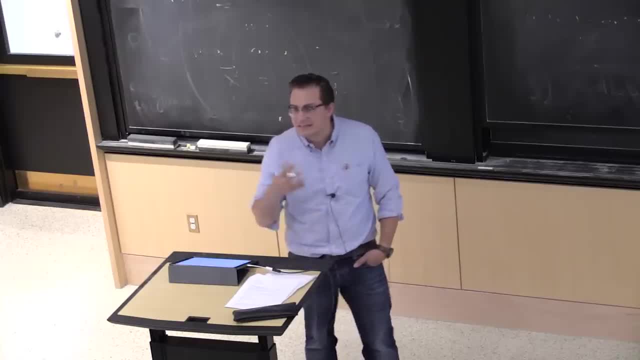 there are genes within the genes in the particular SNPs that I can actually look at, And they're looking at very different questions. Now, when you start asking all these questions, you have to be careful, because you're reusing your data again and it might lead you to wrong conclusions. 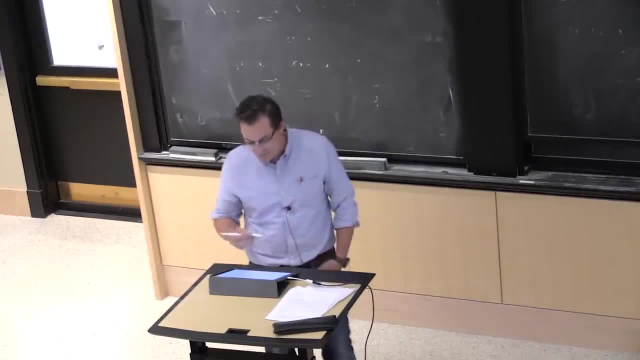 And those are all over the place these days And that's why they go all the way to John Oliver talking about them. Any questions about those examples? So this is really a motivation. Again, we're not going to just take this data set of those cases and look at them in details. 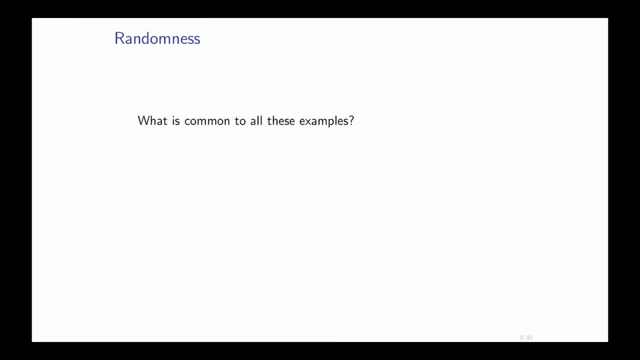 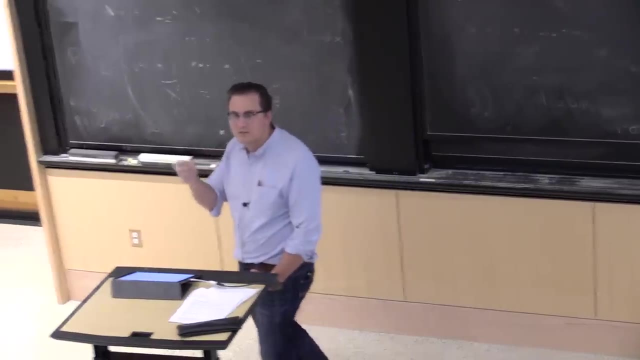 So what is common to all these examples? Why do we have to use statistics for all these things? Well, there's the randomness of the data. There's some effect that we just don't understand. So, for example, the randomness associated with the lighting up of some voxels, or the fact 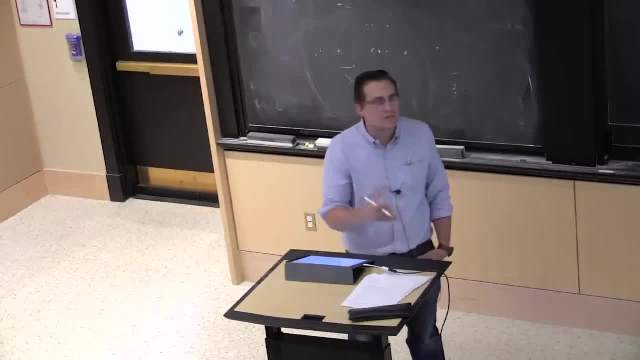 that, as far as the insurance is concerned, whether you're going to break your iPhone or not is essentially a coin cost. Hopefully it's biased, but it's a coin cost. So all these things from the perspective of the statistician, those things. 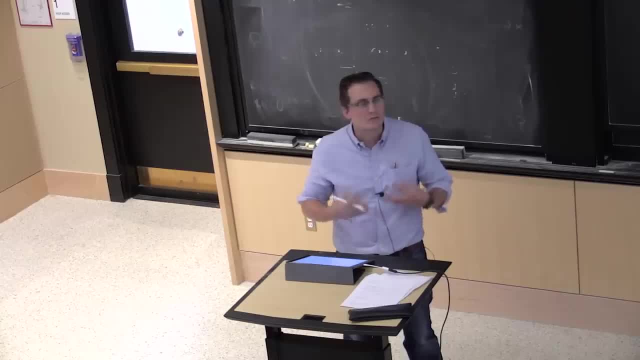 are actually random events And we need to tame this randomness to understand this randomness. Is it going to be a lot of randomness or is it going to be little randomness? Is it going to be something that's like out of their people, out of so? let's see. 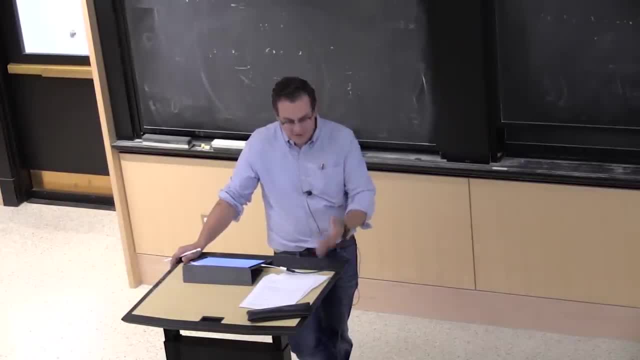 for example, for the floods right Did the floods that I see were consistently almost the same size, with almost the rounding error, or they're just really widespread. All these things we need to understand so we can understand how to build those dikes. 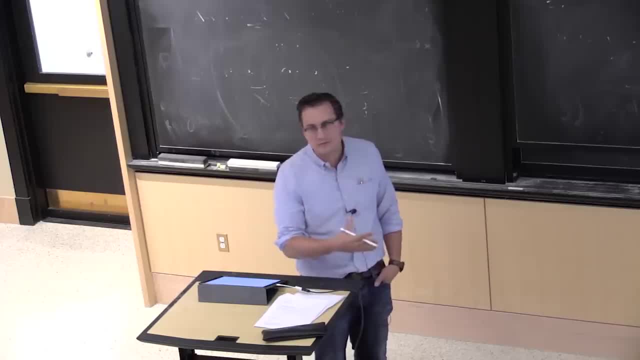 So those are very important questions because we have the technology to target those things, but we need the answers about what those things are. And so there's a bunch of other questions that the minute you're going to talk to a biologist about, say, I can do this and say OK there. 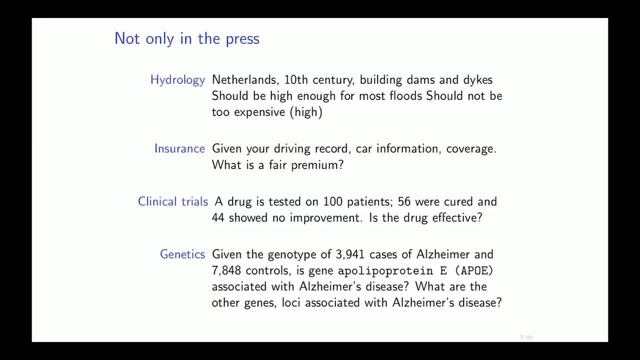 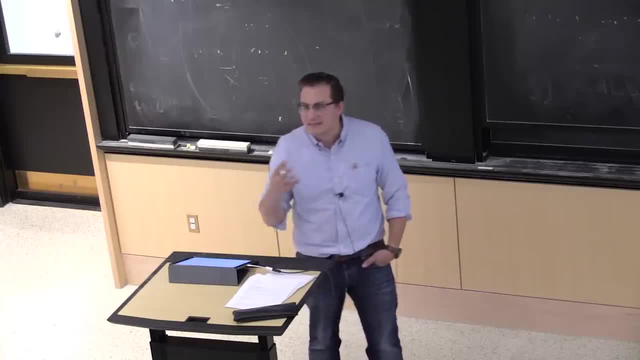 are genes within the genes, the particular SNPs, that I can actually look at, And they're looking at very different questions. Now, when you start asking all these questions, you have to be careful, because you're reusing your data again And it might lead you to wrong conclusions. 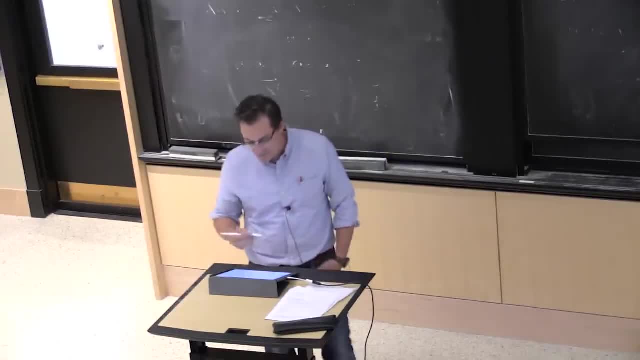 And those are all over the place these days And that's why they go all the way to John Oliver talking about them. Any questions about those examples? So this is really a motivation. Again, we're not going to just take this data set of those cases and look at them in details. 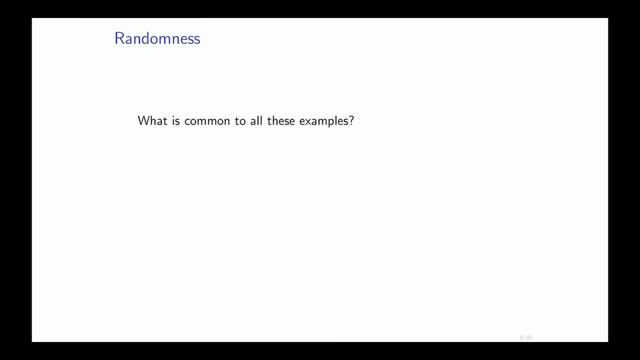 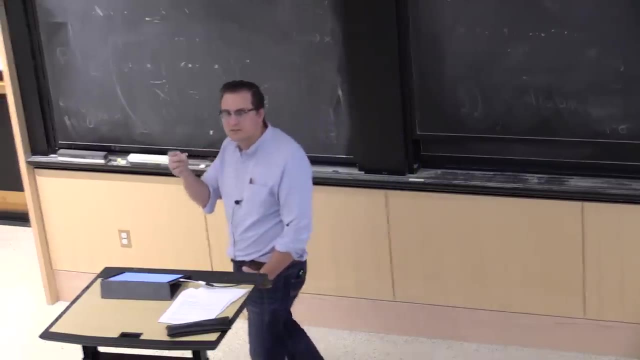 So what is common to all these examples? Why do we have to use statistics for all these things? Well, there's the randomness of the data. There's some effect that we just don't understand. So, for example, the randomness associated with the lighting up of some voxels. 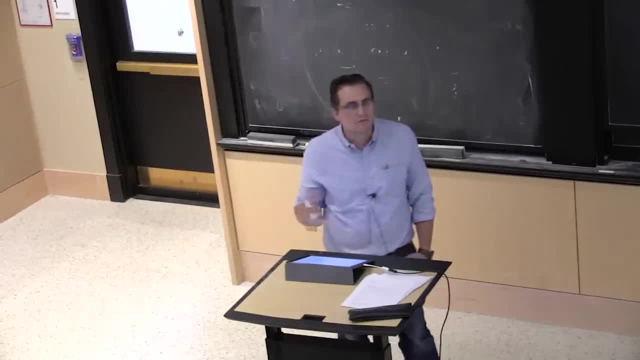 or the fact that, as far as the insurance is concerned, whether you're going to break your iPhone or not is essentially a coin cost. Hopefully it's biased, but it's a coin cost. So all these things from the perspective of the statistician, those things. 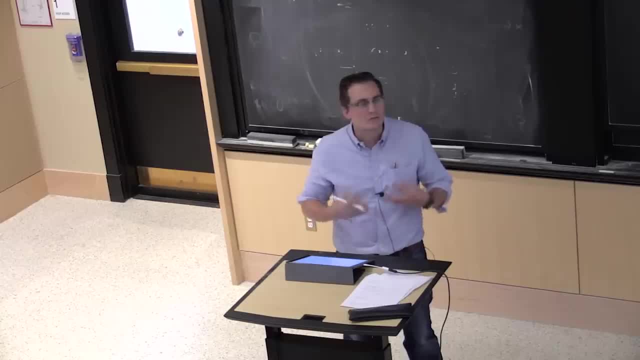 are actually random events And we need to To tame this randomness, to understand this randomness. is it going to be a lot of randomness or is it going to be little randomness? Is it going to be something that's like out of their people, out of so? let's see. 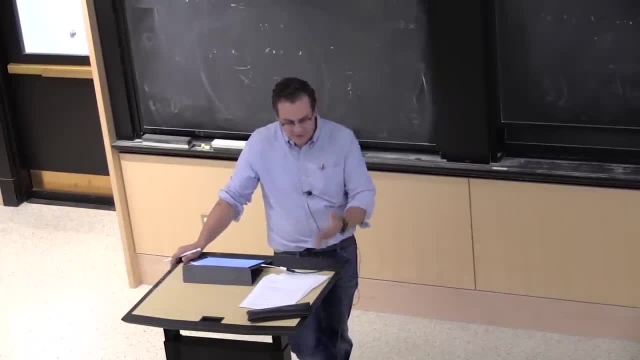 for example, for the floods right Did the floods that I see were consistently almost the same size, with almost the rounding error, or they're just really widespread. All these things we need to understand so we can understand how to build those dikes. 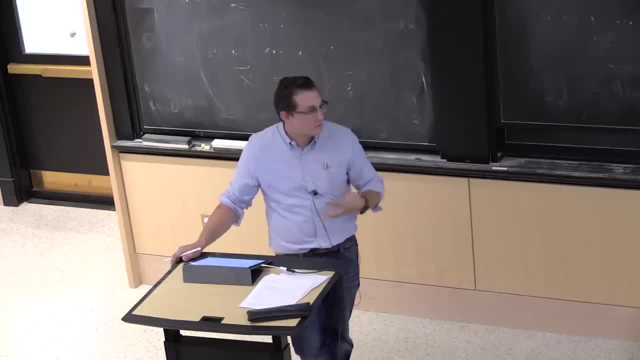 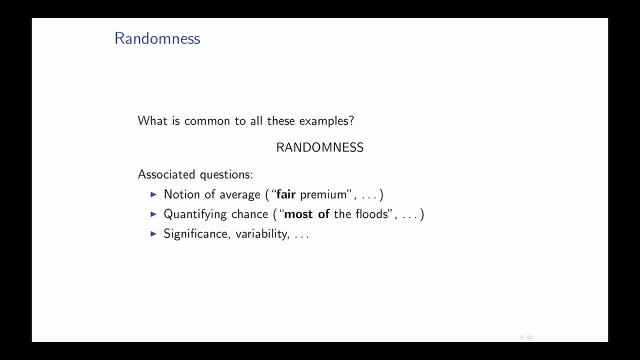 or how to build. We need to understand how to make decisions based on those data and we need to understand this randomness. So the associated questions to randomness were actually hidden in the text. So we talked about the notion of average. So, as far as the insurance is concerned, 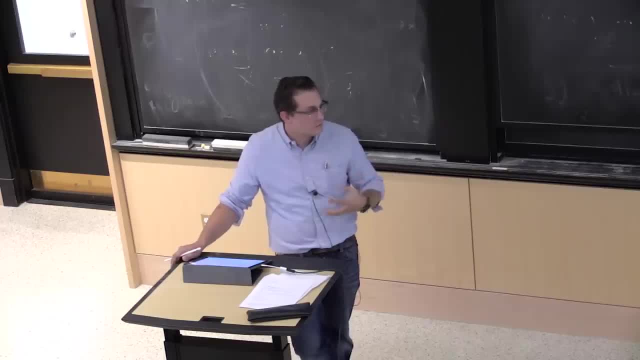 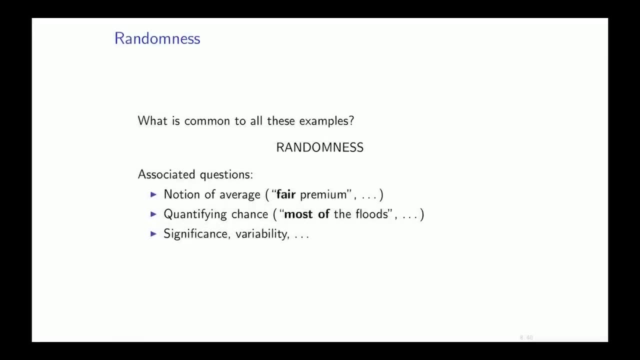 or how to build some. We need to make decisions based on those data and we need to understand this randomness. So the associated questions to randomness were actually hidden in the text. So we talked about the notion of average. So, as far as the insurance is concerned, 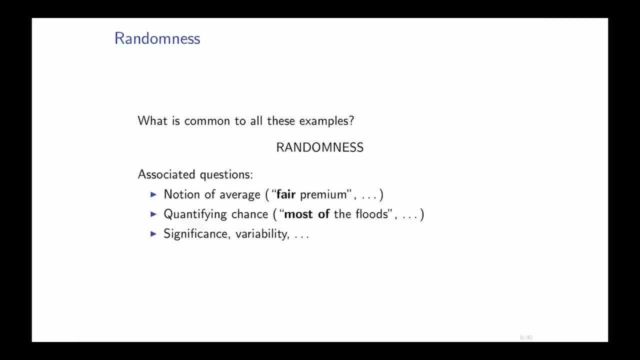 they want to know, in average, what the probability is, What is your chance of actually breaking your iPhone? And that's what came in this notion of fair premium. There's this notion of quantifying chance. Right, We want to talk, maybe, only about average. 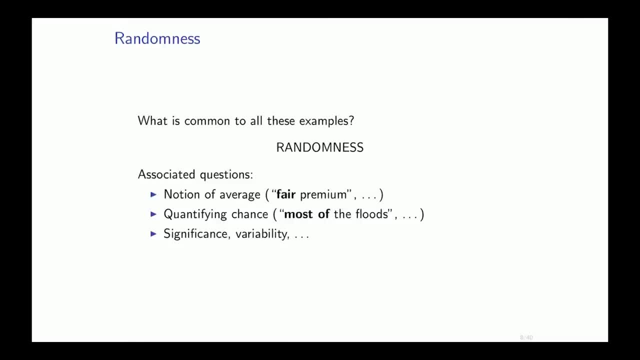 Maybe we want to cover, say, 99% of the floods, So we need to know what is the height of a flood that's higher than 99% of the floods, But maybe there's 1% of them when doomsday come. 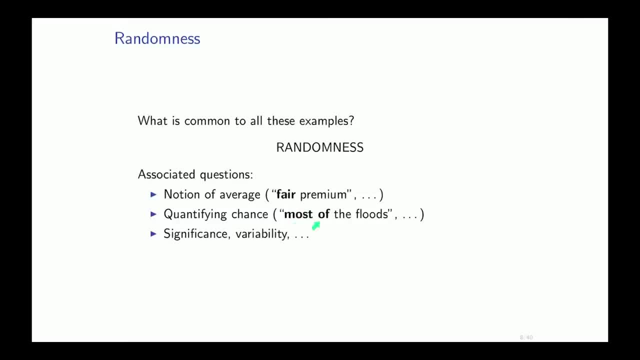 doomsday comes right. We're not going to pay for it. All right. so that's most of the floods, And then there's questions of significance, right? So I gave this example a second ago about clinical trials. I gave you some numbers. 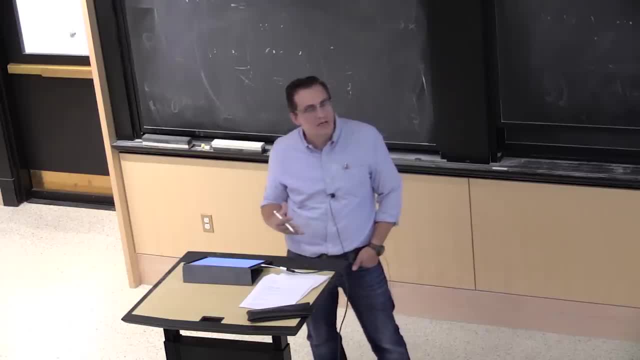 Clearly the drug cured more people than it did not, But does it mean that it's significantly good? or was this just by chance? Maybe it's just that these people just recover. It's like curing a common cold And you feel like, oh, I got cured. 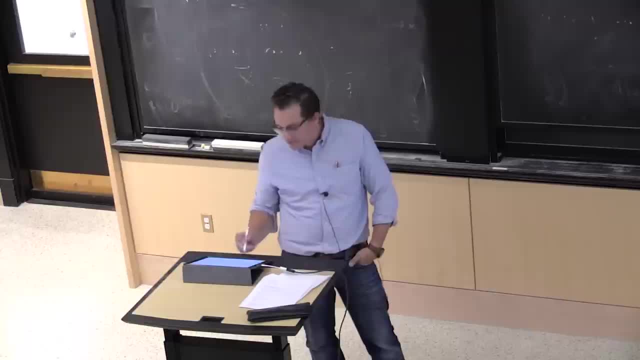 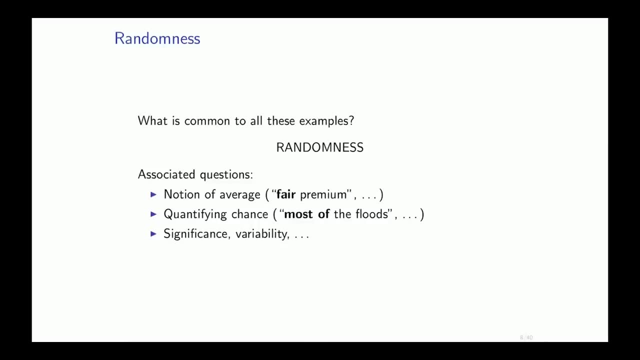 But it's really. you waited five days and then you got cured, All right. so there's this notion of significance of variability. All these things are actually notions that describe randomness and quantify randomness into simple things. Randomness is a very complicated B. 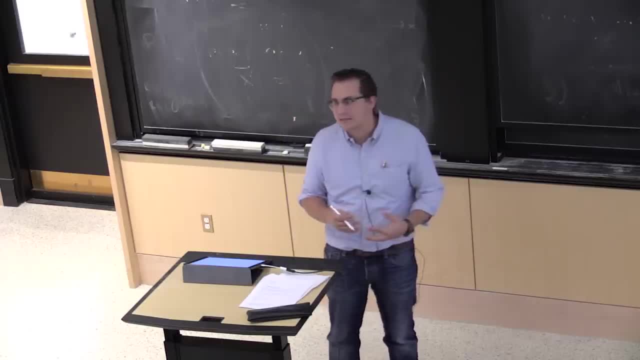 But we can summarize it into things that we understand. Just like I am a complicated object, I'm made of molecules, I'm made of genes. I'm made of very complicated things, But they can be summarized as my name, my email address. 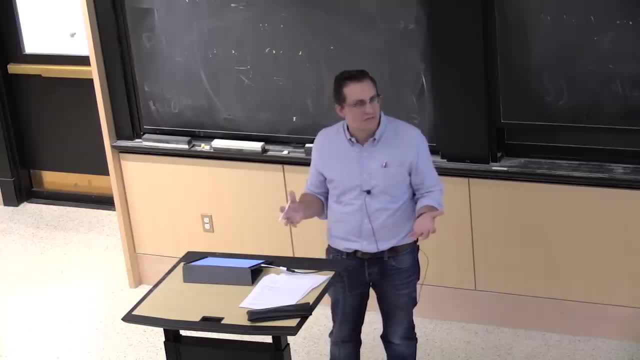 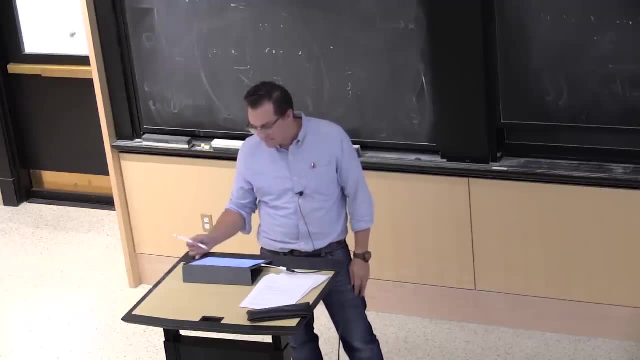 my height and my weight, And maybe for most of you this is basically enough. All right, so you will recognize me without having to do a biopsy on me every time you see me. All right, so to understand randomness, you had to go through probability. 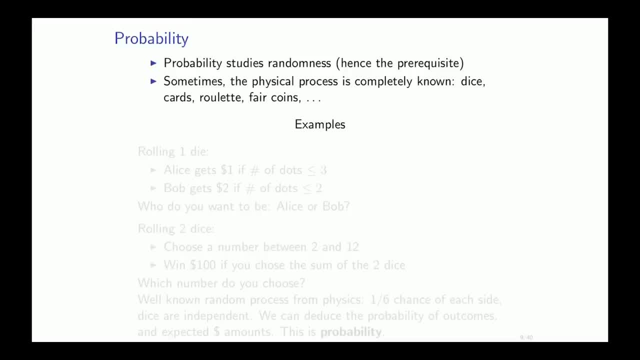 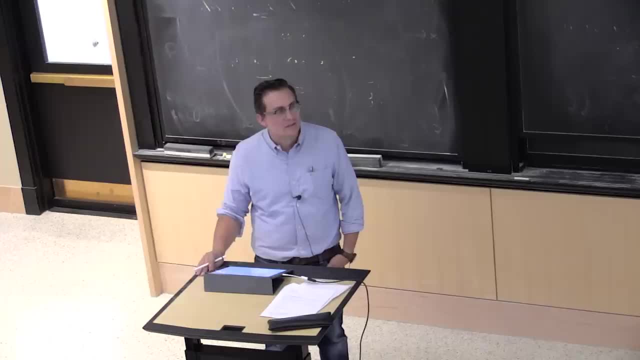 All right, probability is the study of randomness. That's what it is. That's what the first sentence that a lecturer in probability will say, And so that's why I need the prerequisite, because this is what we're going to use to describe the randomness. 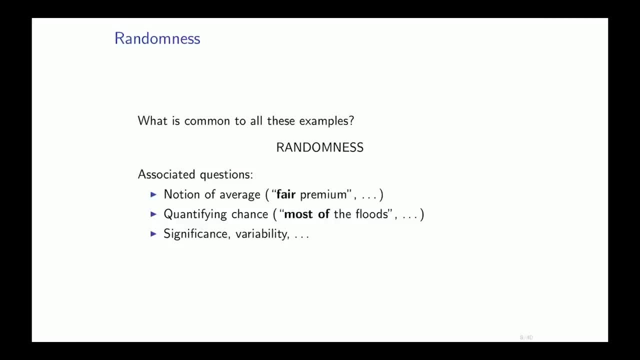 they want to know, in average, what the probability is, What is your chance of actually breaking your iPhone? And that's what came in this notion of fair premium. There's this notion of quantifying chance. We don't want to talk, maybe only about average. 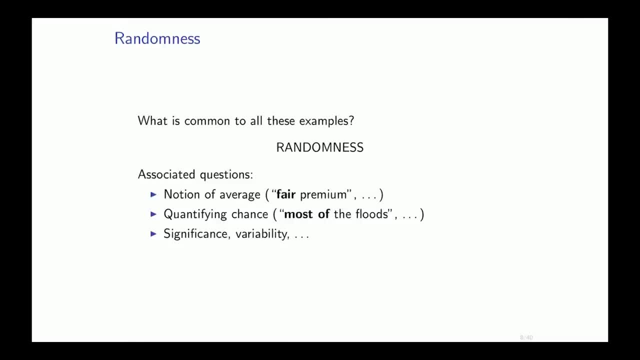 Maybe we want to cover, say, 99% of the floods, So we need to know what is the height of a flood that's higher than 99% of the floods, but maybe there's 1% of them. When doomsday comes, doomsday comes. 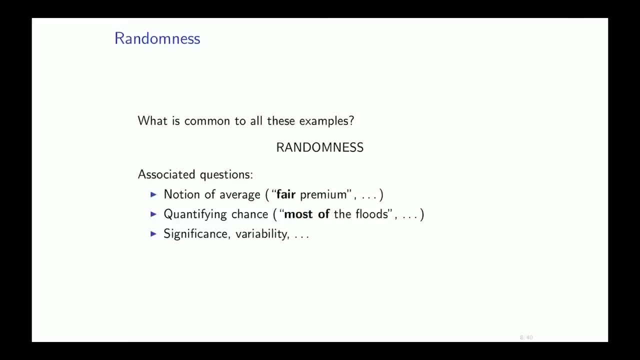 We're not going to pay for it. So that's most of the floods. And then there's questions of significance. So I gave this example a second ago about clinical trials, I gave you some numbers. Clearly, the drug cured more people than it did not. 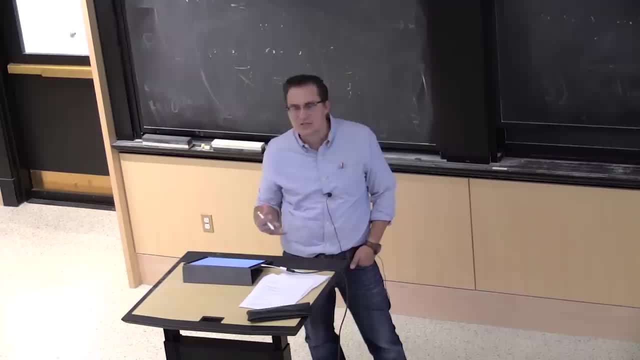 But does it mean that it's significantly good, or was this just by chance? Maybe it's just that these people just recover? It's like curing a common cold And you feel like, oh, I got cured. But it's really. you waited five days and then you got cured. 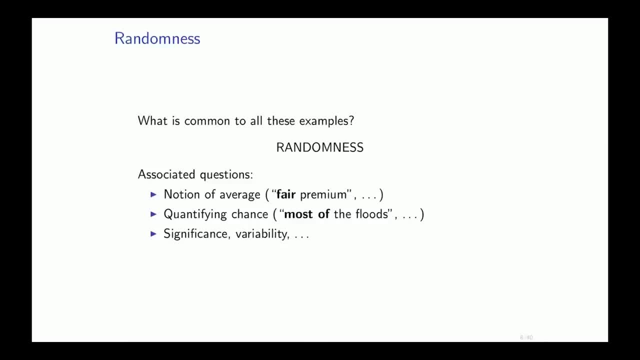 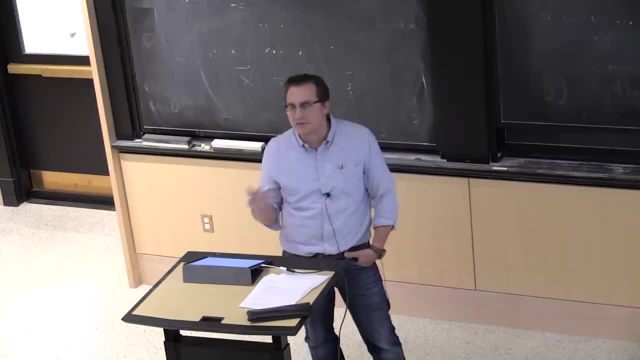 So there's this notion of significance of variability. All these things are actually notions that describe randomness and quantify randomness, And so you can summarize randomness into simple things. Randomness is a very complicated beast, but we can summarize it into things that we understand. 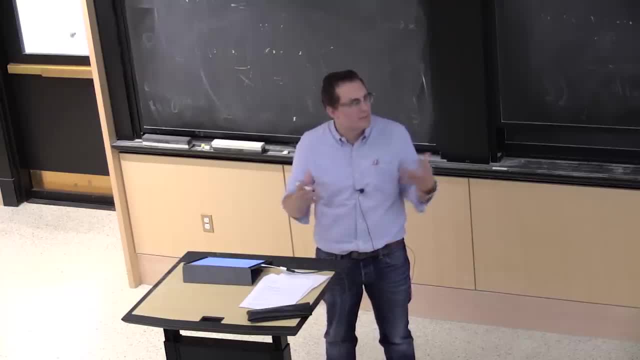 Just like I am a complicated object. I'm made of molecules, I'm made of genes. I'm made of very complicated things, But they can be summarized as my name, my email address, my height and my weight, And maybe for most of you, this is basically enough. 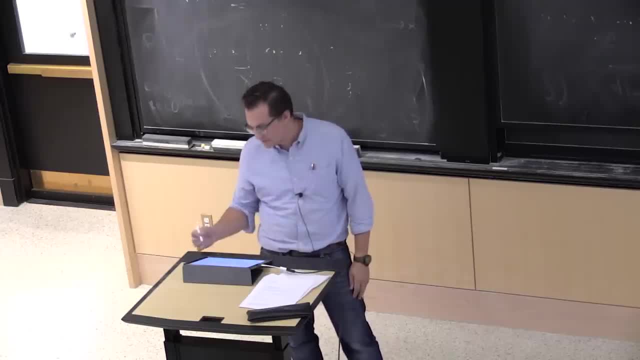 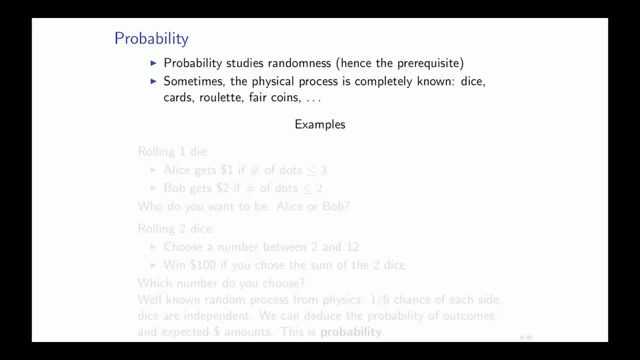 You will recognize me without having to do a biopsy on me every time you see me. All right, So to understand randomness, you had to go through probability. All right, Probability is the study of randomness. That's what it is. That's what the first sentence that a lecturer in probability 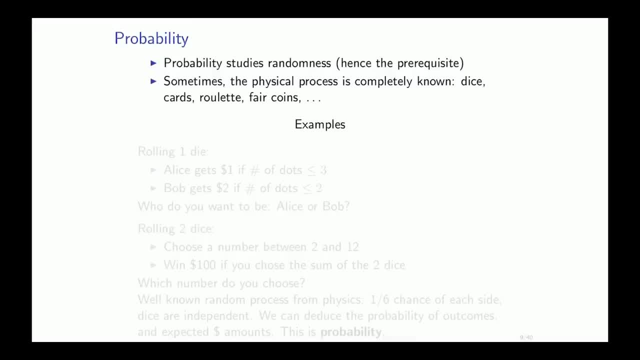 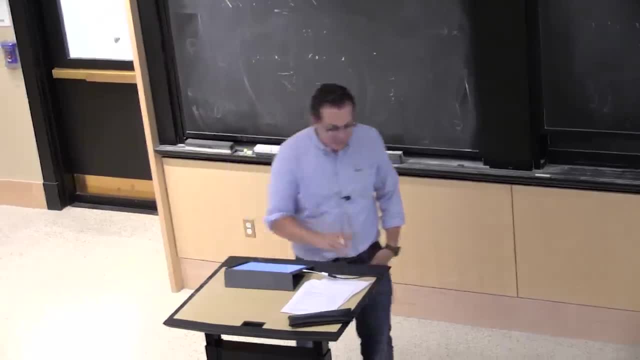 will say: And so that's why I need the prerequisite, because this is what we're going to use to describe the randomness. We'll see in a second how it interacts with statistics. So sometimes, and actually probably most of the time, throughout your semester on probability. 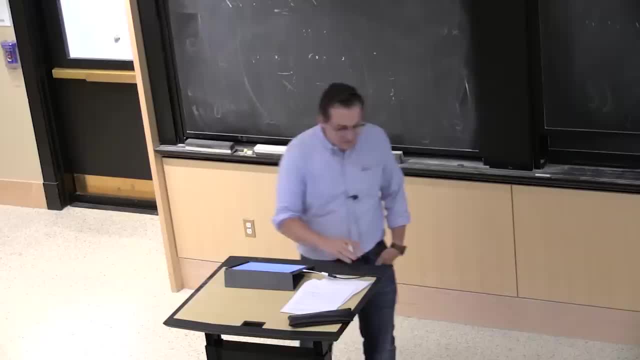 We'll see in a second how it interacts with statistics. So sometimes, and actually probably most of the time, throughout your semester on probability, randomness was very well understood. When you saw a probability problem, here was the chance of this happening. Here was the chance of that. 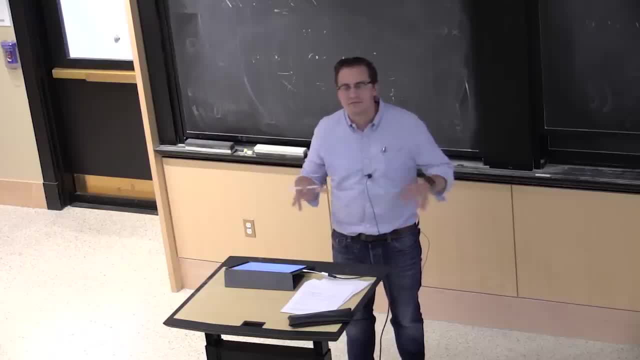 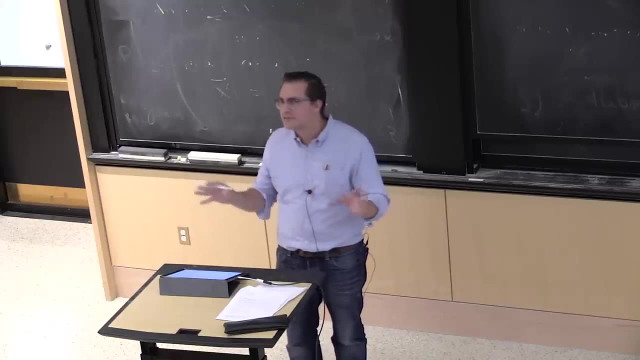 Here was the chance of that happening. Maybe you had more complicated questions, that you had some basic elements to answer. For example, the probability that I have HBO is this much And the probability that I watch Game of Thrones is that much, And given that I play basketball, what is the probability? 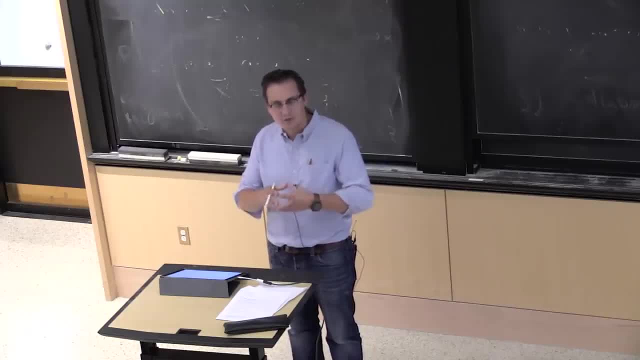 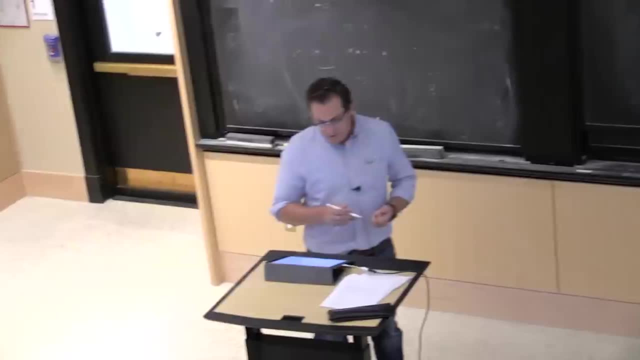 You had all these crazy questions, but you were able to build them And all the basic numbers were given to you. Statistics will be about finding those basic numbers All right. so some examples that you've probably seen were dice cards, roulette, flipping coins. 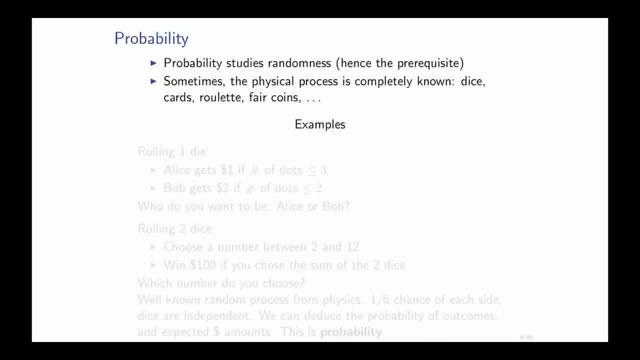 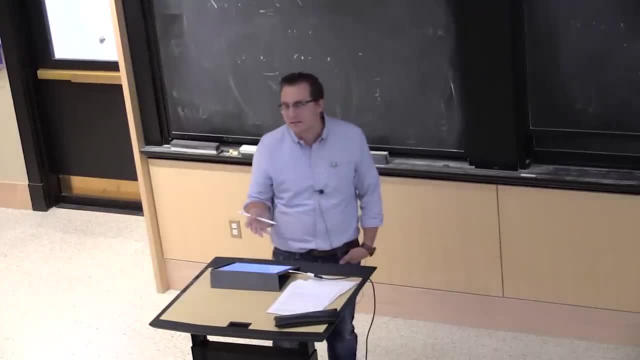 All these things are things that you've seen in a probability class, And the reason is because it's very easy to describe the probability of each outcome For a die. we know that each face is going to come with probability one sec. Now I'm not going to go into debate. 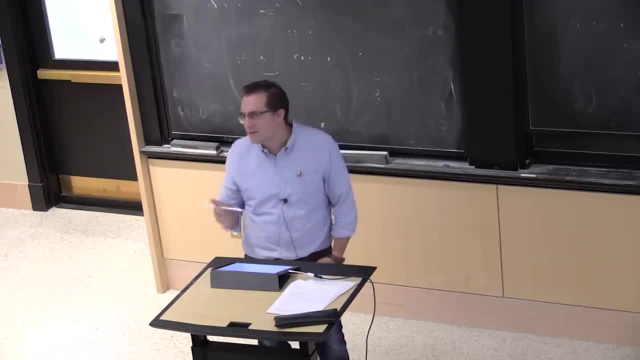 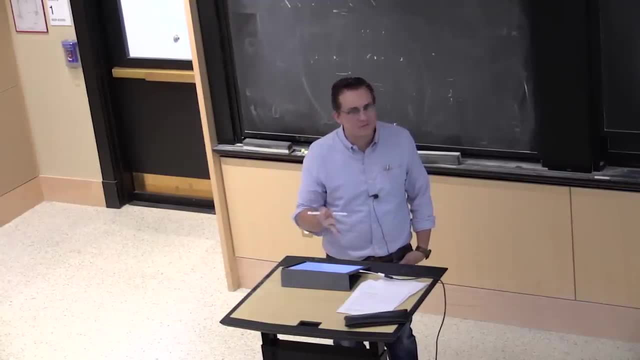 of whether this is pure randomness or this is determinism. I think as a model for actual randomness, die is a pretty good number. Flipping a coin is a pretty good model- OK, But those are actually a good thing. So the questions that you would see, for example, in: 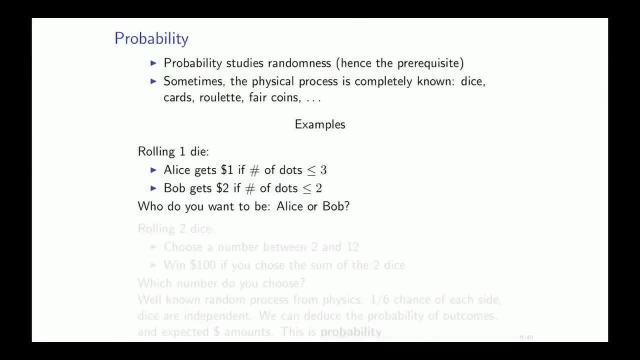 probabilities are the following. I roll one die. Alice gets $1 if the number of dots is less than 3.. Bob gets $2 if the number of dots is less than 2.. Do you want to be Alice or Bob? given that your goal is? 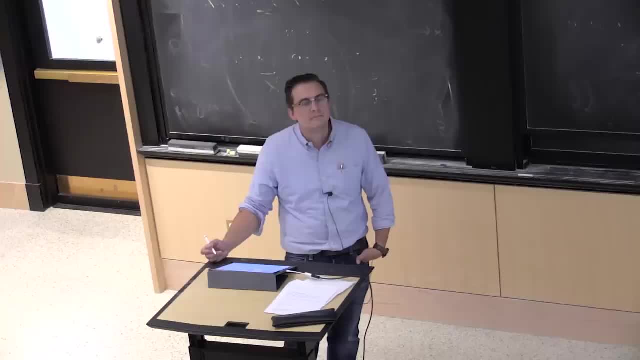 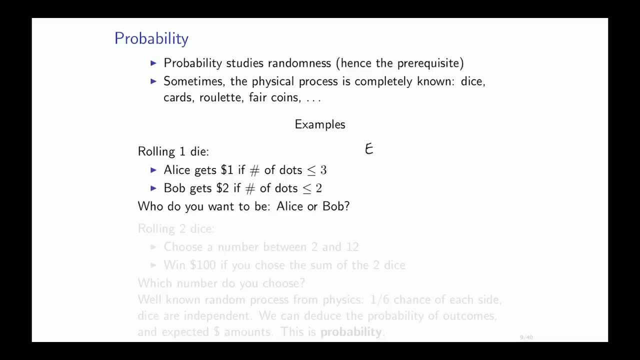 actually to make money. Yeah, You want to be Bob, right? So let's see why. So, if you look at the expectation of what Alice makes, so let's call it A. This is $1 with probability 1 1⁄2, right. 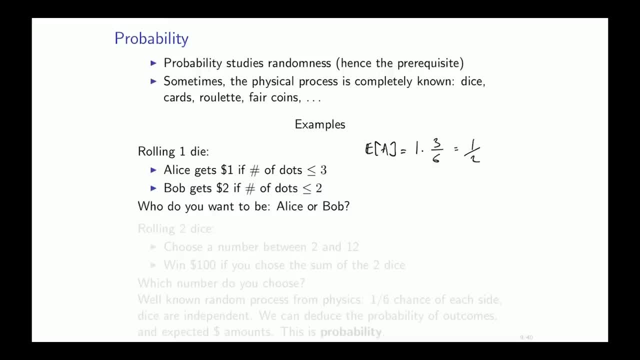 So 3, 6,, so that's 1, 1⁄2.. And the expectation of what Bob makes this is $2, with probability 2, 6, and that's 2, 1⁄3, which is definitely larger than 1 1⁄2.. 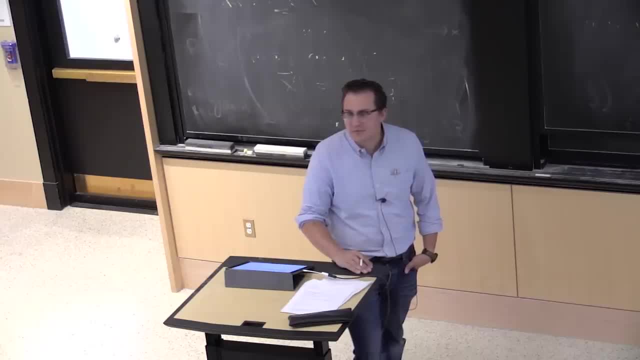 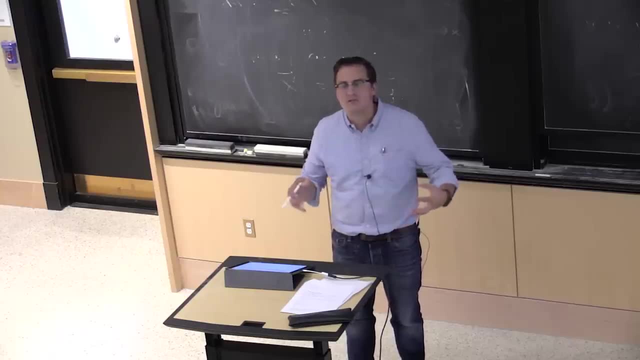 randomness was very well understood. When you saw a probability probability- you were like, oh, this is a very good problem. Here was the chance of this happening. Here was the chance of that happening. Maybe you had more complicated questions, that you had some basic elements to answer. 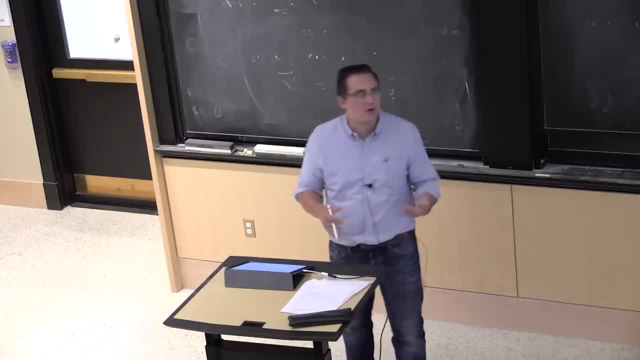 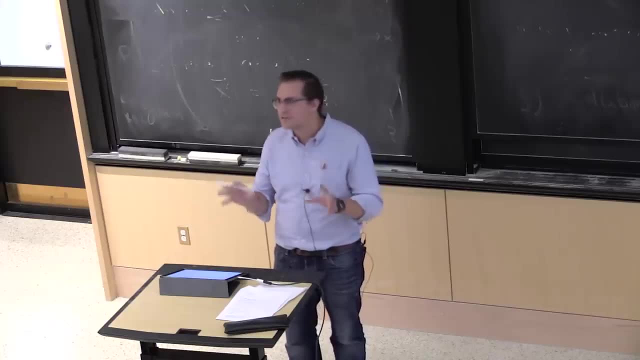 For example, the probability that I have HBO is this much And the probability that I watch Game of Thrones is that much, And, given that I play basketball, what is the probability? You had all these crazy questions, but you were able to build them. 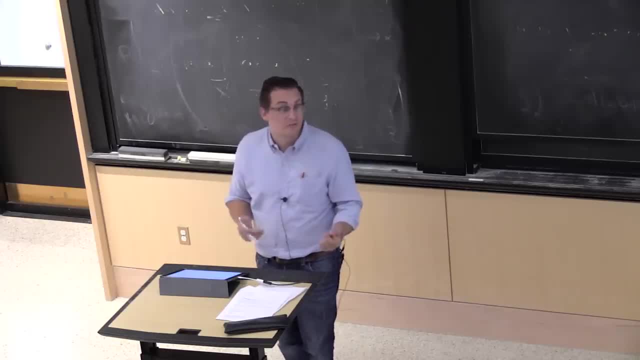 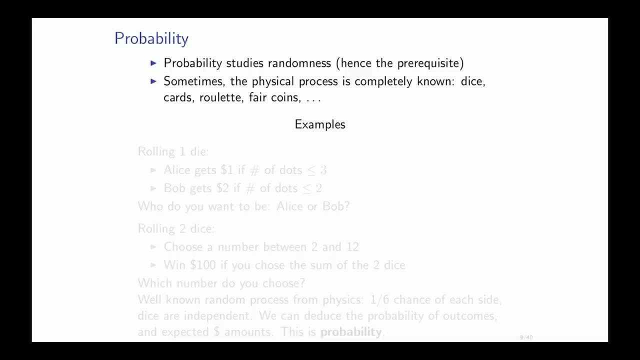 But all the basic numbers were given to you. Statistics will be about finding those basic numbers, All right. so some examples that you've probably seen were dice cards, roulette, flipping coins. All these things are things that you've seen in a probability class. 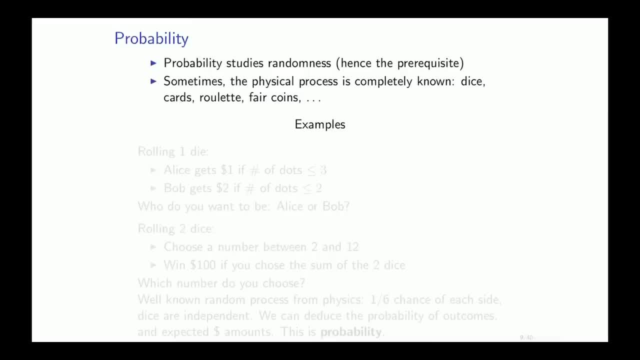 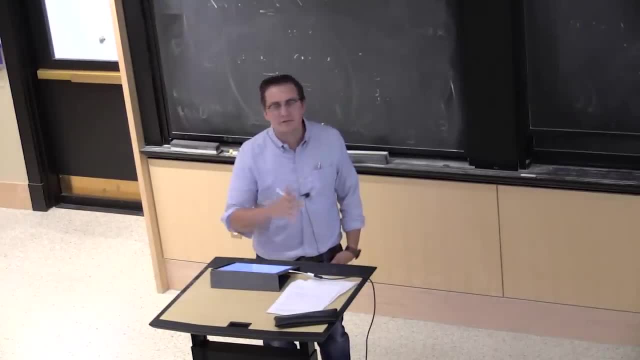 And the reason is because it's very easy to describe the probability of each outcome For a die. we know that each face is going to come with probability one set. Now I'm not going to go into debate of whether this is pure randomness. 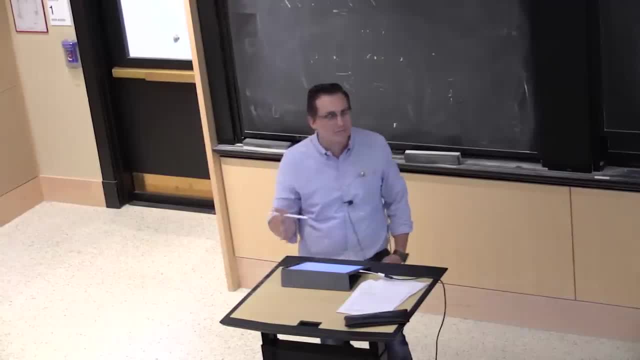 or this is determinism, I think, as a model for actual randomness, a die is a pretty good example. A die is a pretty good number. Flipping a coin is a pretty good model, So those are actually a good thing. So the questions that you would see, for example, 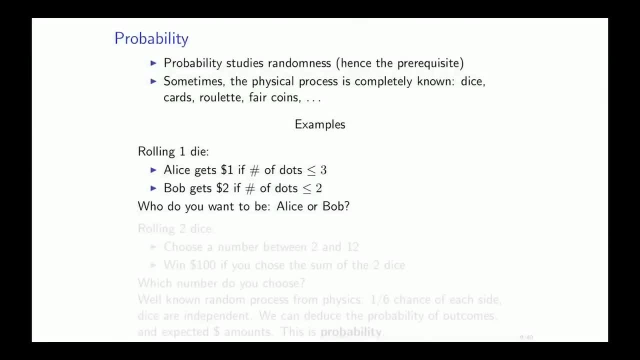 in probabilities are the following: I roll one die. Alice gets $1 if the number of dots is less than 3.. Bob gets $2 if the number of dots is less than 2.. Do you want to be Alice or Bob? given that your role is actually? 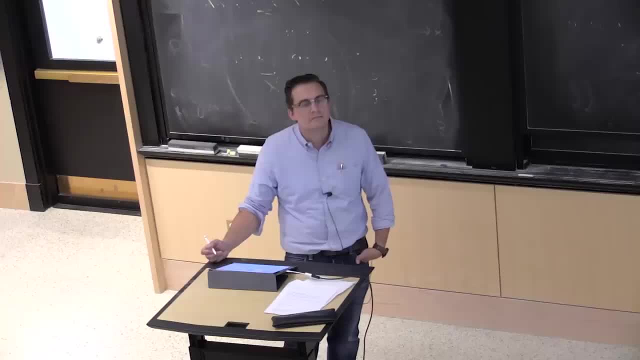 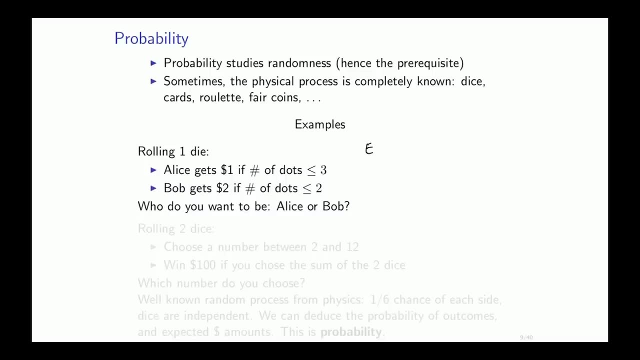 to make money. You want to be Bob, right? So let's see why. Let's look at the expectation of what Alice makes, So let's call it A. This is $1, with probability 1, half right. So 3 sixths. 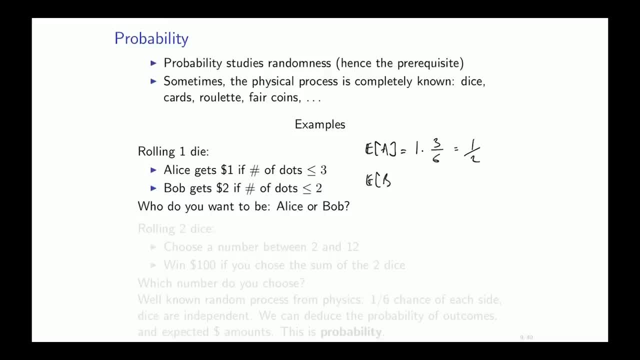 So that's 1 half, And the expectation of what Bob makes this is $2, with probability 2 sixths, And that's 2 thirds, which is definitely larger than 1 half. So Bob's expectation is actually a bit higher. 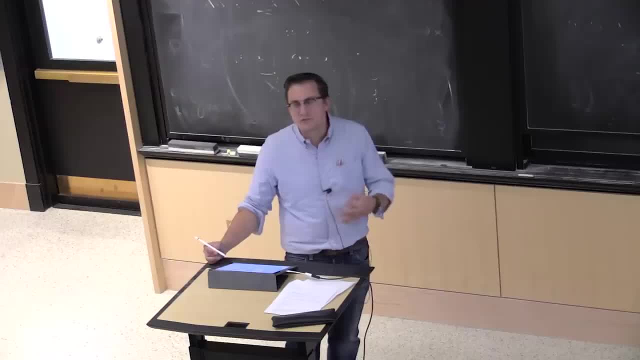 OK, So those are the kind of questions that you may ask with probability I described to you exactly. You used the fact that the die would get less than 3 dots with probability 1 half. You knew that And I didn't have to describe to you what's going on there. 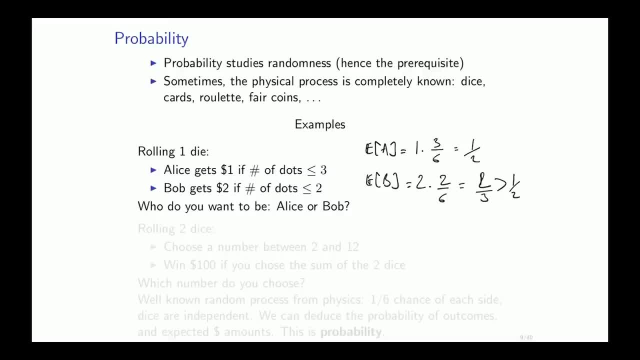 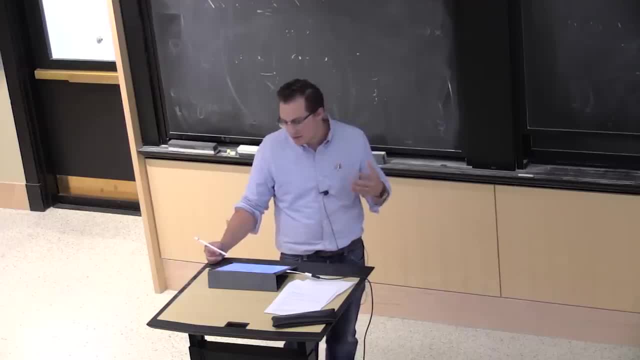 So Bob's expectation is actually a bit higher. OK, So those are the kind of questions that you may ask with probability, And I didn't have to describe to you exactly. You used the fact that the die would get less than 3 dots. 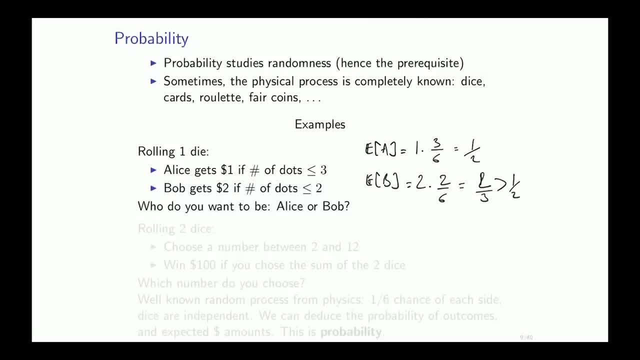 with probability 1 1⁄2.. You knew that and I didn't have to describe to you what's going on there. You didn't have to collect data about a die. Same thing: You roll two dice, You choose a number between 2 and 12, and you win $100. 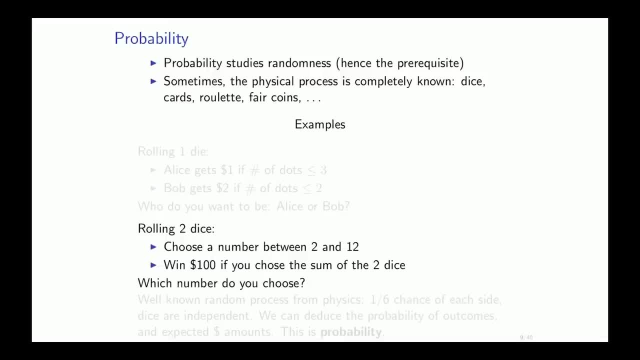 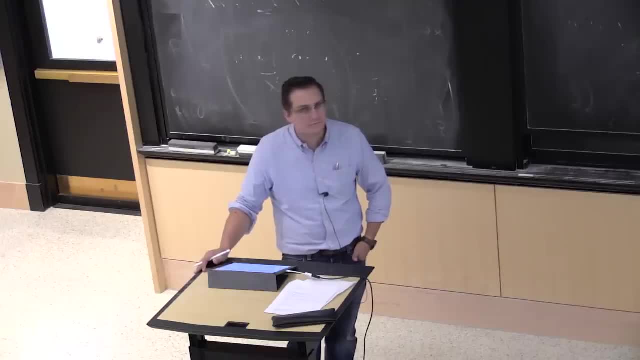 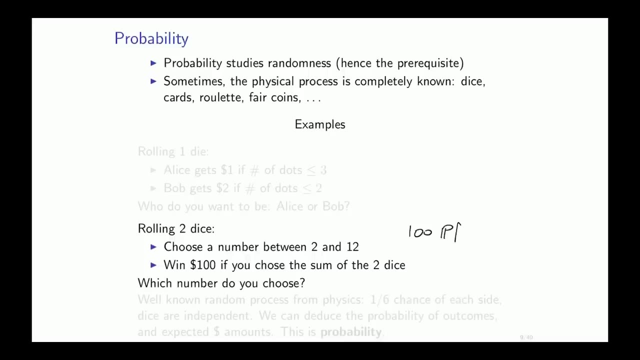 if you choose the sum of the two dice, Which number do you pick? What? 7?? Why 7?? It's the most likely one, right? So your gain here will be $100 times the probability that the sum of the two dice- let's say x plus y. 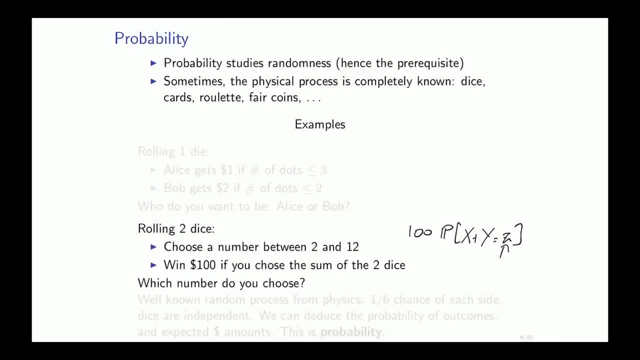 is equal to your little z, where little z is the number you pick. So 7 is the most likely to happen and that's the one that maximizes this function of z, And for this you need to study a more complicated function. 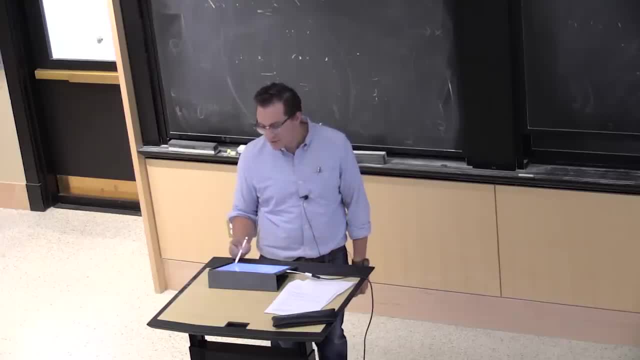 but it's a function that involves two dice. But you can compute The probability that x plus y is equal to z for every z between 2 and 12.. So you know exactly what the probabilities are and that's how you start probability. 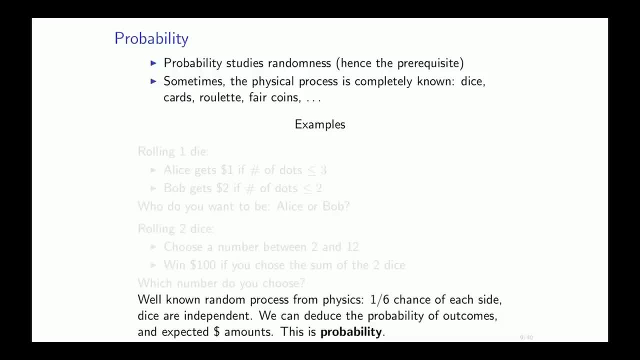 So here that's exactly what I said is, you have a very simple process that describes basic events, probably 1 sixth for each of them, And then you can build up on that and understand the probability of more complicated events. You can throw in some money. 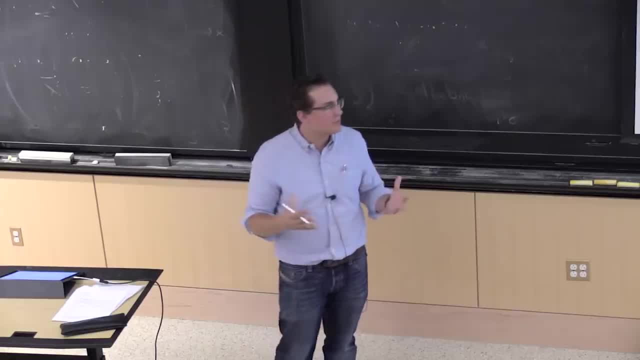 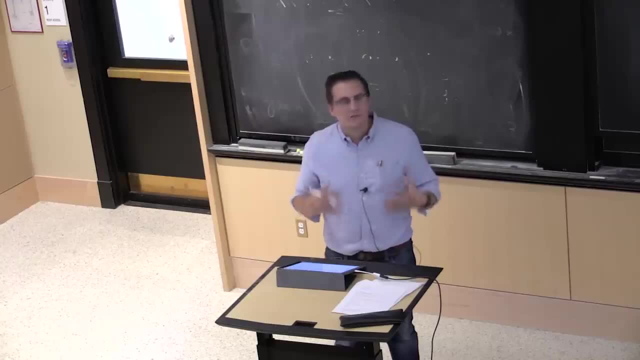 You can put money in there, You can build functions, You can do very complicated things building on that. Now, if I was a statistician, a statistician would be the guy who just arrived on Earth and never seen a die and needs to understand. 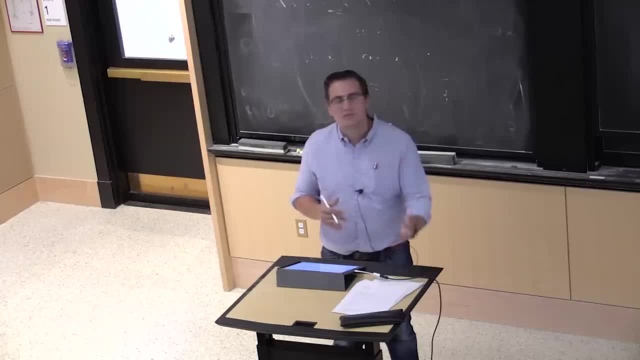 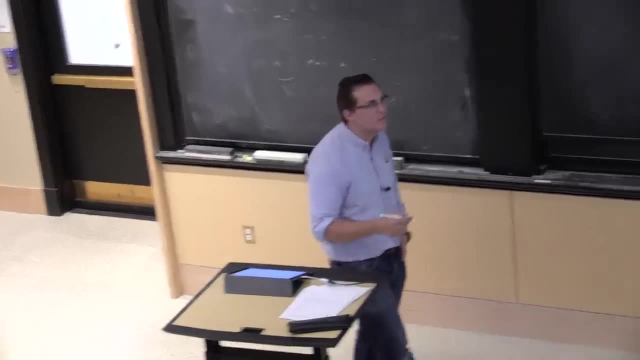 that a die comes with probability 1, sixth on each side, And the way he would do it is just to roll the die until he gets some counts and try to estimate those things, And maybe the guy would come and say: well, actually. 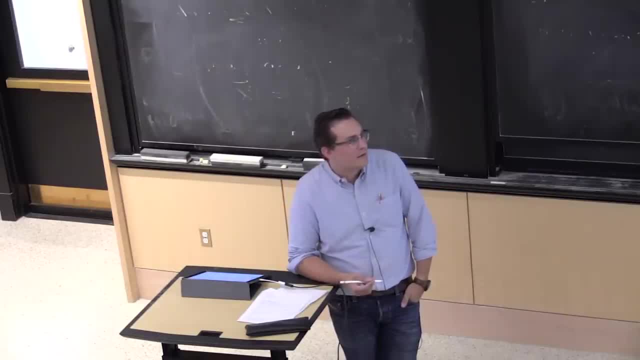 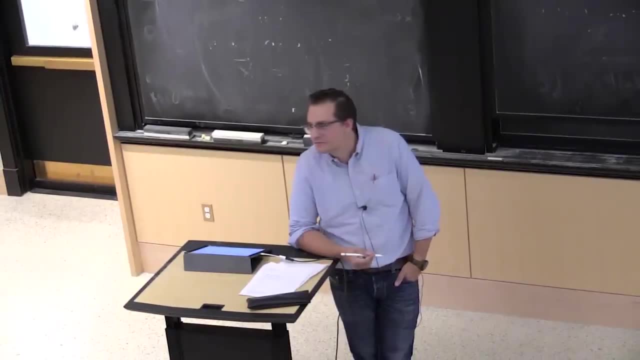 the probability that I get a 1 is 1 sixth plus 0.001.. And the probability that I get a 2 is 1 sixth minus 0.005.. And there would be some fluctuations around this. And it's going to be his role as a statistician to say: 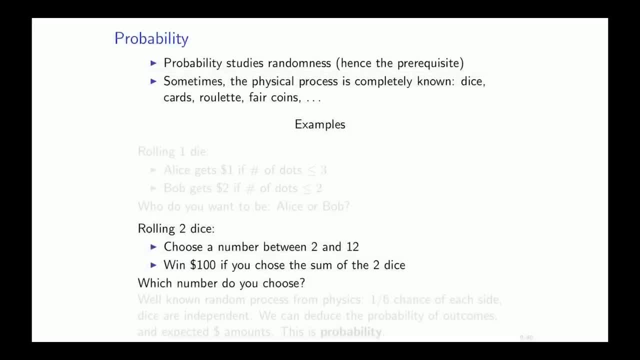 You didn't have to collect data about a die. Same thing: You roll two dies, You choose a number between 2 and 12. And you win $100. if you choose the sum of the two dies, Which number do you pick? 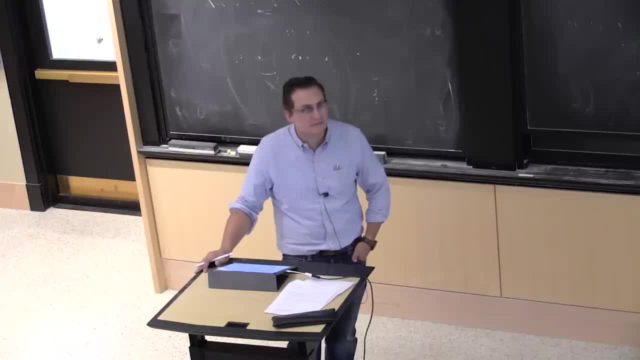 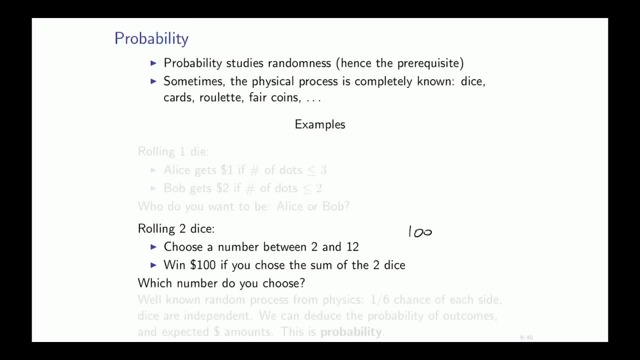 What? 7. 7. Why 7?? It's the most likely one. It's the most likely one, Right? So your gain here will be $100 times the probability that the sum of the two dies. let's say x plus y. 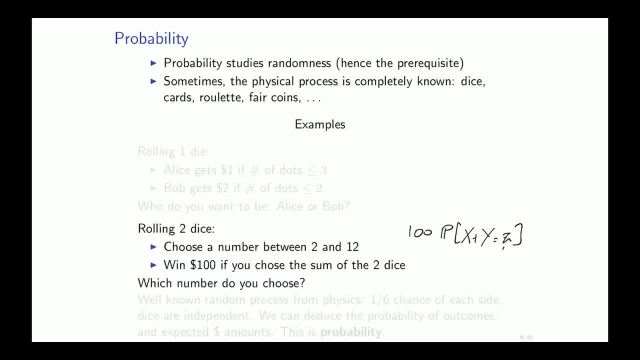 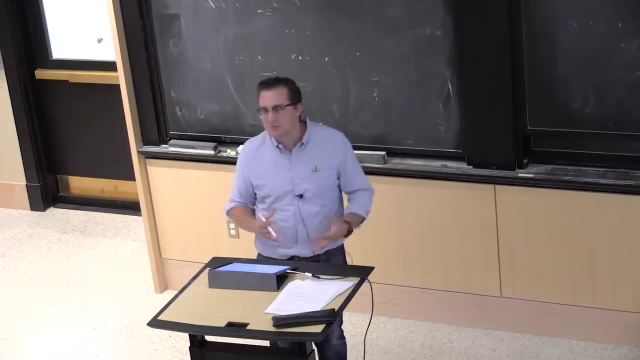 is equal to your little z, where little z is the number you pick. OK, So 7 is the most likely to happen And that's the one that maximizes this function of z. OK, OK, And for this you need to study a more complicated function. 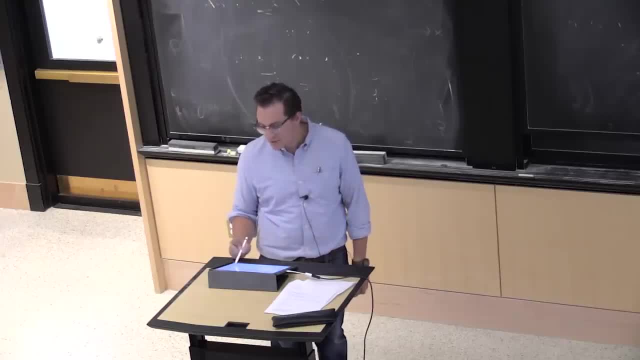 but it's a function that involves two lines. But you can compute the probability that x plus y is equal to z for every z between 2 and 12.. OK, So you know exactly what the probabilities are and that's how you start probability. 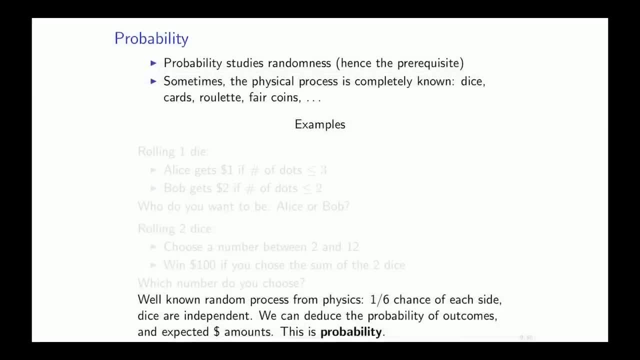 OK, so let's OK. so here, that's exactly what I said- is, you know, you have a very simple process that describes basic events, probably 1, 6 for each of them, And then you can build up on that and understand the probability of more complicated events. 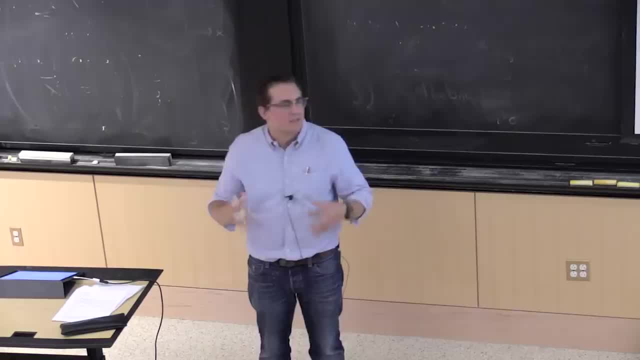 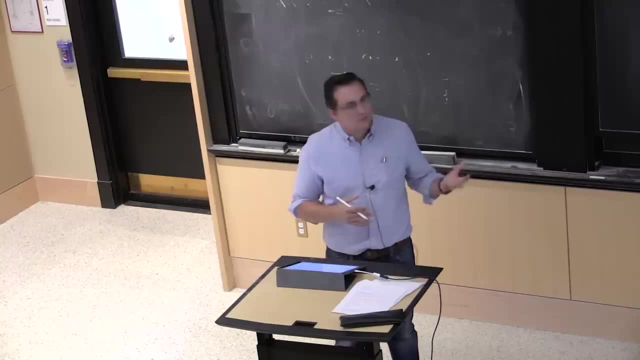 You can throw in some money in there, You can build functions, You can do very complicated things building on that. Now, if I was a statistician, a statistician would be the guy who just arrived on Earth and never seen a die and needs to understand that a die comes. 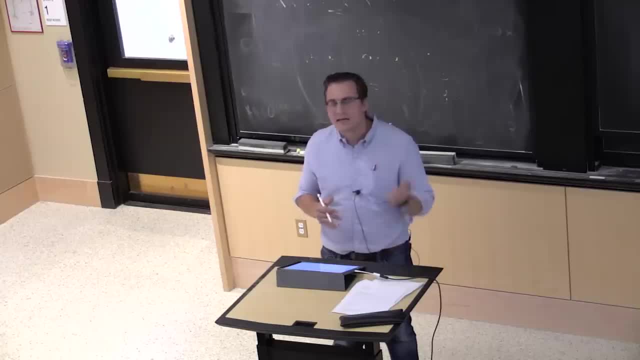 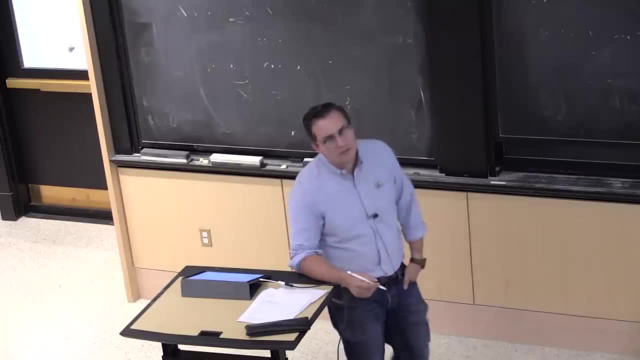 with probability 1- 6 on each side, And the way he would do it is just to roll the die until he gets some counts and try to estimate those things. OK, And maybe the guy would come and say: well, you know. 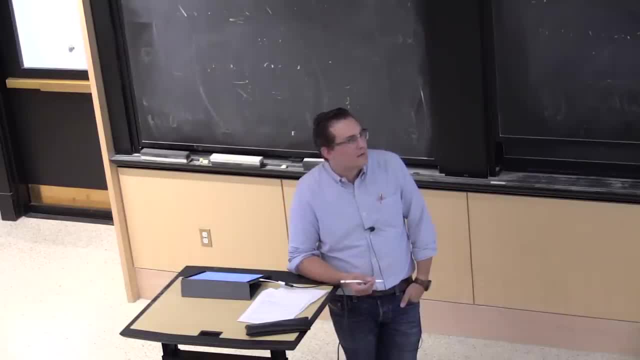 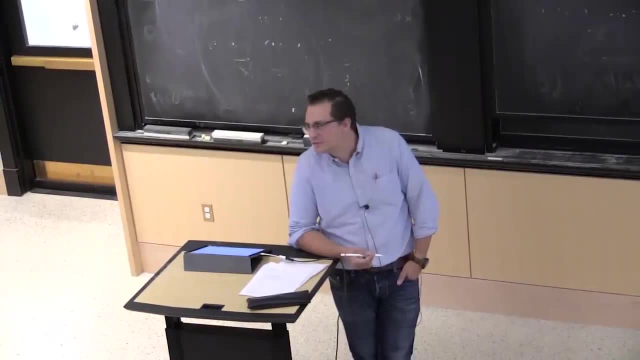 actually, the probability that I get a 1 is 1: 6 plus 0.001.. And the probability that I get a 2 is 1, 6 minus 0.005.. And you know there would be some fluctuations around this. 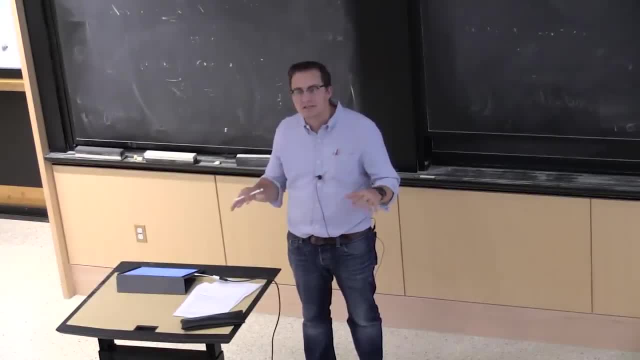 And it's going to be his role as a statistician- to say: listen, this is too complicated of a model for this thing And they should all be the same numbers. Just looking at the data, it should be all the same numbers. 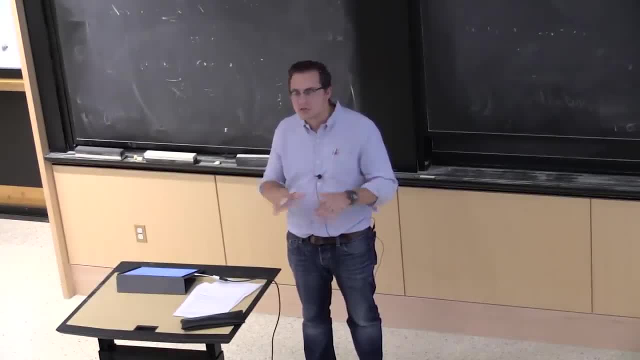 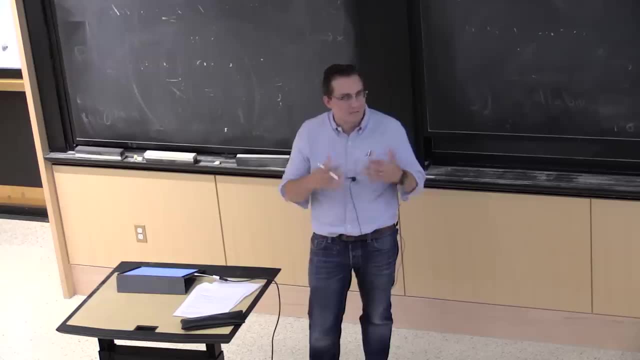 listen, this is too complicated of a model for this thing And they should all be the same numbers. Just looking at the data, it should be all the same numbers And that's part of the modeling. You make some simplifying assumptions that essentially 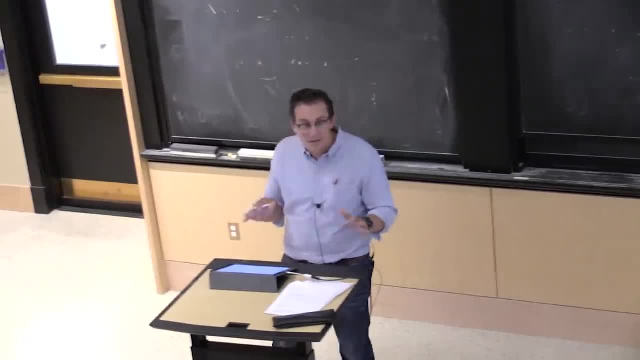 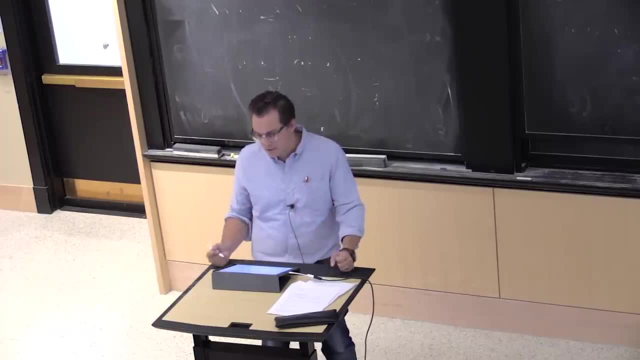 make your questions more accurate. That's the way you do it. If your question is more accurate, now, of course, if your model is wrong, if it's not true that all the faces arrive with the same probability, then you have a model error here. 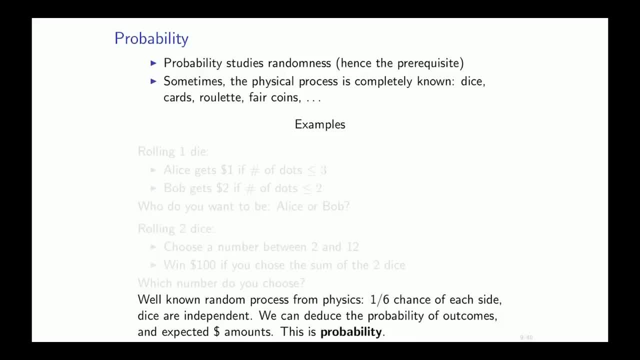 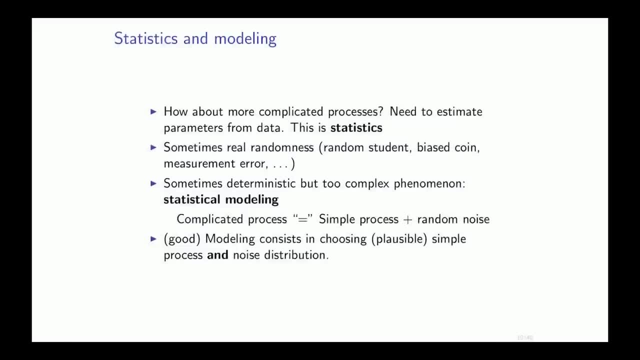 So we will be making model errors, But that's going to be the price to pay to be able to extract anything from our data. OK, so for more complicated processes. so of course, nobody's going to waste their time rolling dice. I'm sure you might have done this in AP Stats or something. 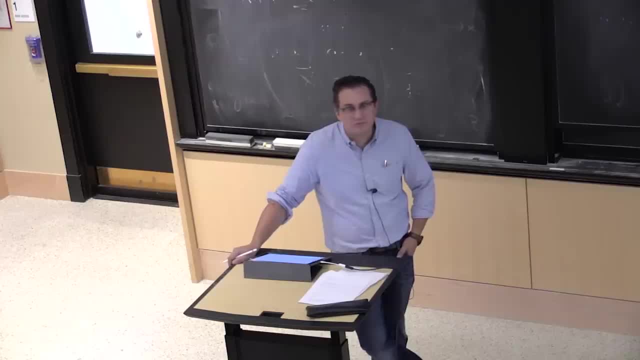 But the need to do it, Yeah, Yeah, The need is to estimate parameters from data, All right. so for more complicated things, you might want to estimate some density parameter on a particular thing set of material, And for this maybe you need to beam something to it. 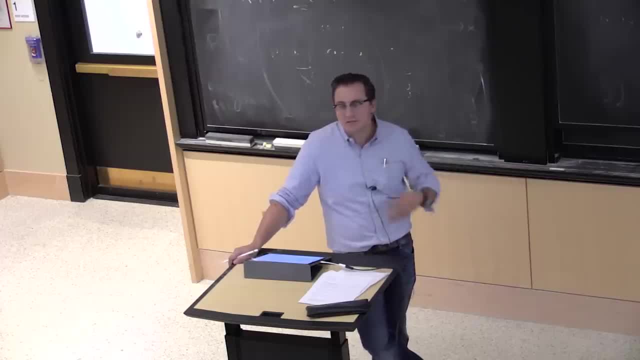 and measure how fast it's coming back And you're going to have some measurement errors And maybe you need to do that several times And you need to have a model for the physical process that's actually going on, And physics is usually a very good way. 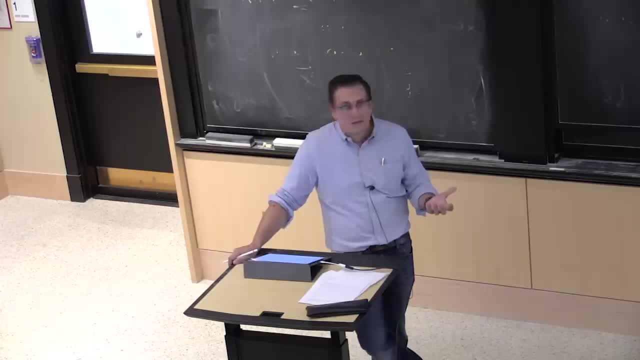 to get models for engineering perspective, But there's models for sociology where we have no physical system right. I mean, God knows how people interact And maybe I'm going to say that the way I make friends is by first flipping a coin in my pocket. 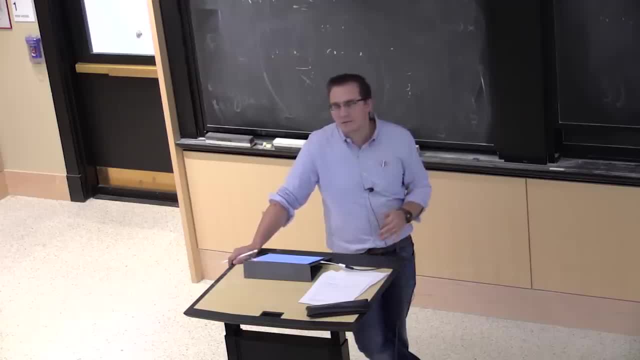 And with probably 2 thirds I'm going to make my friend at work And with probably 1 third, I'm going to make my friend at soccer. And once I make my friend at soccer, I decide to make my friend at soccer. 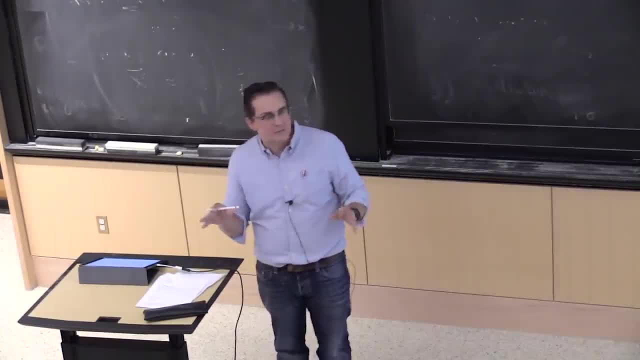 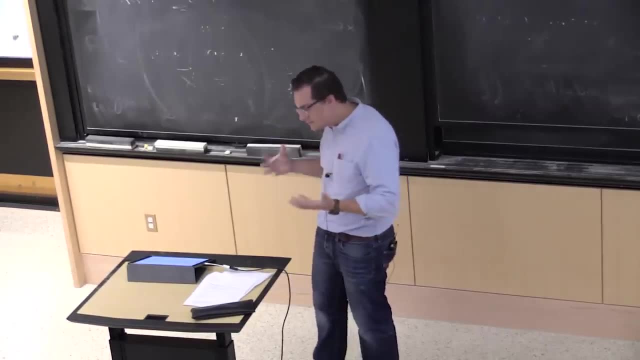 then I will face someone who's flipping the same coin with maybe slightly different parameters, But those things actually go. They actually exist right. There's models about how friendships are formed, And this is the one I described. It's called the mixed membership model. 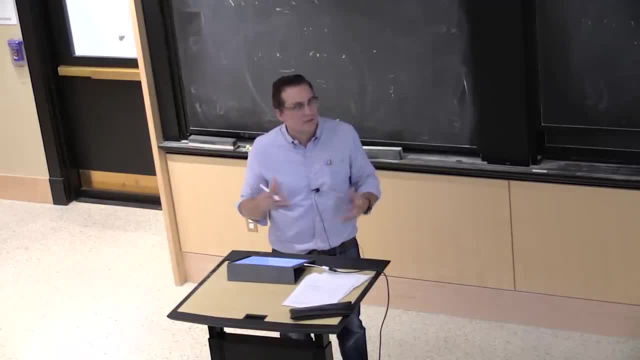 So those are models that are sort of hypothesized And they're more reasonable than there was taking into account all the things that made you meet that person at that particular time. OK, so the goal here? So based on data. now, once we have the model, 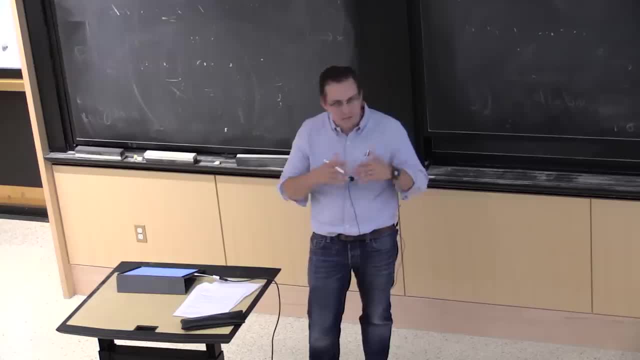 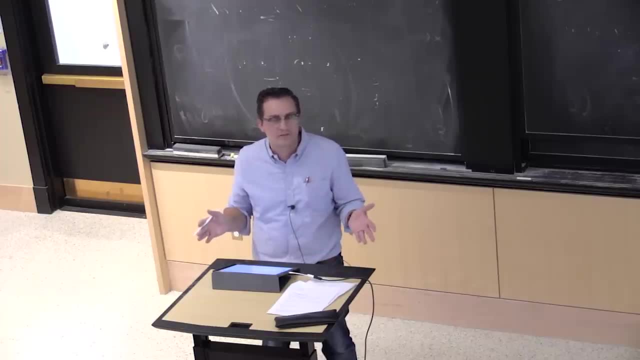 And that's part of the modeling. You make some simplifying assumptions That essentially make your questions more accurate. Now, of course, if your model is wrong, if it's not true that all the faces arrive with the same probability, then you have a model error here. 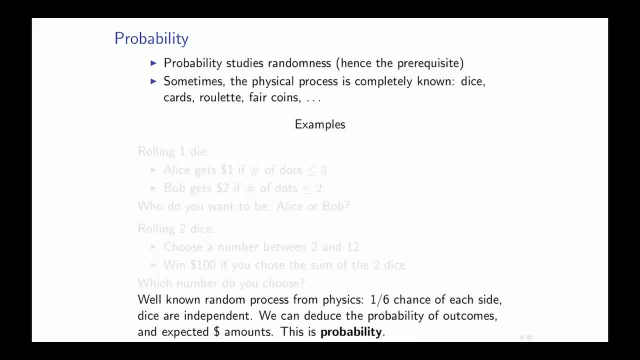 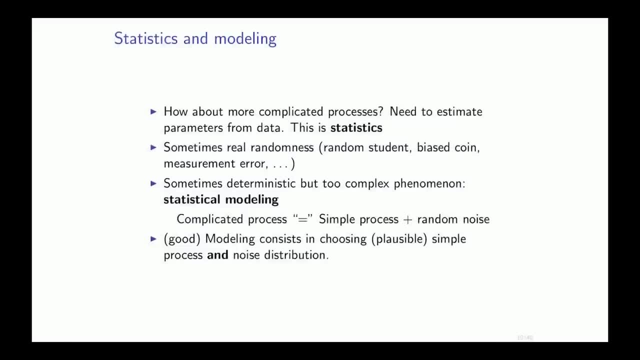 So we will be making model errors, But that's going to be the price to pay to be able to extract anything from our data. OK, so for more complicated processes. so of course, nobody's going to waste their time rolling dice. I mean, I'm sure you might have done this. 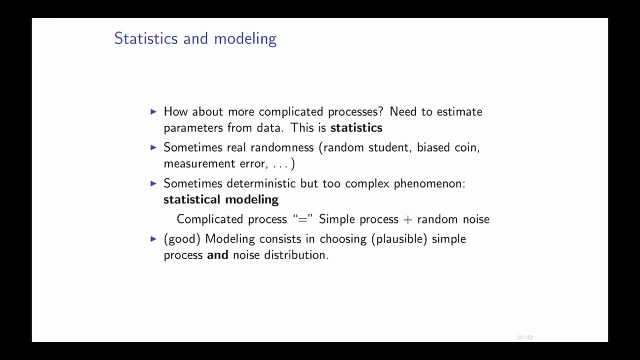 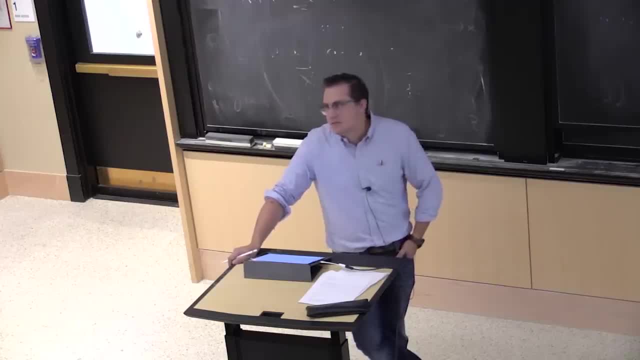 in AP Stats or something, But the need is to estimate parameters from data. All right, so for more complicated things, you might want to estimate some density parameter on a particular thing set of material, And for this maybe you need to beam something to it. 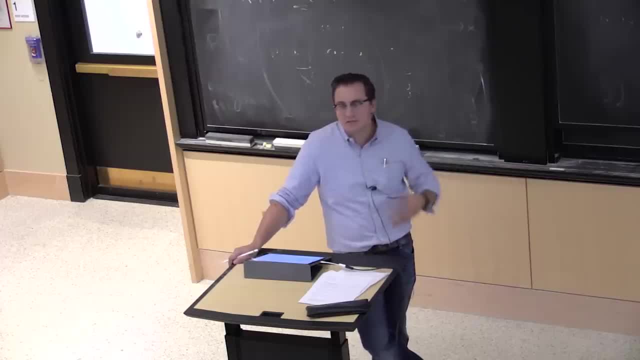 and measure how fast it's coming back And you're going to have some measurement errors And maybe you need to do that several times And you need to have a model for the physical process that's actually going on, And physics is usually a very good way. 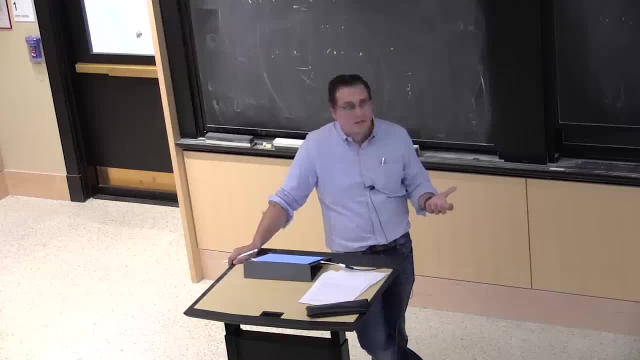 to get models for engineering perspective, But there's models for sociology where we have no physical system right. I mean, God knows how people interact And maybe I'm going to say that the way I make friends is by first flipping a coin in my pocket. 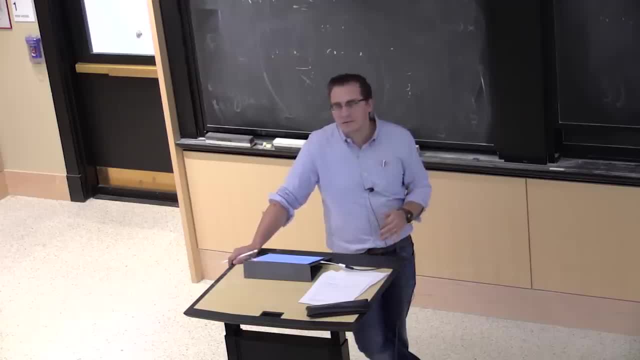 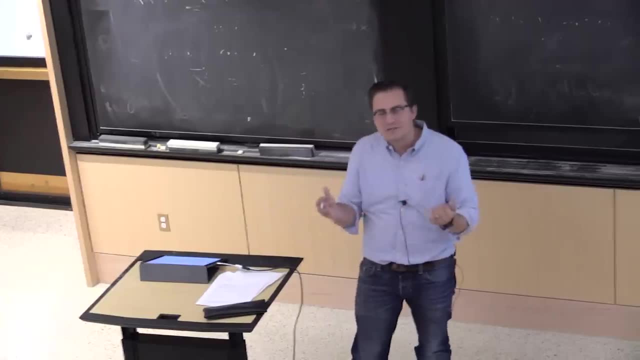 And with probably 2 thirds I'm going to make my friend at work And with probably 1 third I'm going to make my friend at soccer. And once I make my friend at soccer, I decide to make my friend at soccer. then I will face someone. 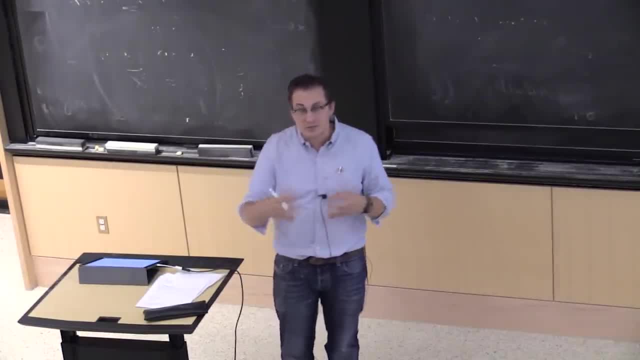 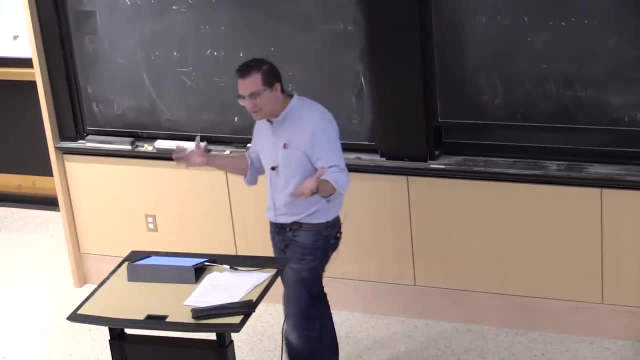 OK, So you have a friend who's flipping the same coin with maybe slightly different parameters, But those things actually exist. right? There's models about how friendships are formed, And this is the one I described. It's called the mixed membership model. 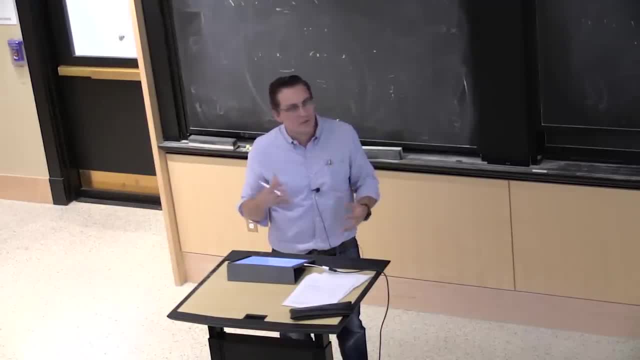 So those are models that are sort of hypothesized And they're more reasonable than there was taking into account all the things that made you meet that person at that particular time. OK, so the goal here? so based on data. now, once we have the model, it's going to be reduced to maybe. 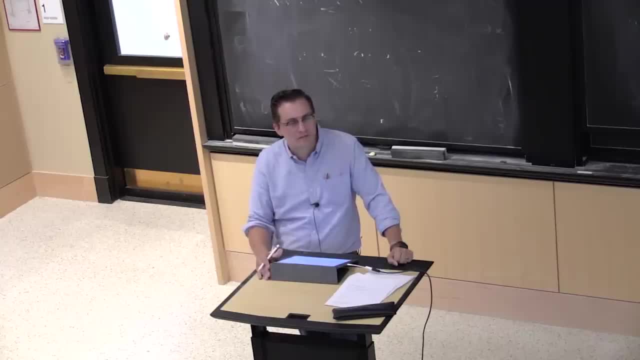 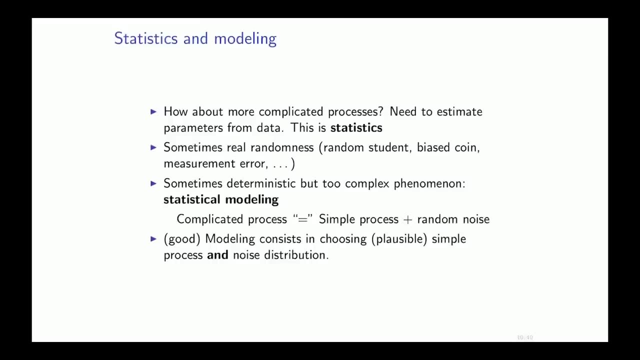 maybe two, three, four parameters, depending on how complex the model is, And then your goal will be to estimate those parameters. So sometimes the randomness that we have here is real right. So there's some true randomness in some surveys. If I pick a random student as long 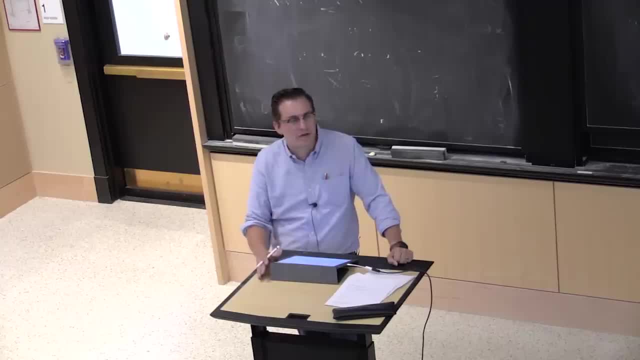 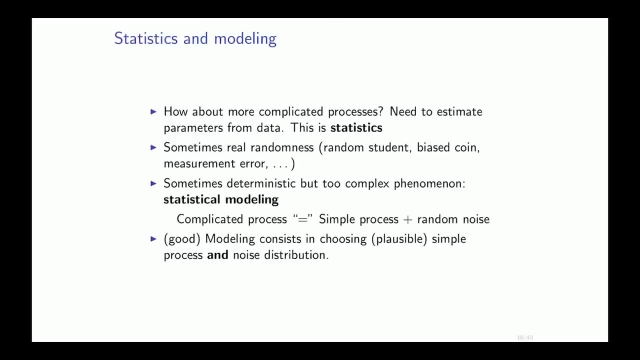 it's going to be reduced to maybe 2,, 3, 4 parameters, depending on how complex the model is, And then your goal will be to estimate, And then your goal will be to estimate those parameters. So sometimes the randomness that we have here is real right. 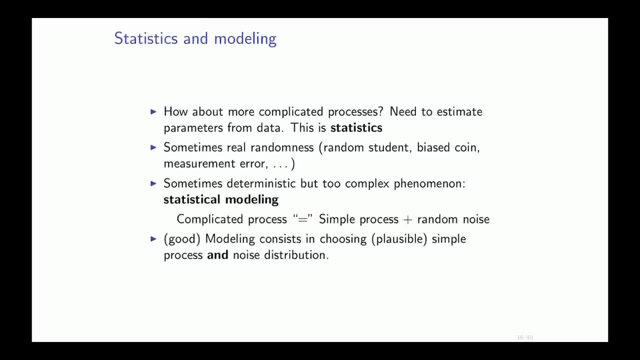 So there's some true randomness in some surveys. If I pick a random student, as long as I believe that my random number generator that will pick your random ID is actually random, there is something random about you, right, The student that I pick at random. 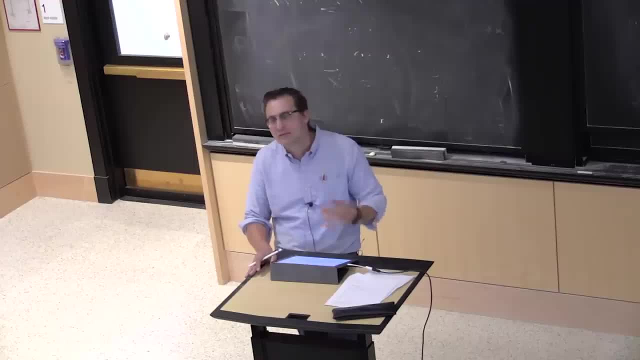 will be a random student. The person that I call on the phone is a random person, right? So there's some randomness that I can build into my system by drawing something from a random number generator. A biased coin is a random thing, right? 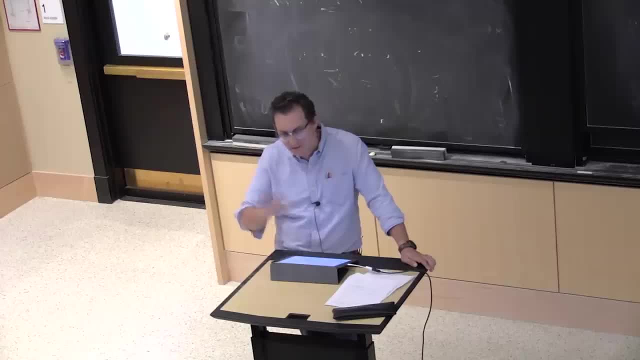 It's not a very interesting random thing. but it is a random thing again if I wash out the fact that it actually is a deterministic mechanism But a certain accuracy, a certain granularity. this can be thought of as a truly random experiment. 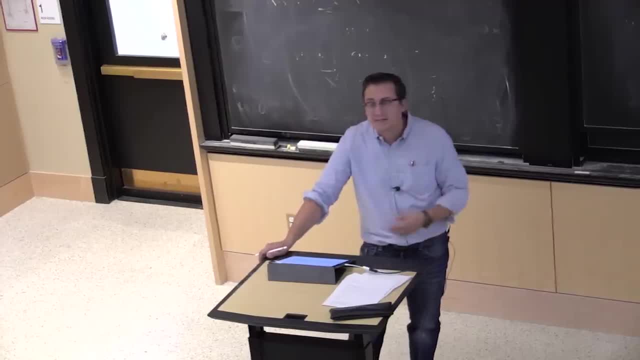 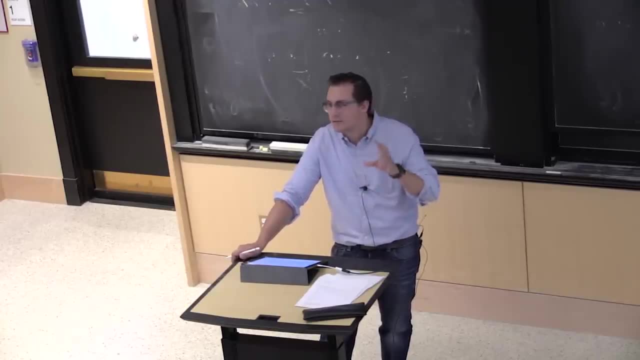 Measurement error. for example, if you buy some measurement device or some optics device, for example, you will have standard deviation and things that come on the side of the box And it tells you this will be making some measurement error And it's usually thermal noise maybe or things like this. 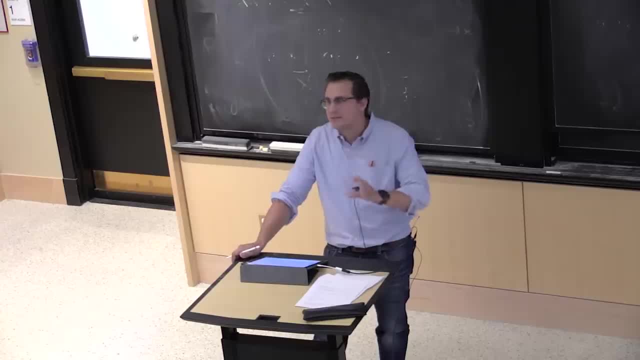 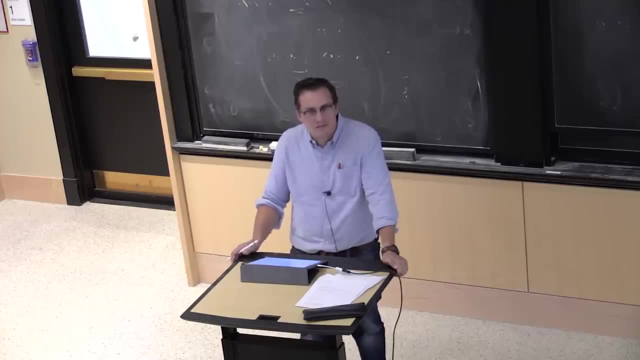 And those are very accurately described by some random phenomenon. But sometimes- I'd say most times- there's no randomness. There's no randomness. It's not like breaking your iPhone is a random event. This is just something that we sweep. Randomness is a big rug under which we sweep everything. 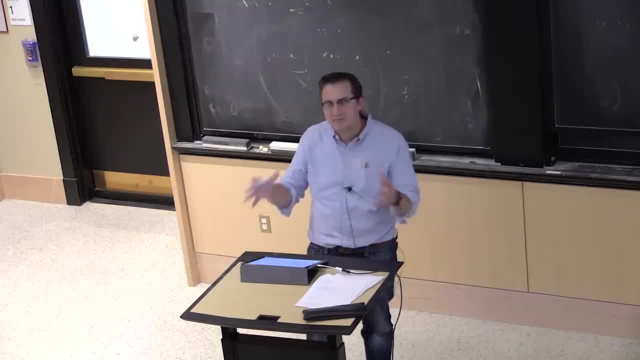 we don't understand And we just hope that, And in average, we've captured the average effect of what's going on And the rest it might fluctuate to the right, might fluctuate to the left, But what remains is just randomness. 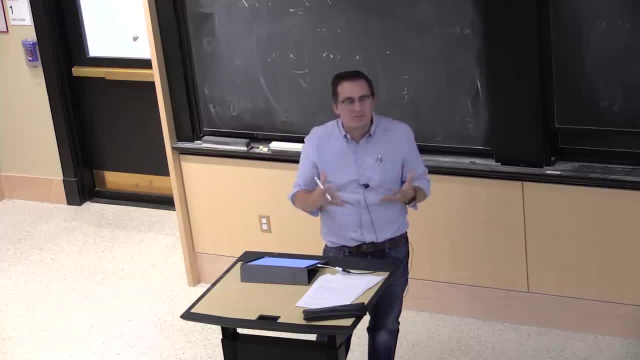 that can be averaged out. So, of course, this is where the leap of faith is. We do not have. we do not know whether we're correct of doing this. Maybe we make some huge systematic biases by doing this. Maybe we forget a very important component. 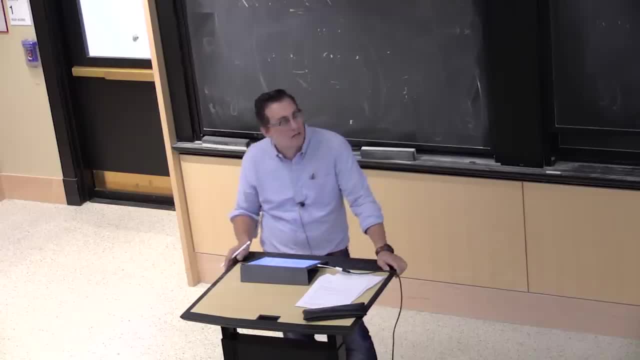 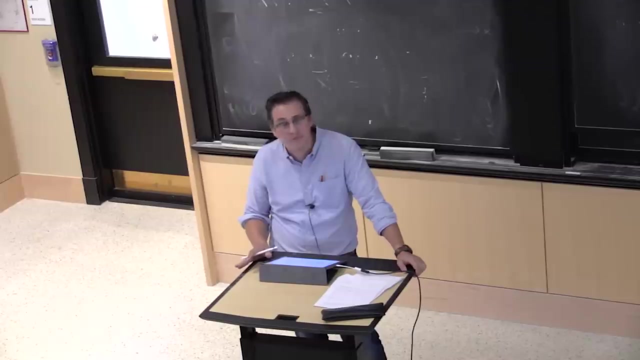 For example, if I have- I don't know, let's think of something- a drug for breast cancer, And I throw out the fact that my patient is either a man or a woman, I'm going to have some serious model biases. 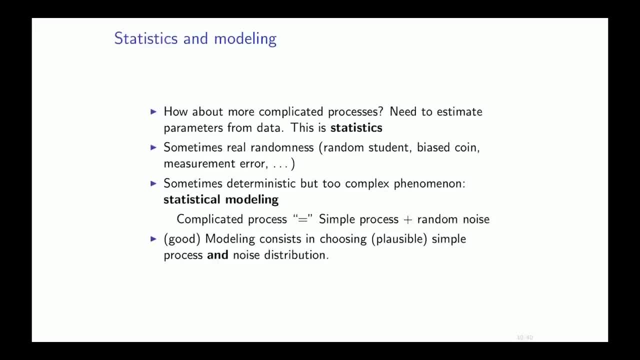 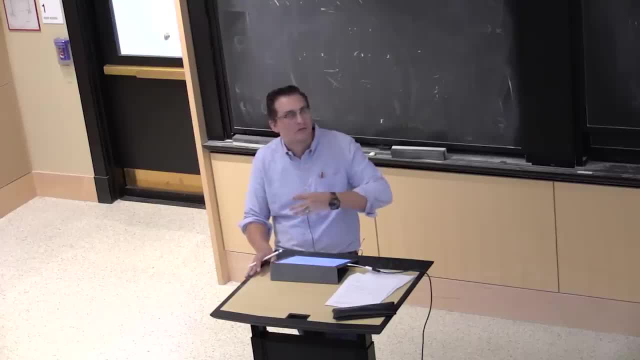 as I believe that my random number generator that will pick your random ID is actually random. there is something random about you, right? The student that I pick at random will be a random student. The person that I call On the phone is a random person, right? 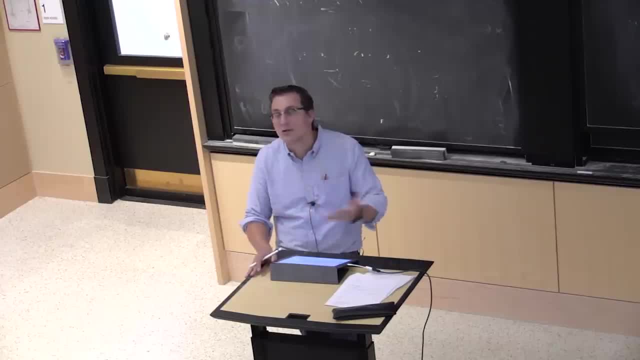 So there's some randomness that I can build into my system by drawing something from a random number generator. A biased coin is a random thing, right, It's not a very interesting random thing, but it is a random thing again if I. 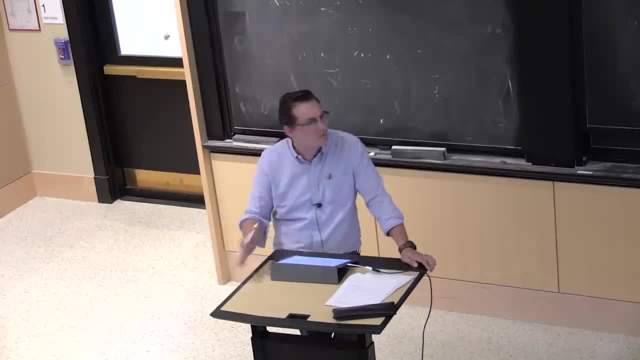 wash out the fact that it actually is a deterministic mechanism But a certain accuracy, a certain granularity. this can be thought of as a truly random experiment, Measurement error, for example. if you buy some measurement device or some Some optics device, for example, you 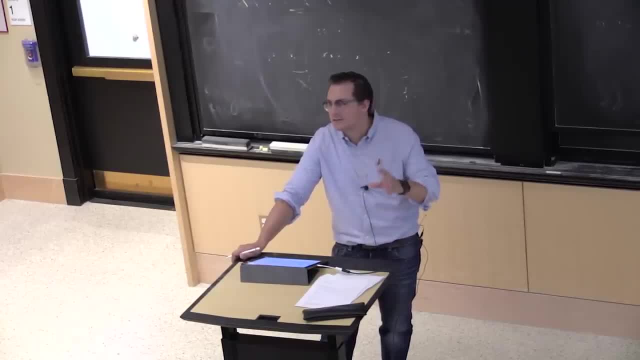 will have standard deviation and things that come on the side of the box And it tells you this will be making some measurement error, And it's usually thermal noise maybe, or things like this, And those are very accurately described by some random phenomenon. 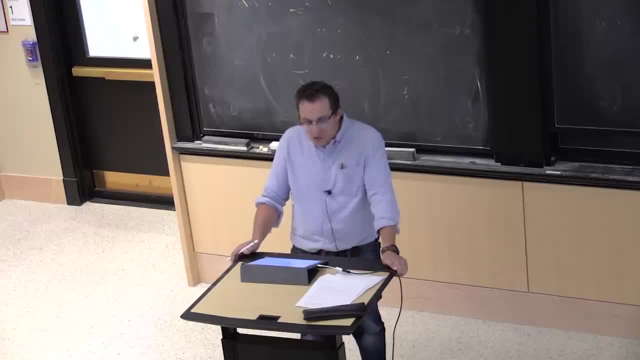 But sometimes- I'd say most times- there's no randomness. There's no randomness. It's not like you're breaking your iPhone is a random event. This is just something that we sweep. Randomness is a big rug under which we sweep everything. 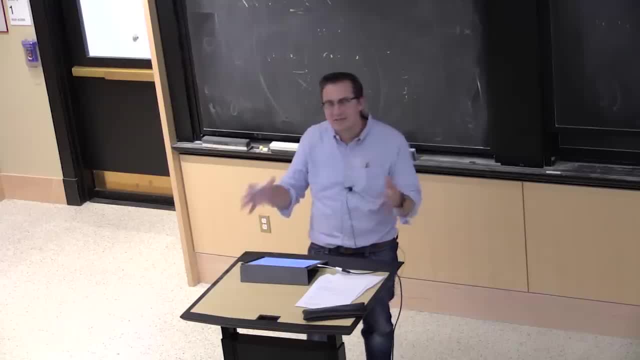 we don't understand And we just hope that in average we've captured sort of the average effect of what's going on And the rest it might fluctuate to the right, might fluctuate to the left, but that what remains is just sort of randomness that can be averaged out. 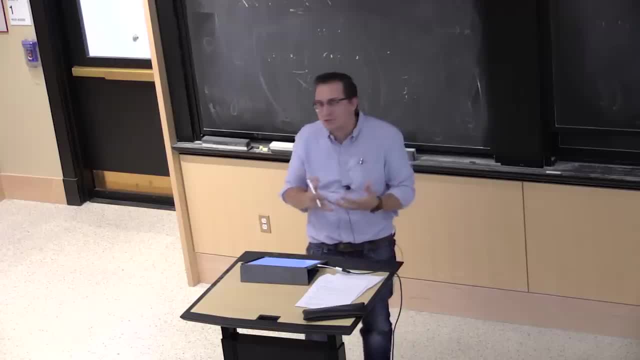 So, of course, this is where the leap of faith is. We do not have. we do not know whether we're correct of doing this. Maybe we make some huge systematic biases by doing this. Maybe we'll forget a very important component, right? 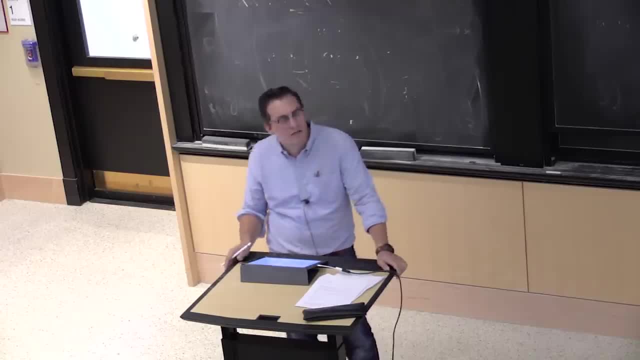 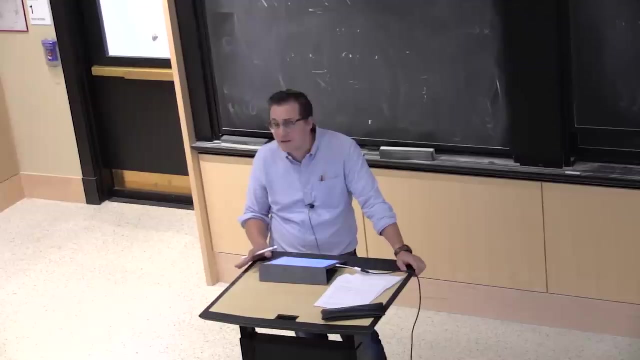 For example, if I have- I don't know, let's think of something- a drug for breast cancer, and I throw out the fact that my patient is either a man or a woman, I'm going to have some serious model biases. 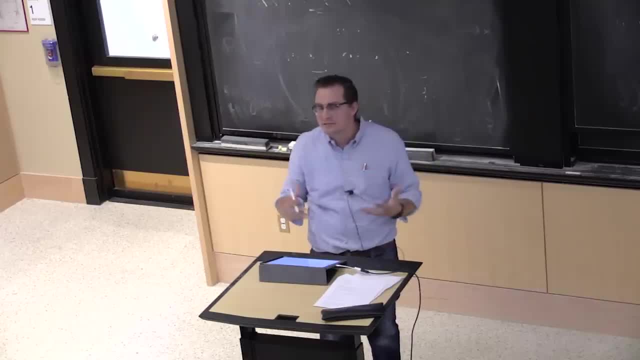 So if I say I'm going to collect some random patients and I'm going to start doing this, there's some information that I really need clearly to build into my model, And so a model should be complicated enough, but not too complicated, right? 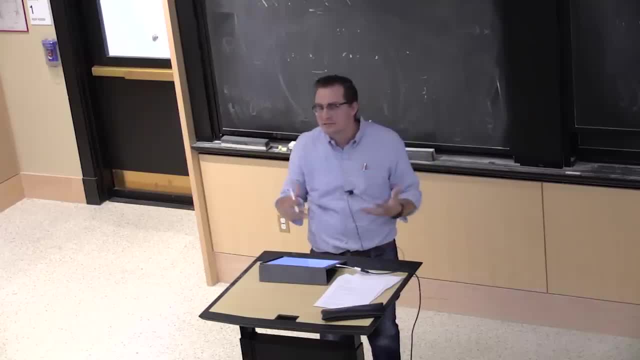 So if I say I'm going to collect some random patients and I'm going to start doing this, there's some information that I really need clearly to build into my model, And so a model should be complicated enough, but not too complicated. 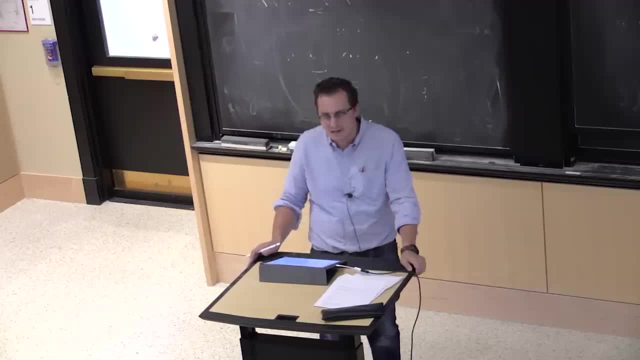 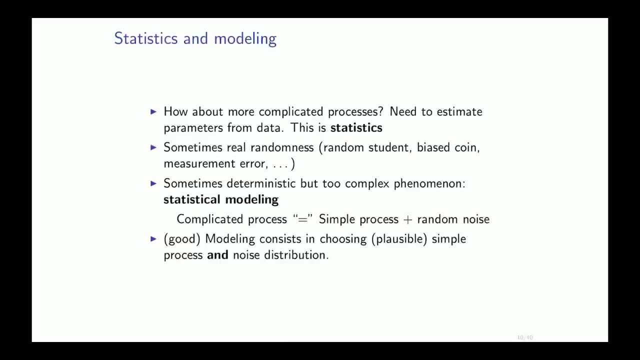 So it should take into account things that will systematically be important. So, in particular, the simple rule of thumb is: when you have a complicated process, you can think of it as being a simple process, and some random noise. Now, again, the random noise is everything. 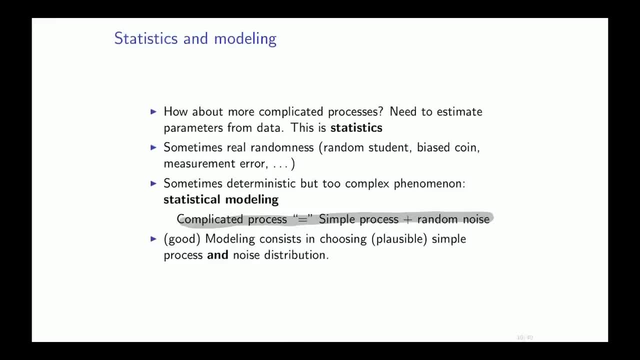 you don't understand about the complicated process, And the simple process is everything you actually do. So good modeling- and this is not what we'll be seeing in this class- consists in choosing plausible, simple models, And this requires a tremendous amount of domain knowledge. 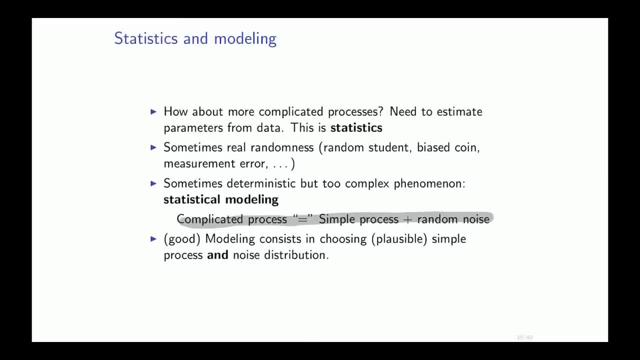 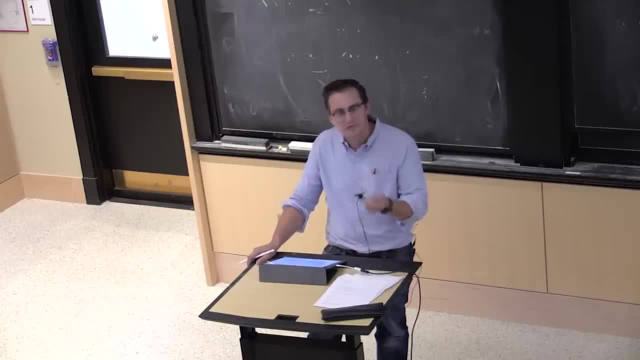 And that's why we're not doing it in this class. This is not something where I can make a blanket statement about making good modeling. You need to know, If I were a statistician working on a study, I would have to grill the person in front of me, the expert. 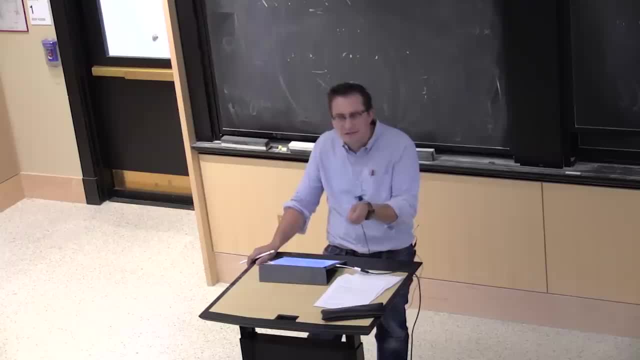 for two hours to know: oh, but how about this, How about that, How about? how does this work? So it requires to understand a lot of things. There's this famous statistician to whom this sentence, this sentence, is attributed, and it's probably not his, then. 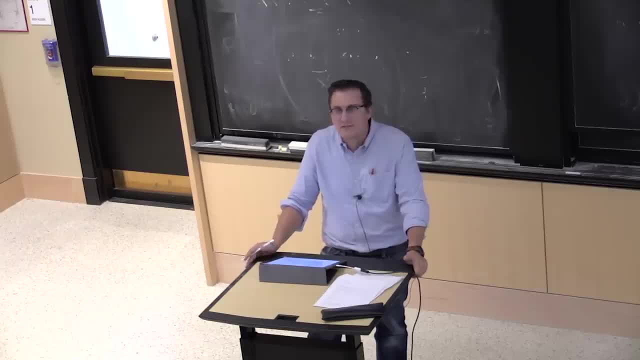 But Tukey said that he loves being a statistician because you get to play in everybody's backyard. So you get to go and see people and you get to understand, at least to a certain extent, what their problems are, enough that you can actually 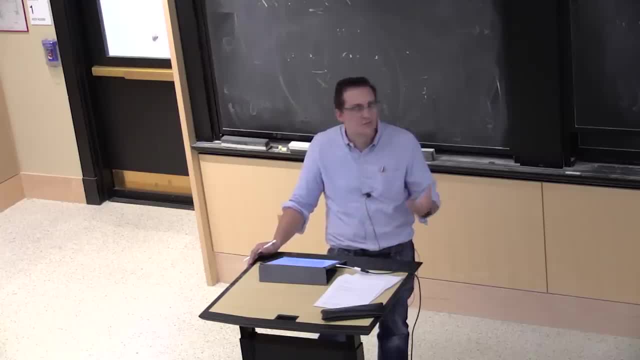 build a reasonable model for what they're actually doing. So you get to do some sociology, get to do some biology, get to do some engineering and you get to do a lot of different things. So he was actually at some point predicting the political 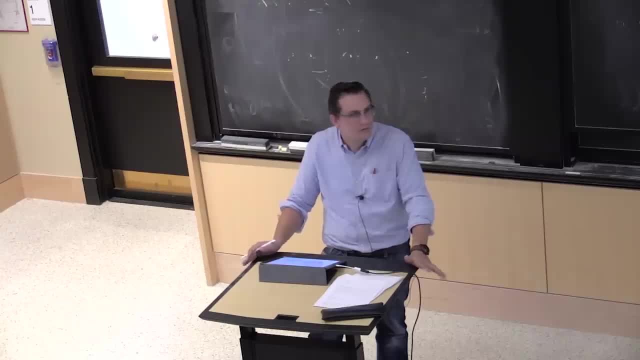 the presidential election. So you see, you get to do a lot of different things, but it requires a lot of time to understand what problem you're working on And if you have a particular application in mind. you're the best person to actually understand this. 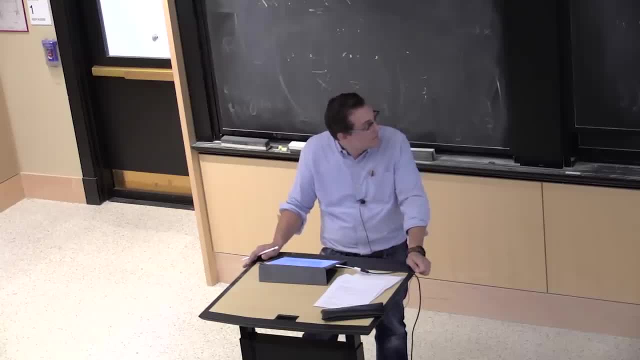 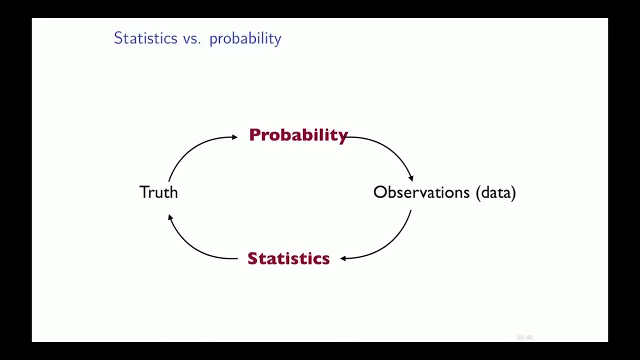 So I'm just going to give you the basic tools. OK, so this is the circle of trust. No, this is really just the simple, simple graphic that tells you what's going on. When you do probability, you're given the truth. 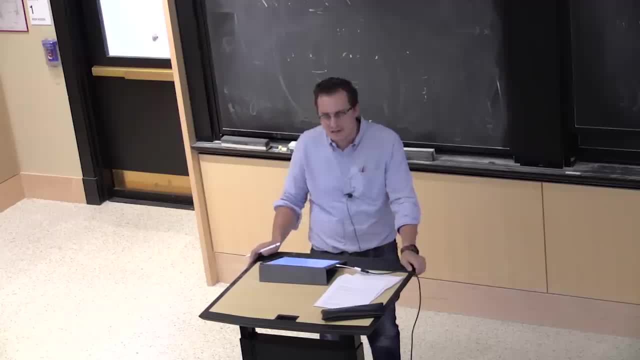 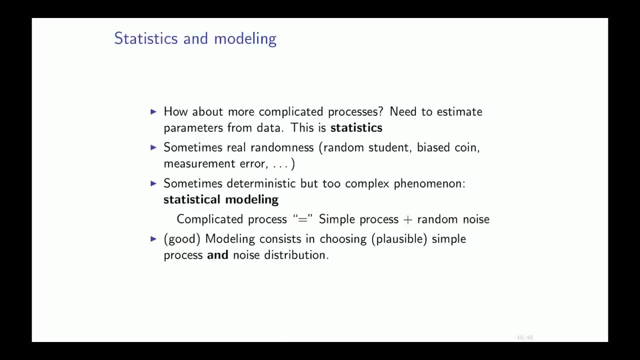 So it should take into account things that will systematically be important. OK, so, in particular, the simple rule of thumb is: when you have a complicated process, you can think of it as being a simple process, and some random noise. Now, again, the random noise is everything. 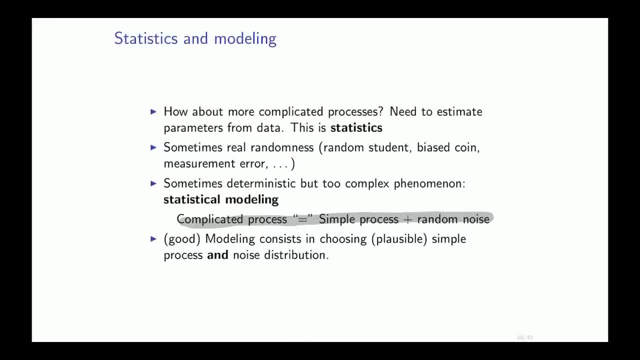 you don't understand about the complicated process, and the simple process is everything you actually do, OK. So Good modeling- and this is not what we'll be seeing in this class- consists in choosing plausible, simple models, And this requires a tremendous amount of domain knowledge. 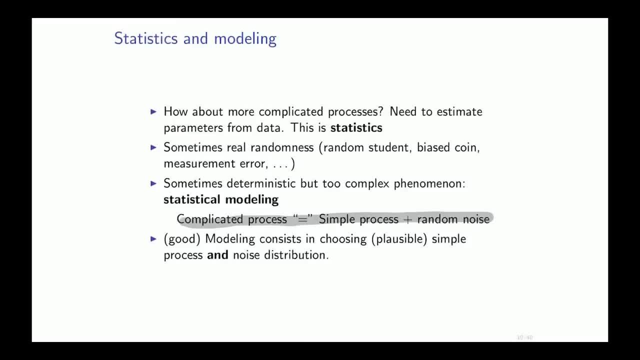 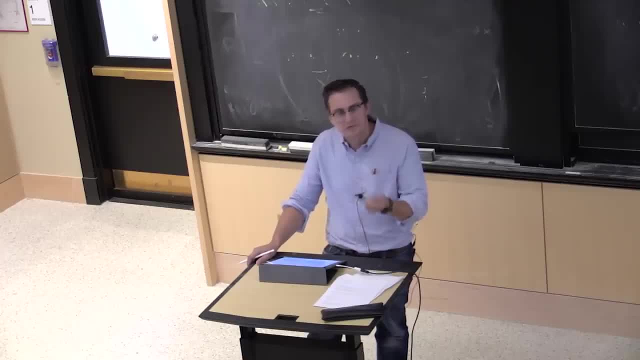 And that's why we're not doing it in this class. This is not something where I can make a blanket statement about making good modeling. You need to know, If I were a statistician working on a study, I would have to grill the person in front of me, the expert. 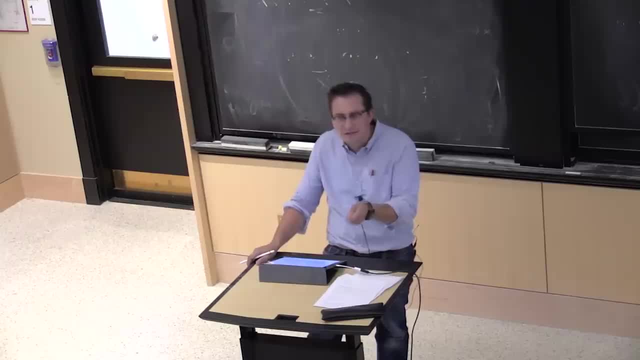 for two hours to know: oh, but how about this, How about that, How about? how does this work? So it requires to understand a lot of things. There's this famous statistician to whom this sentence is attributed, and it's probably not his- then. 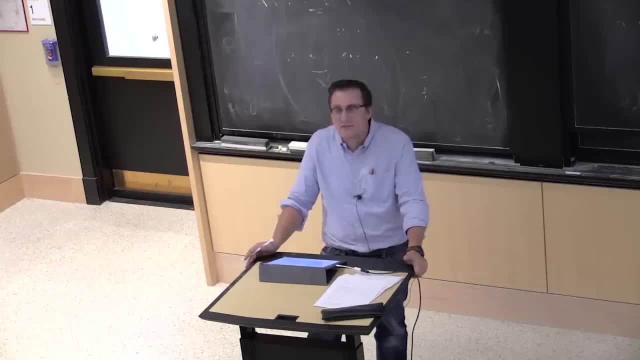 But Tukey said that he loves being a statistician because you get to play in everybody's backyard. So you get to go and see people and you get to understand, at least to a certain extent, what their problems are, enough that you can actually 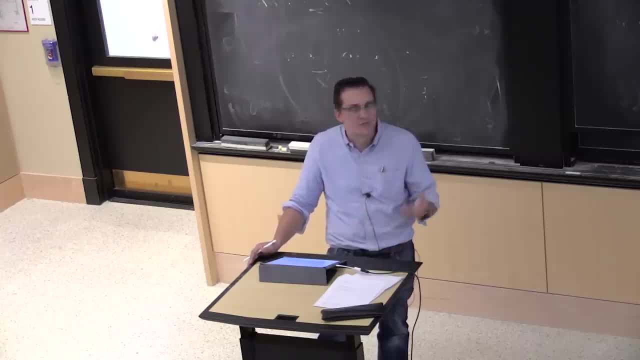 build a reasonable model for what they're actually doing. So you get to do some sociology, You get to do some biology, You get to do some engineering And you get to do a lot of different things. So he was actually at some point. 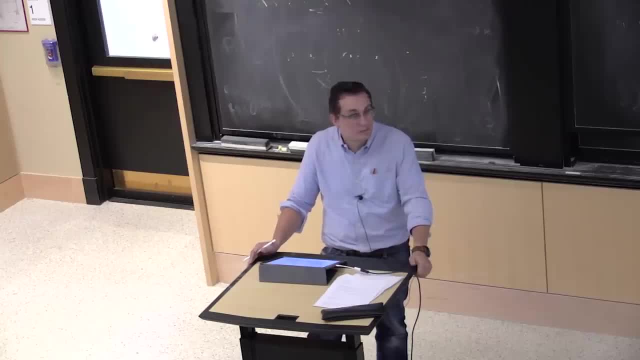 predicting the political, the presidential election. So you see, you get to do a lot of different things, but it requires a lot of time to understand what problem you're working on And if you have a particular application in mind. you're the best person to actually understand this. 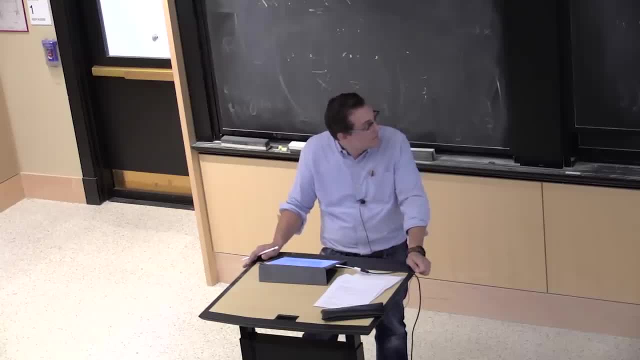 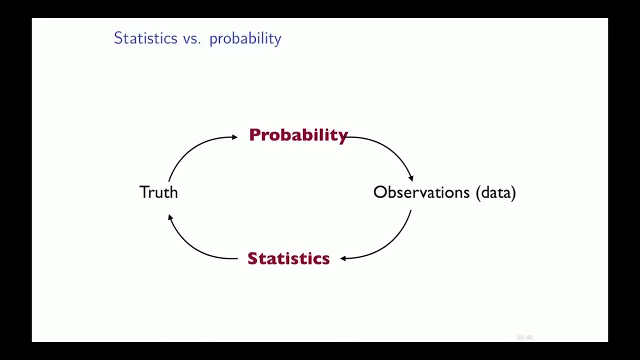 So I'm just going to give you the basic tools. OK, so this is the- Yeah, you know the circle of trust. No, this is really just a simple graphic that tells you what's going on. When you do probability, you're given the truth. 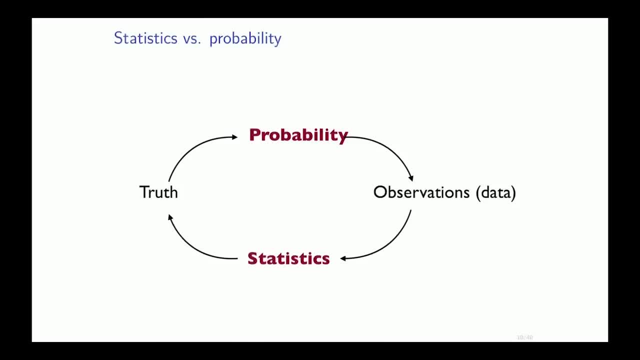 Somebody tells you: what die, God is rolling all right. So you know exactly what the parameters of the problems are, And what you're trying to do is to describe what the outcomes are going to be. OK, You can say: well, there's, you know. 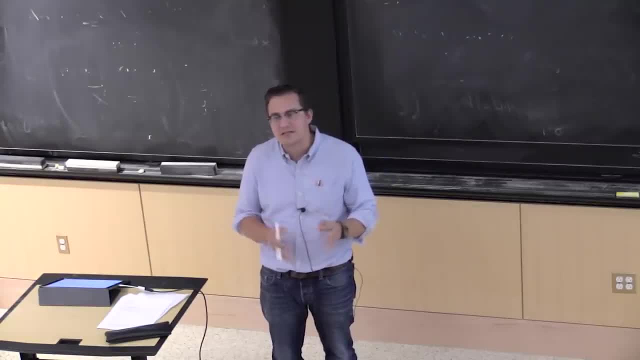 if you're rolling a fair die, you're going to have one-sixth of the time in your data you're going to have one. One-sixth of the time you're going to have one. Yeah Yeah, You're going to have two. 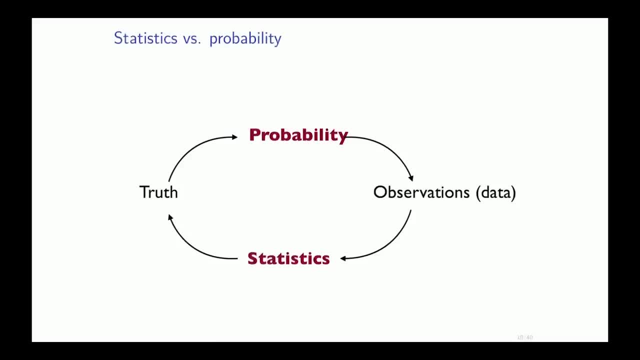 And so you can describe. If I told you what the truth is, you could actually go into a computer either generate some data, or you could describe to me some more macro properties of what the data would be like. Oh, I would see a bunch of numbers. 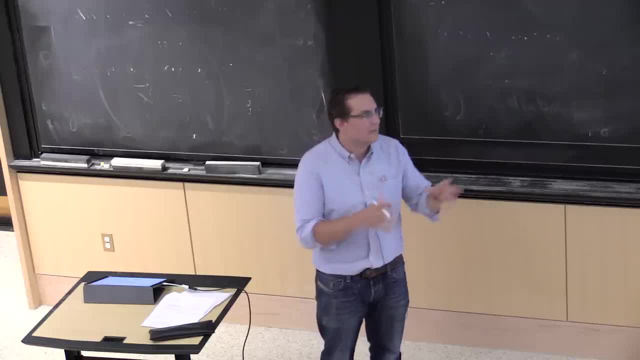 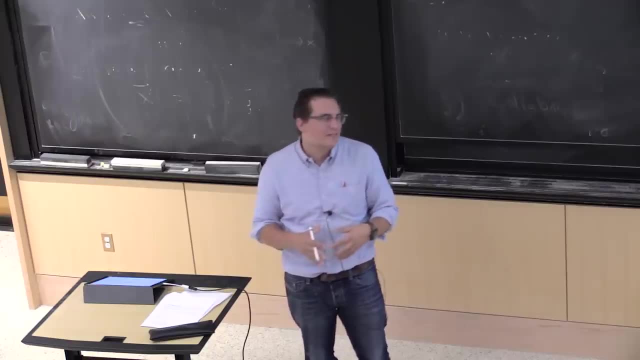 that would be centered around 35 if I drew from a Gaussian distribution centered at 35, right, You would know this kind of thing. I would know that it's very unlikely that if my Gaussian has standard deviation It's centered 0 and 0, say with standard deviation 3,. 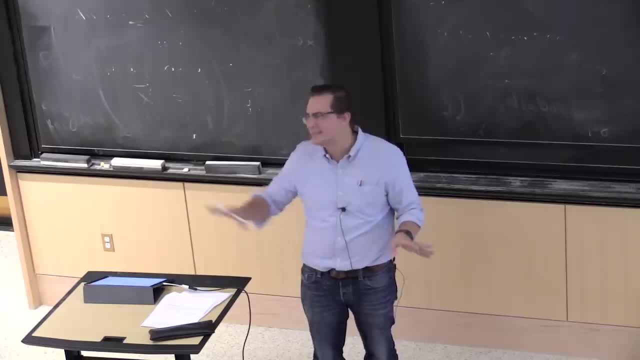 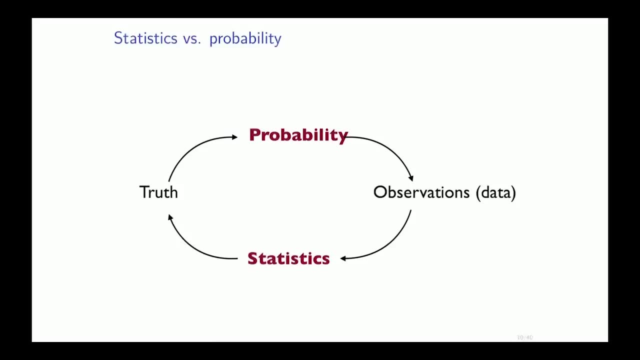 it's very unlikely that I will see numbers below minus 10 and above 10, right, You know this, that you basically will not see them. So you know from the truth, from the distribution of a random variable that does not have mu or sigma. 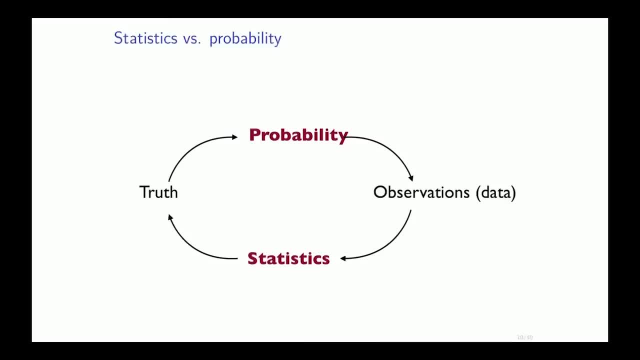 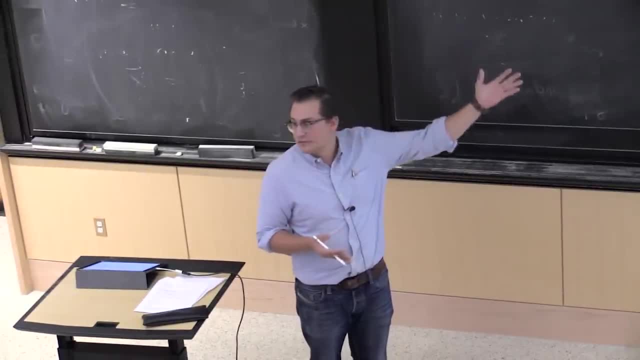 it's really numbers there. You know that you're going to be, what data you're going to be having. Statistics is about going backwards. It's saying, if I have some data, what was the truth that generated it? And since there's so many possible truths, 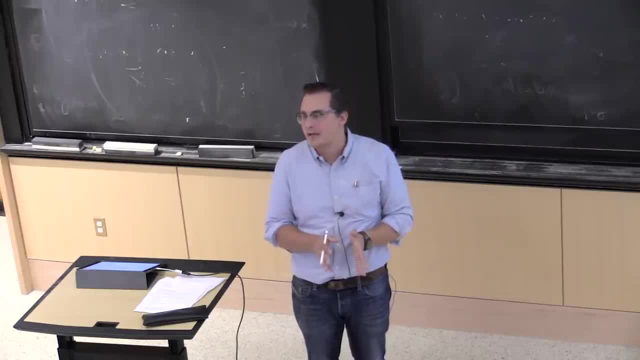 modeling says you have to pick one of those simpler possible truths so that you can average out Statistics. basically means averaging. You're averaging when you do statistics And averaging means that if I say that I receive the, so if I collect all your GPAs, for example in my model, 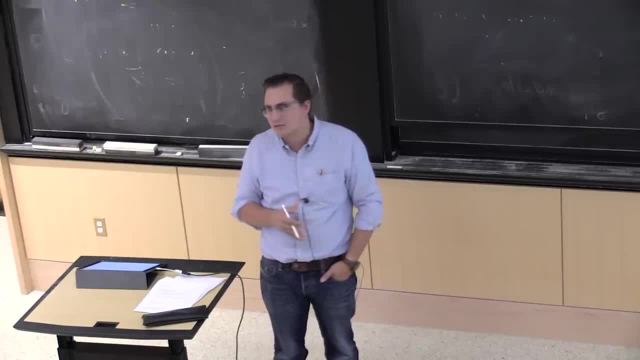 is that, well, the possible GPAs or any possible numbers, and anybody can have any possible GPA. this is going to be a serious problem. But if I can summarize those GPAs into two numbers, right, Two numbers say mean and standard deviation. 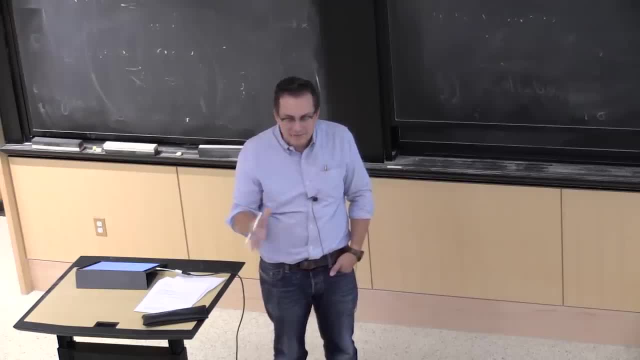 then I have a pretty good description of what is going on, rather than having to have to predict a full list. right, If I learn a full list of GPAs and I say, well, this was the distribution, then it's not going to be of any use for me to predict what the next GPA would. 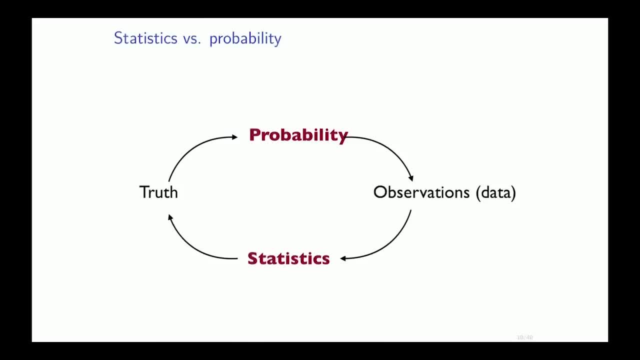 Somebody tells you what die God is rolling. So you know exactly what the parameters of the problems are, And what you're trying to do is to describe what the outcomes are going to be. You can say: well, if you're rolling a fair die, 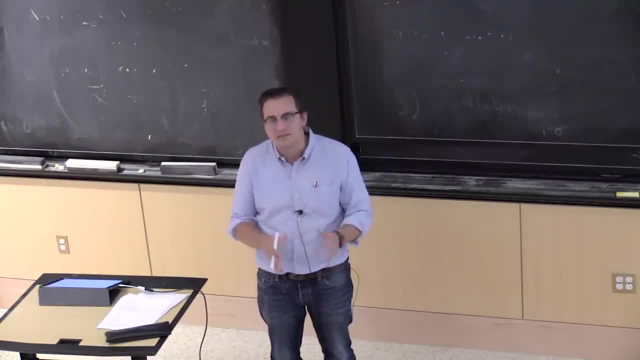 you're going to have one-sixth of the time in your data. you're going to have one, One-sixth of the time you're going to have two, And so you can describe if I told you what the truth is. 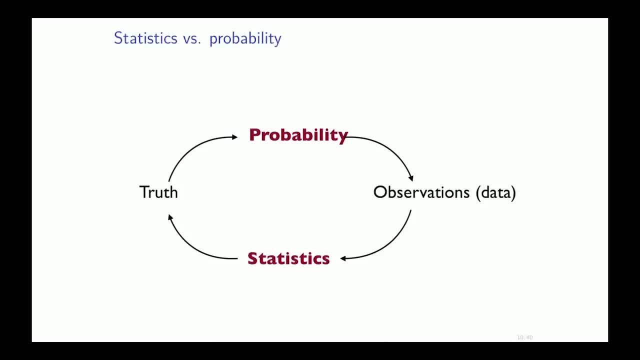 you could actually go into it. You could go into a computer, either generate some data or you could describe to me some more macro properties of what the data would be like. Oh, I would see a bunch of numbers that would be centered around 35 if I 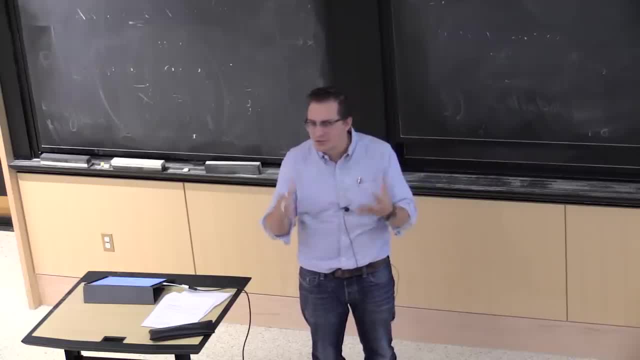 drew from a Gaussian distribution centered at 35. You would know this kind of thing. I would know that it's very unlikely that if my Gaussian has standard deviation is centered 0 and 0, say with standard deviation 3. It's very unlikely that I will see numbers below minus 10. 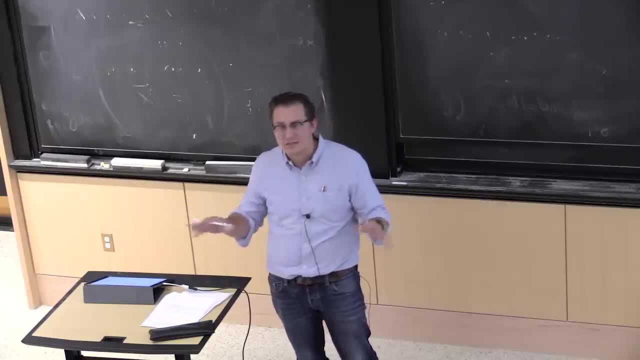 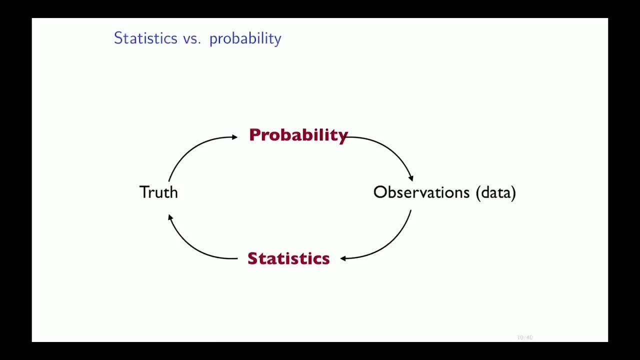 and above 10.. You know this, that you basically will not see them. So you know, from the truth, from the distribution of a random variable that does not have mu or sigma, it's really numbers. there You know what data you're going to be having. 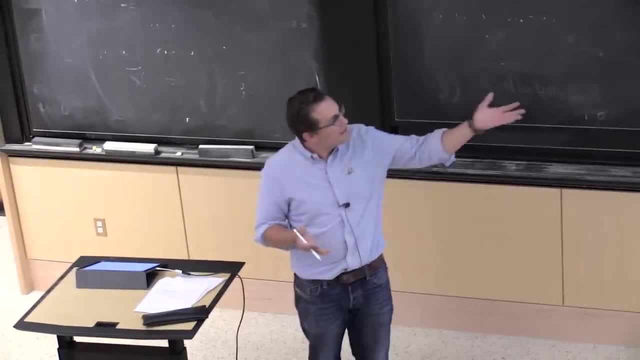 Statistics is about going backwards. It's saying: if I have some data, what was the truth that generated it? And since there's so many possible truths, modeling says you have to pick one of those simpler possible truths so that you can average out. 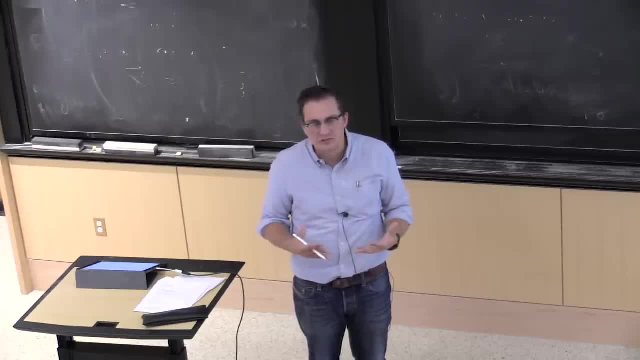 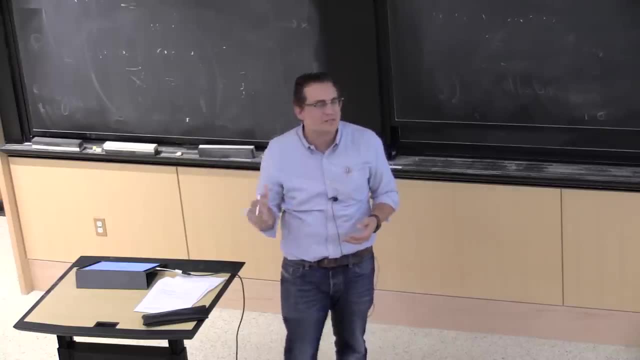 Statistics basically means averaging. You're averaging when you do statistics And averaging means that if I say that I receive the, so if I collect all your GPAs, for example in my model, is that well the possible GPAs or any possible numbers? 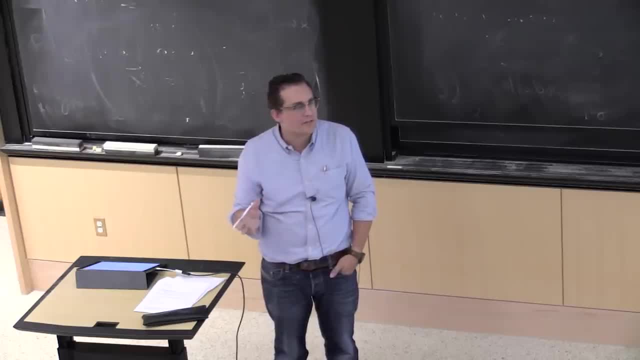 and anybody can have any possible GPA. this is going to be a serious problem, But if I can summarize those GPAs into two numbers, say mean and standard deviation, then I have a pretty good description of what is going on, rather than having to have 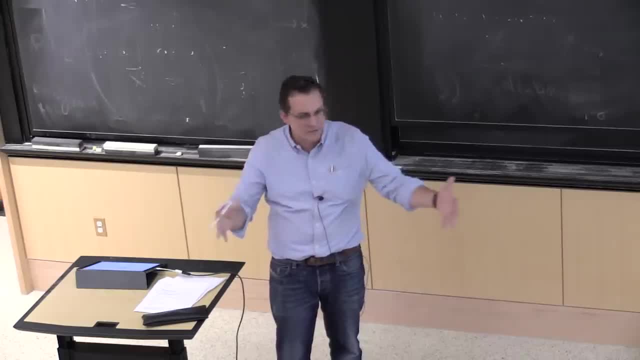 to predict a full list. If I learn a full list of GPAs and I say, well, this was the distribution, then it's not going to be of any use for me to predict what the next GPA would be. or some random student walking in. 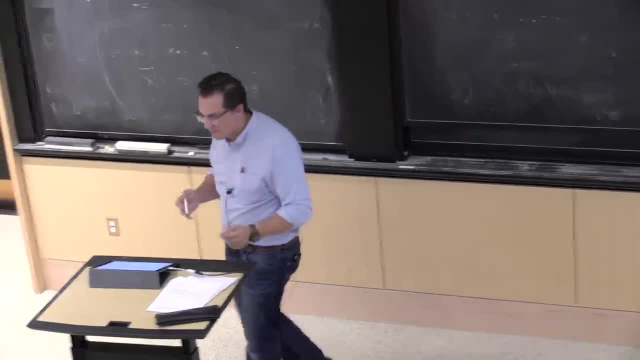 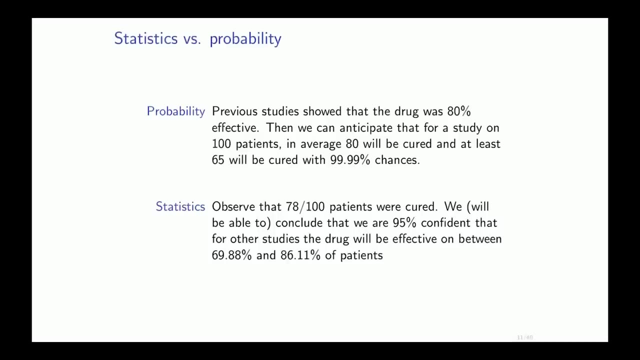 be, or some random student walking in or something like this. OK, so just to finish my rant about probability versus statistics, this is a question you would see on. this is a probabilistic question and this is a statistical question. The probabilistic question is previous study. 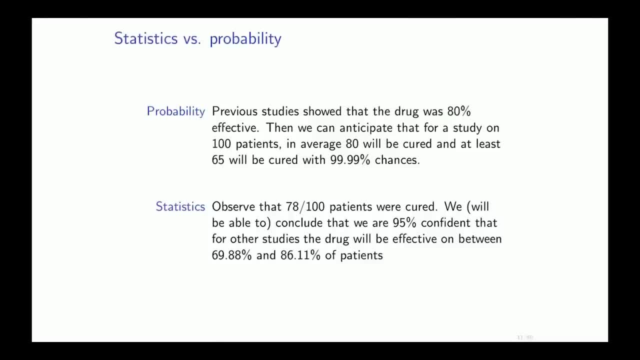 showed that the drug was 80% effective. So you know that This is the effectiveness of the drug It's given to you. This is how your problem starts. Then we can anticipate that for a study on 100 patients, in average 80 will be cured and at least 65. 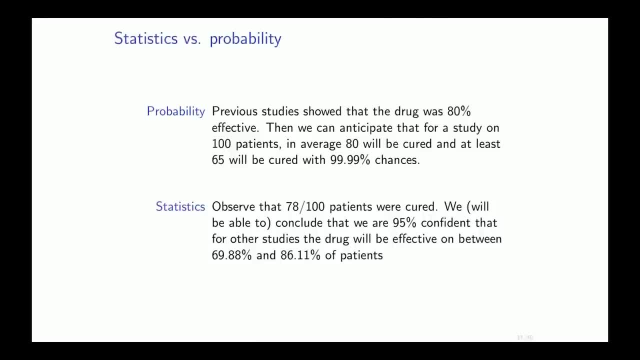 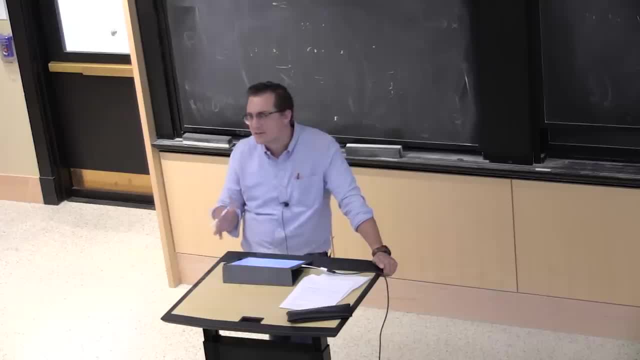 will be cured with 99% chances. So again, this are not. I'm not predicting on 100 patients, exactly the number of them that are going to be cured and the number of them that are not, But I'm actually sort of predicting. 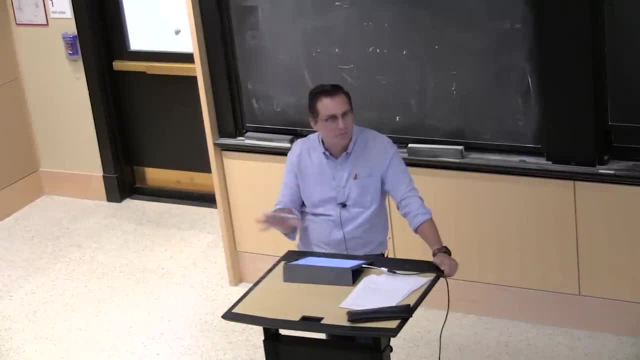 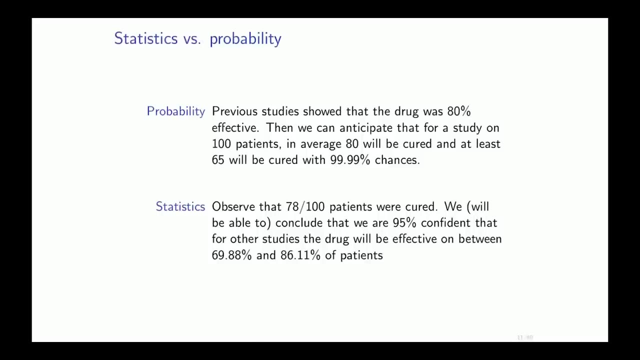 what things are going to look like in average or some macro properties of what my data sets will look like. So with 99% chances, that means that in 99.99% of the data sets you will draw from this particular drug 99.99% of the cohort of 100 patients. 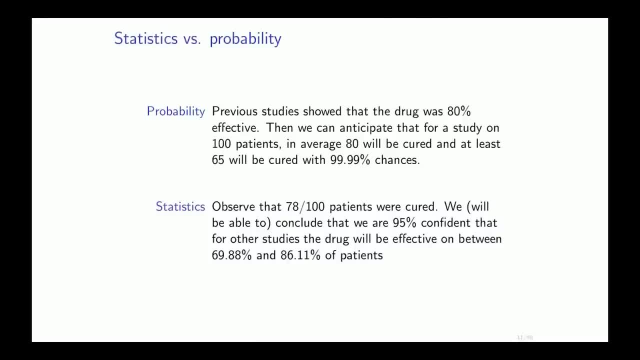 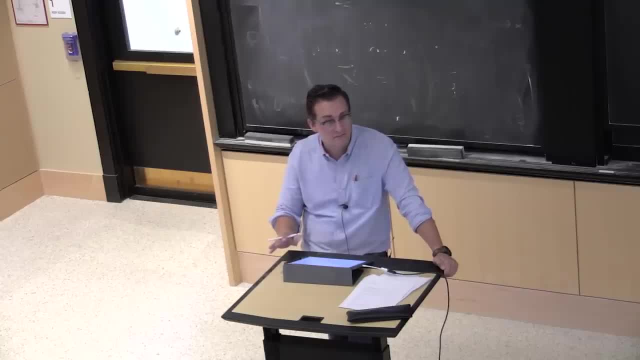 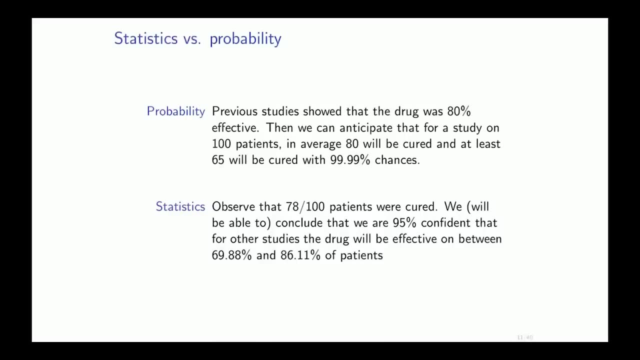 to whom you administer this drug, I will be able to conclude that at least 65 of them will be cured on 99.99% OK. So that's a pretty accurate prediction of what's going to happen. Statistics is the opposite. It says: well, I just know that 78 out of 100 were cured. 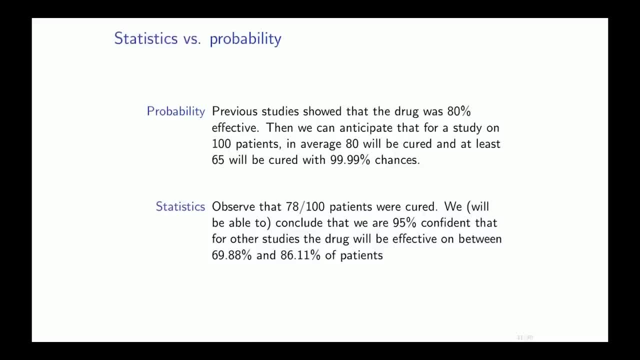 I have only one data set. I cannot make predictions for all data sets. But I can go back to the probability, make some inference about what my probability will look like and then say: OK, then I can make those predictions later on. 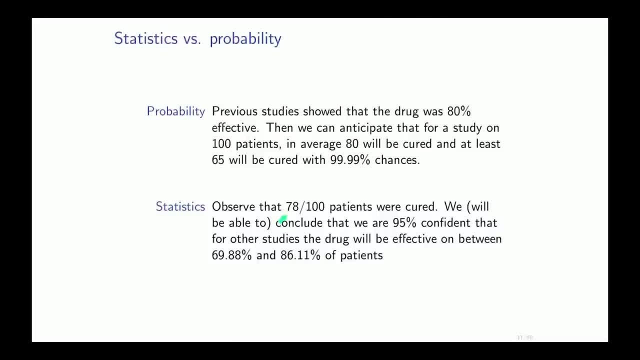 So when I start with 78 over 100, then maybe I can make predictions for 100. Then maybe I'm actually in this case. I just don't know. My best guess here is that I'm confident. I have to add the extra error that I may be making by predicting. 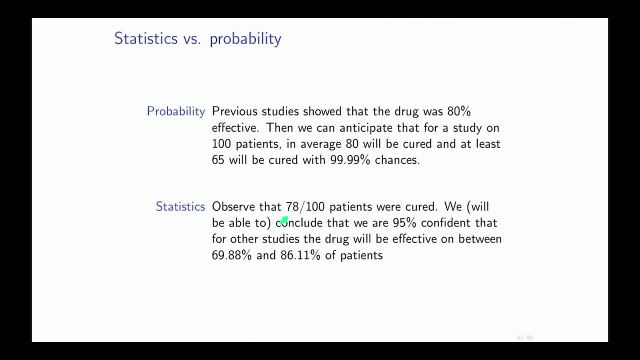 that here the drug is not 80% effective but 78% effective, And I need some error bars around this that will hopefully contain 80%, And then, based on those error bars, I'm going to make slightly less precise predictions for the future. 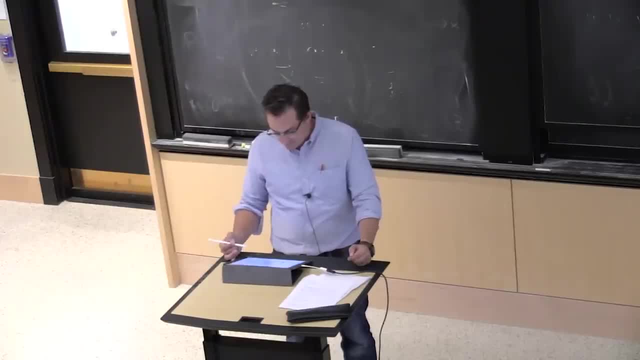 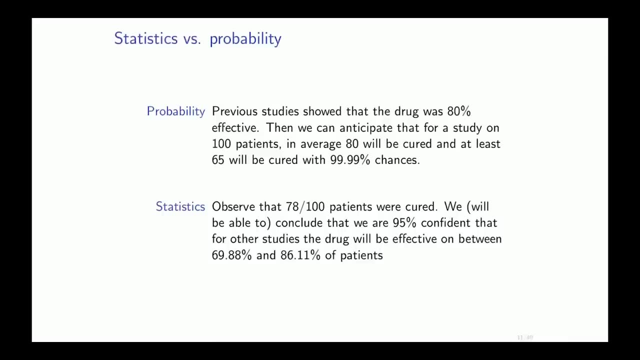 or something like this. So just to finish my rant about probability versus statistics, this is a question you would see in a probabilistic question and this is a statistical question. The probabilistic question is: previous studies showed that the drug was 80% effective. 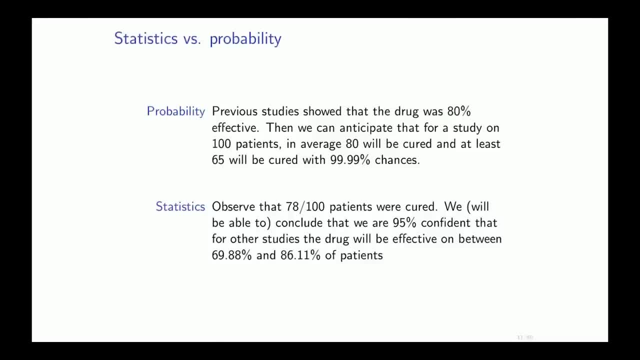 So you know that This is the effectiveness of the drug It's given to you. This is how your problem starts. Then we can anticipate that for a study on 100 patients, in average 80 will be cured and at least 65. 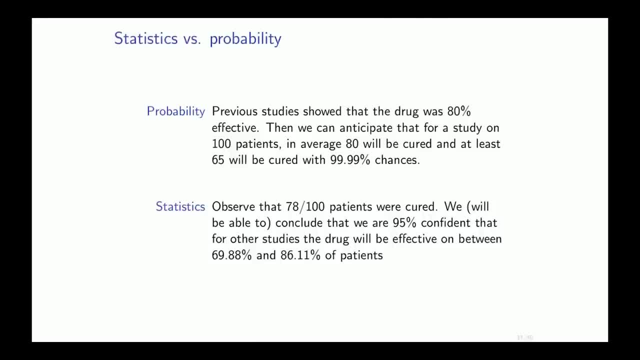 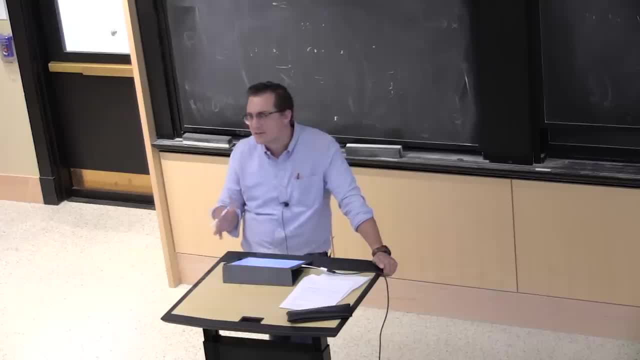 will be cured with 99% chances. So again, I'm not predicting on 100 patients exactly the number of them that are going to be cured and the number of them that are not, but I'm actually sort of predicting what things are going. 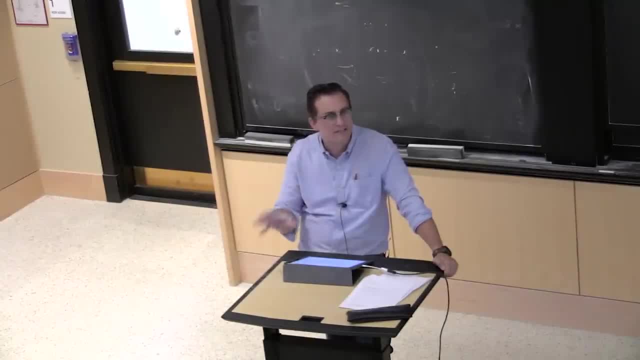 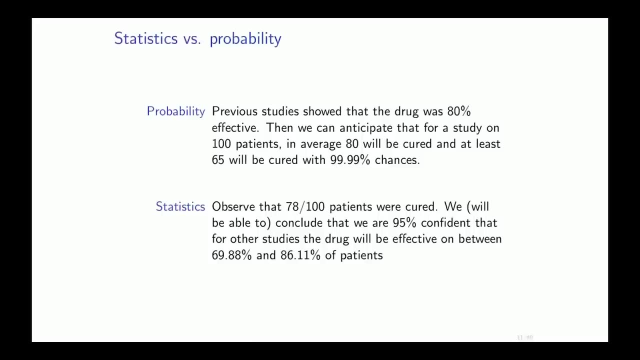 to look like. I'm predicting the average or some macro properties of what my data sets will look like. So with 99% chances, that means that in 99.99% of the data sets you will draw from this particular drug 99.99% of the cohort of 100 patients. 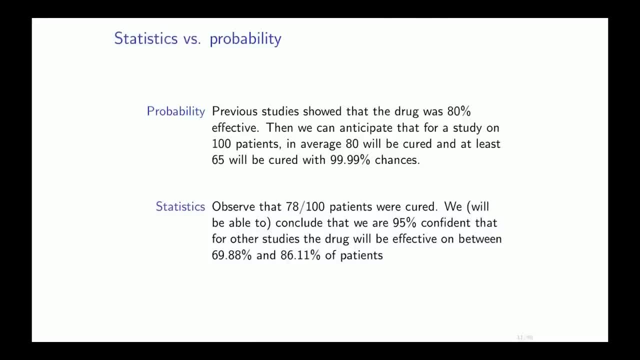 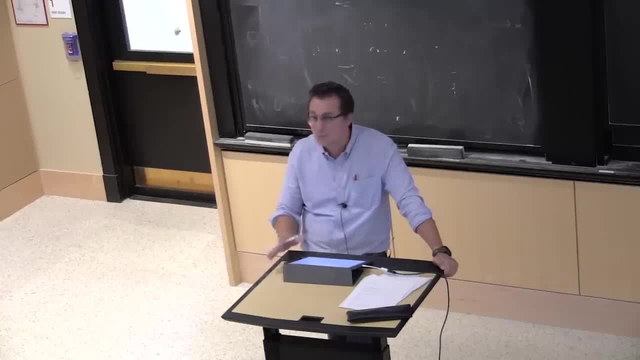 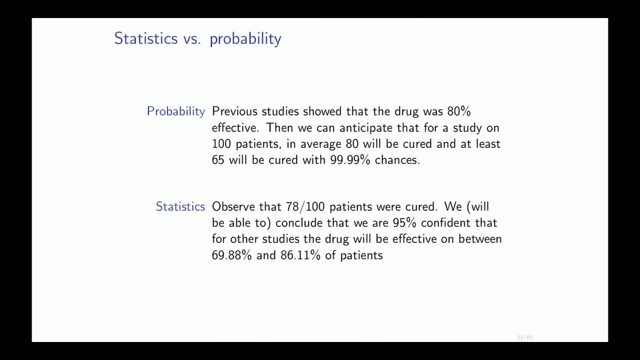 to whom you administer this drug, I will be able to conclude that at least 65 of them will be cured. on 99.99% of those data sets, That's my prediction of what's going to happen. Statistics is the opposite. It says: well, I just know that 78 out of 100 were cured. 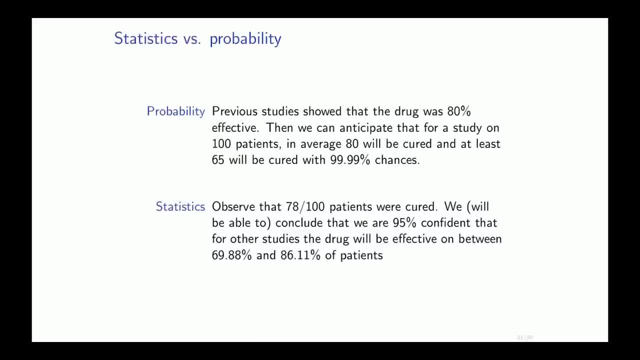 I have only one data set. I cannot make predictions for all data sets, but I can go back to the probability, make some inference about what my probability will look like and then say: OK, then I can make those predictions later on. 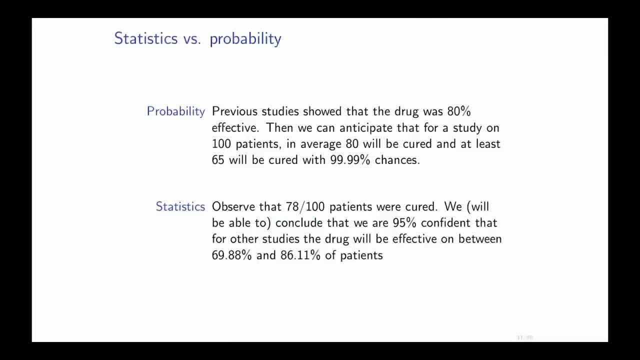 So when I start with 78 over 100, then maybe I'm actually in this case. I just don't know. My best guess here Is that I'm confident. I have to add the extra error that I may be making by predicting that here the drug is not. 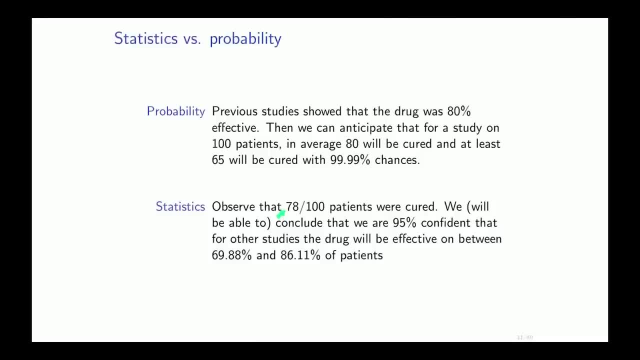 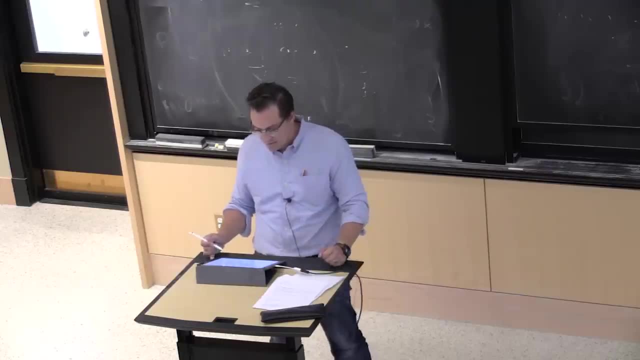 80% effective but 78% effective, And I need some error bars around this that will hopefully contain 80%, And then, based on those error bars, I'm going to make slightly less precise predictions for the future. OK, so to conclude, 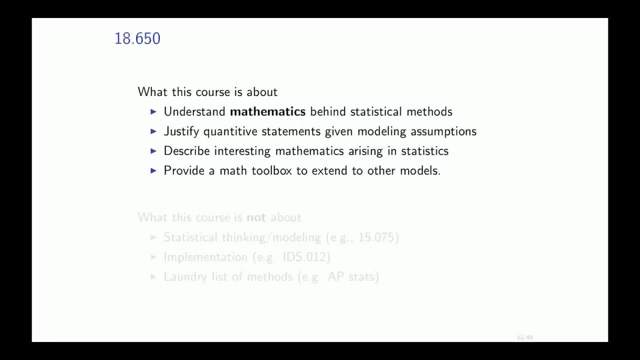 OK. So to conclude, so this was why statistics. So what is this course about? It's about understanding the mathematics behind statistical methods. It's more of a tool. We're not going to have fun and talk about algebraic geometry just for fun in the middle of it. 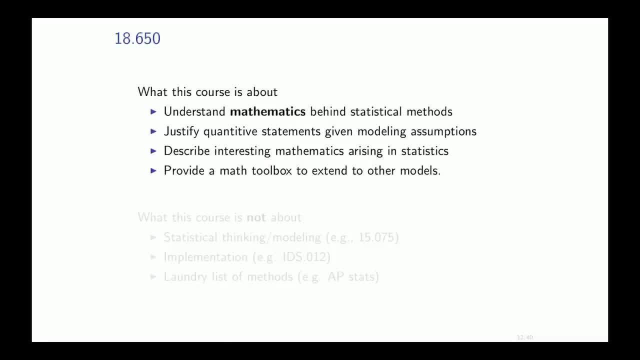 So justify quantitative statements given some modeling assumptions. So we will, in this class, mostly admit that the modeling assumptions are correct in the first part In this introduction. we will go through them, because it's very easy to forget what assumptions you're. 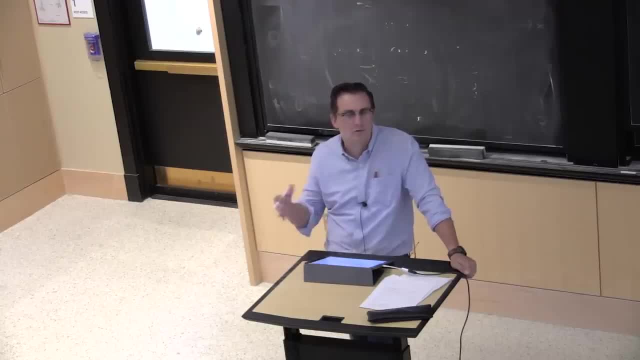 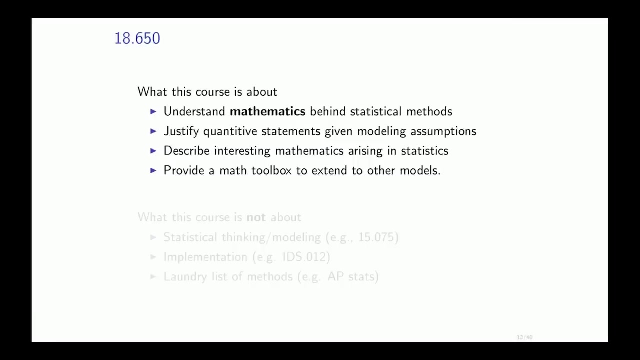 actually making, But this will be a pretty standard thing. The words you will hear a lot are IID, Independent and Identically Distributed. That means that your data is basically all the same And one data point is not impacting another data point. Hopefully, we can describe some interesting mathematics arising. 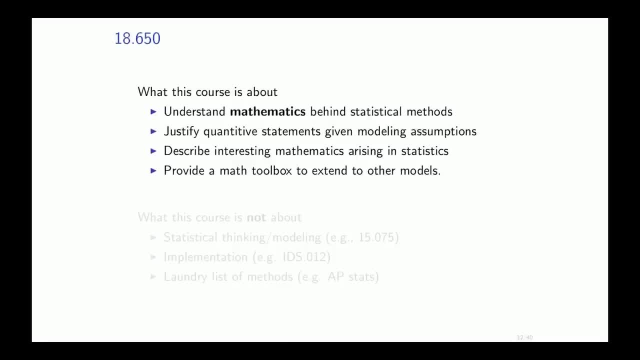 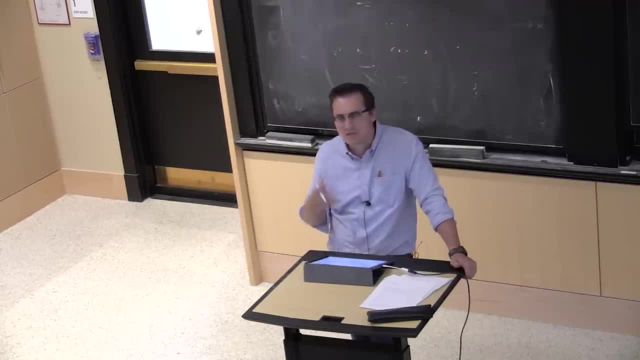 in statistics. If you've taken linear algebra, maybe we can explain to you why. If you've done some calculus, maybe we can do some interesting calculus. We'll see how, in the spirit of applied math, those things answer interesting questions. 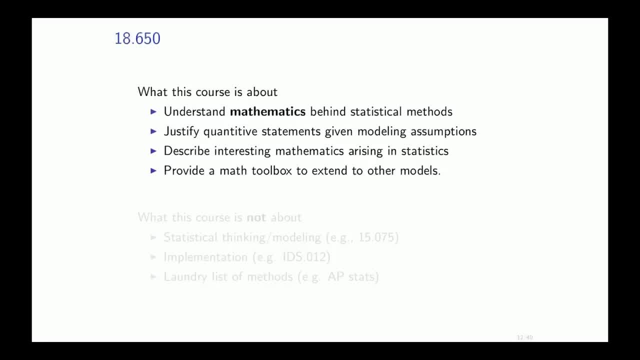 And basically we'll try to carve out a math toolbox that's useful for statistics And maybe you can extend it to more sophisticated methods that we did not cover in this class, In particular in your machine learning class. hopefully you'll be able to have some statistical intuition. 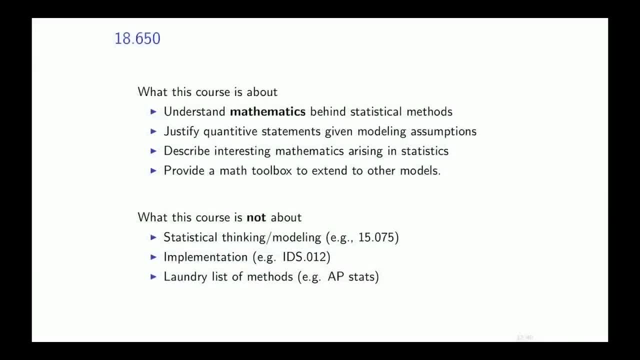 about what is going on. So what this course is not about, it's not about, you know, spending a lot of time looking at data sets and trying to understand some statistical thinking when it comes to questions. So this is more of an applied statistic perspective. 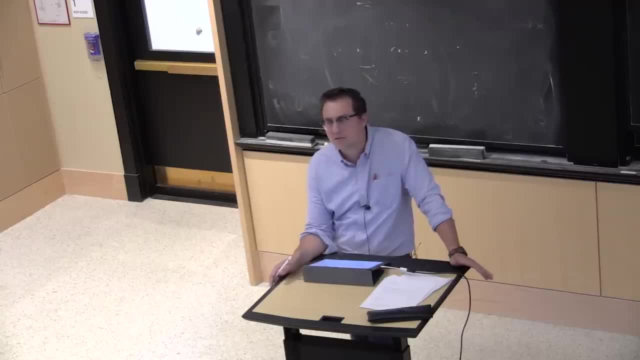 on things or more modeling. So I'm going to typically give you the model, So I'm going to say this is the model And this is how we're going to build an estimator in the framework of this model. So, for example, 18.075, to a certain extent. 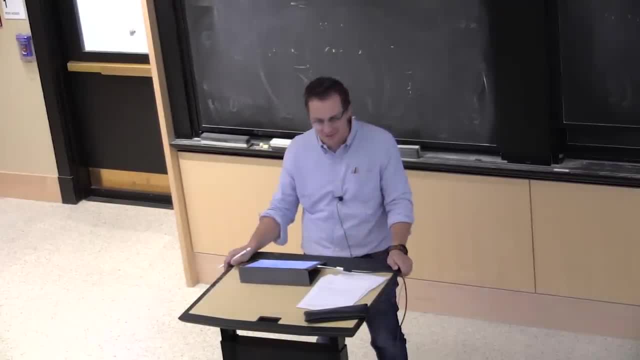 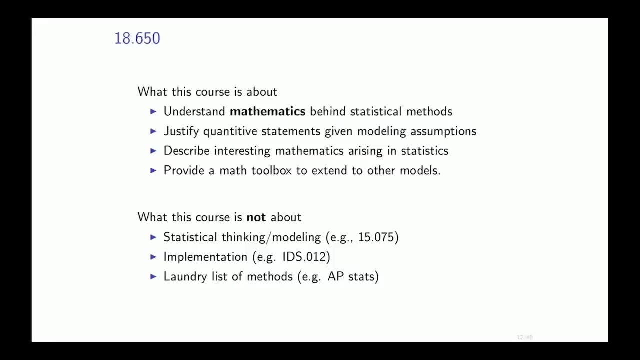 is called statistical thinking and data analysis, So I'm hoping there is some statistical thinking in there. We will not talk about software implementation. Unfortunately, there's just too little time in a semester. There's other courses that are giving you some overview. 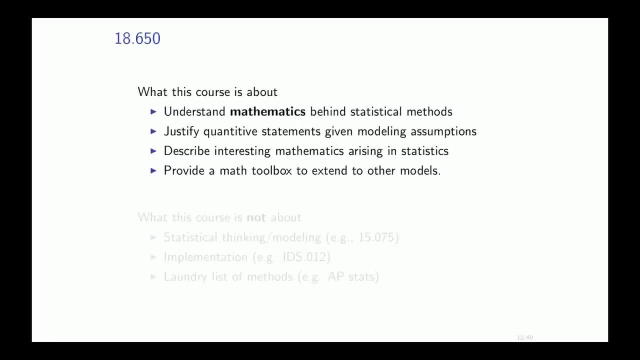 So this was why statistics. So what is this course about? It's about understanding the mathematics behind statistical methods. It's more of a tool. We're not going to have fun and talk about algebraic geometry just for fun in the middle of it. 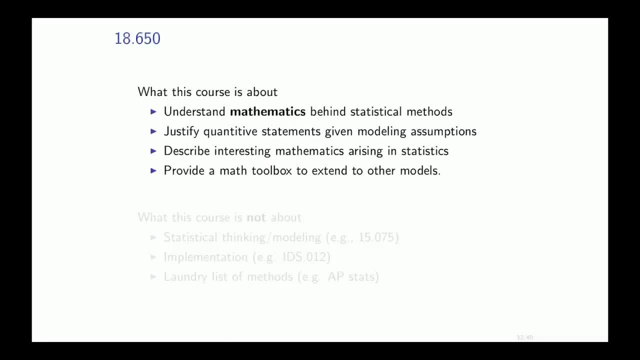 So justify quantitative statements given some modeling assumptions. So we will, in this class, mostly admit that the modeling assumptions are correct In the first part in this introduction. we will go through them, because it's very easy to forget what assumptions 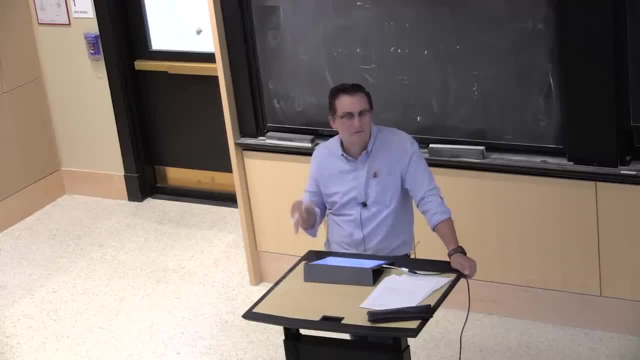 You're actually making, But this will be a pretty standard thing. The words you will hear a lot are IID independent and identically distributed. That means that your data is basically all the same and one data point is not impacting another data point. 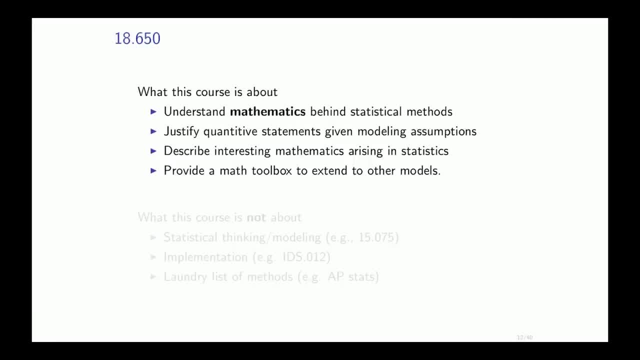 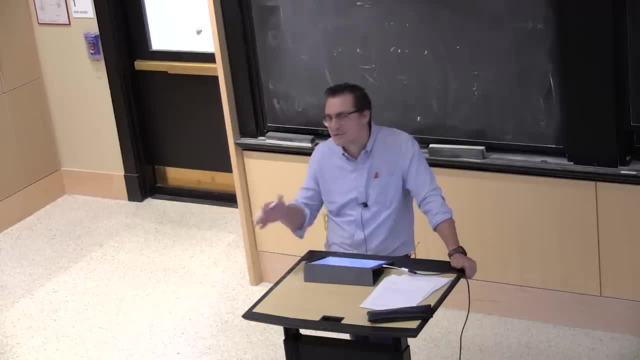 Hopefully we can describe some interesting mathematics arising in statistics. If you've taken linear algebra, maybe we can explain to you why. If you've done some calculus, maybe we can do some interesting calculus. We'll see how, in the spirit of the data. 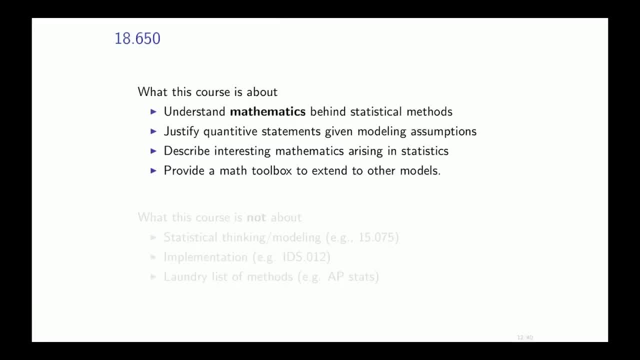 in the spirit of applied math. those things answer interesting questions And basically we'll try to carve out a math toolbox that's useful for statistics And maybe you can extend it to more sophisticated methods that we did not cover in this class, in particular in your machine learning class. 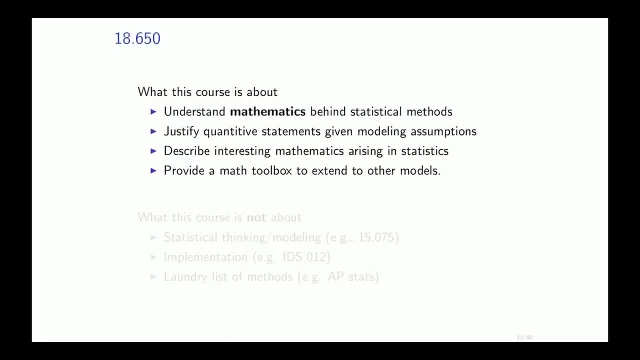 Hopefully you'll be able to have some statistical intuition about what is going on. So what this course is not about? it's not about spending a lot of time looking at data sets and trying to understand. It's about looking at some statistical thinking. 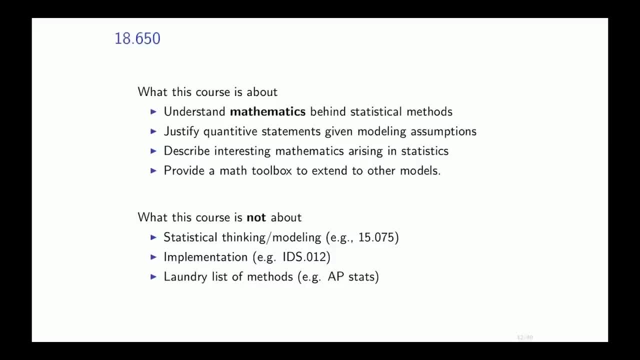 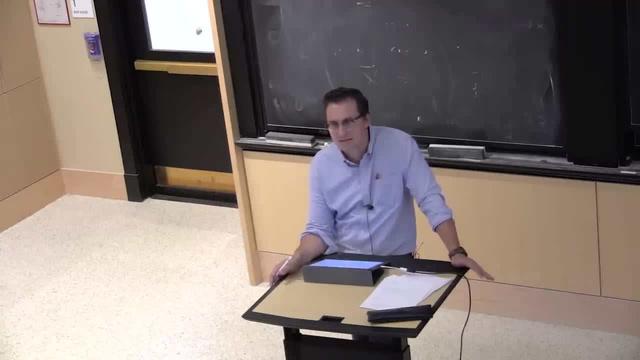 kind of questions. So this is more of an applied statistic perspective on things or more modeling. So I'm going to typically give you the model. I'm going to say: this is the model and this is how we're going to build an estimator. 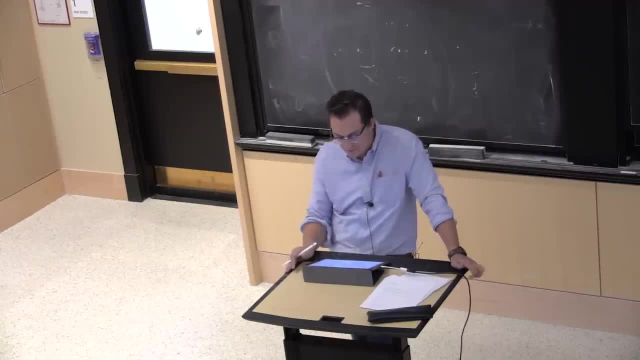 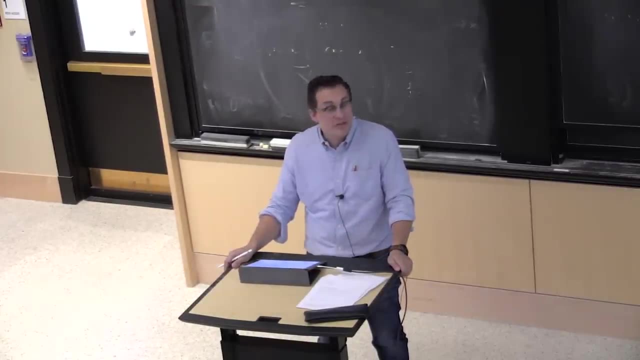 in the framework of this model. So, for example, 18.075, to a certain extent is called statistical thinking and data analysis, So I'm hoping there is some statistical thinking in there. We will not talk about software implementation, unfortunately. 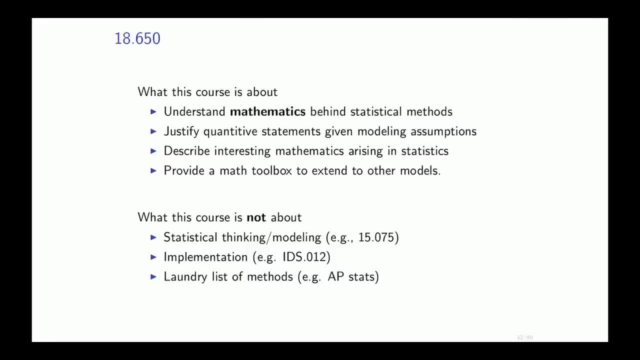 There's just too little time, So I'm going to give you a little bit of an overview of what we're going to do in a semester. There's other courses that are giving you some overview. So the main softwares these days are: 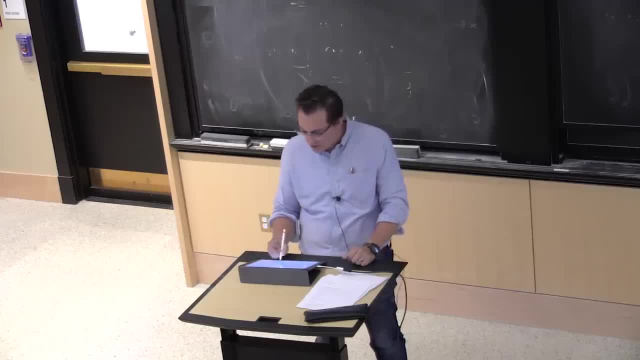 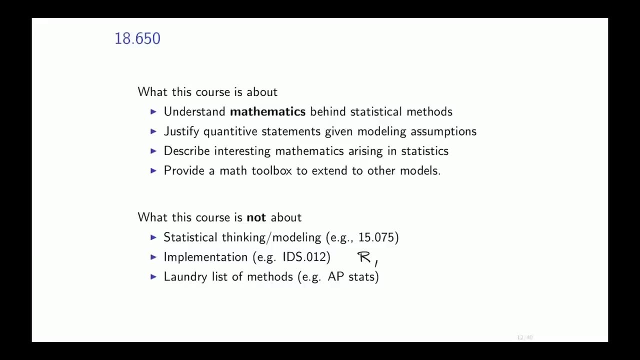 So the main softwares these days are: so R is the leading software, I'd say, in statistics, both in academia and industry. Lots of packages, one every day, that's probably coming out, But there's other things, right. So now you know Python is probably catching up. 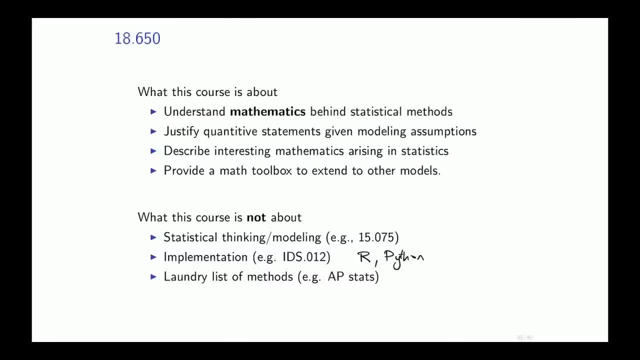 with all this. You know scikit-learn packages that are coming up. Julia has some statistics in there. But really, R, if you were to learn statistical software- and let's say you love doing this- this would be the one that would prove most useful for you. 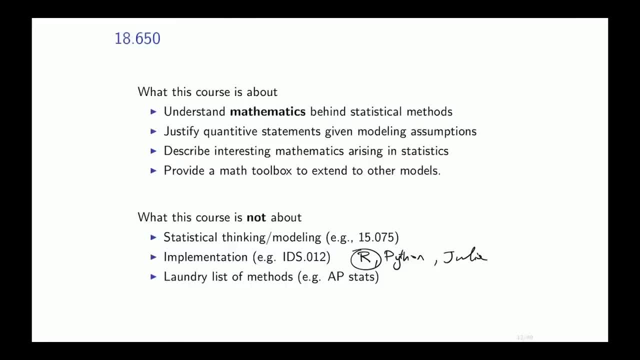 in the future. It does not scale super well to high-dimensional data. So there's a class in IDSS that actually uses R. It's called IDS 012.. And I think it's called statistics, computation and applications or something like that. Yeah. 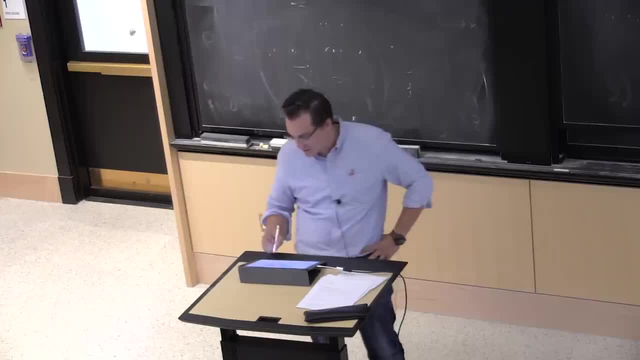 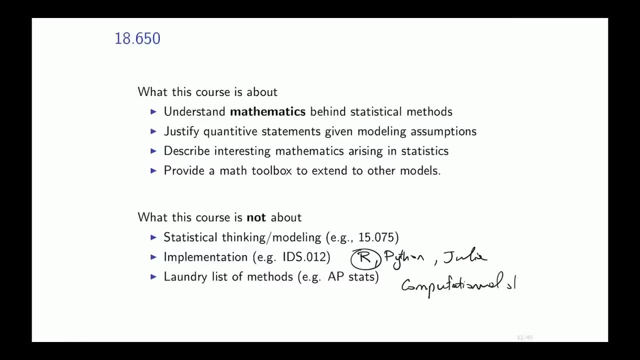 Yeah, Yeah, Something like this. I'm also preparing, with Peter Kempthorne, a course called Computational Statistics. It's going to be offered this spring as a special topics, And so Peter Kempthorne will be teaching it, And this class will actually focus on using R. 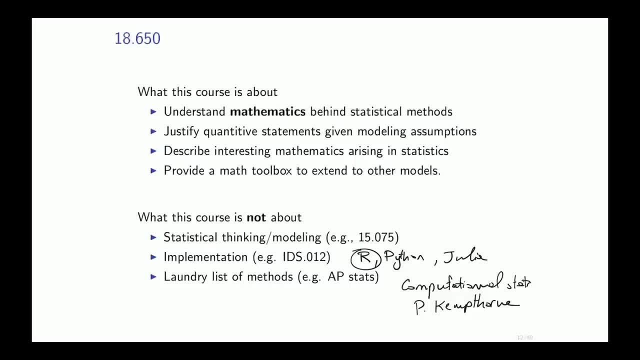 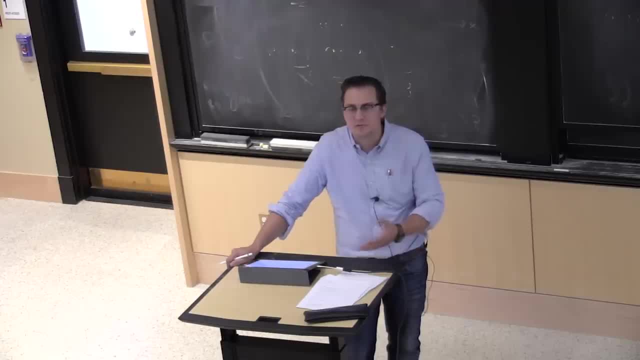 And even beyond that, it's not just going to be about using, It's going to be about understanding. the same way, we're going to see how math- How math helps you do statistics- is going to help see how math helps you do algorithms for statistics. 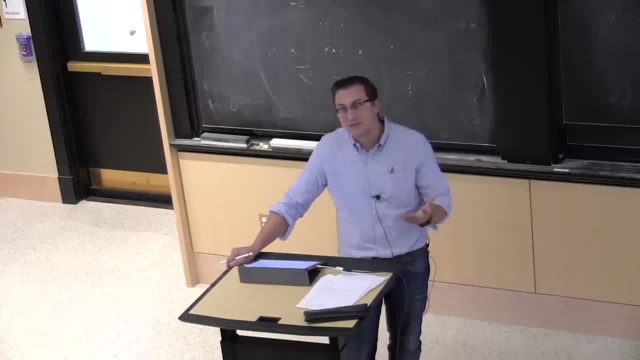 So we'll talk about maximum likelihood estimator. We'll need to maximize some function. There's optimization toolbox to do that And we'll see how we can have specialized for statistics for that and what are the principles behind it. And, of course, if you've taken AP Stats, 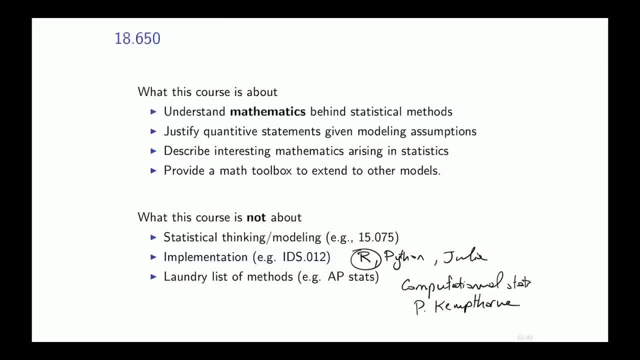 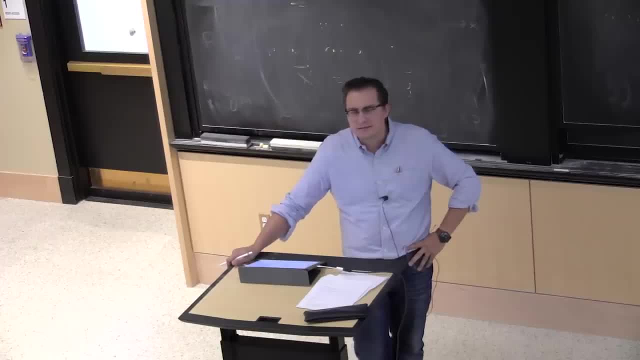 you probably think that Stats is boring to death because it was just a long laundry list that spent a lot of time on t-test. I'm pretty sure we're not going to talk about t-test. Well, maybe once, But this is not a matter of saying you're going to do this. 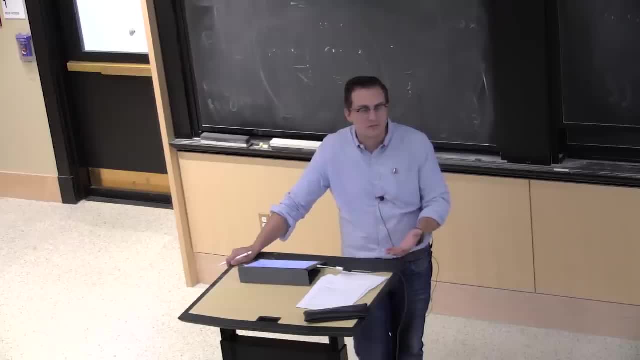 and this is a slight variant of it. We're going to really try to understand what's going on. So, admittedly, you have not chosen the simplest way to get an A in statistics on campus. This is not the easiest class. It might be challenging at times. 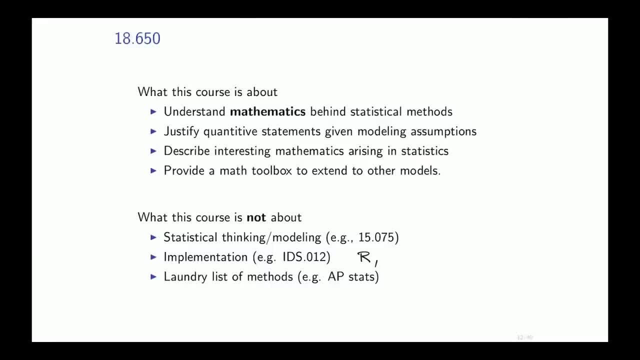 so R is the leading software, I'd say, in statistics, both in academia and industry. Lots of packages, one every day that's probably coming out, But there's other things, right. So now Python is probably catching up with all this. 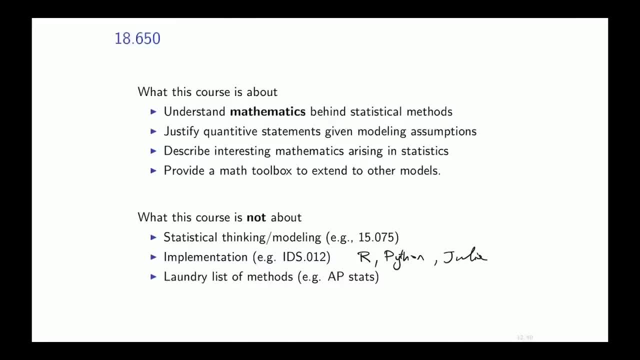 and Julia has some statistics in there, But really R. if you were to learn statistical software- and let's say you love doing this- this would be the one that would prove most useful for you in the future. It does not scale super well to high-dimensional data. 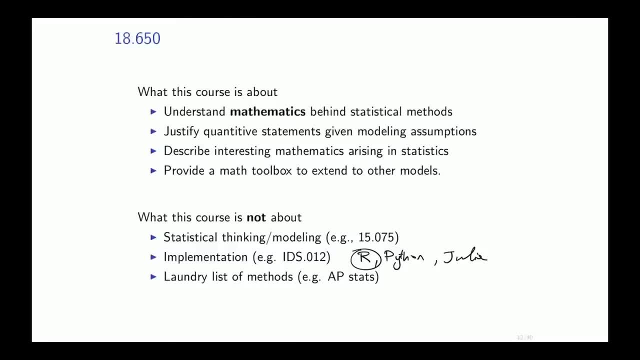 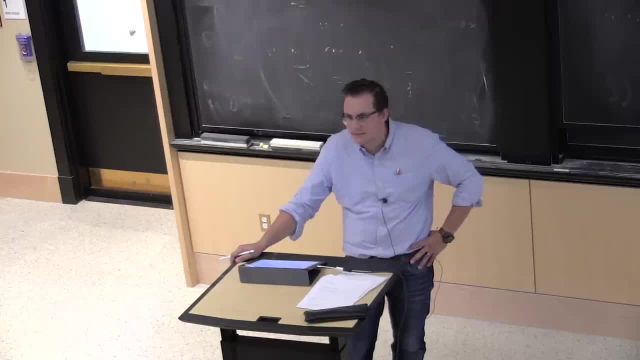 So there's a class in IDSS that actually uses R. It's called IDS 012, and I think it's called Statistics, Computation and Applications or something like this. I'm also preparing with Peter Kempthorne a course called Computational Statistics. 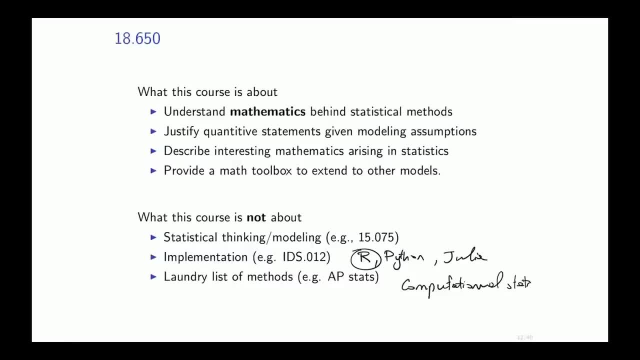 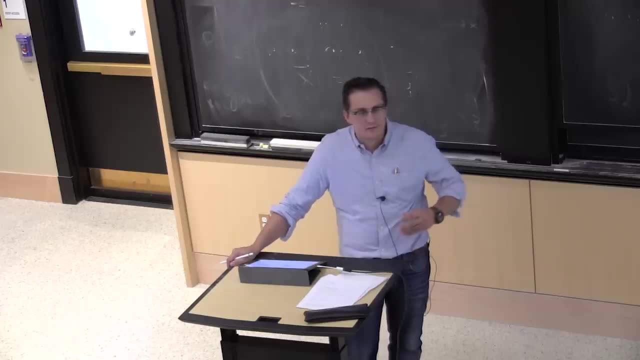 It's going to be offered this spring as a special topics, And so Peter Kempthorne will be teaching it, And this class will actually focus on using R And even beyond that. it's not just going to be about using, It's going to be about understanding. 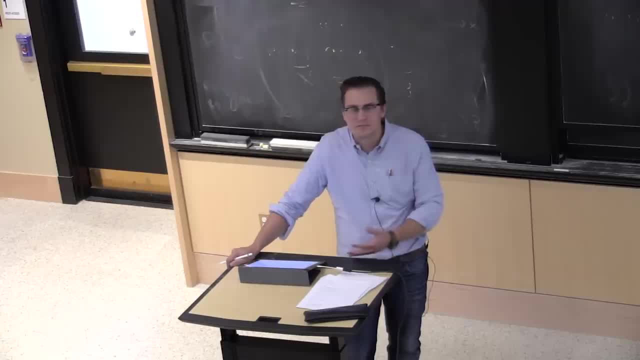 The same way we're going to see how math helps you do statistics is going to help see how math helps you do algorithms for statistics. So we'll talk about maximum likelihood estimator. We'll need to maximize some function. There's an optimization toolbox to do that. 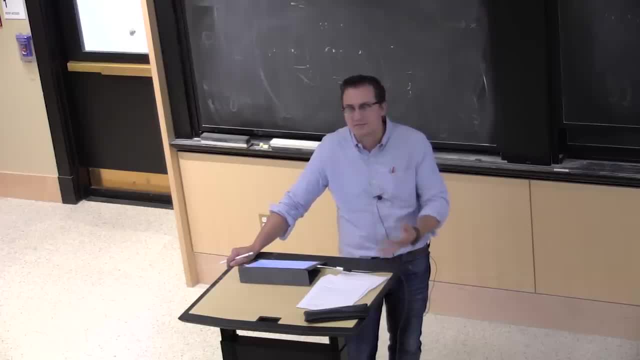 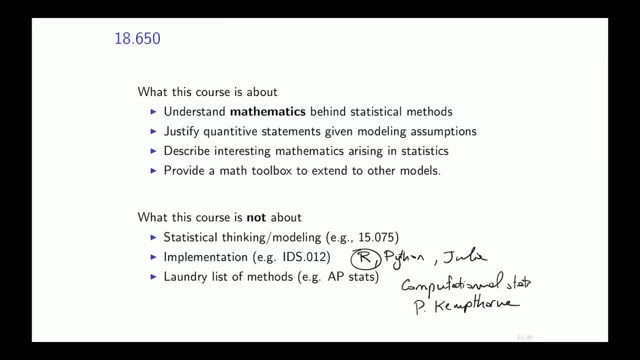 And we'll see how we can have specialized for statistics for that and what are the principles behind it. And, of course, if you've taken AP Stats, you probably think that Stats is boring to death because it was just a long laundry list that. 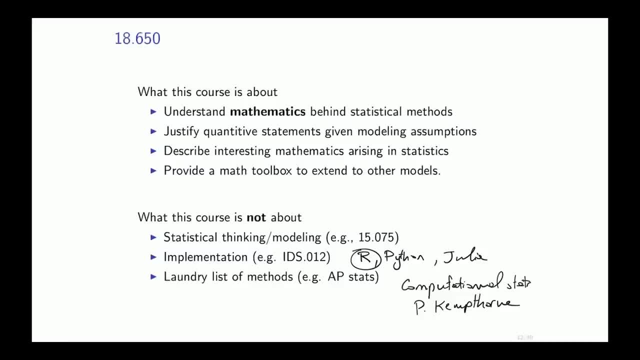 spent a lot of time on t-test. I'm pretty sure we're not going to talk about t-test. well, maybe once, But this is not a math test. We're going to talk about it in a little bit. So we're going to talk about it in a little bit. 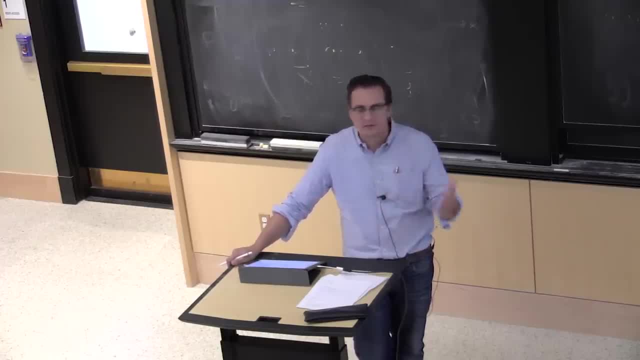 So we're going to talk about it in a little bit. So we're going to talk about it in a little bit. It's not a matter of saying you're going to do this and this is a slight variant of it. We're going to really try to understand what's going on. 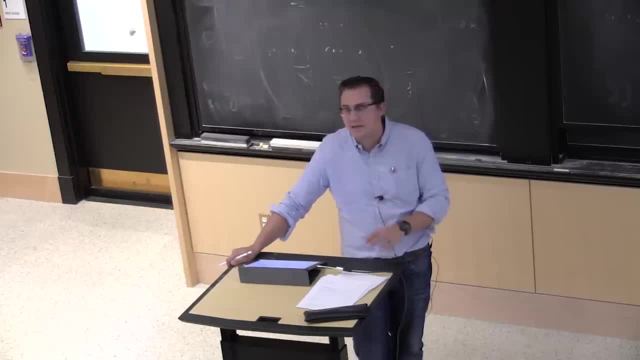 So, admittedly, you have not chosen the simplest way to get an A in statistics on campus. This is not the easiest class. It might be challenging at times, but I can promise you that you will maybe suffer, but you will learn something by the time you're. 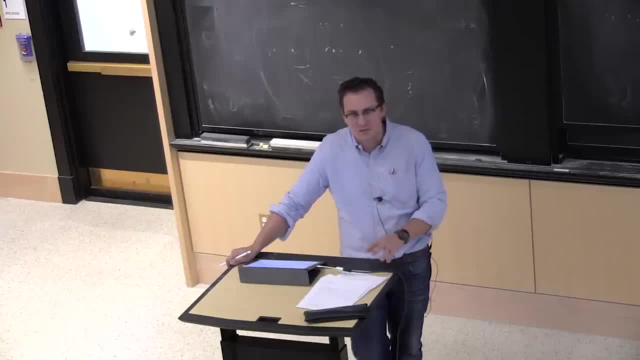 but I can promise you that you will maybe suffer, but you will learn something by the time you're out of this class. This will not be a waste of your time And you will be able to understand, And not having to remember by heart- how those things actually 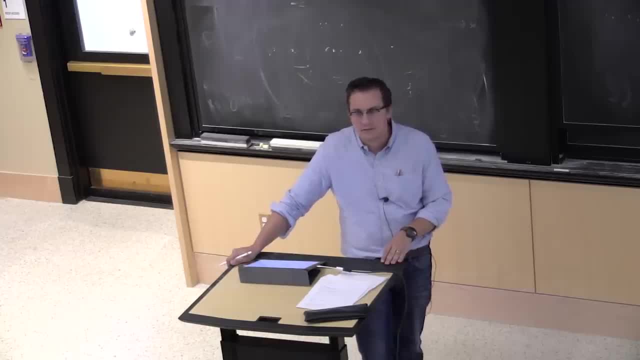 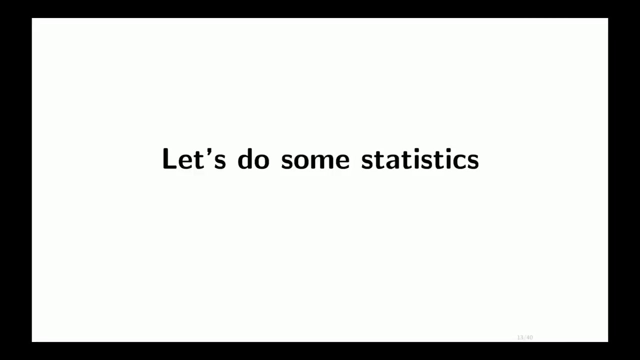 work. Are there any questions? Anybody wants to go to another stats class on campus? Maybe it's not too late. OK, So let's do some statistics. So I see the time now And it's 1156.. So we have another 30 minutes. 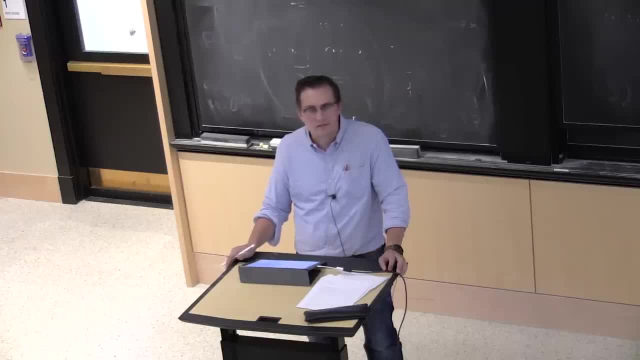 I will typically give you a three, four minutes break, if you want to stretch, if you want to rent the bathroom, if you want to check your texts or Instagram. There was very little content in this class. Hopefully it was entertaining enough that you don't need the break. 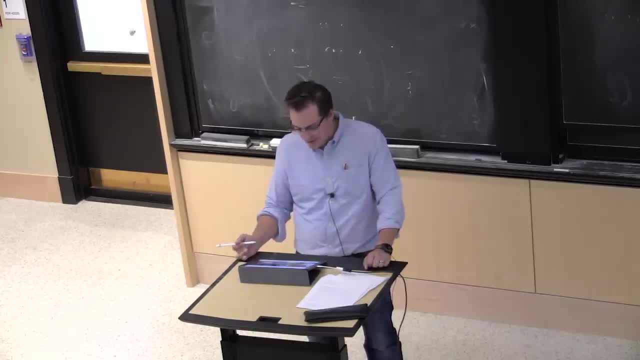 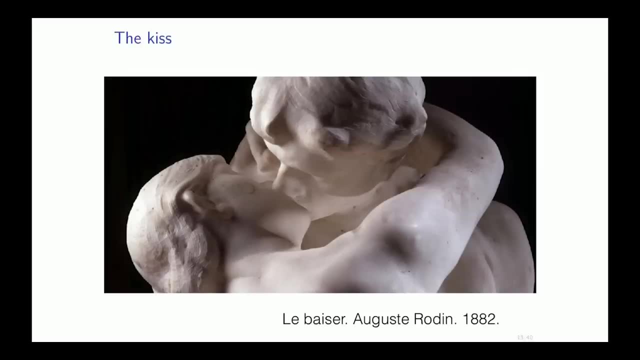 But just in the future. so you know you will have a break. OK, so statistics. this is how it starts. All right, I'm French. What can I say? I need to put some French words. So that's it. So this is not how office hours are going to go down. 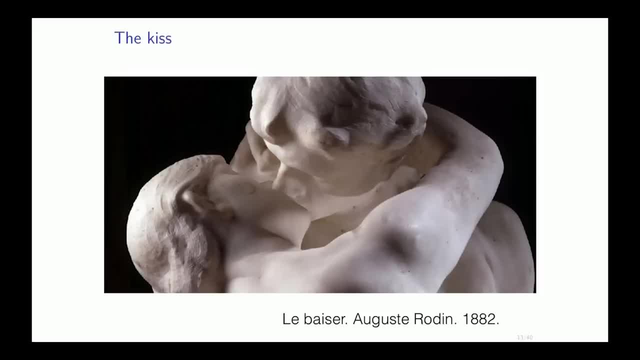 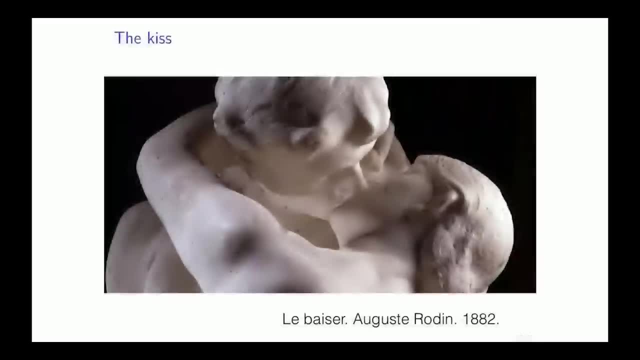 So anybody knows this sculpture by Alvedo The kiss. Maybe probably the thinker is more famous, but this is actually a pretty famous one. But is it really this one or is it this one? Anybody knows which one? it is This one. 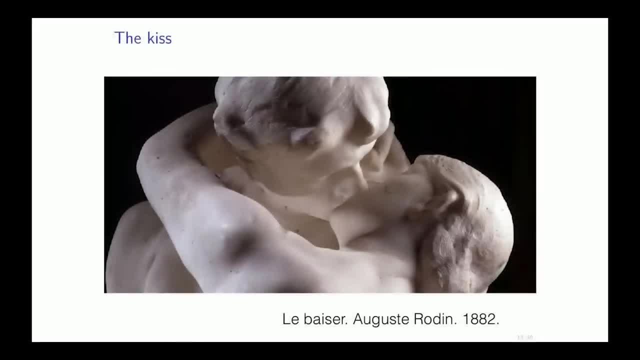 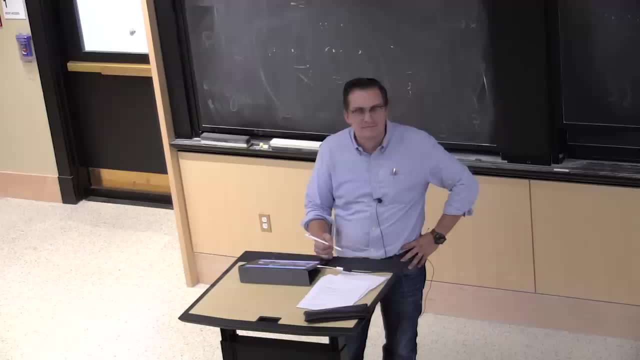 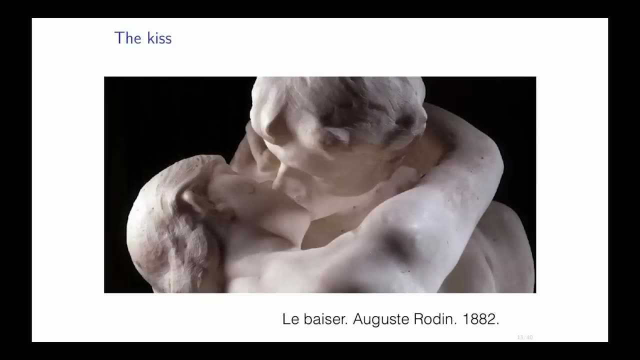 Or this one? What's that? This one? It's this one. Five minutes, Yeah, Anybody Who votes for this one? OK, Who votes for that one? Thank you, I love that you do not want to pronounce yourself with no data. 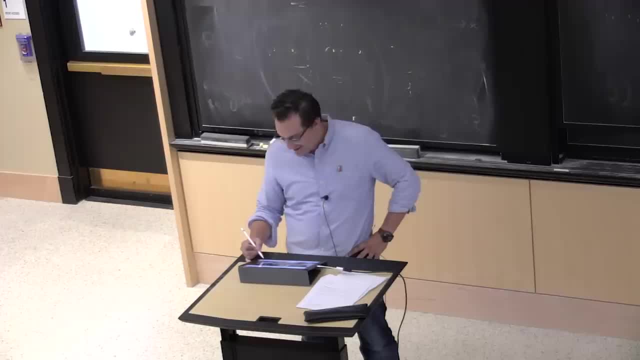 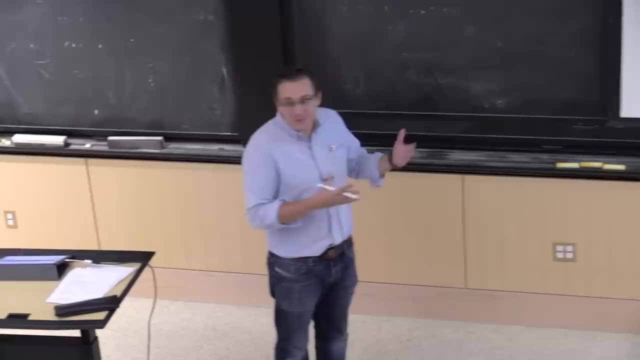 actually to make any decision. This is a tool going to us, right. Turns out that there is data and there's. in the very serious journal Nature, Someone published a very serious paper which actually looks pretty serious, right, If you look at it, it's like human behavior, adult. 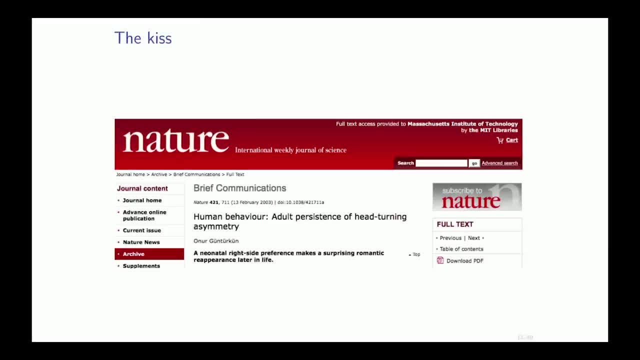 persistence of head turning asymmetry. I mean, there's a lot of fancy words in there. Yeah, Yeah, And I'm not kidding you. This study is about collecting data of people kissing and knowing if they bend their head to the right. 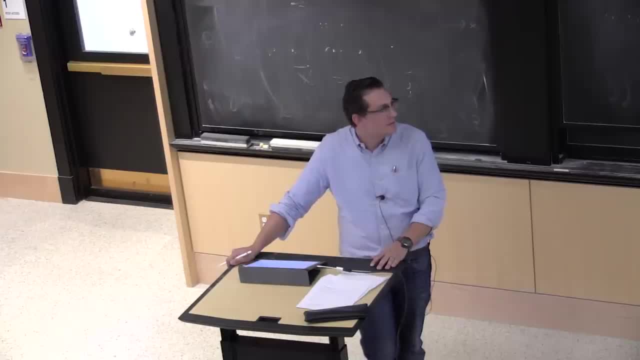 out of this class. This will not be a waste of your time And you will be able to understand, and not having to remember by heart, how those things actually work. Are there any questions? Anybody wants to go to another stats class on campus? 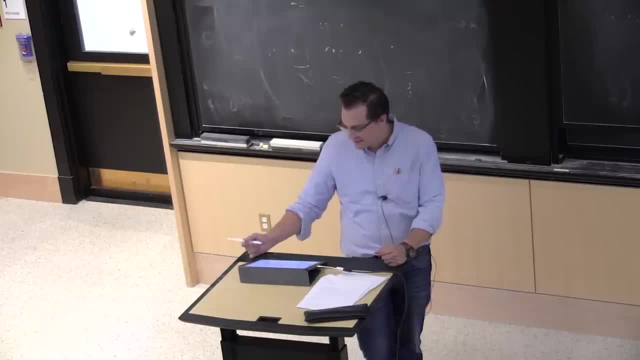 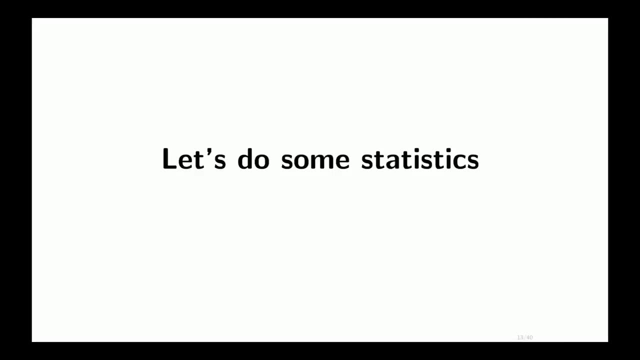 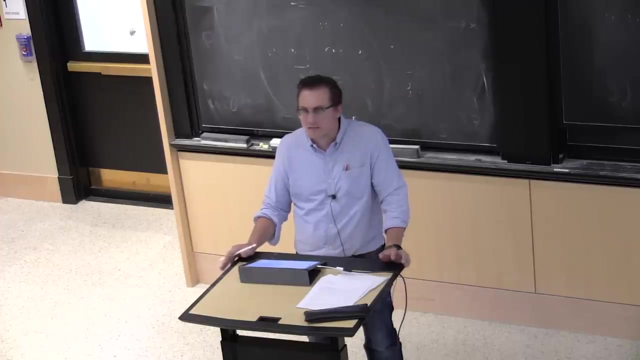 Maybe it's not too late, OK, So let's do some statistics. So I see the time now and it's 1156.. So we have another 30 minutes. I will typically give you a three, four minutes break if you want to stretch, want to rent the bathroom. 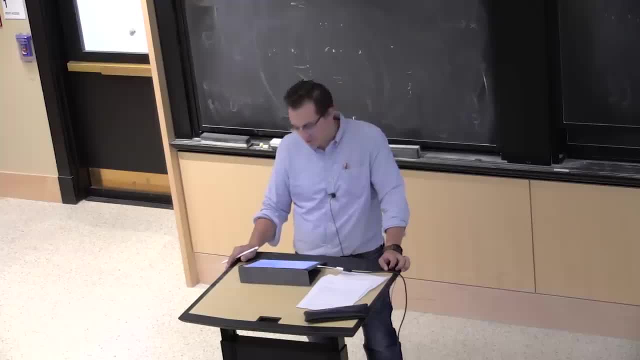 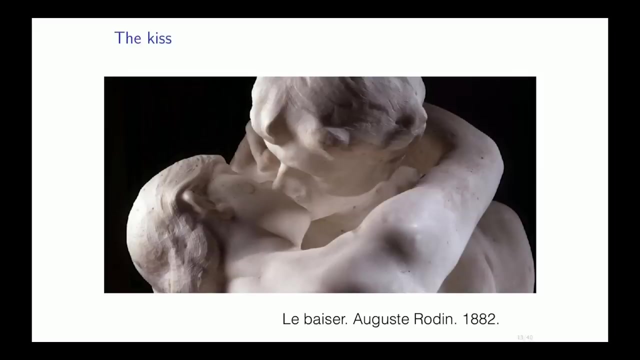 if you want to check out, Check your texts or Instagram. There was very little content in this class. Hopefully it was entertaining enough that you don't need the break, But just in the future, so you know you will have a break. OK, so statistics is. this is how it starts, all right. 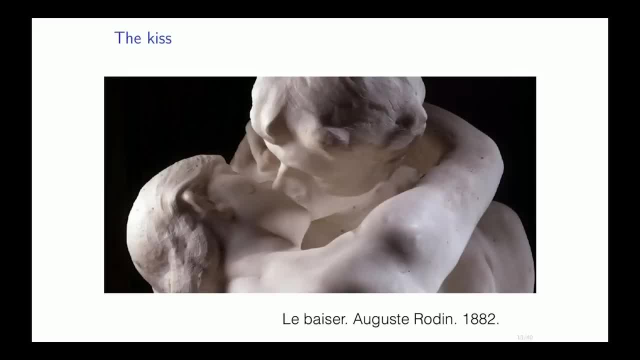 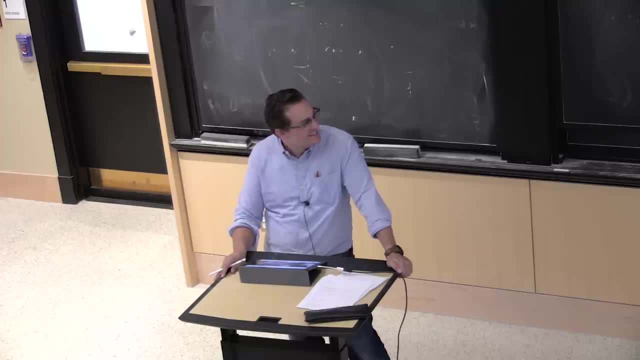 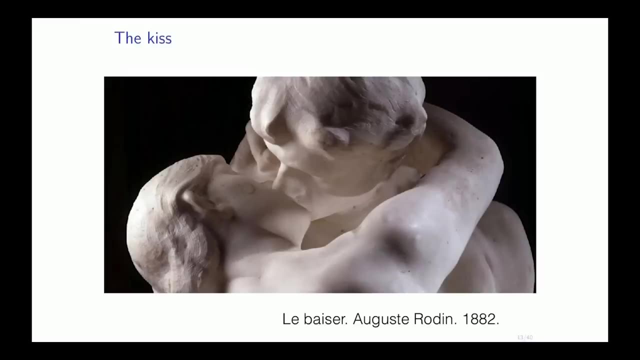 I'm French. What can I say? I need to put some French words. So this is not how office hours are going to go down. So anybody knows this sculpture by Rodin, The Kiss. Maybe probably the thinker is more famous. 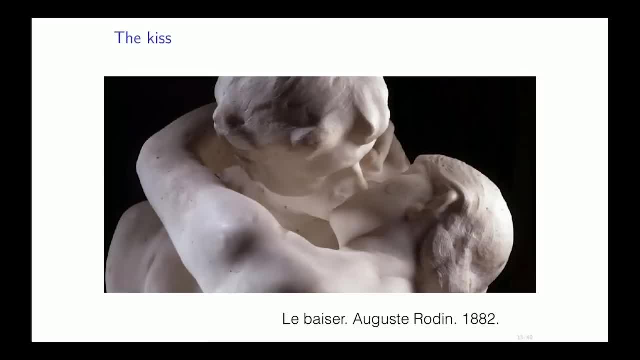 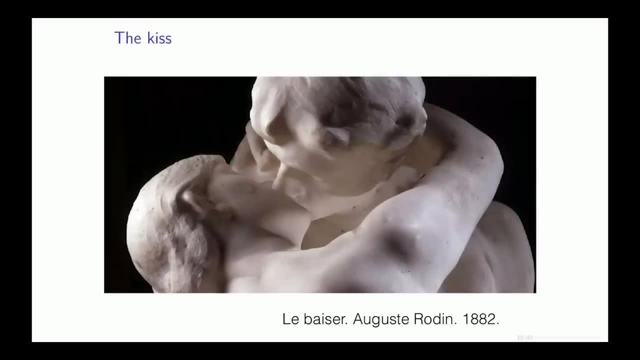 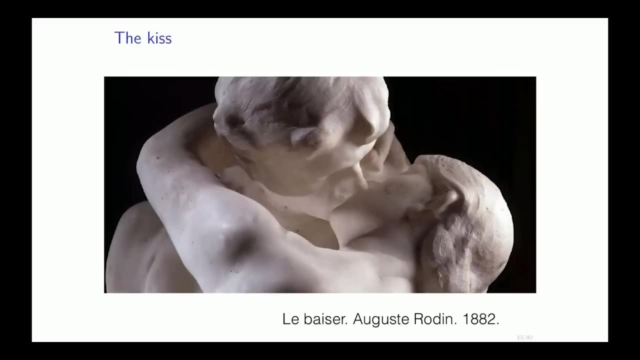 but this is actually a pretty famous one. But is it really this one, or is it this one? Anybody knows which one. it is This one or this one? What's that? This one? It's this one. Five minutes Yeah. 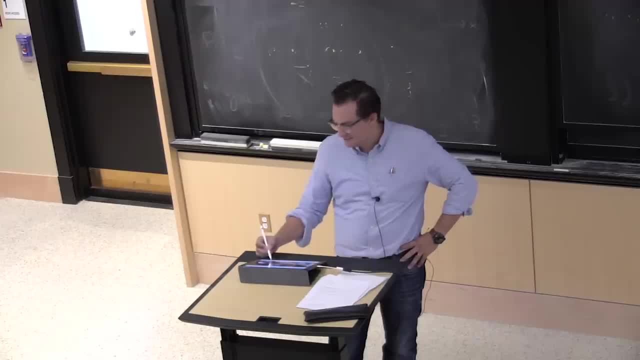 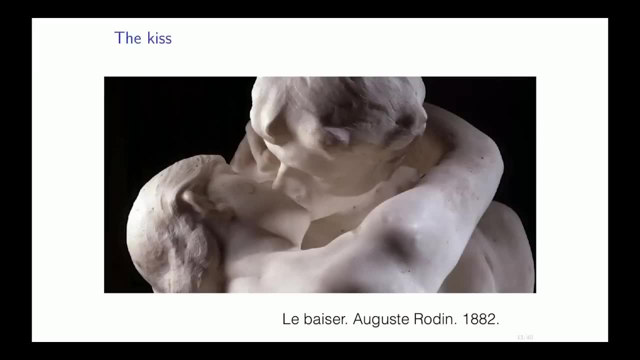 Who votes for this one? OK, OK, OK, OK, Who votes for that one? Thank you, I love that you do not want to pronounce yourself with no data actually to make any decision. This is a tool going to us, right. 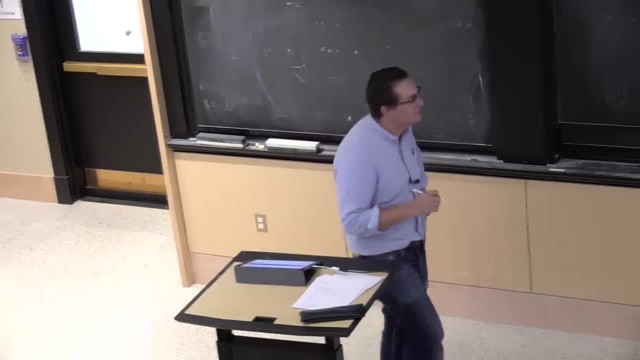 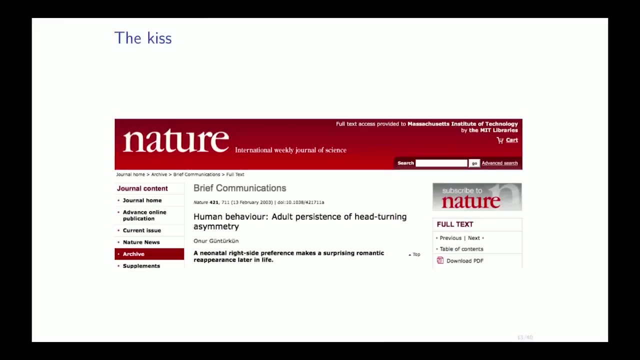 Turns out that there is data and there's in the very serious journal Nature, Someone published a very serious paper which actually looks pretty serious, right, If you look at it, it's like human behavior, adult persistence of head turning, asymmetry. 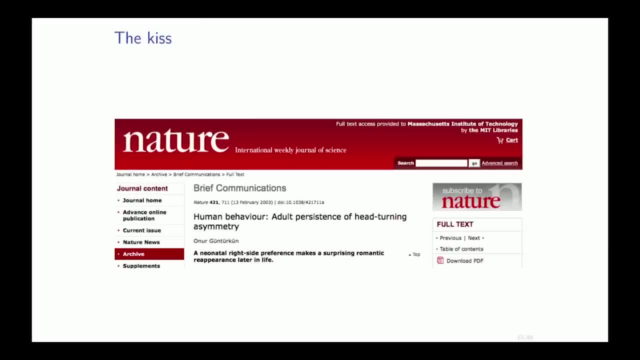 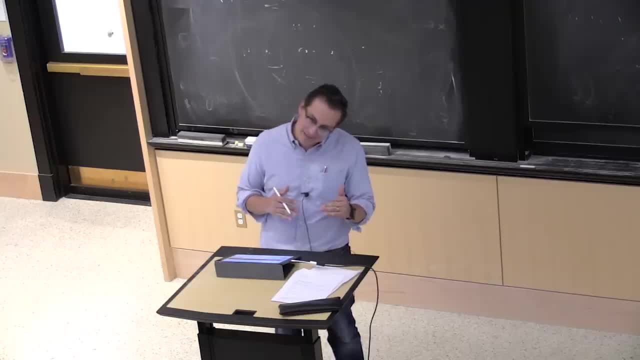 I mean, there's a lot of fancy words in there And I'm not kidding you. This study is about collecting data of people. OK, And it's a very hard part, But if you burned your head in a party with a woman, 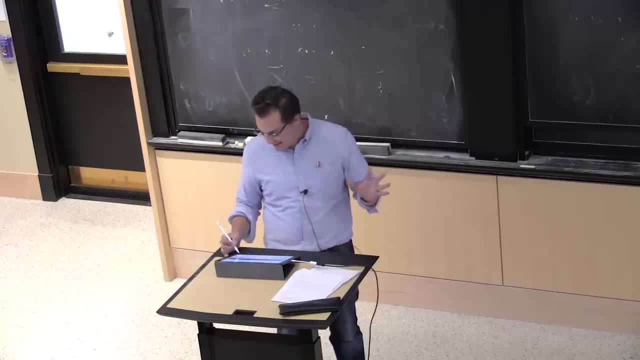 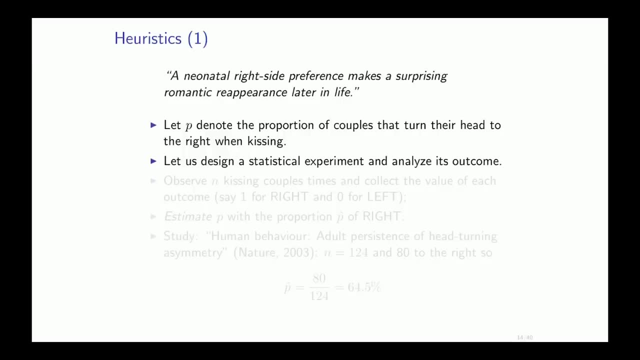 or if they bend their head to the left, And that's all it is. And so a neonatal right side preference makes a surprising romantic reappearance in later life. There's an explanation for it, All right. so if we follow this nature, which one is the one? 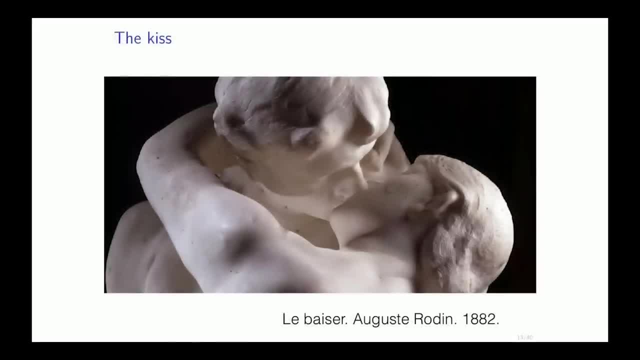 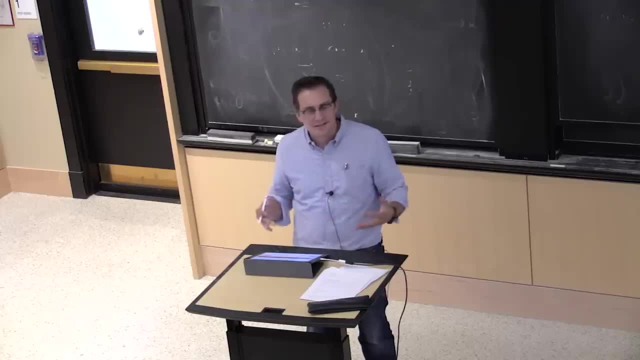 This one or this one, This one right. So head to the right. And to be fair for this class, I was like, oh, I'm going to go and show them what Google Images does. when you Google kissing couple, It's inappropriate after maybe, the first picture. 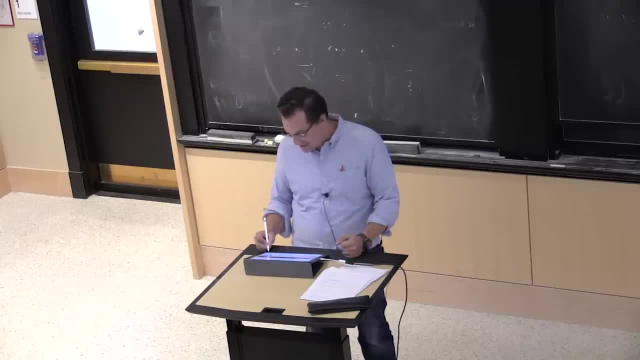 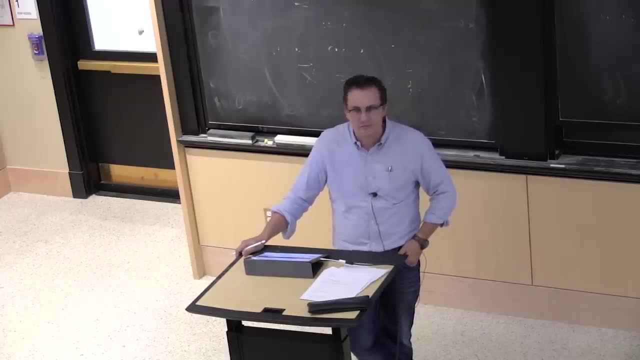 And so I cannot show you this, but you can check for yourself, Though I would argue so. this person here actually went out in airports and took pictures of strangers kissing and collecting the data, This data, And can somebody guess why they did just not stay home? 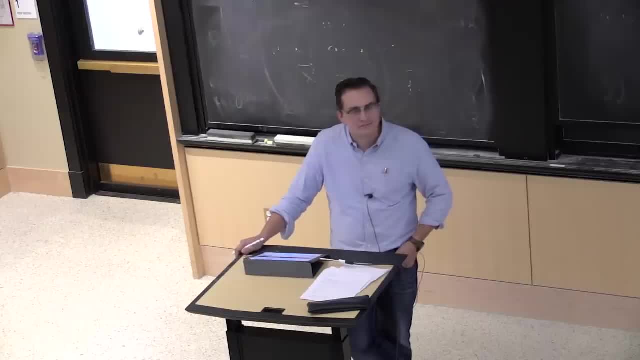 and collect data from Google Images by just Googling kissing couples. What's wrong with this data? I didn't know, actually, before I actually went on Google Images. It can be altered. PHILIPPE RIGOLLET- What's that? 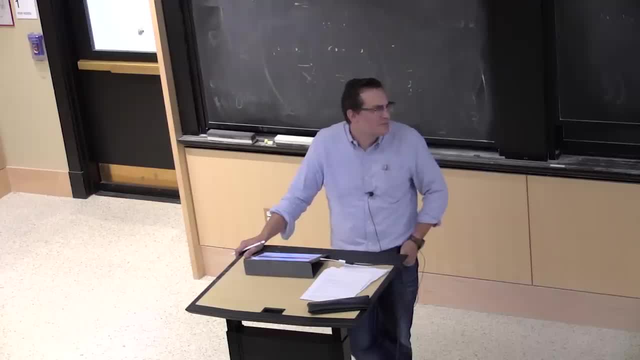 It can be altered. PHILIPPE RIGOLLET- It can be altered, But who would want to do this? I mean, there's no particular reason why you would want to flip an image before putting it out there. I mean you might, but maybe they. 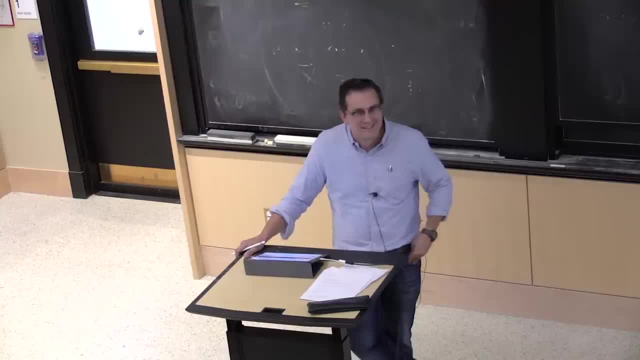 want to hide the brand of your Gap shirt or something? Yeah, I guess the people who post pictures of themselves kissing on Google Images are not representative of the general public. PHILIPPE RIGOLLET- Yeah, that's very true. 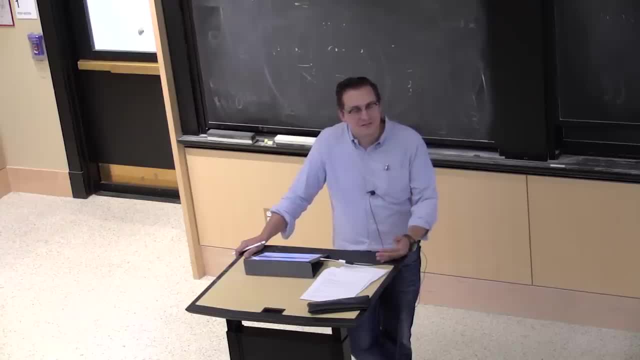 And actually it's even worse than that. The people who post pictures of themselves are not posting pictures of themselves. They're putting pictures of the people they took a picture of And there usually is a stock watermark on this And it's basically stock images. 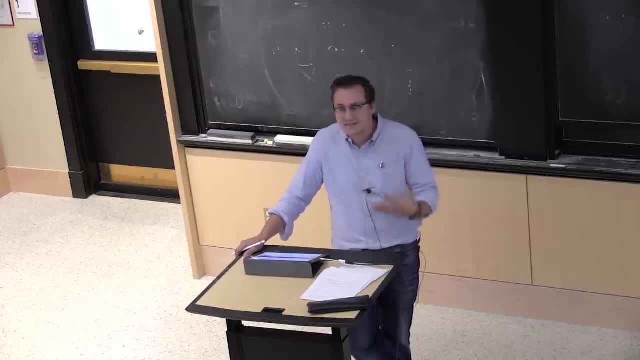 Those are actors And so they've been directed to kiss, And this is not a natural thing to do. And actually, if you go on Google Images- and I encourage you to do this unless you don't want to see inappropriate pictures of them- 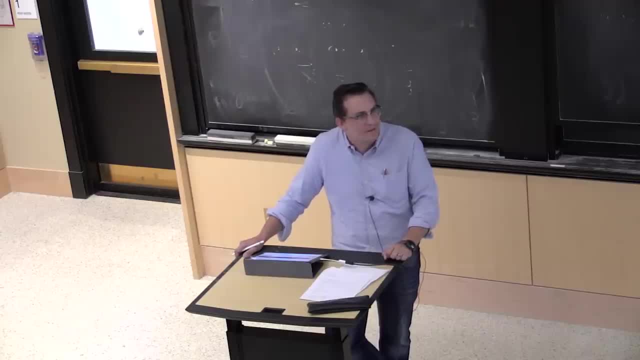 They're mightily inappropriate And basically you will see that this study is actually not working at all. I mean, I looked briefly- I didn't actually collect numbers- But I didn't find a particular tendency to have been right. If anything, it was actually probably the opposite. 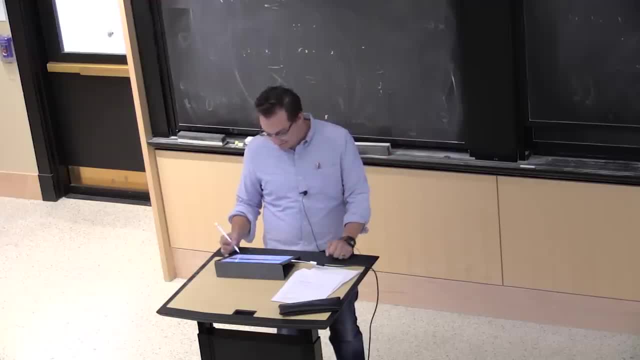 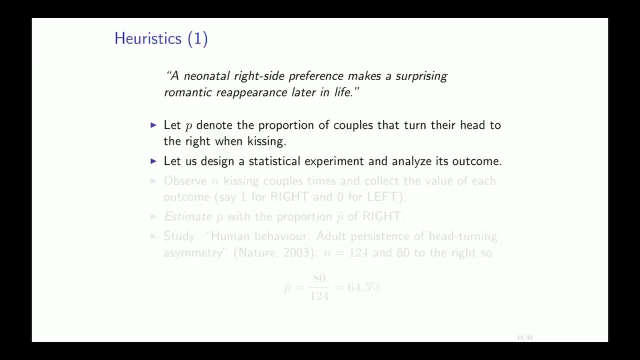 you probably wouldn't have seen a woman kissing and knowing if they bent their head to the right or if they bent their head to the left, And that's all it is. And so a neonatal right-side preference makes a surprising romantic reappearance in later life. 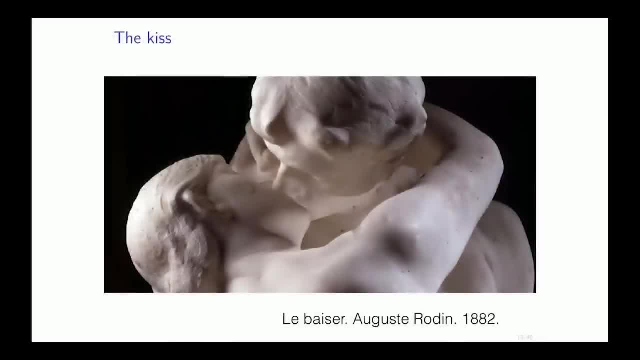 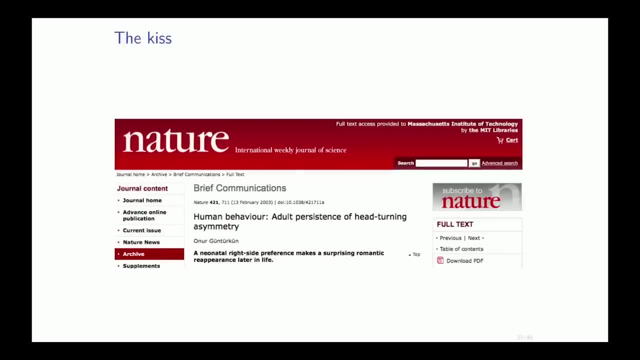 There's an explanation for it, All right. So if we follow this nature, which one is the one? This one, or this one, This one, right? And to be fair for this class, I was like, oh, I'm going to go and show them what you. 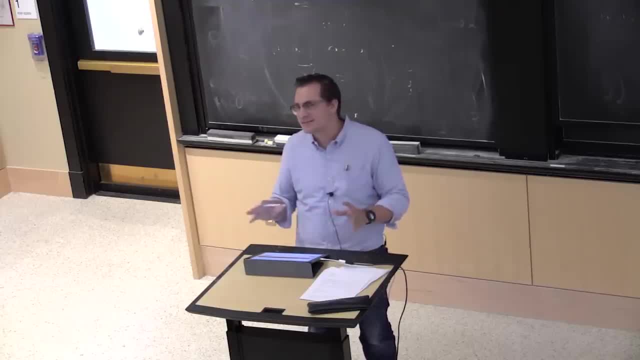 know Google Images does when you Google kissing couple. It's inappropriate after maybe the first picture, And so I cannot show you this. but you know you can check for yourself, Though I would argue so this person here actually went out in airports and took pictures. 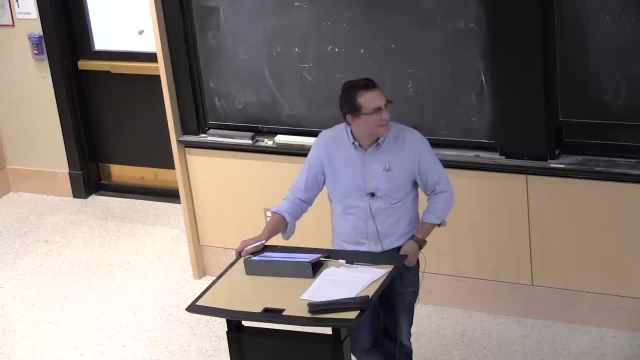 of strangers kissing and collecting this data, And can somebody guess why they did just not stay home and collect data from Google Images by just Googling? you know, kissing couples. What's wrong with this data? I didn't know, actually, before I actually went on Google Images. 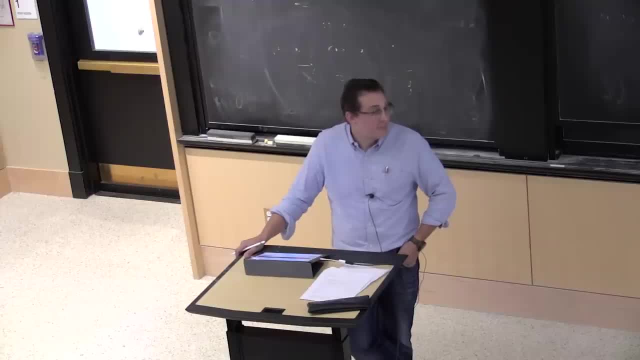 It can be altered. PHILIPPE RIGOLLET, It can be altered, but you know who would want to do this. I mean, there's no particular reason why you would want to flip an image before putting it out there. 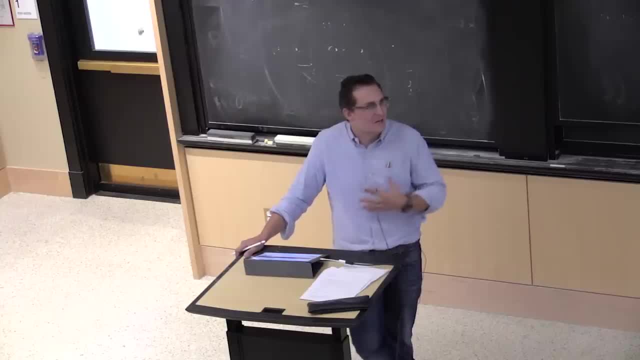 I mean, you know you might, but you know, maybe they want to hide the brand of your Gap shirt or something. Yeah, I guess the people who post pictures of themselves kissing on Google Images are not representative of the general public. 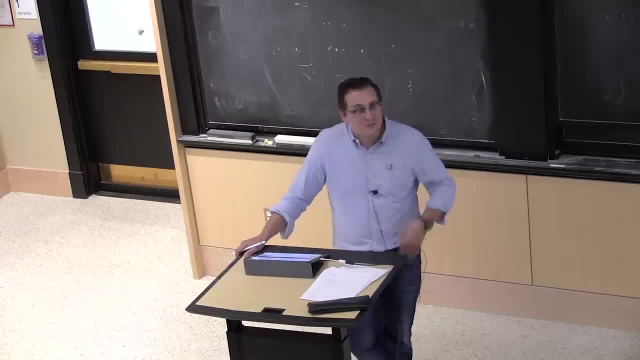 PHILIPPE RIGOLLET. Yeah, that's very true, And actually it's even worse than that. The people who post pictures of themselves are not posting pictures of themselves. They're putting pictures of the people they took a picture of. 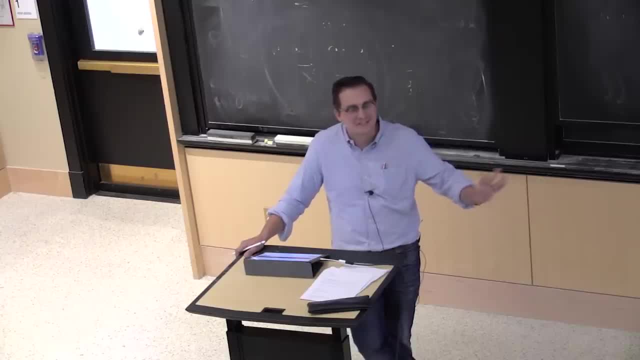 And there usually is a stock- you know, watermark on this and it's basically stock images. Those are actors And so they've been directed to kiss and this is not a natural thing to do. And actually, if you go on Google Images- and I encourage you to do this- unless you 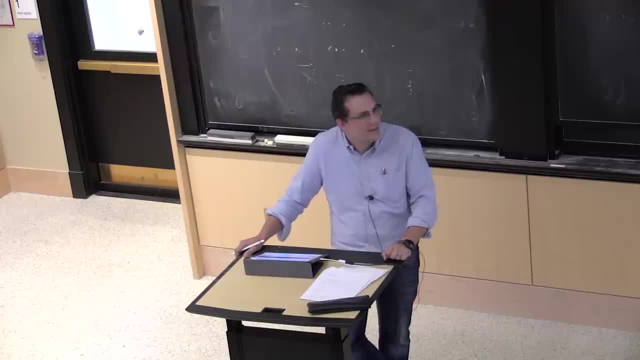 don't want to see inappropriate pictures. I mean they're mightily inappropriate And basically you will see that this study is actually not working at all. I mean, I looked briefly, I didn't actually collect numbers, but I didn't find a particular tendency to have been right. 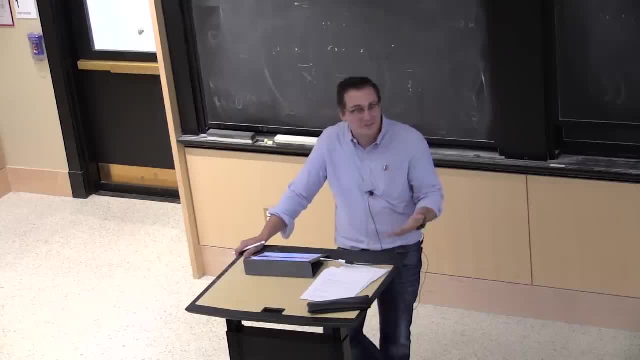 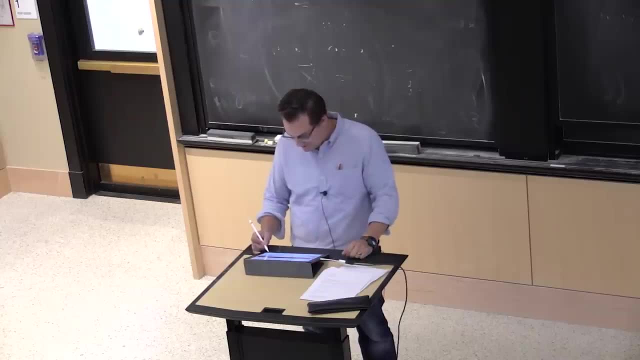 If anything, it was actually probably the opposite, And it's because those people were directed to do it and they actually think about doing it, And also because I think you need to justify writing a nature paper more than I said on front of my computer. 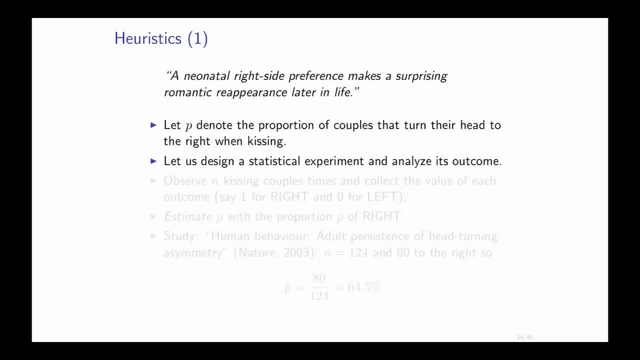 So again this first sentence here: a neonatal right-side preference is there? a right-side preference is not a mathematical question, But we can start saying: let blah and put some variables and ask questions about those variables. all right, 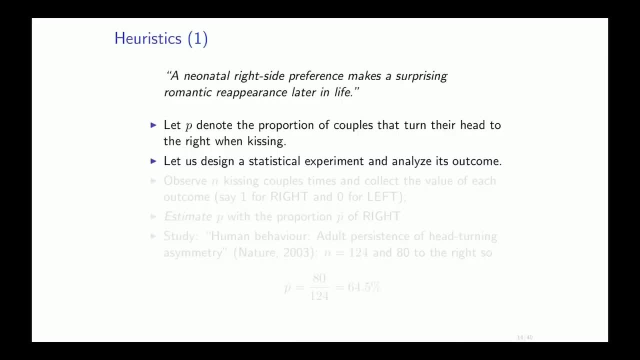 So you know x is actually not a variable that's used very much in statistics for parameters. p is one for parameter, And so you're going to take your parameter of interest, p, and here is going to be the proportion of couples. 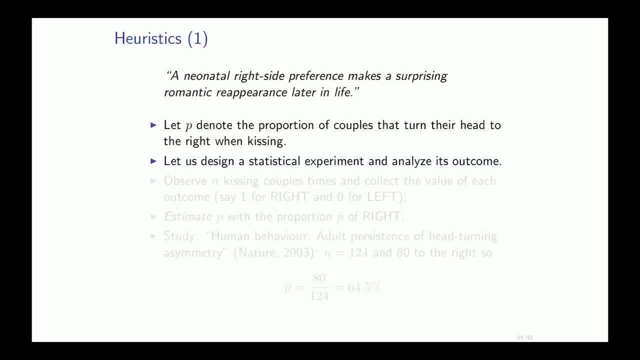 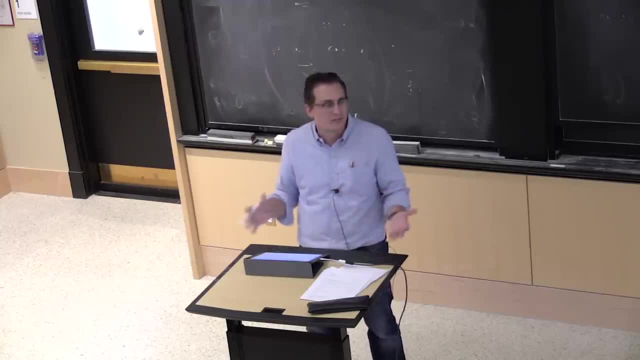 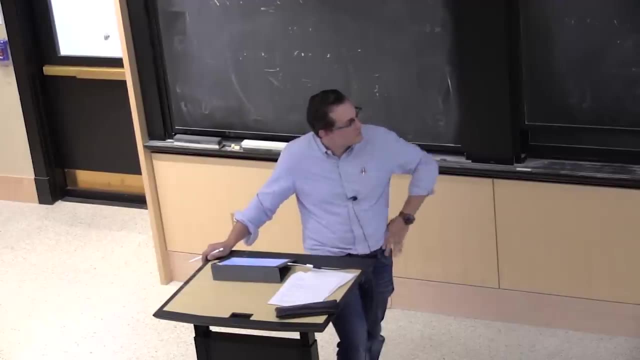 And that's among all couples. So here, if you talk about statistical thinking, there would be a question about what population this would actually be representative of. So usually this is a call to your sorry. I should not forget this word. 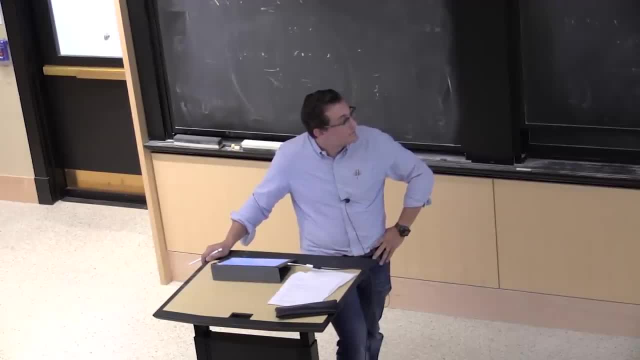 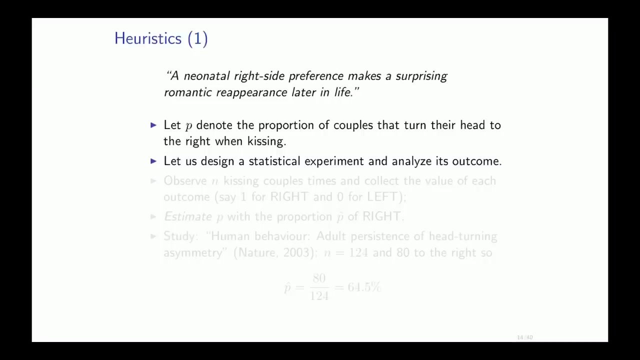 It's important for you. OK, I forget this word, Sorry. So this is OK. so, if you look at this proportion, maybe these couples that are in this study might be representative only of couples in airports. Maybe they actually put on a show for the other passengers. 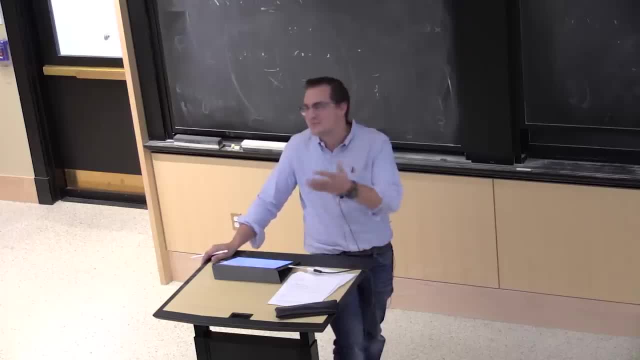 Who knows, Like, oh, let's just do this well, And just like the people on Google Images are actually doing it, So maybe you want to just restrict it. But of course, clearly, if it's appearing in nature, it should not be only about couples. 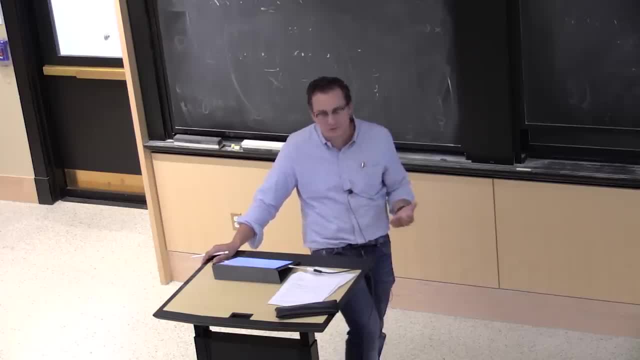 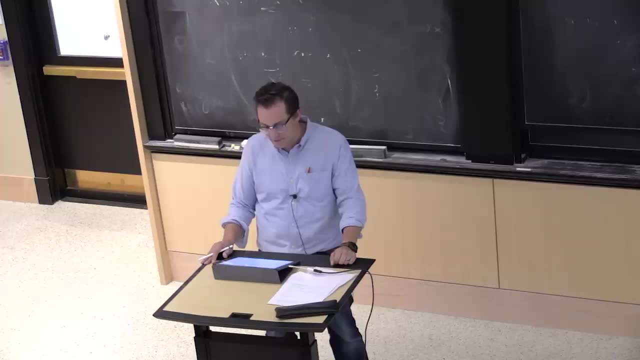 in airports. It should be representative of all couples in the world, And so here let's just keep it vague, But you need to keep in mind what population this is actually making a statement about. So you have this full population of people in the world. 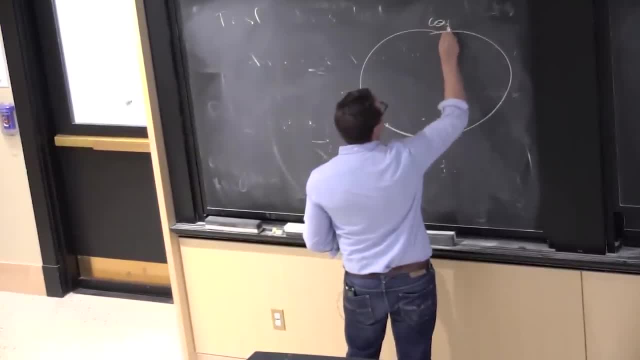 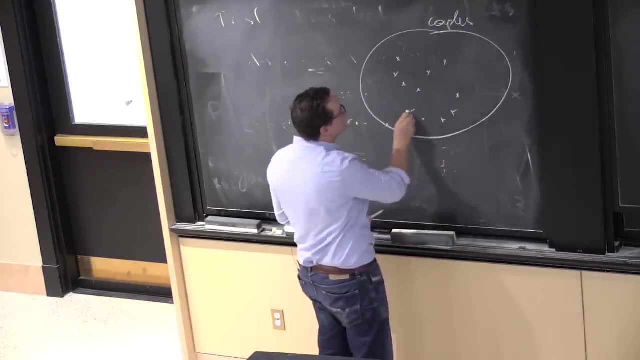 All right. so those are all the couples, And this person went ahead and collected data about a bunch of them And we know that in this thing there's basically a proportion of them that's like p, And that's the proportion of them. 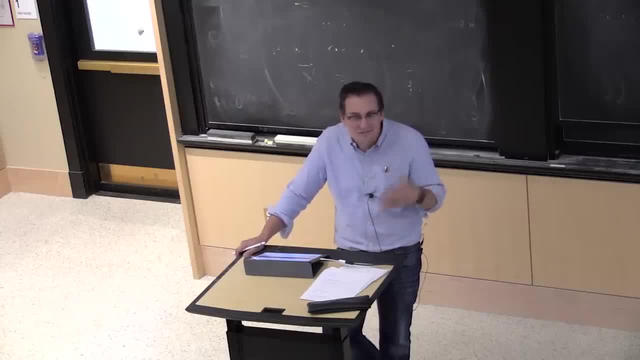 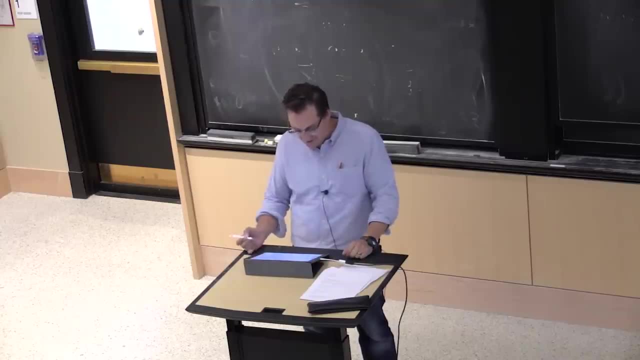 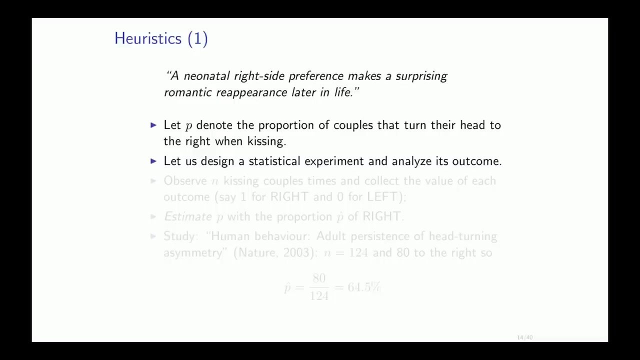 And it's because those people were directed to do it. They just don't actually think about doing it. OK, And also because I think you need to justify writing a nature paper more than I said on front of my computer. So again, this first sentence here. 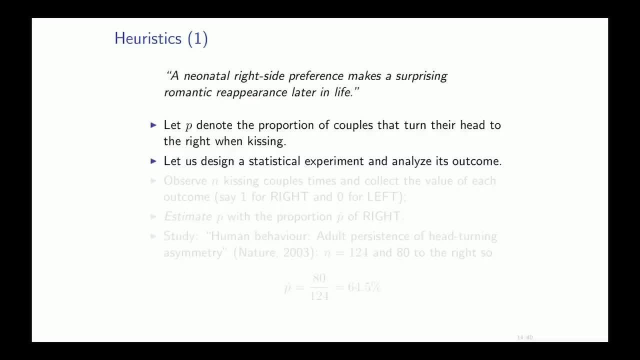 a neonatal right-side preference is there? a right-side preference is not a mathematical question, But we can start saying: let blah and put some variables and ask questions about those variables. So x is actually not a variable that's used very much. 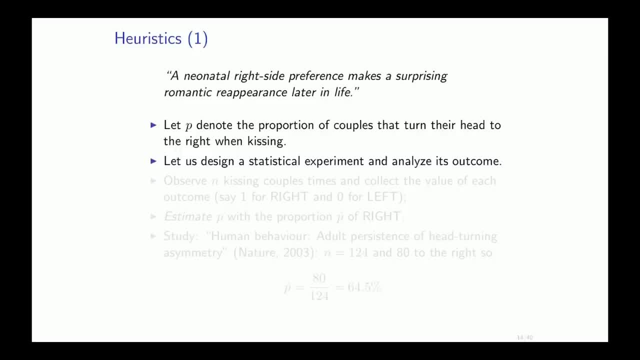 OK, In statistics for parameters, But p is one for parameter And so you're going to take your parameter of interest, p, And here is going to be the proportion of couples And that's among all couples. So here, if you talk about statistical thinking, 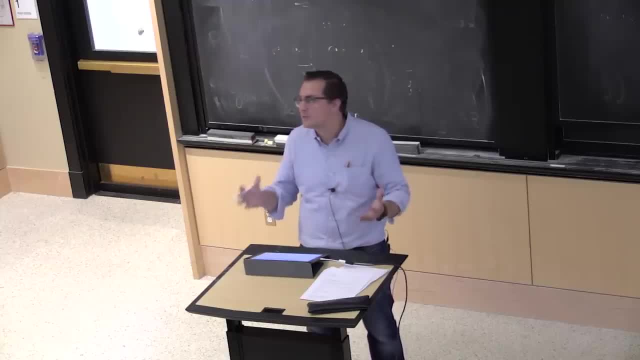 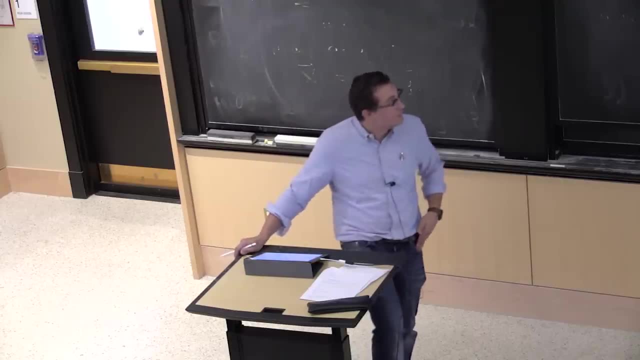 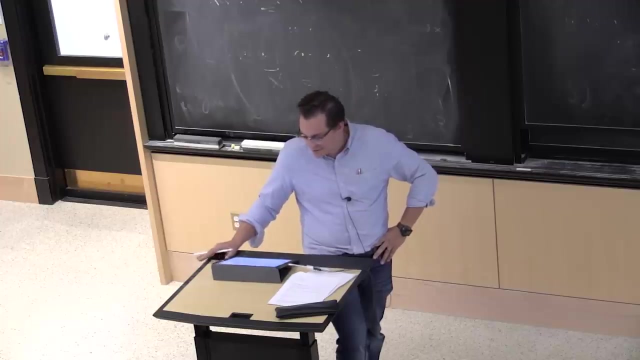 there would be a question about what population this would actually be representative of. So usually this is a call to your. sorry, I should not forget this word. It's important for you. OK, I forget this word, So this is OK. 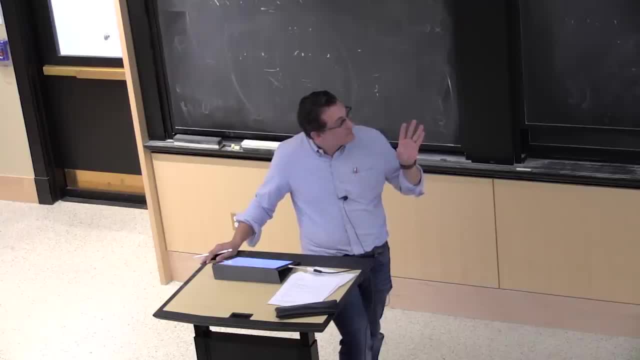 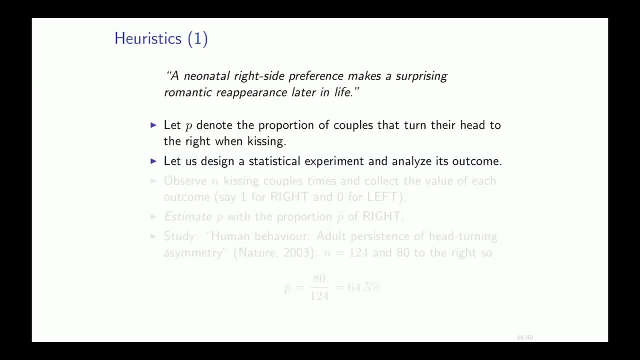 So, if you look at this proportion, maybe these couples that are in the study might be representative only of couples in airports. Maybe they actually put on a show for the other passengers, Who knows? Oh, let's just do this well, And just like the people on Google Images. 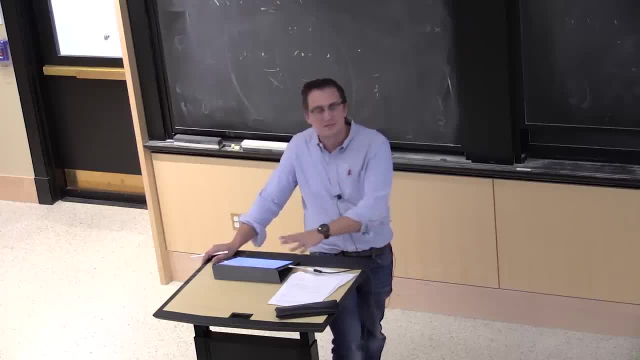 are actually doing it, So maybe you want to just restrict it. But of course, clearly, if it's appearing in nature, it should not be only about couples, OK, So if you look at the number of couples in airports, it's supposedly representative of all couples in the world. 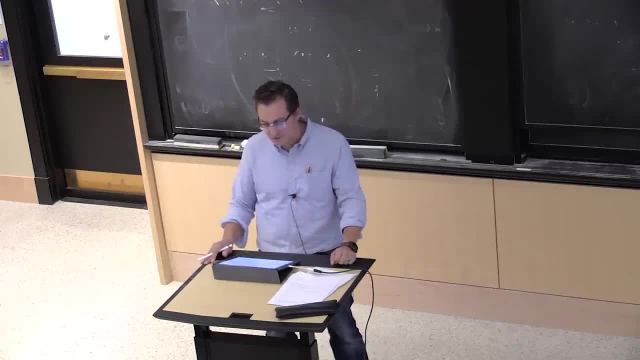 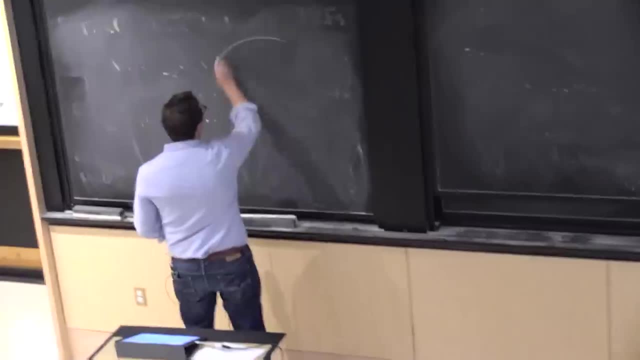 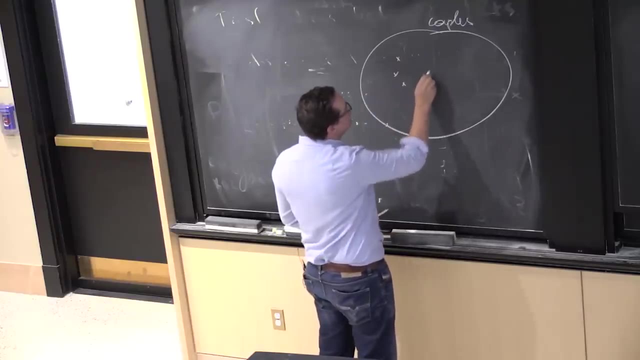 And so here let's just keep it vague, But you need to keep in mind what population this is actually making a statement about. So you have this full population of people in the world. So those are all the couples, And this person went ahead and collected data. 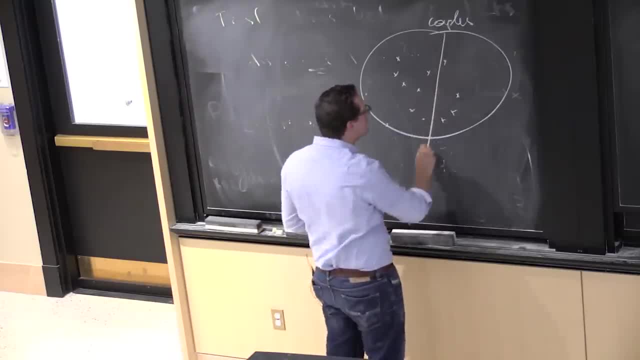 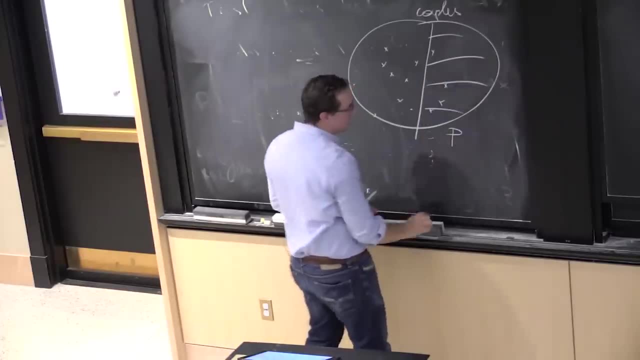 about a bunch of them. OK, And we know that in this thing there's basically a proportion of t And that's the proportion of them that's bending their head to the right. So everybody on this side is bending their head to the right. 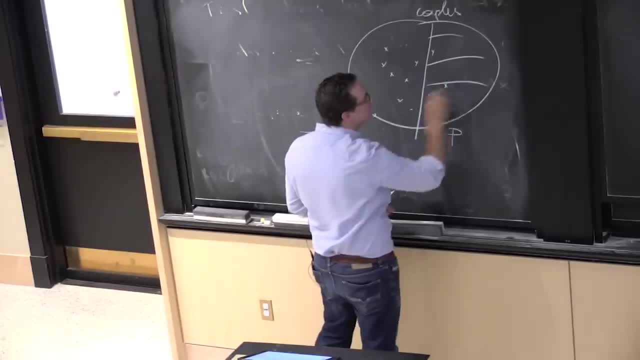 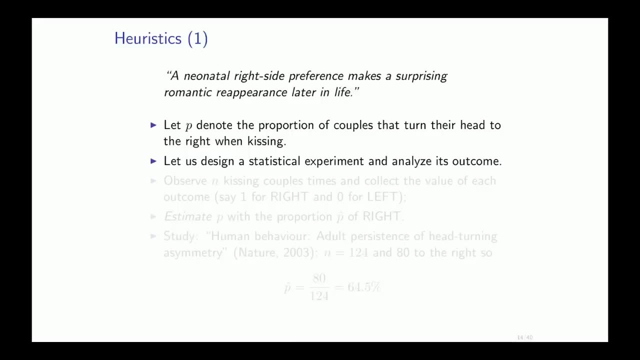 That's bending their head to the right, And this is so. everybody on this side is bending their head to the right, And hopefully we can actually sample this thing uniformly. That's basically the process that's going on. So this is the statistical experiment. 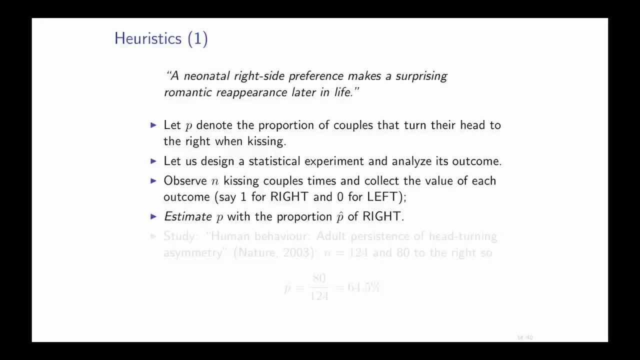 We're going to observe n kissing couples, right? So here we're going to put as many variables as we can, so we don't have to stick with numbers, And then we'll just plug in the numbers: n kissing couples. And n is also in statistics, by the way. 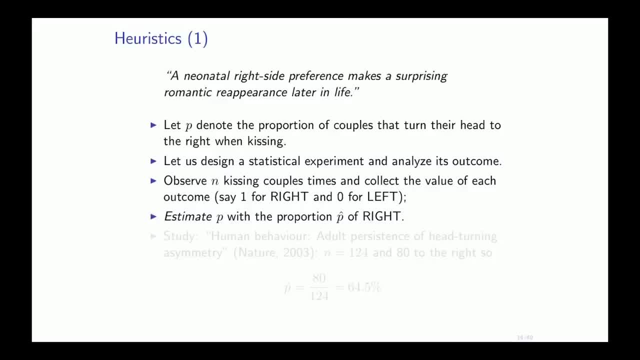 n is the size of your sample. 99.9% of the time, And collectively, we're going to put as many variables as we can, So we don't have to stick with numbers And then we'll just plug in the numbers. 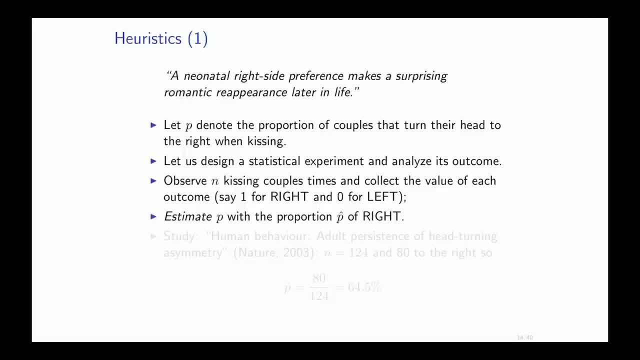 And then we'll just plug in the value of each outcome. OK, So we want numbers. We don't want right or left, So we're going to code them by 0 or 1, pretty naturally, And then we're going to estimate p, which is a known right. 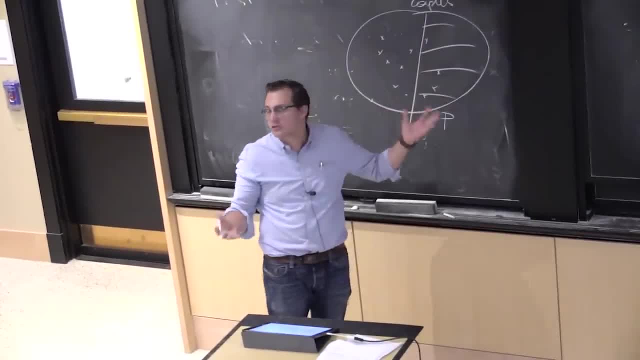 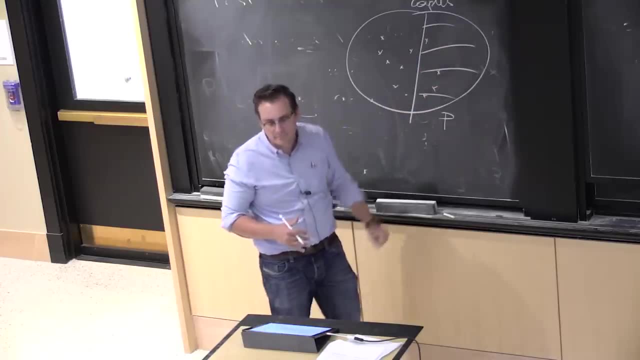 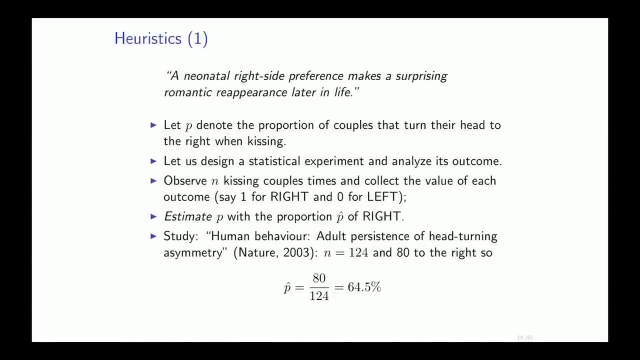 So p is this area, And we're going to estimate it simply by the proportion of right right, So the proportion of crosses that actually fell in the right side. OK, So in this study, what you will find is that The numbers that were collected were 124 couples. 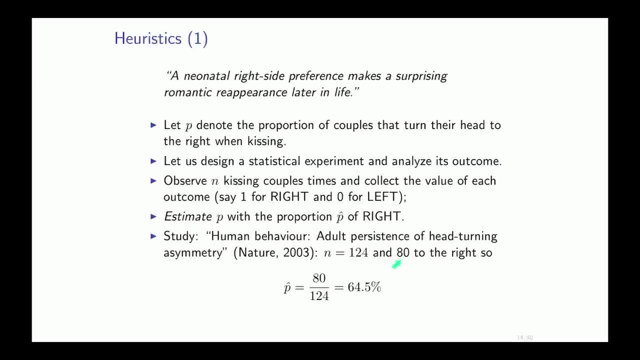 And that out of those 124, 80 of them turned their head to the right. OK, So p? hat is a proportion. How do we do it? Well, don't need statistics for that. You're going to take 80 divided by 124. 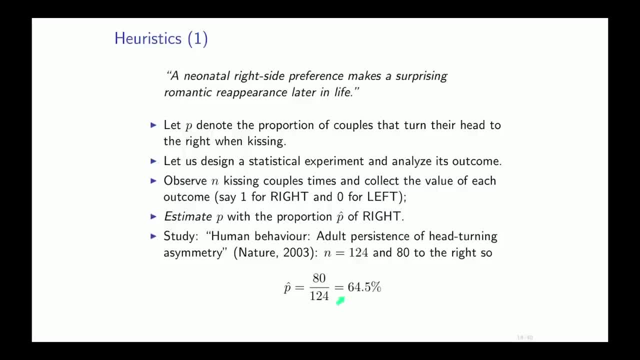 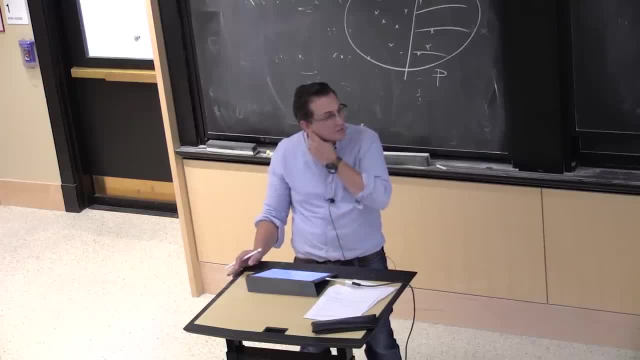 And you will find that in this particular study, 64.5% of the couples were bending their head to the right. That's a pretty large number, right? The question is, If I picked another 124 couples, maybe at different airports, different times- would? 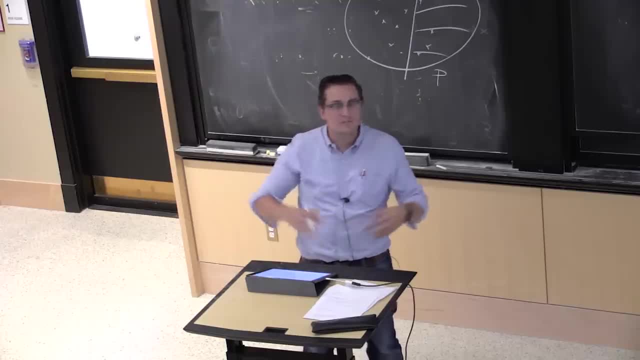 I see the same number. Would this number be all over the place? Would it be sometimes very close to 120, or sometimes very close to 10?? Or would it be? is this number actually fluctuating? a lot, right, And so hopefully not too much right. 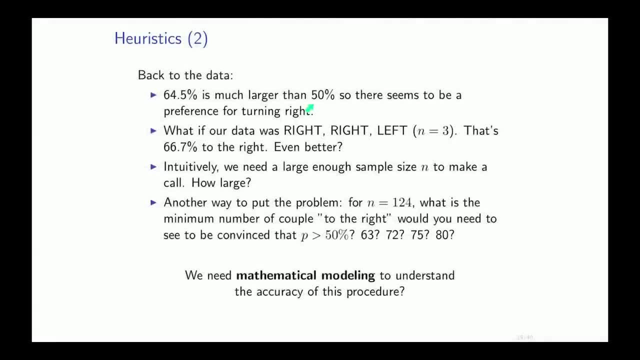 So 64.5% is definitely much larger than 50%, And so there seems to be this preference. OK, And now we're going to have to quantify how much of this preference. Is this number significantly larger than 50%? OK, 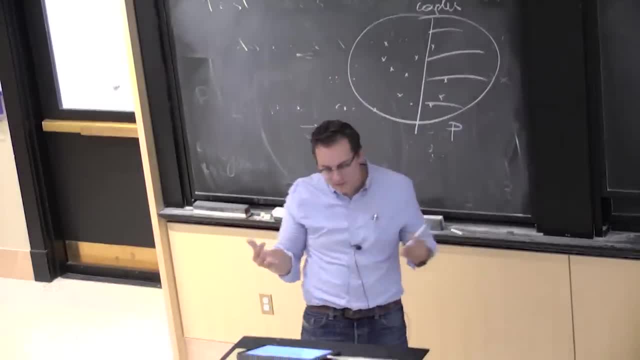 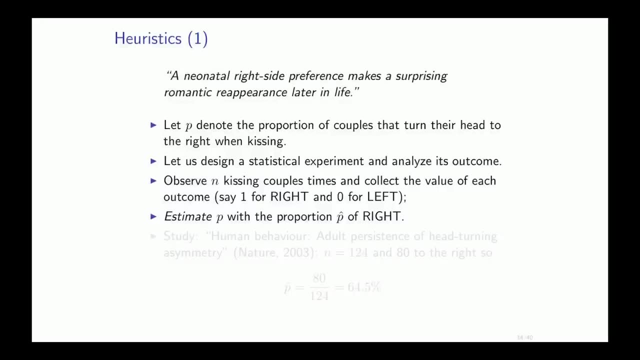 And hopefully we can actually sample this thing uniformly. That's basically the process that's going on. So this is the statistical experiment. We're going to observe n kissing couples. So here we're going to put as many variables as we can. 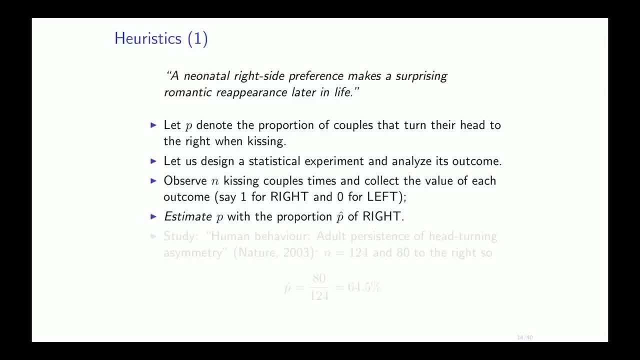 So we don't have to stick with numbers And then we'll just plug in the numbers. n kissing couples, And n is also in statistics, by the way. n is the size of your sample, 99.9% of the time. 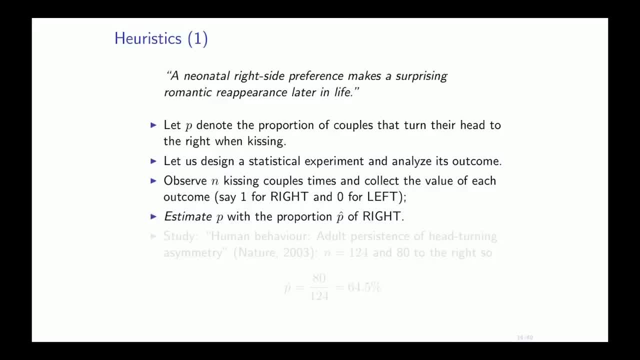 And collect the value of each outcome. OK, So we want numbers, We don't want right or left, So we're going to code them by 0 or 1, pretty naturally, And then we're going to estimate p, which is unknown. 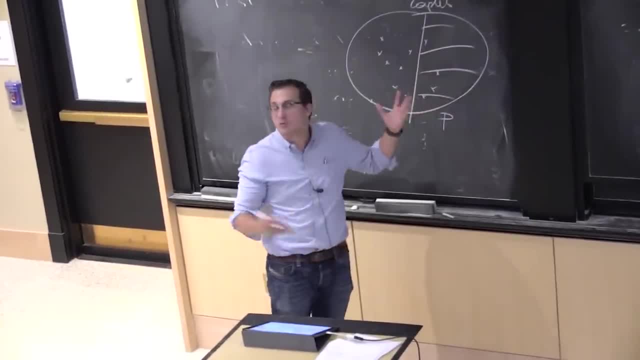 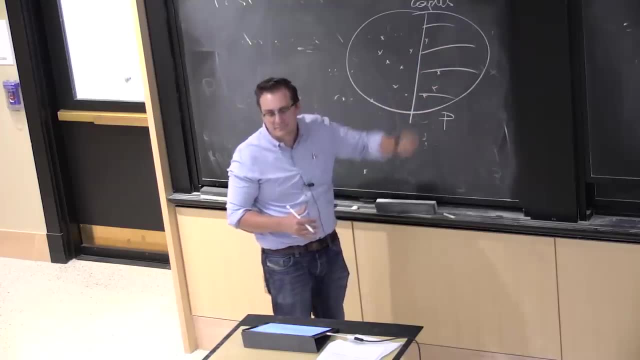 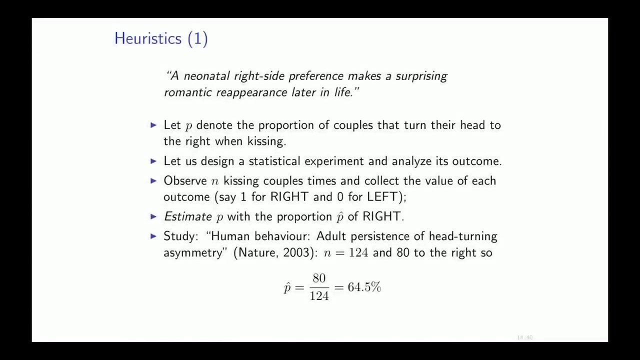 Right. So p is this area, And we're going to estimate it simply by the proportion of right Right, So the proportion of crosses that actually fell in the right side. OK, so in this study, what you will find is that the numbers that were collected were 124 couples. 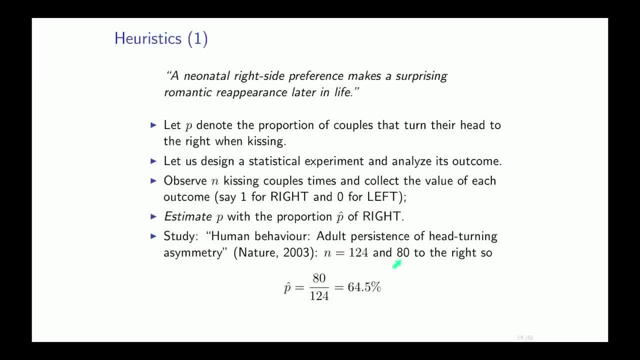 And that out of those 124, 80 of them turned their head to the right. OK, So p? hat is a proportion. How do we do it? Well, don't need statistics for that. You're going to take 80 divided by 124. 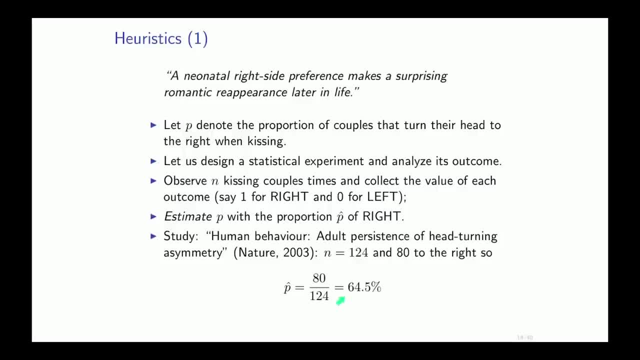 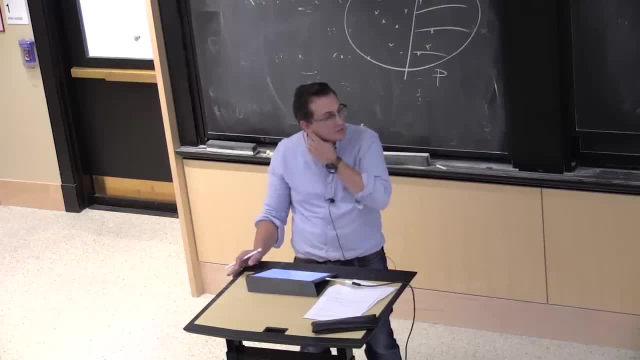 And you will find that in this particular study, 64.5% of the couples were bending their head to the right. That's a pretty large number, Right? The question is, if I picked another 124 couples, maybe at different airports, different times? 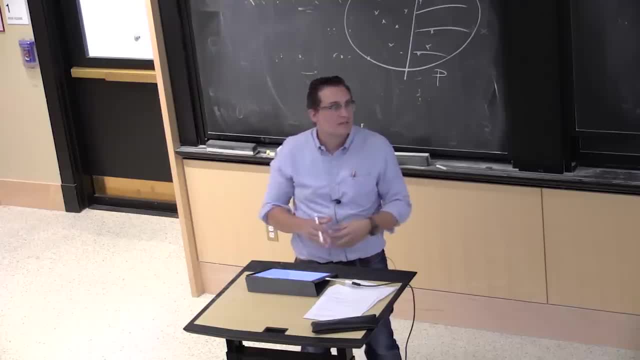 would I see the same number? Would this number be all over the place? Would it be sometimes very close to 120, or sometimes very close to 10?? Or would it be? is this number actually fluctuating a lot, Right, And so hopefully not too much? 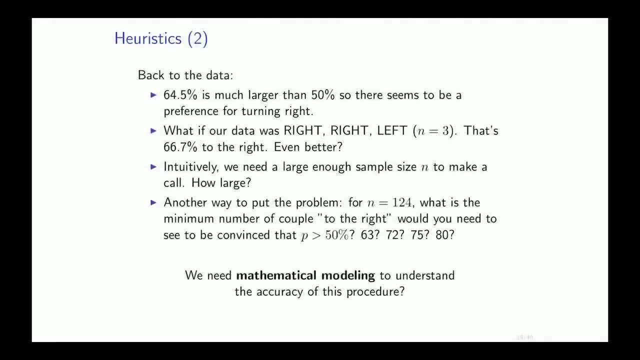 Right, So 64.5% is definitely much larger than 50%, And so there seems to be this preference. OK, and now we're going to have to quantify How much of this preference. Is this number significantly larger than 50%? 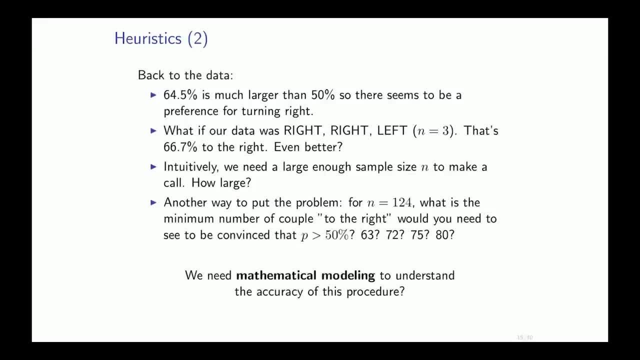 OK. so if our data, for example, was just three couples, OK, I'm just going there, I'm going to Logan, I call it, I do right, left, right, And then I see what's the name of the fish place there. 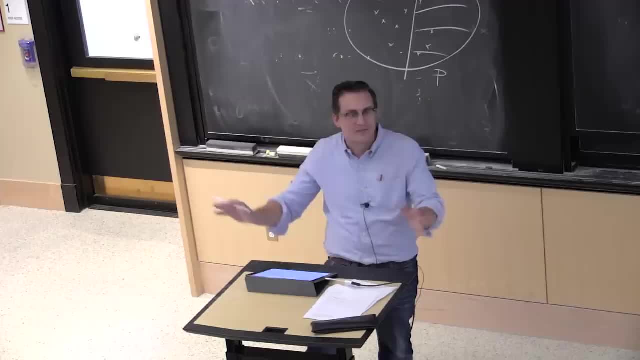 I go to Wahlburgers at Logan And I'm like: OK, I'm done for the day. I collect this data. I go home and I'm like: well, 66.7% to the right, That's a pretty big number. 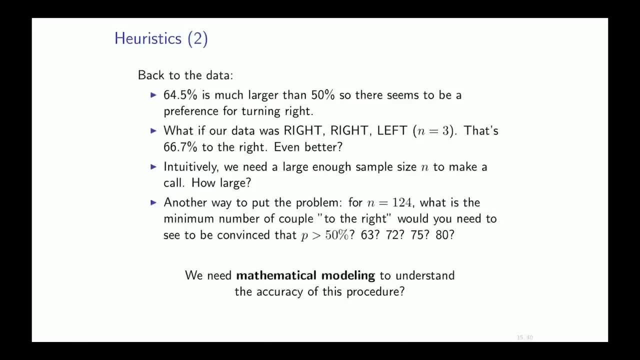 It's even farther from 50% than this other guy, So I'm doing even better, But of course you know that this is not true. right? Three people is definitely not representative. If I stopped at the first two, I would have even 100%. 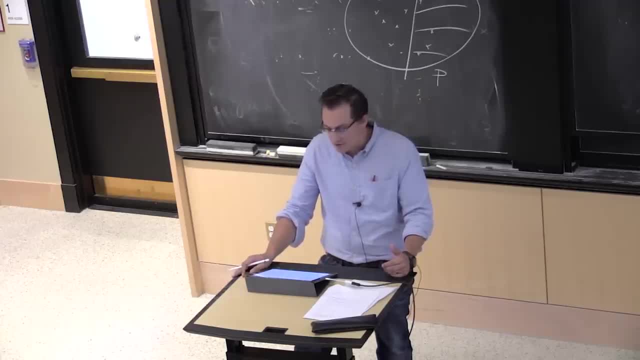 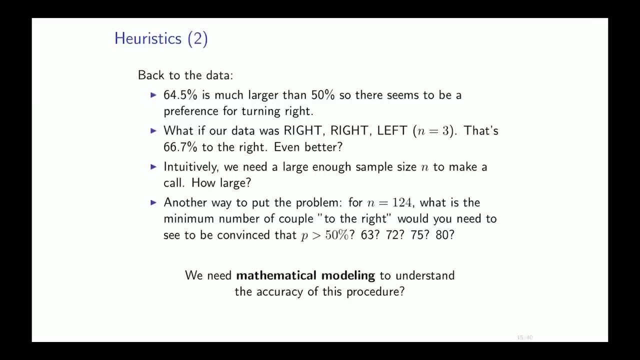 So the question that statistics is going to help us answer is: how large should the sample be? For some reason- I don't know if you guys received it- I'm an affiliate with the Broad Institute And since then I receive one email per day that says: 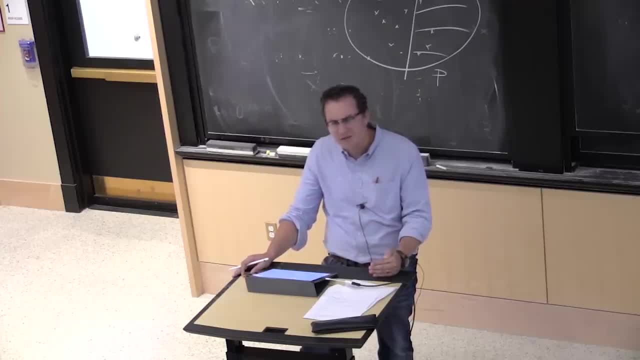 sample size determination. How large should your sample be? I know how large should my sample be. I've taken 18650 multiple times And so I know. But the question is: is 124 a large enough number or not? Well, the answer is actually, as usual: it depends. 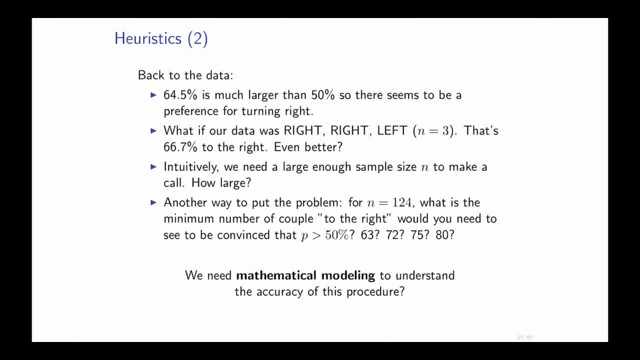 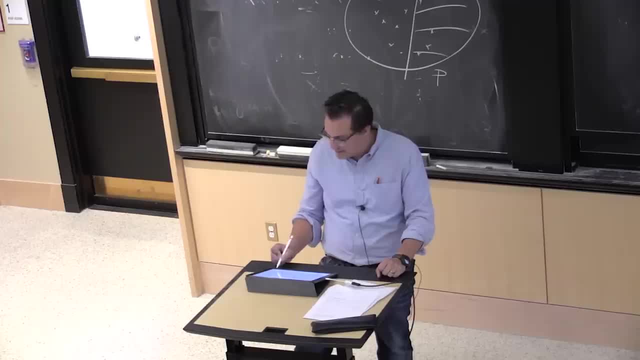 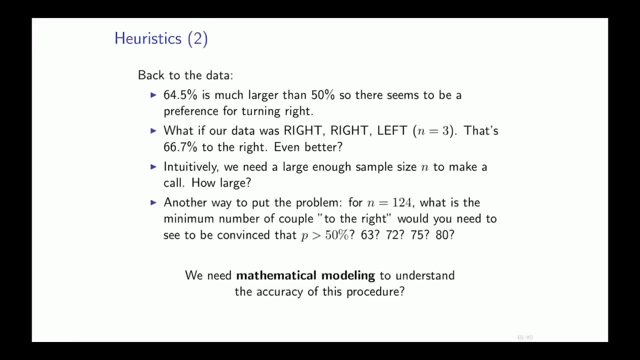 It will depend on the true unknown value of p, But from those particular values that we got. so 120, and how many couples was there? 80, we actually can make some question Right. So here we said that 80 was allowing us to conclude at 64.5%. 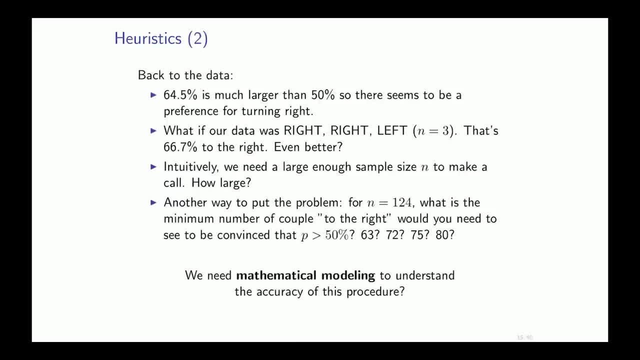 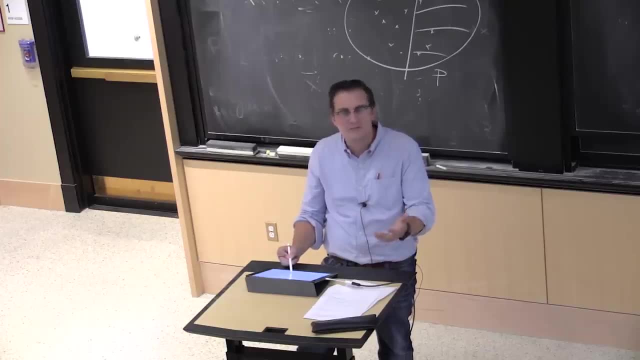 So it could be one reason to say that it was larger than 50%. 50% of 124 is 62. So the question is, would I be willing to make this conclusion at 63?? Is that a number that would convince you? 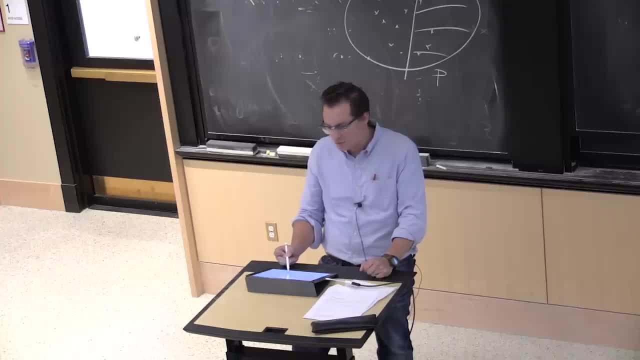 Who would be convinced 63.. Who would be convinced by 72?? Who would be convinced by 75?? Hopefully, the number of hands that are raised should grow. Who would be convinced by 80?? All right, So basically those numbers, actually. 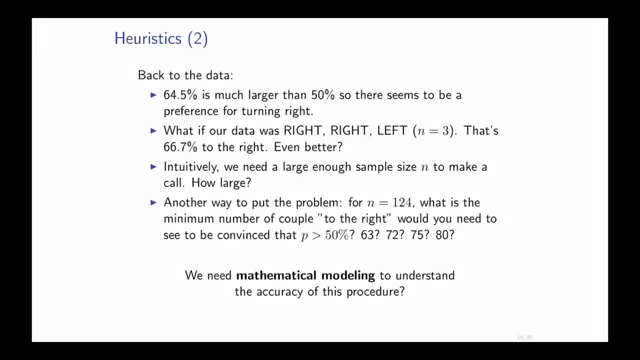 So if our data, for example, was just three couples, OK, I'm just going there, I'm going to Logan, I call it, I do right, left, right, And then I see what's the name of the fish place there. 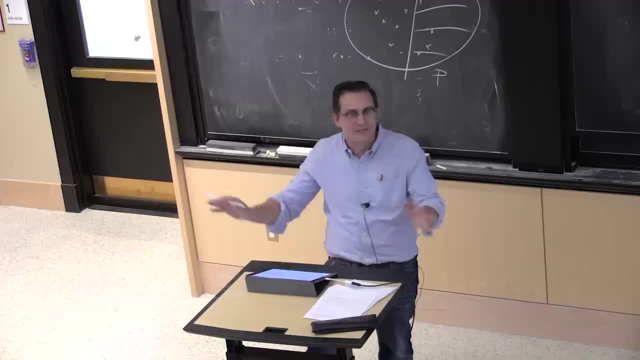 I go to Wahlburgers at Logan And I'm like, OK, I'm done for the day. I collect this data. I go home And I'm like, wow, 66.7% to the right, That's a pretty big number. 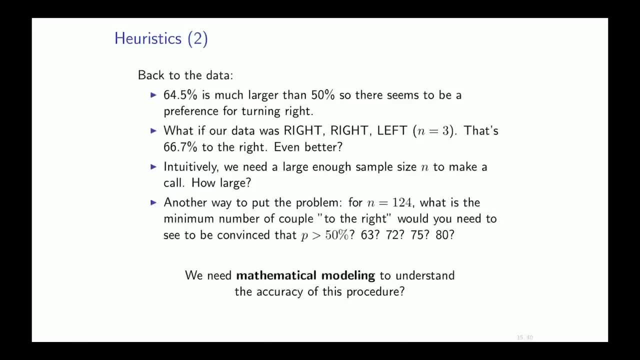 It's even farther from 50% than this other guy, So I'm doing even better, But of course you know that this is not true. right? Three people is definitely not representative. If I stopped at the first two, I would have even 100%. 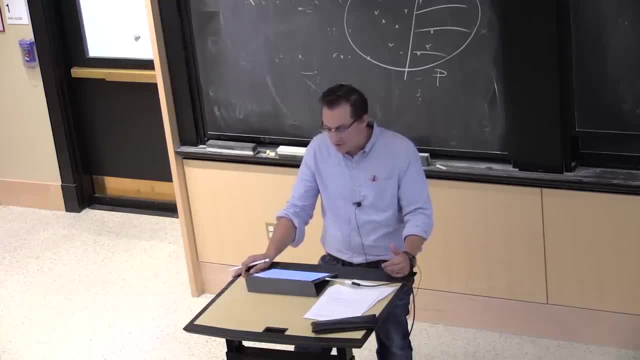 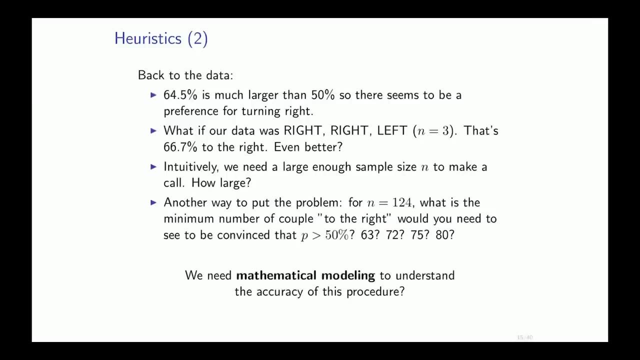 So the question that statistics is going to help us answer is: how large should the sample be? For some reason- I don't know if you guys received it- I'm an affiliate with the Broad Institute And since then I receive one email per day that says: 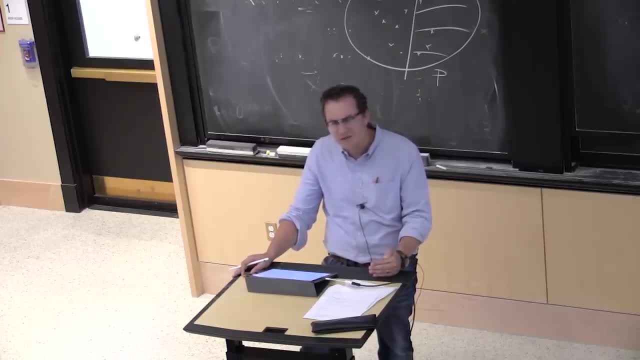 sample size determination. how large should you sample be? I'm like I know how large should my sample be. I've taken 18650 multiple times And so I know. But the question is, is 124 a large enough number or not? 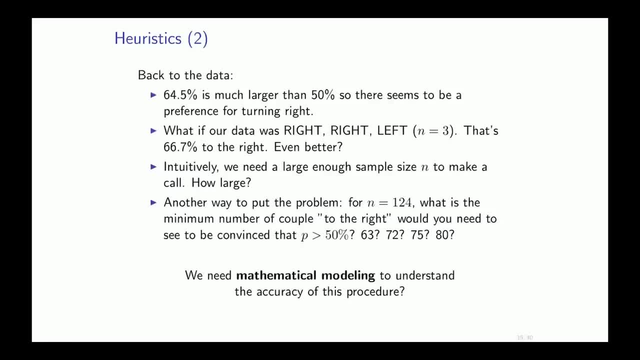 Well, the answer is actually, as usual, it depends. It will depend on the true unknown value of p, But from those particular values that we got. so 120, and how many couples was there? 80, we actually can make some question, right. 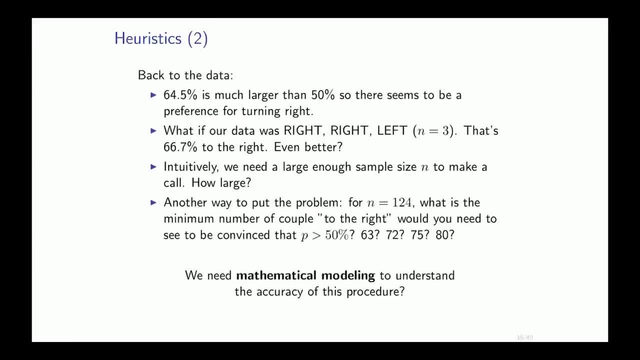 So here. So here we said that 80 was allowing us to conclude at 64.5%, So it could be one reason to say that it was larger than 50%. 50% of 124 is 62. So the question is, would I be willing to make? 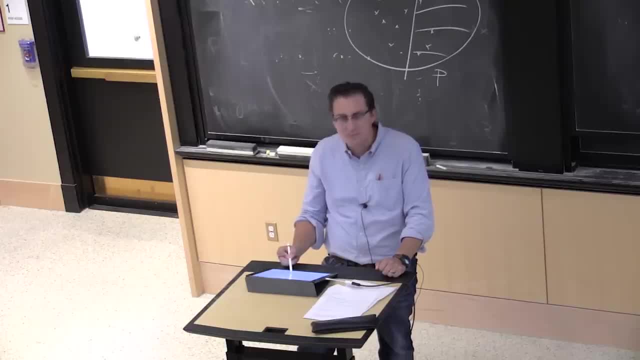 this conclusion at 63?. Is that a number that would convince you? Who would be convinced by 63?? Who would be convinced by 72?? Who would be convinced by 75?? Hopefully, the number of hands that are raised should grow. 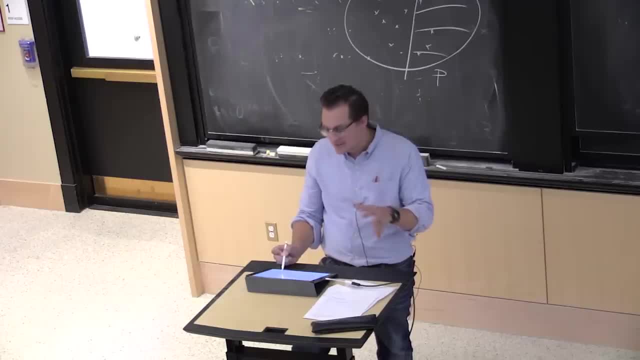 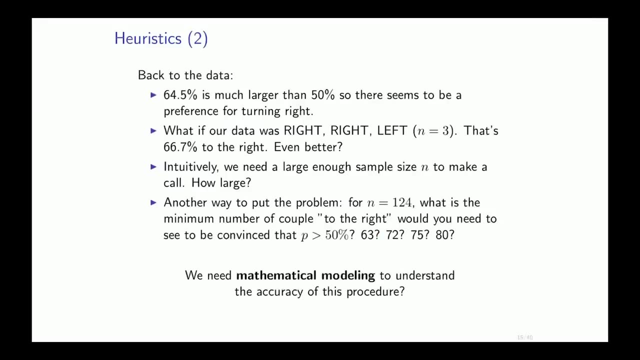 Who would be convinced by 80?? All right, So basically those numbers actually don't come from anywhere. This 72, would be the number that you would need for a study. Most statistical studies would be the number that they would retain. 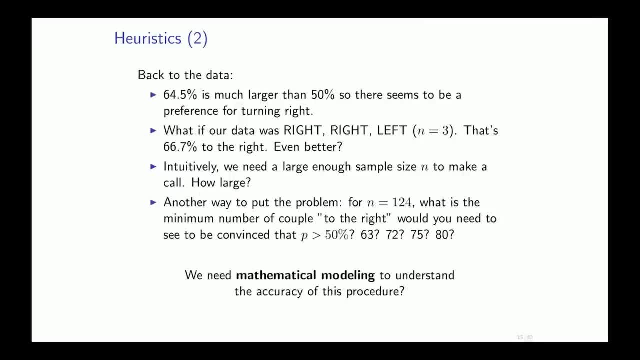 For 124,, you would need to see 72.5%, So this is the number that you would need to make this conclusion, And then 75,. so we'll see that there's many ways to come to this conclusion Because, as you can see, this was published in Nature with 80. 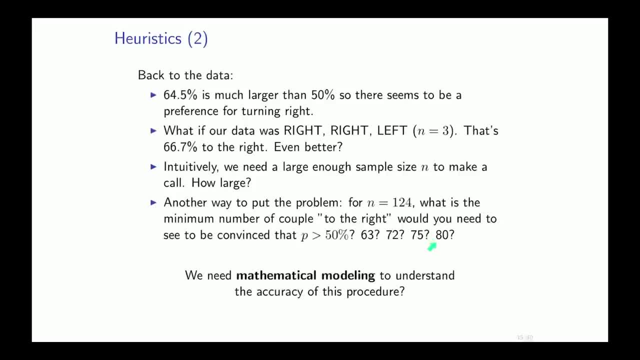 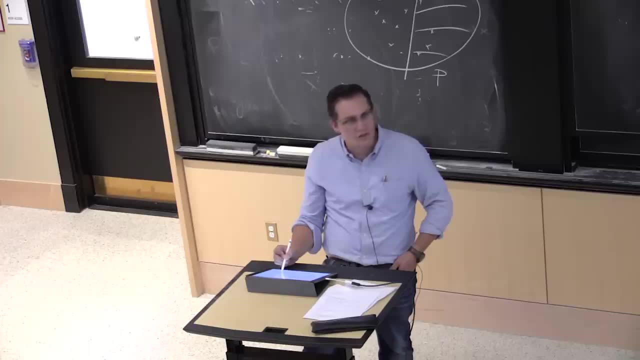 So that was OK. So 80 is actually a very large number. This is 99%. no, So this is 95% confidence, this is 99% confidence and this is 99.9% confidence. All right, So if you said 80, you are a very conservative person. 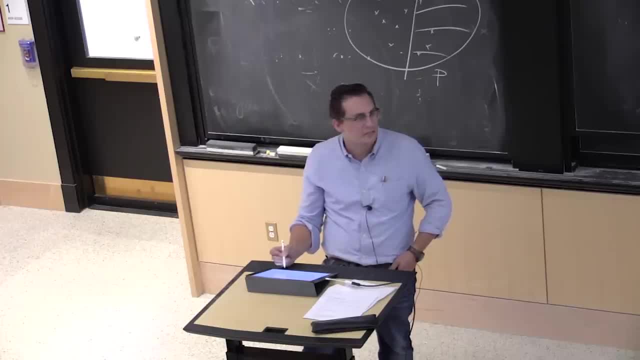 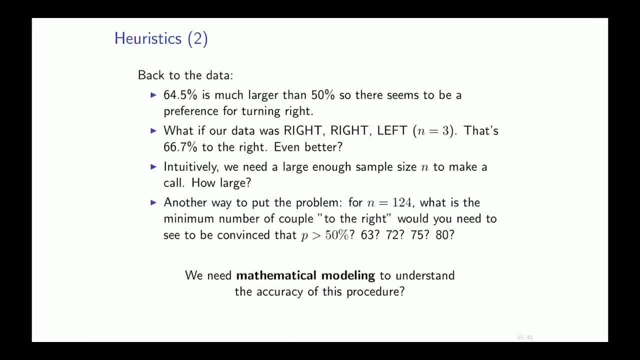 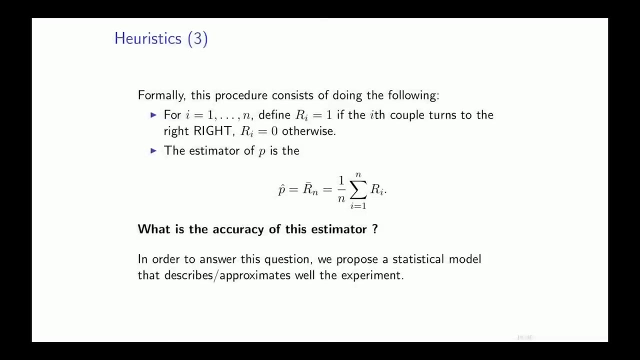 OK, So starting at 72, you can start making this conclusion. So to understand this, we need to do our little mathematical kitchen here and we need to do some modeling. So we need to understand by modeling. we need to understand what random process we think. 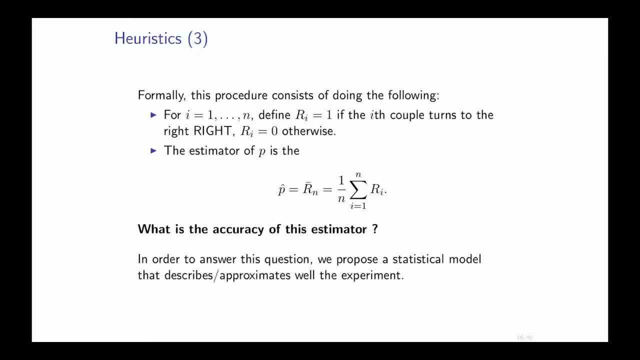 this data is generating from, So it's going to have some unknown parameters, unlike in probability, But we need to have just basically everything written except for the values of the parameters. right, When I said a die is coming uniformly with probability 1,. 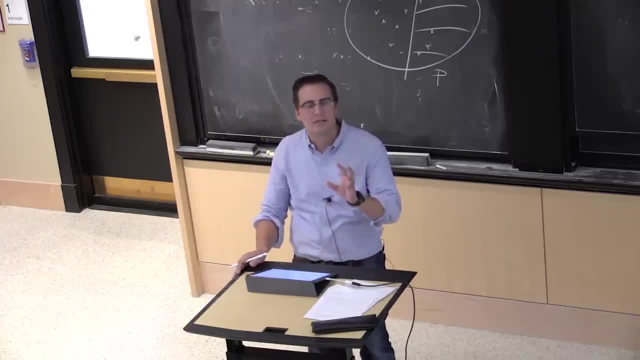 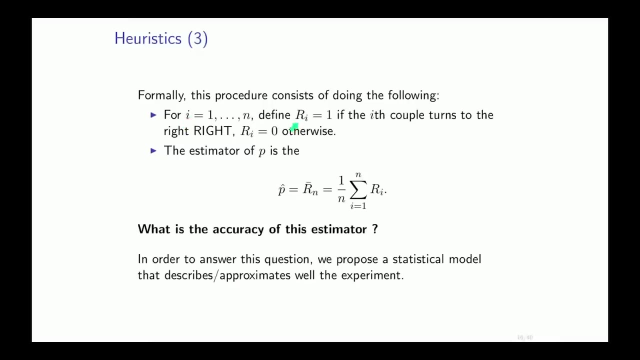 6, then I need to have say, maybe with probability, maybe I should say here are six numbers and I need to just fill those numbers. OK, So for i equal 1 to n. I'm going to define ri to be the indicator. 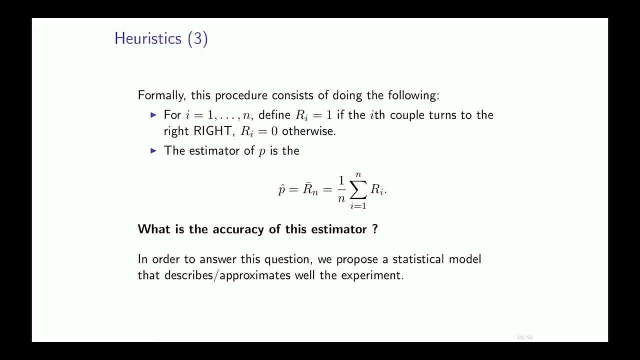 An indicator is just something that takes value: 1 if something is true and 0 if not. So it's an indicator. It's an indicator that i-th couple turns the head to the right. OK, So ri. so it's indexed by i. 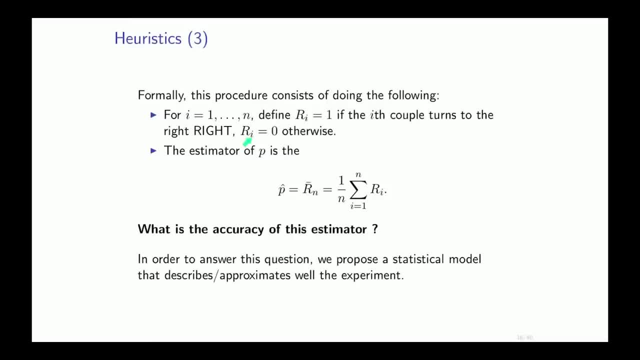 And it's 1 if the i-th couple turns their head to the right and 0 if it's well. actually, I guess they can probably kiss straight right? So that would be weird, but they might be able to do this. 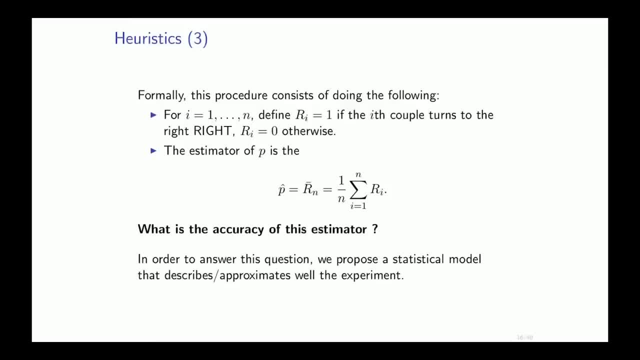 So let's say not right. OK, Then the estimator of p we said was p hat, It was just the ratio of two numbers. But really what it is is I sum those ri's, Since I only add those that take value 1,. what this sum is 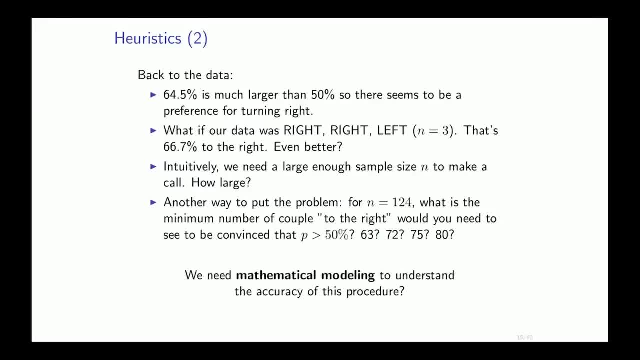 don't come from anywhere. This 72 would be the number that you would need for a study. Most statistical studies would be the number that they would retain For 124.. You would need to see 72 that turn their head right to actually make this conclusion. 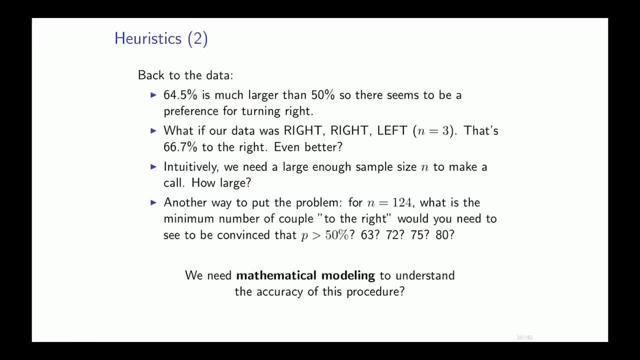 And then 75,. so we'll see that there's many ways to come to this conclusion because, as you can see, this was published in Nature with 80. So that was OK. So 80 is actually a very large number. This is 99% confidence. 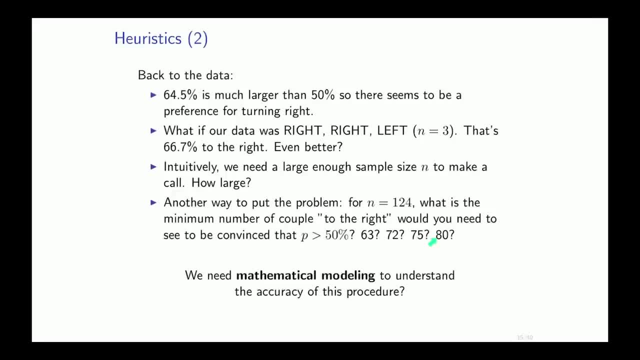 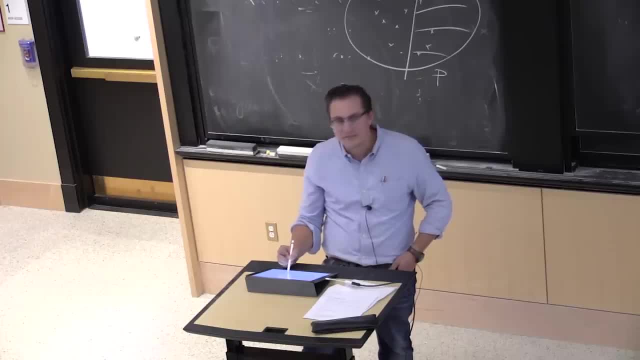 This is 99% confidence And this is 99.9% confidence. All right. so if you said 80,, you are very conservative. All right, You are a conservative person. Starting at 72, you can start making this conclusion. 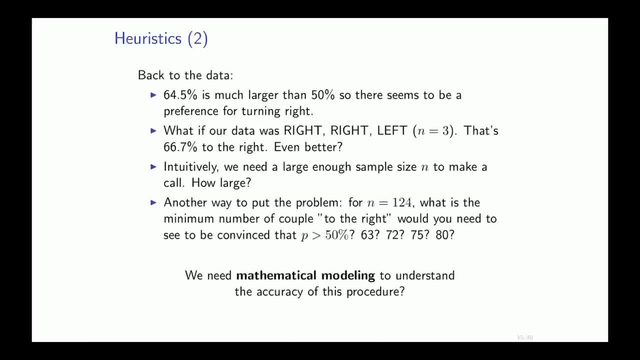 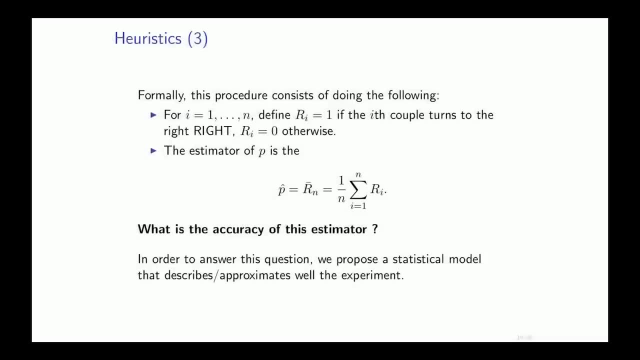 So to understand this, we need to do our little mathematical kitchen here and we need to do some modeling. So we need to understand by modeling, we need to understand what random process we think this data is generating from. So it's going to have some unknown parameters. 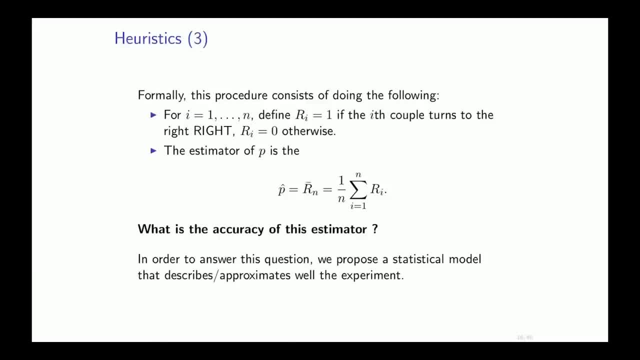 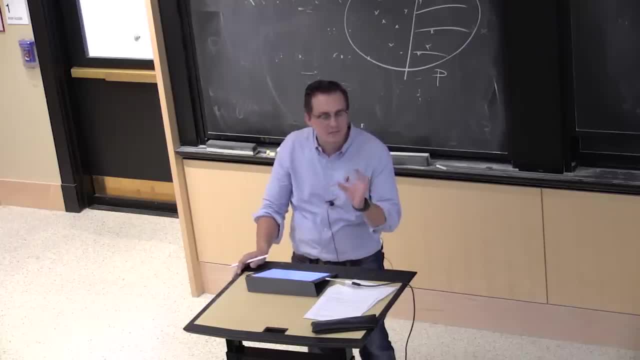 unlike in probability. but we need to have just basically everything written except for the values of the parameters. When I said a die is coming uniformly with probability 1, 6, then I need to have say, maybe with probability. maybe I should say here are six numbers. 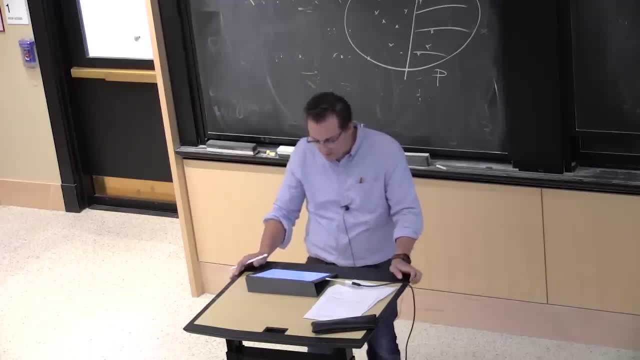 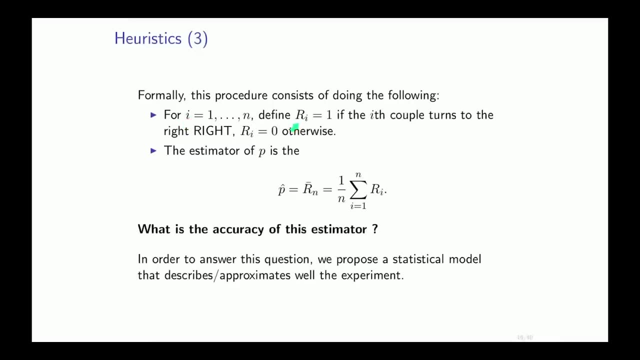 and I need to just fill those numbers. So for i equal 1 to n, I'm going to define ri to be the indicator. An indicator is just something that takes value: 1 if something is true and 0 if not. So it's an indicator that i-th couple turns the head. 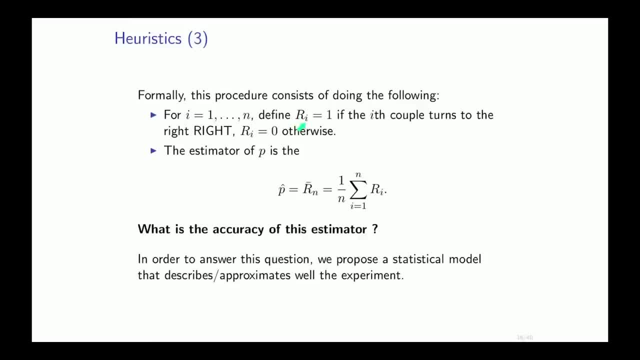 to the right, So ri. so it's indexed by i and it's 1 if the i-th couple turns their head to the right and 0 if it's well. actually, I guess they can probably kiss straight, So that would be weird, but they might be able to do this. 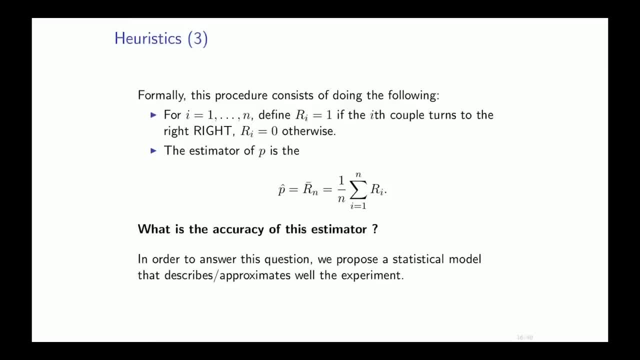 So let's say not right. Then the estimator of p we said was p hat, It was just the ratio of two numbers. But really what it is is, I count, I sum those ri's, Since I only add those that take value 1,. what this sum is. 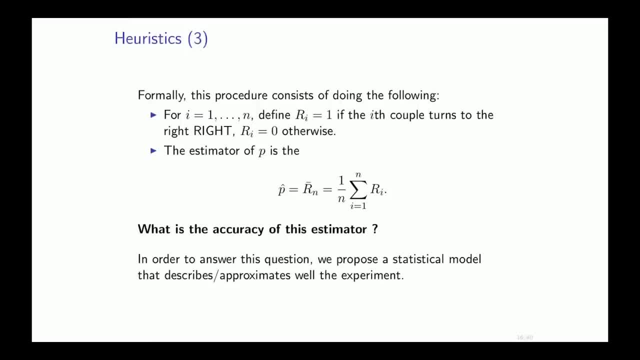 it's really. this sum here is actually just counting the number of 1's, which is another way to say. it's counting the number of couples that are kissing to the right, And here I don't even have to tell you anything about the numbers or anything. 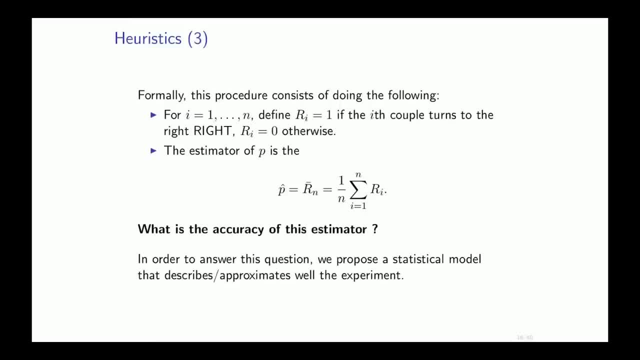 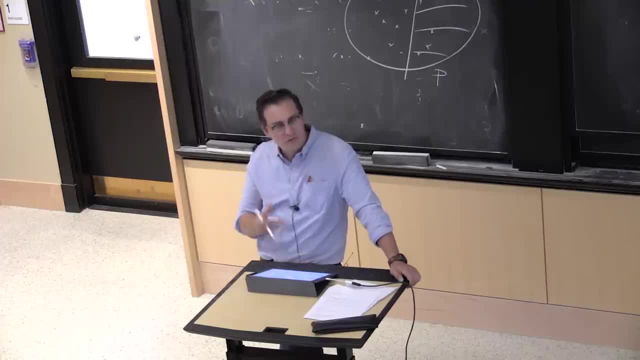 I can only keep track of: first couple is a 0,, second couple is a 1, third couple is a 0.. The data set you can actually find online is actually a sequence of 0's and 1's. Now clearly for the question we're asking. 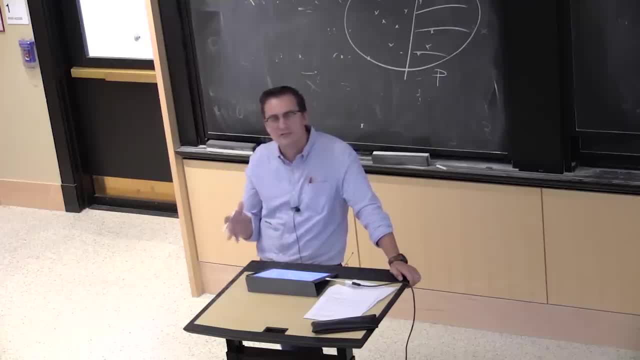 about this proportion. I don't need to keep track of all this information. All I need to keep track of is the number of 0's and the number of 1's. Those are completely interchangeable. I'm not, there's no matter. 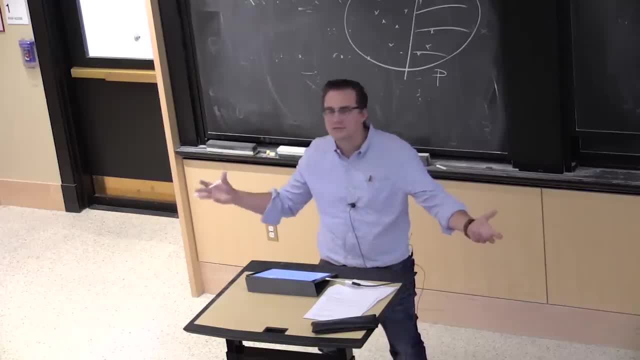 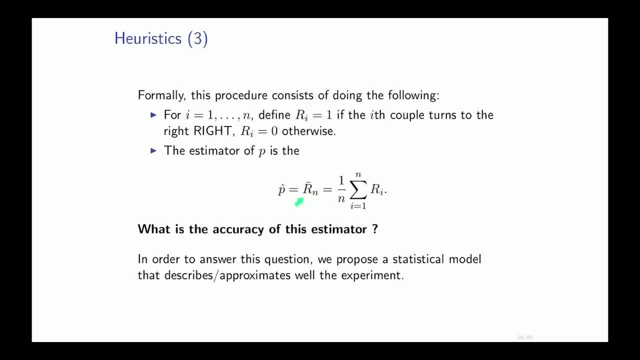 There's no time effect in this. There's no. the first couple is no different than the 15th couple. OK, so we call this Rn bar and that's going to be a very standard notation that we use. R might be replaced by other letters, like x. 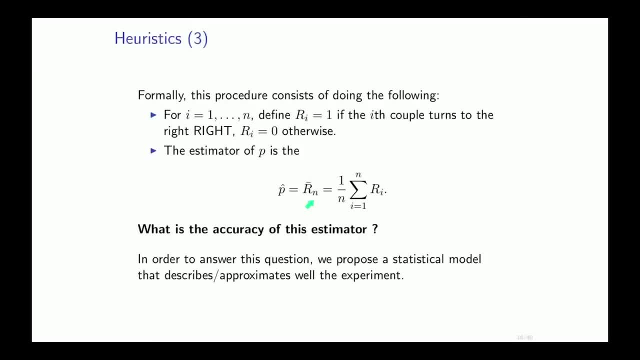 So xn bar yn bar, And this thing essentially means that I average the R or the Ri's over n of them, and the bar means the average. So I divide by n the total number of 1's. So here this sum was equal to 80 in our example. 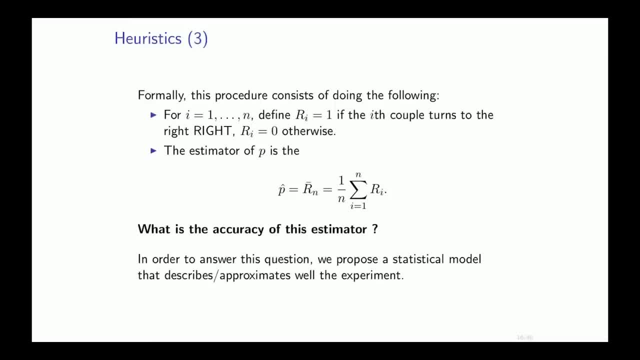 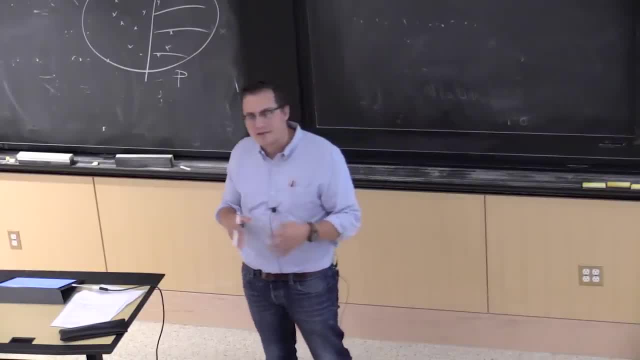 and n was equal to 124.. Now, this is an estimator, So an estimator is different from an estimate. An estimate is a number. My estimate was 64.5.. My estimator is this thing where I keep all the variables free. 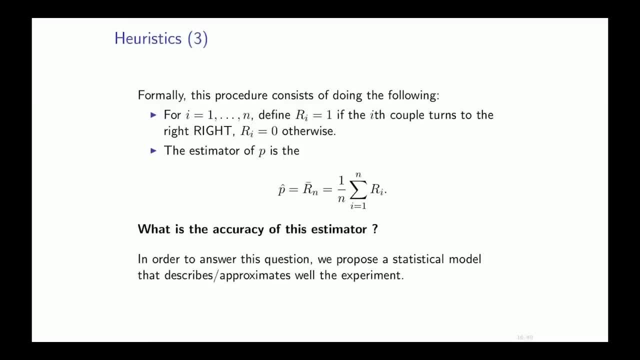 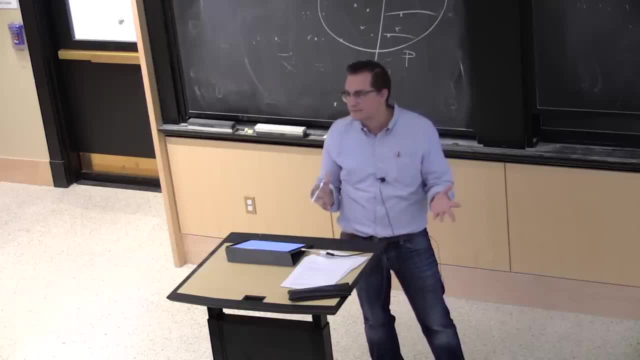 And, in particular, I keep those variables to be random, because I'm going to think of a random couple kissing left or right as the outcome of a random process, just like flipping a coin beginning heads or tails, And so this thing here is a random variable, Ri. 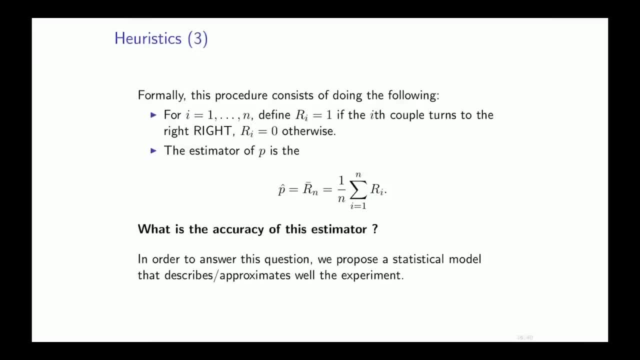 And this average is, of course, an average of random variables. It's itself a random variable, So an estimator is a random variable. An estimate is the realization of a random variable, or, in other words, is the value that you get for this random variable once you plug in the numbers. 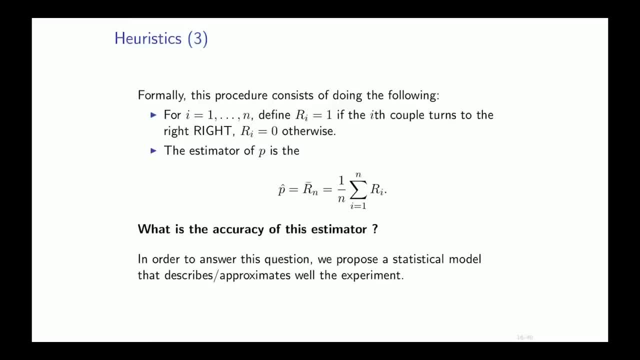 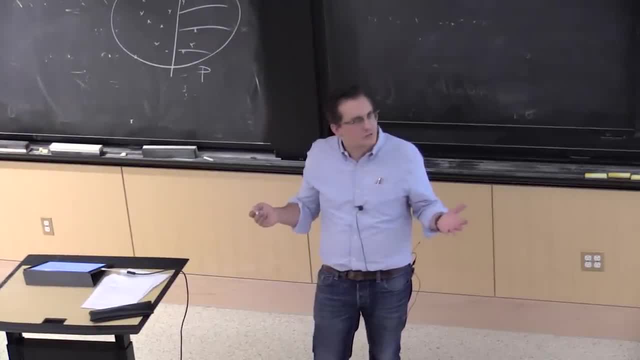 that you've collected, So I can talk about the accuracy of an estimator. Accuracy means what? Well, what would we want for an estimator? Maybe we don't want it to fluctuate too much. right, It's a random variable. So I'm talking about the accuracy of a random variable. 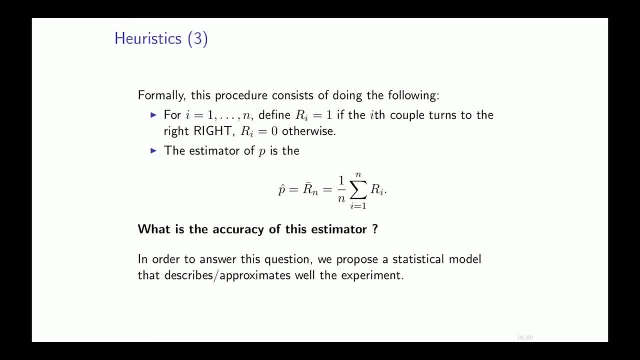 it's really. this sum here is actually just counting the number of 1's, which is another way to say. it's counting the number of couples that are kissing to the right, And here I don't even have to tell you anything about the numbers or anything. 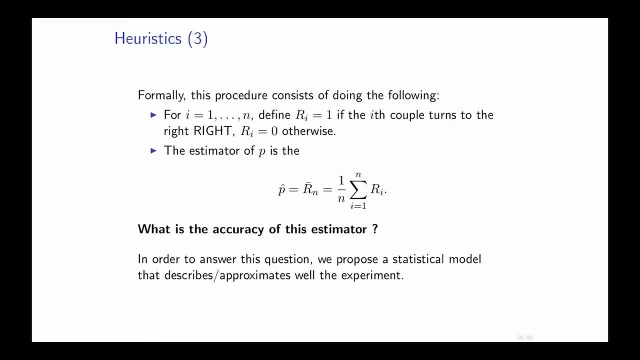 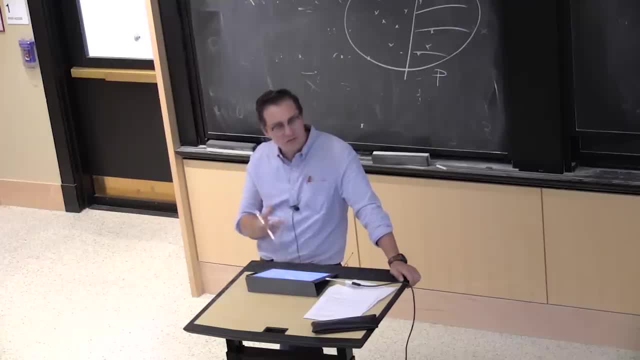 I can only keep track of. first couple is a 0,. second couple is a 1, third couple is a 0. The data set you can actually find online is actually a sequence of 0's and 1's. Now clearly for the question. 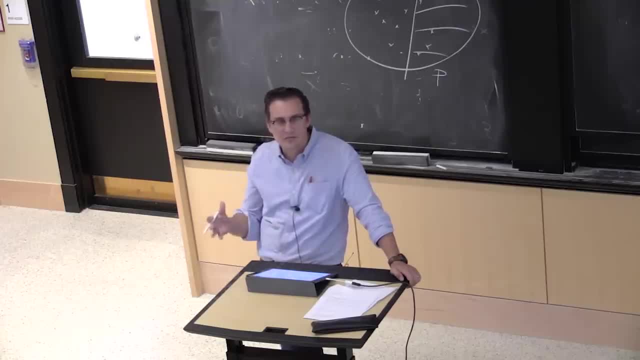 we're asking about this proportion. I don't need to keep track of all this information. All I need to keep track of is the number of 0's and the number of 1's. Those are completely interchangeable. There's no matter. 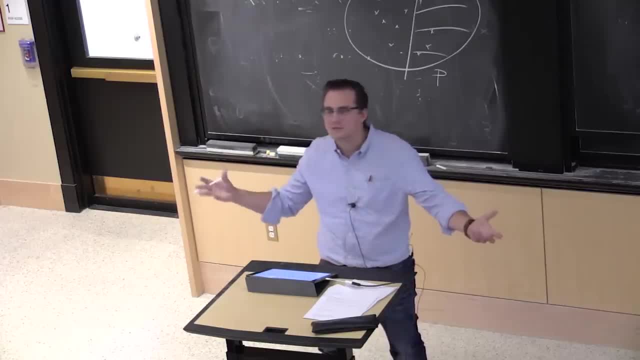 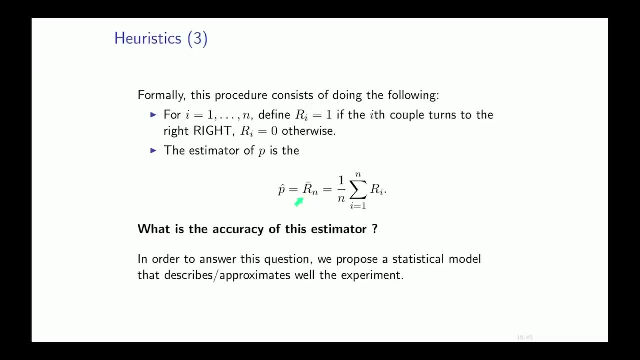 There's no time effect in this. The first couple is no different than the 15th couple, So we call this Rn bar, And that's going to be a very standard notation that we use. R might be replaced by other letters, like x. 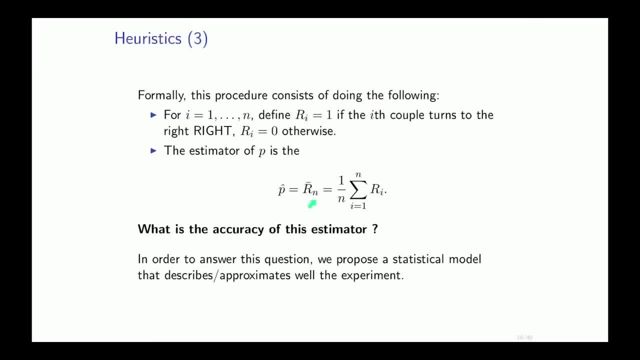 So xn bar yn bar, And this thing essentially means that I average the R's or the Ri's over n of them, And the bar means the average. So I divide by n the total number of 1's. So here this sum was equal to 80 in our example. 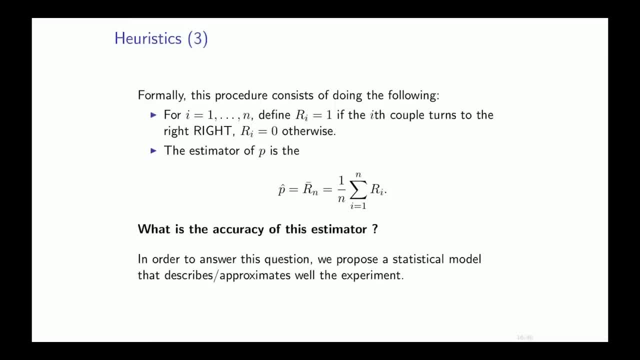 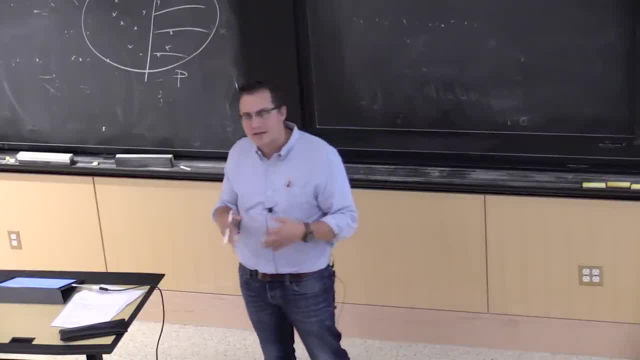 And n was equal to 124.. Now, this is an estimator, So an estimator is different from an estimate. An estimate is a number. My estimate was 64.5.. My estimator is this thing where I keep all the variables free. 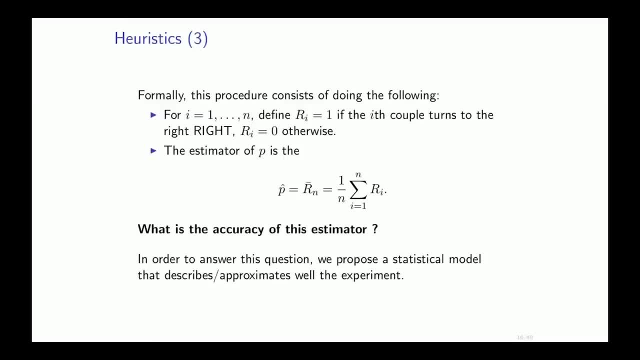 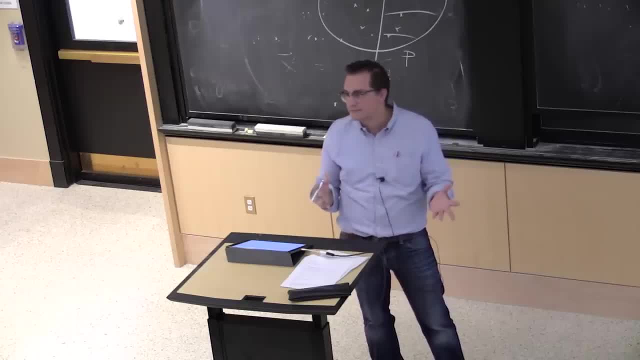 And, in particular, I keep those variables because I'm going to think of a random couple kissing left or right as the outcome of a random process, just like flipping a coin beginning heads or tails, And so this thing here is a random variable, Ri. 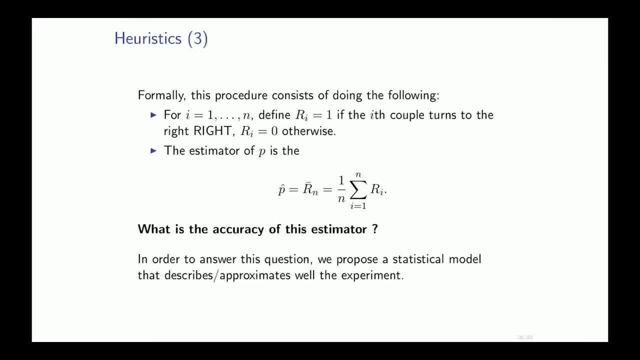 And this average is, of course, an average of random variables. It's itself a random variable, So an estimator is a random variable. An estimate is the realization of a random variable, or, in other words, is the value that you get for this random variable once you plug in the numbers. 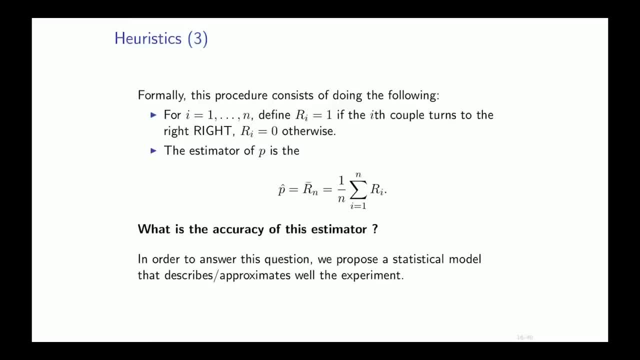 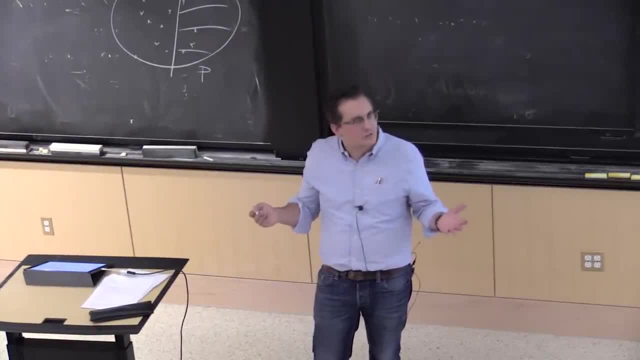 that you've collected, So I can talk about the accuracy of an estimator. Accuracy means what? Well, what would we want for an estimator? Maybe we don't want it to fluctuate too much. It's a random variable, So I'm talking about the accuracy of a random variable. 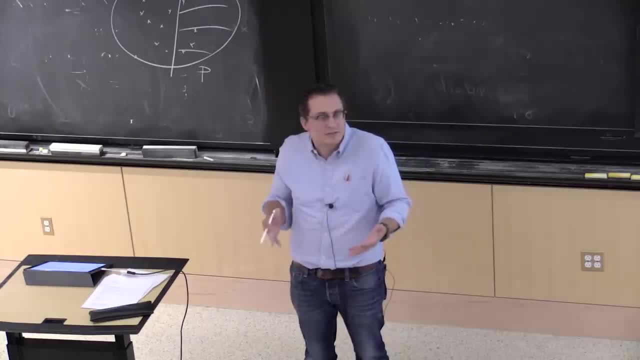 So maybe I don't want it to be too volatile. I could have one estimator which would be: just throw out 182 couples, keep only two and average those two numbers. That's definitely a worse estimator than keeping all of the 124.. 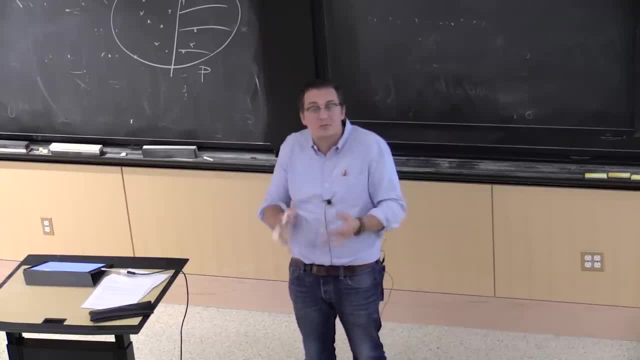 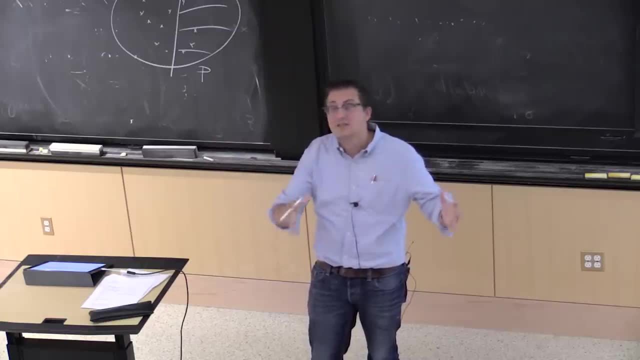 So I need to find a way to say that, And what I'm going to be able to say is that the number is going to be fluctuating. If I take another two couples, I'm probably going to get a completely different number, But if I take another 124 couples two days later, 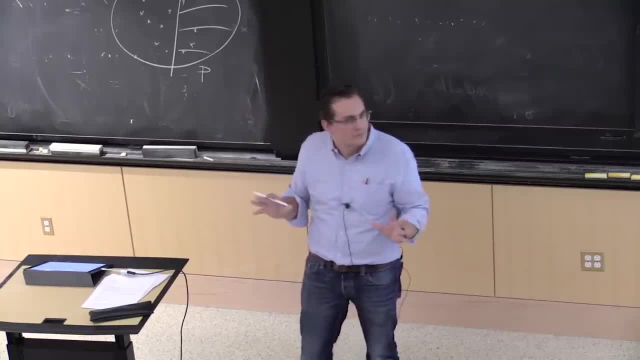 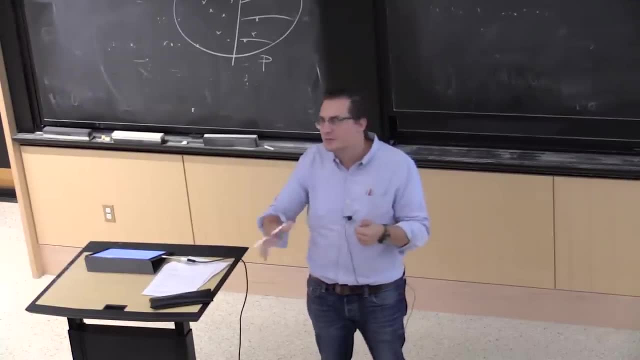 maybe I'm going to have a number that's very close to 64.5%. So that's one way. The other thing we would like about this estimator: maybe it's not too volatile, but also we want it to be close to the number that we're looking for. 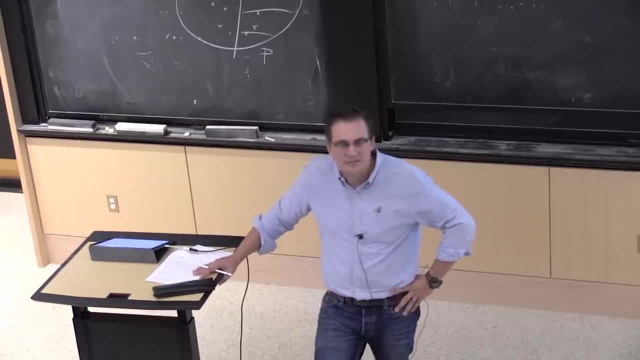 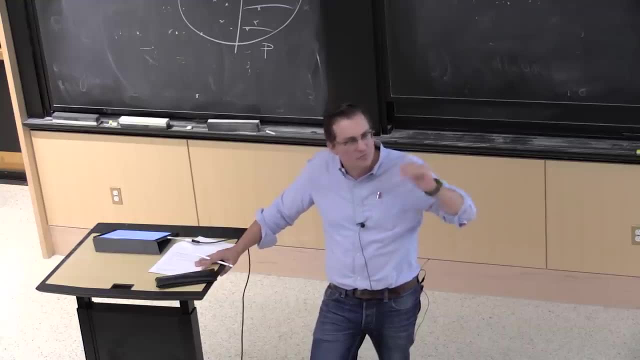 Here's an estimator. It's a beautiful random variable: 72%, That's an estimator. Go out there, Just do your favorite study about drug performance And then they're going to call you upon MIT student taking statistics and say: so how are you? 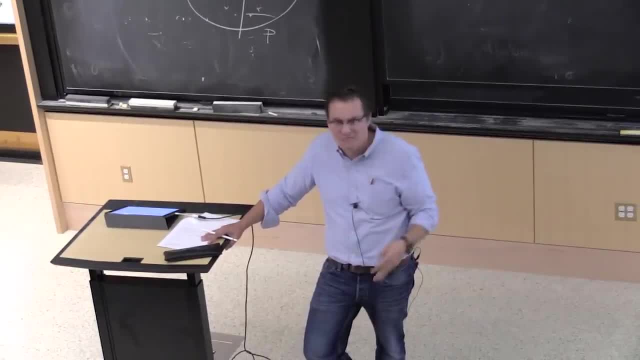 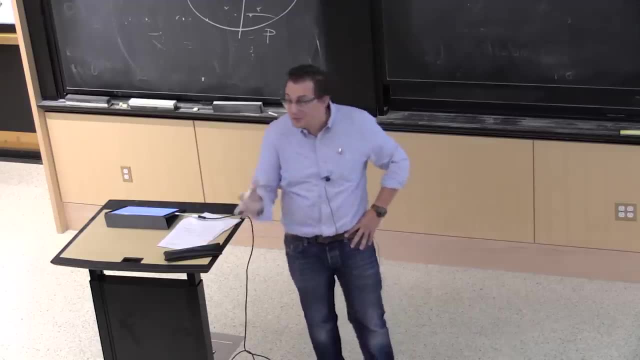 going to build your estimator. We've collected those 5,000 estimators. I'm just going to spit out 72%. whatever the data says, That's an estimator. It's a stupid estimator, but it is an estimator. But this estimator is very not volatile. 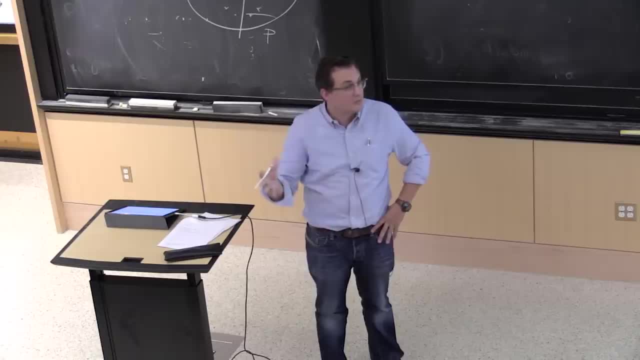 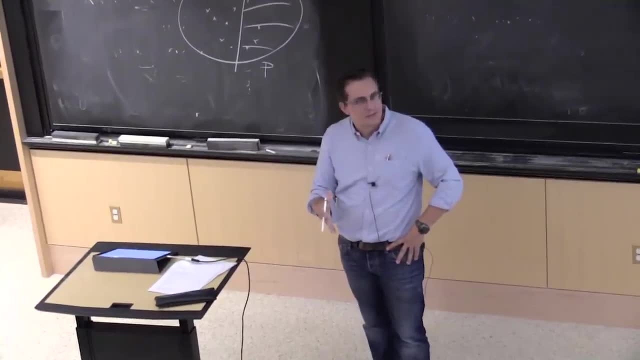 Every time you're going to have a new study. even if you change fields, it's still going to be 72%. This is beautiful. The problem is that it's probably not very close to the value you're actually trying to estimate, And so we need two things. 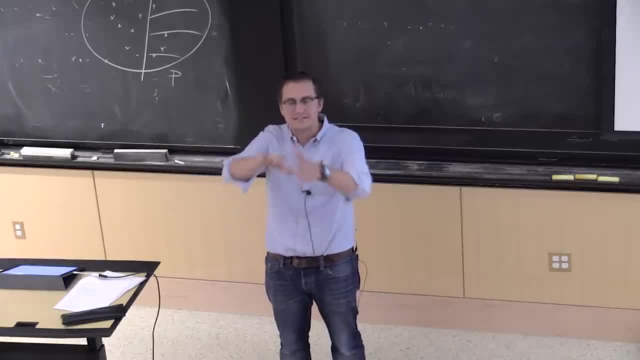 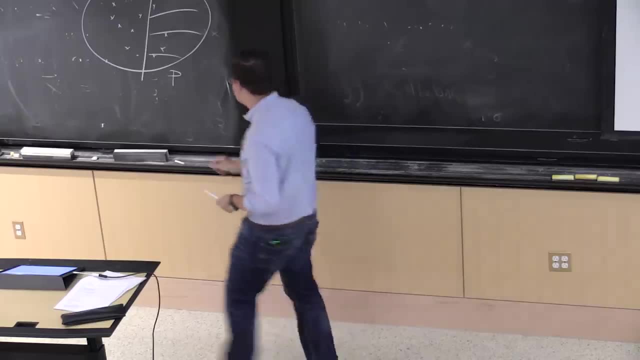 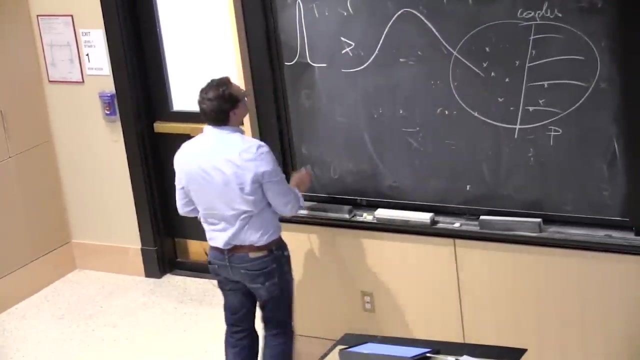 We need our estimator to be a random variable. So think in terms of densities. We want the density to be pretty narrow, We want this thing to have very little to be right, So this is definitely better than this, But also we want the number that we're interested in: p. 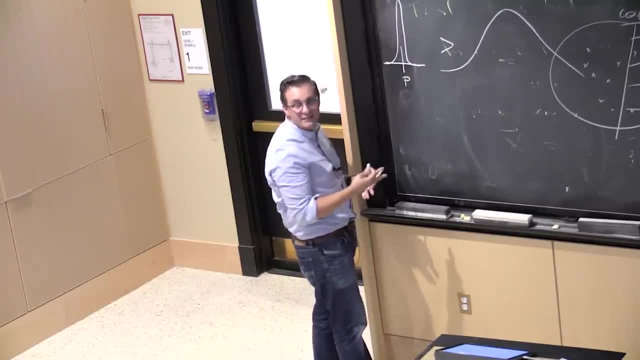 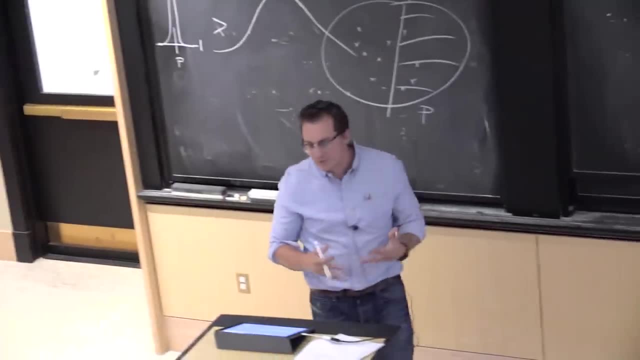 to be very close to this, to be close to the values that this thing is likely to take If p is here. this is not very good for us. So that's basically the thing we're going to be looking at. The first one is referred to as variance. 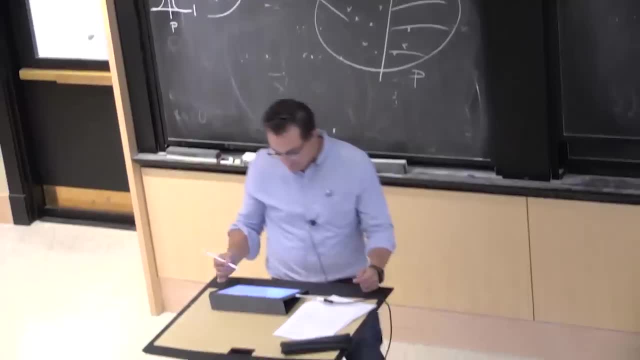 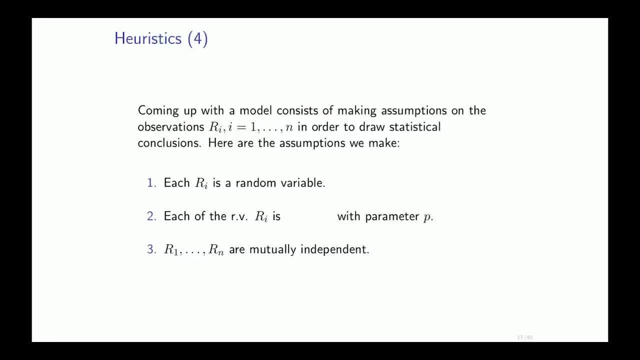 The second one is referred to as bias. Those things come all over in statistics. So we need to understand a model. So here's the model that we have for this particular problem. So we need to make assumptions on the observations that we see. 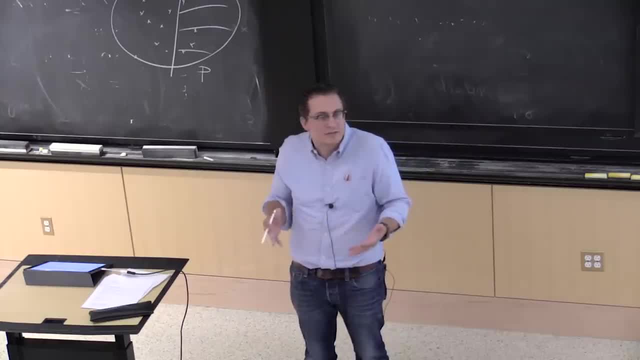 So maybe I don't want it to be too volatile. right, I could have one estimator which would be: just throw out 182 couples, keep only two and average those two numbers. That's definitely a worse estimator than keeping all of the 124.. 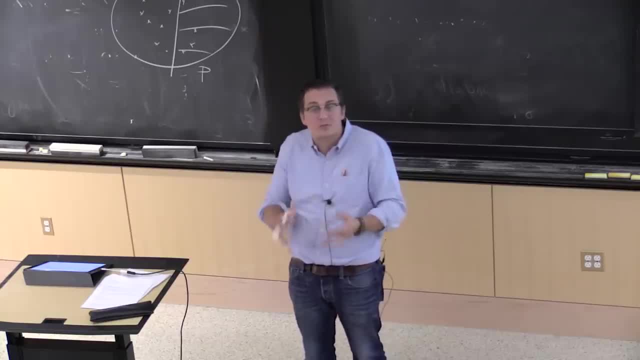 So I need to find a way to say that, And what I'm going to be able to say is that the number is going to be fluctuating. if I take another two couples, I'm going to be able to- I'm probably going to- get a completely different number. 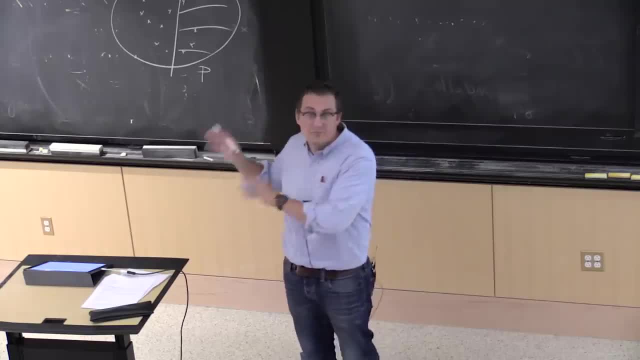 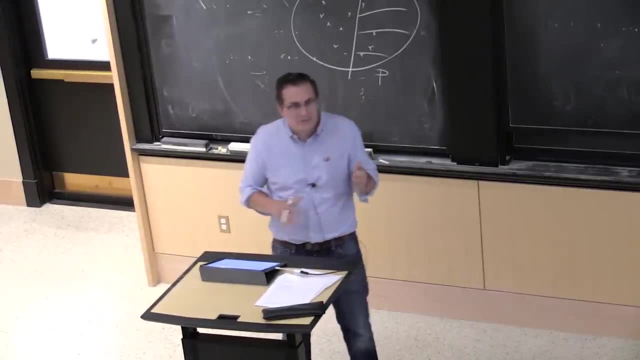 But if I take another 124 couples two days later, maybe I'm going to have a number that's very close to 64.5%. So that's one way. The other thing we would like about this estimator, it's actually maybe it's not too volatile. 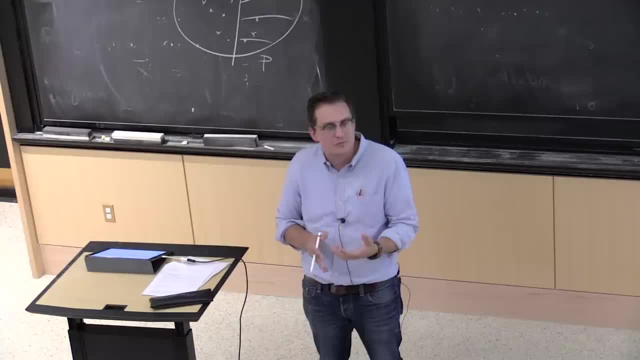 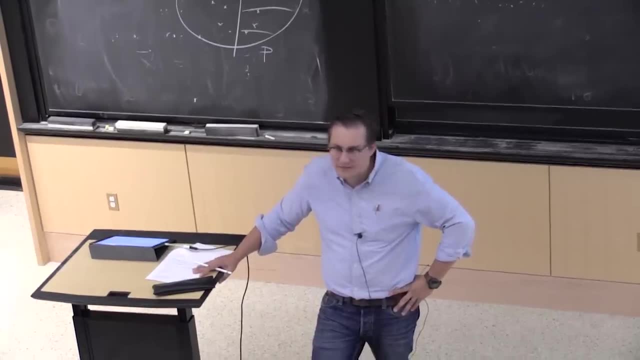 but also we want it to be close to the number that we're looking for. right, If the number here's an estimator, It's a beautiful random variable: 72%, That's an estimator. Go out there, just do your favorite study. 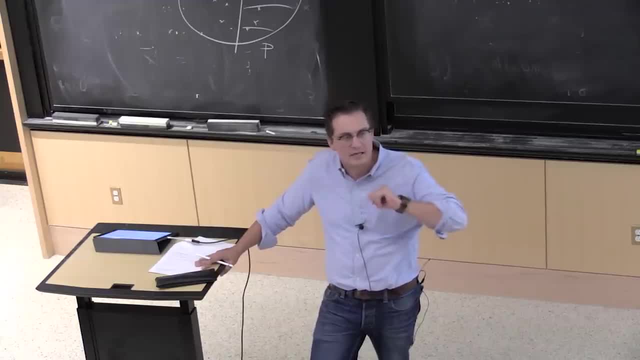 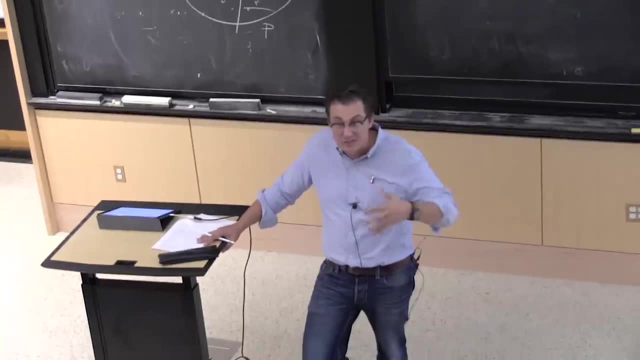 about drug performance and then they're going to call you upon MIT student taking statistics and say: so how are you going to build your estimator? We've collected those $5 on estimator. I'm just going to spit out 72%. whatever the data says. 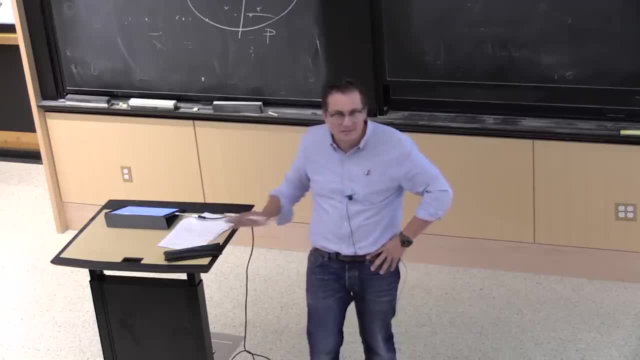 That's an estimator. It's a stupid estimator, but it is an estimator. But this estimator is very not volatile. Every time you're going to have a new study. even if you change fields, it's still going to be 72%. 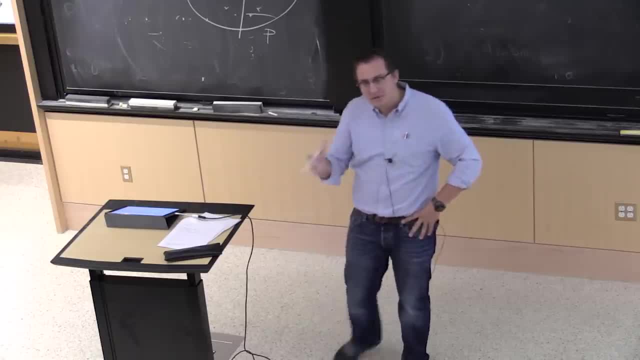 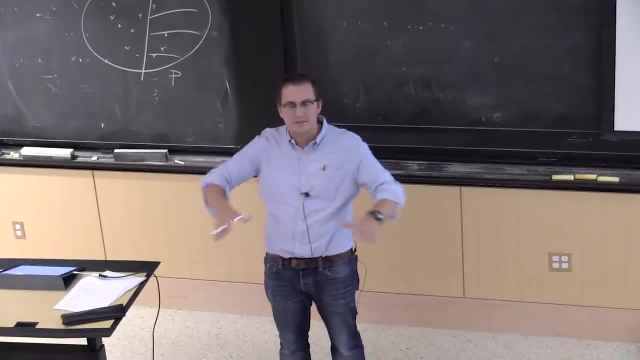 This is beautiful, And that's it. The problem is that it's probably not very close to the value you're actually trying to estimate, And so we need two things. We need our estimator to be a random variable, So think in terms of densities. 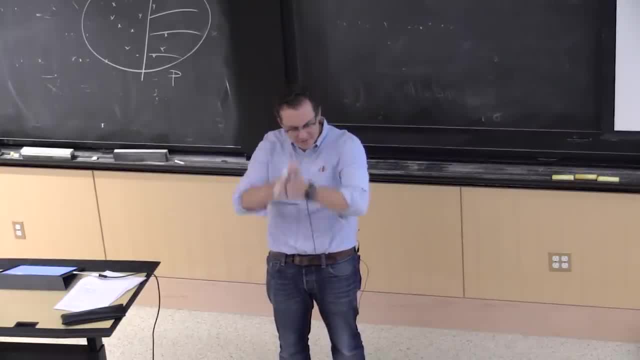 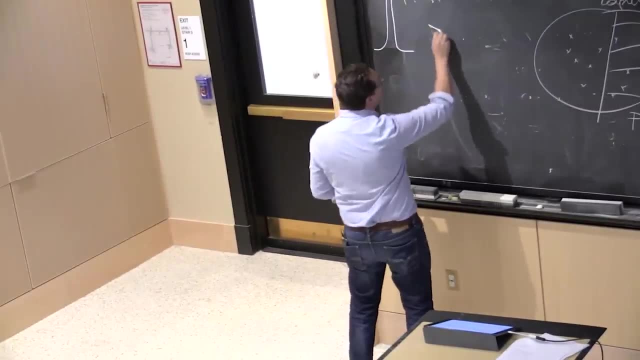 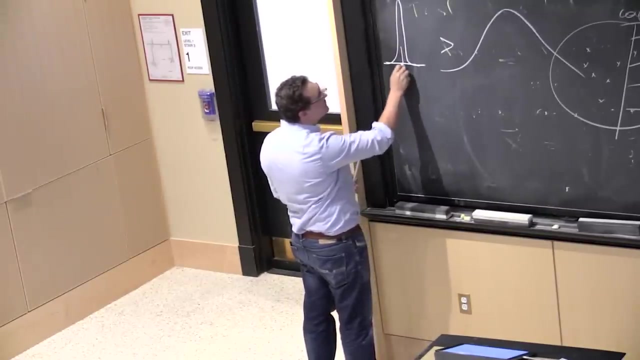 We want the density to be pretty narrow. We want this thing to have very little to be right, So this is definitely better than this. But also we want the number that we're interested in, p, to be very close to this, to be close to the values. 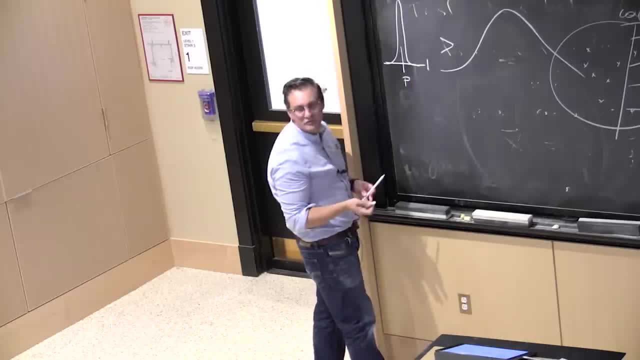 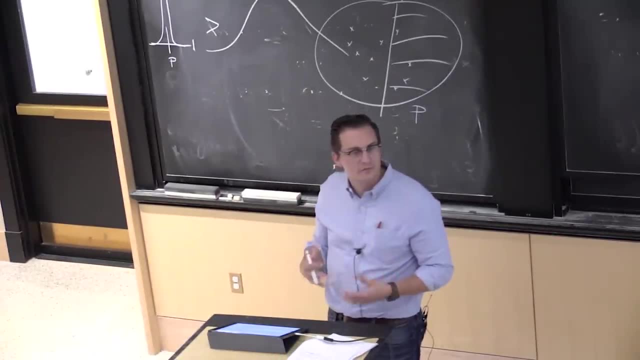 that this thing is likely to take. If p is here, this is not very good for us, OK, So that's basically the thing we're going to be looking at. The first one is referred to as variance. The second one is referred to as bias. 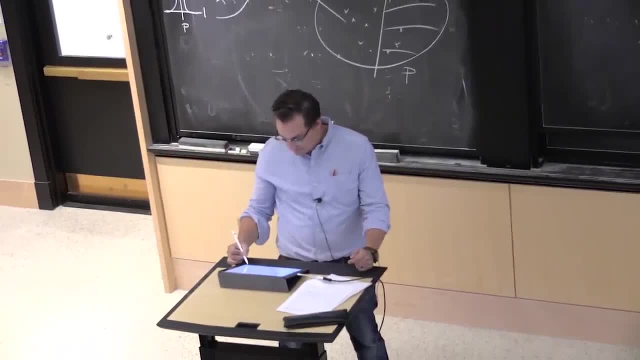 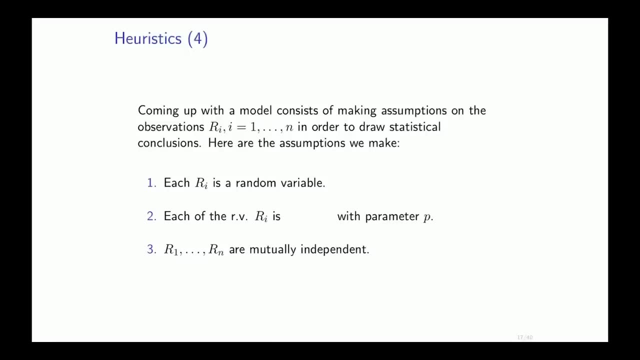 Those things come all over in statistics. OK, so we need to understand a model, right? So here's the model that we have for this particular problem. So we need to make assumptions on the observations that we see right. So we said we're going to assume that the random variable, that's 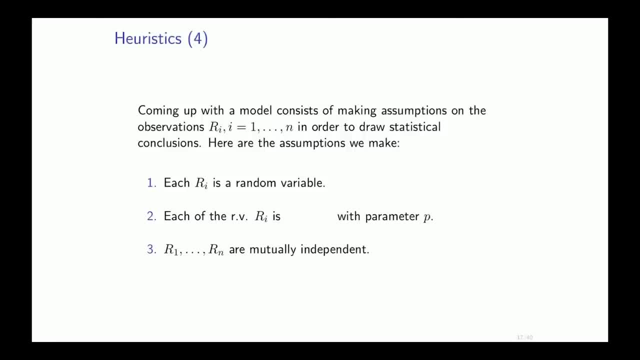 not too much of a leap of faith. We're just sweeping under the rug everything we don't understand about those couples, And the assumption that we make is that each ri is a random variable. OK, this one you will forget very soon. The second one is that each of the ri's is 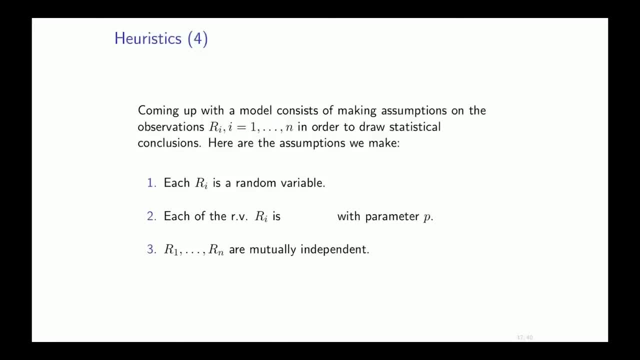 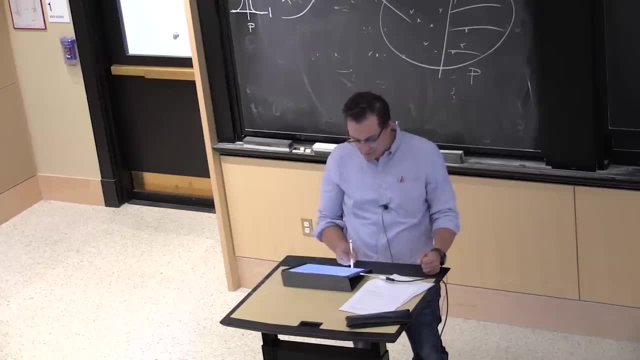 So it's a random variable that takes value 0 or 1.. Anybody can suggest the distribution for this random variable. What Bernoulli? right, And it's actually beautiful. This is where you have to do the least statistical modeling. 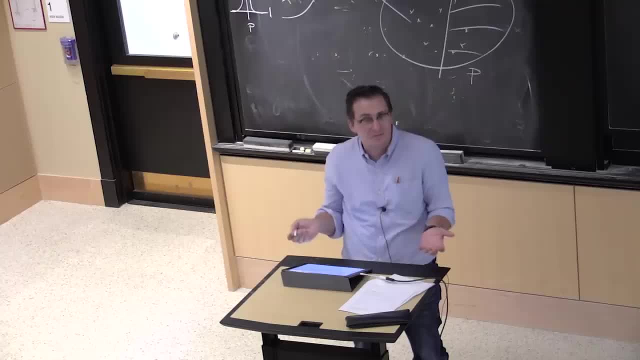 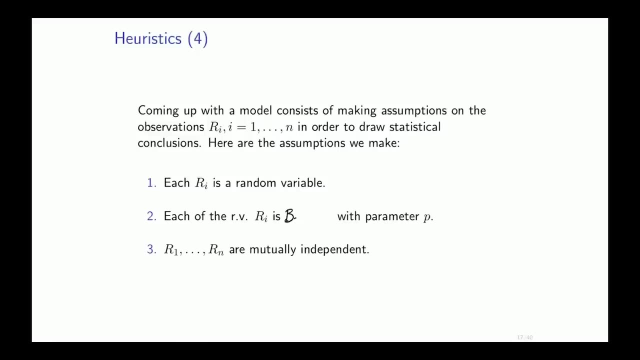 The random variable that takes value 0 or 1 is always a Bernoulli. That's the simplest variable that you can ever think of, right? Any variable that takes only two possible values can be reduced to a Bernoulli. OK, so this is a Bernoulli. 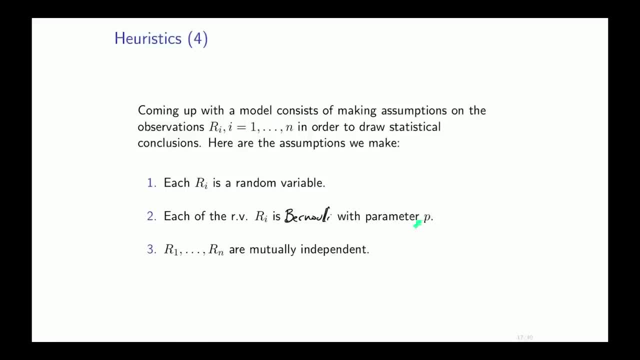 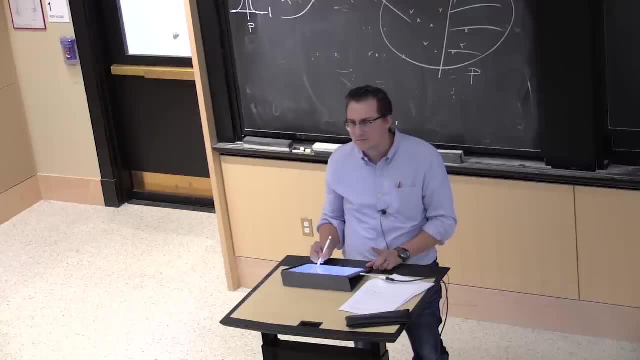 And here we make the assumption that it actually takes parameter p right, And there is an assumption here. Anybody can tell me what the assumption is? Yeah, it's the same right. I could have said pi, but it's p. 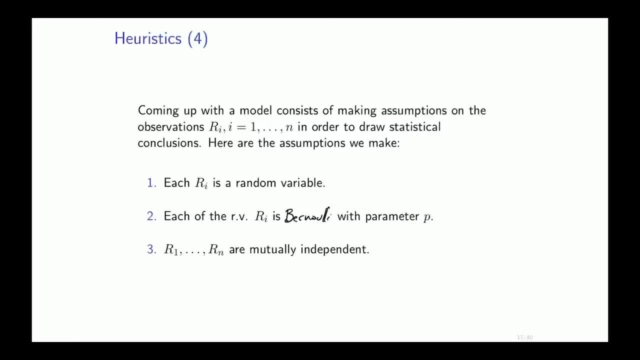 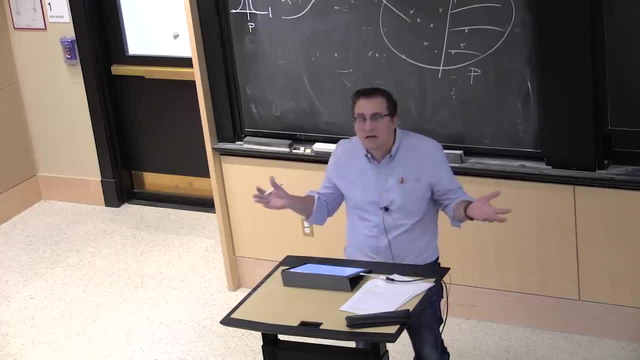 And that's where I'm going to be able to start getting to do some statistics- is that I'm going to start to be able to pull information across all my guys. If I assume that they're all pi's completely uncoupled with each other, then I'm in trouble. 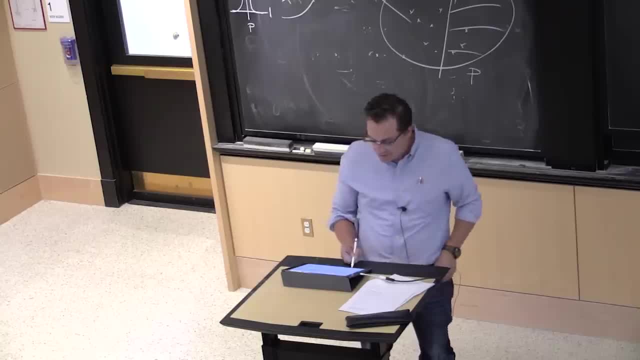 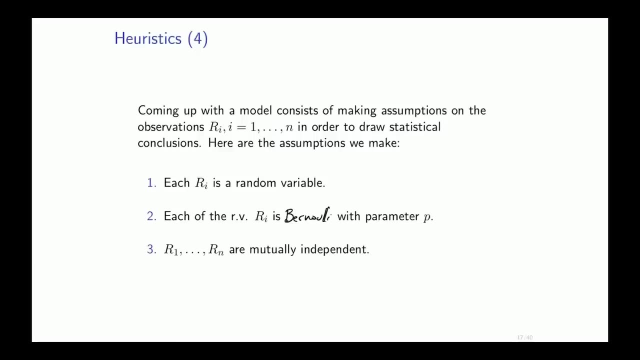 There's nothing I can actually get, And then I'm going to assume that those guys are mutually independent And most of the time they will just say independent, meaning that it's not like all this guy called each other and it's actually a flash mob. 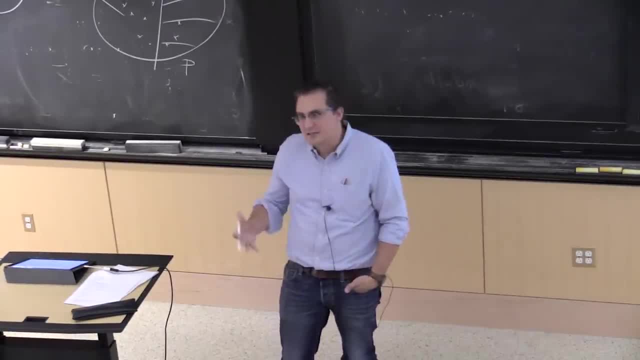 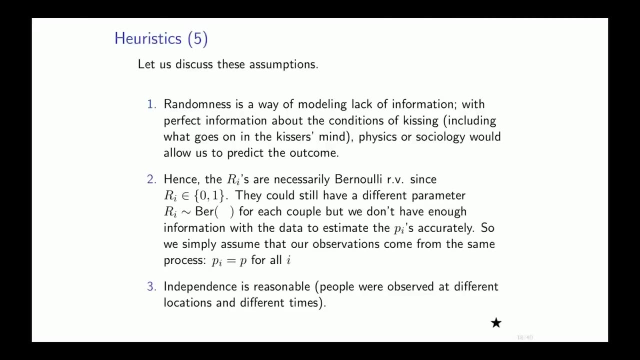 And they were like: let's all turn our heads to the left, And then this is definitely not going to give you a valid conclusion. OK, So again, randomness is a way of modeling lack of information. Here there is a way to figure it out. 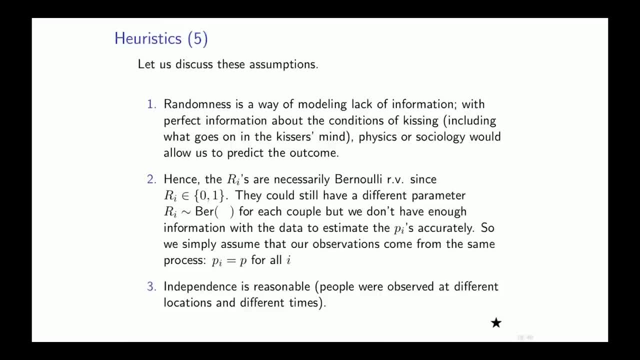 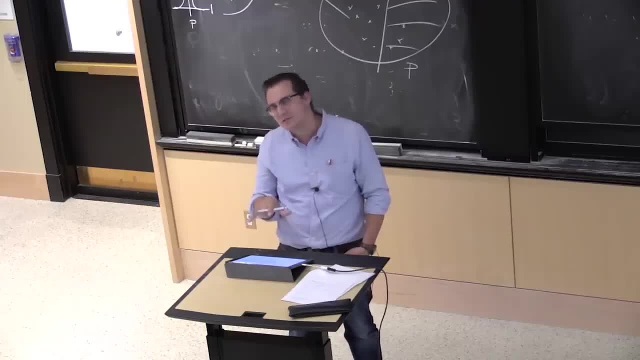 Maybe I could have followed all those guys and know exactly what they were. Maybe I could have looked at pictures of them in the womb and guessed how they were turning. Oh, by the way, that's one of the conclusions: They're guessing that we turn our head to the right. 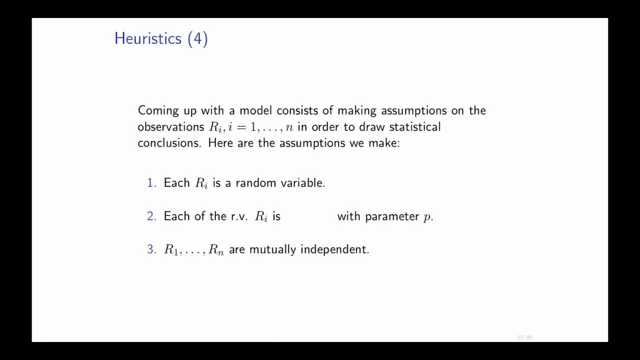 So we said we're going to assume that the random variable that's not too much of a leap of faith. We're just sweeping under the rug everything we don't understand about those couples And the assumption that we make is that each ri is a random variable. 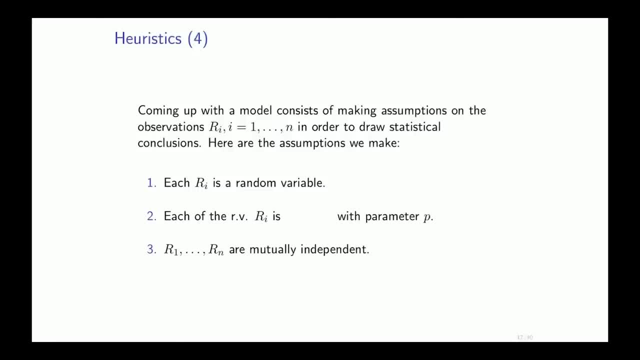 This one you will forget very soon. The second one is that each of the ri's is, So it's a random variable that takes value 0, 1.. Anybody can suggest the distribution for this random variable? What Bernoulli right. 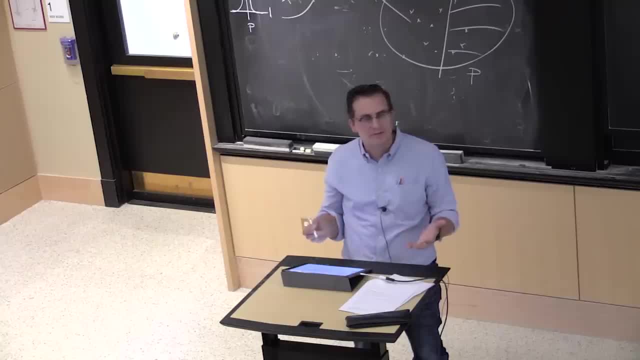 And it's actually beautiful. This is where you have to do the least statistical modeling. The random variable that takes value 0, 1 is always a Bernoulli. That's the simplest variable that you can ever think of. Any variable that takes only two possible values. 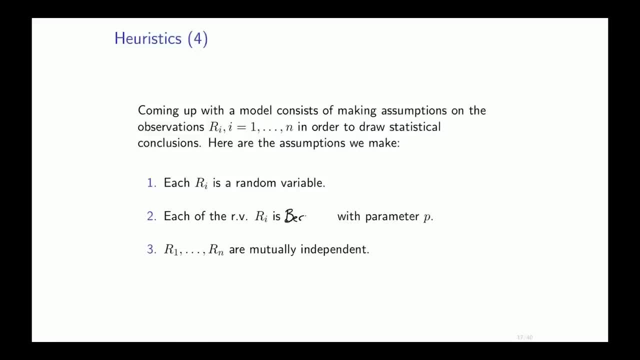 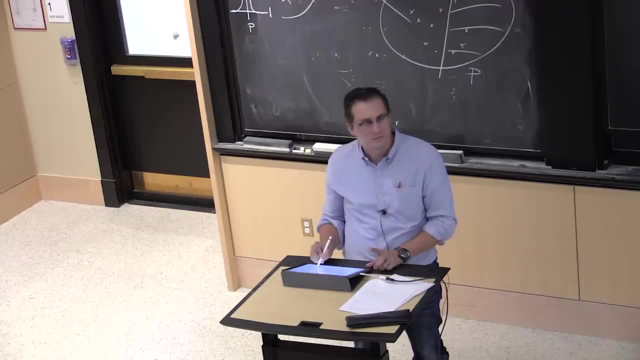 can be reduced to a Bernoulli. So this is a Bernoulli And here we make the assumption that it actually takes parameter p And there is an assumption here. Anybody can tell me what? the assumption is Same, whatever, PHILIPPE RIGOLLET, Yeah, it's the same. 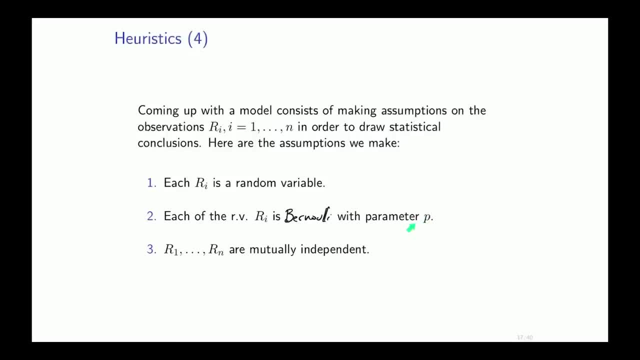 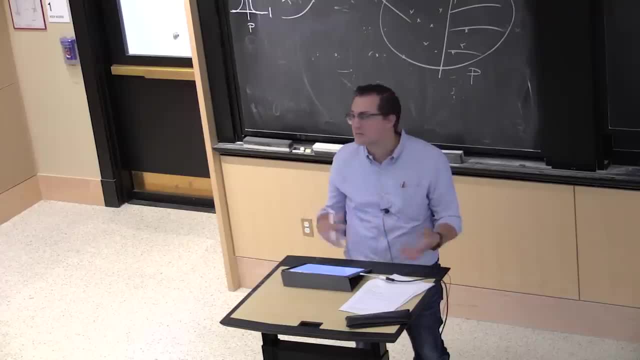 I could have said pi, but it's p And that's where I'm going to be able to start getting to do some statistics, Because I'm going to start to be able to pull information across all my guys, If I assume that they're all pi's completely uncoupled. 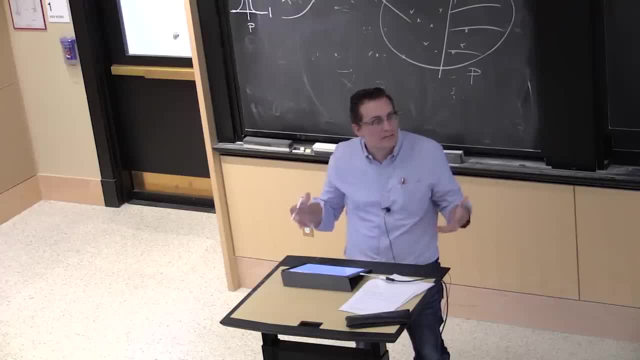 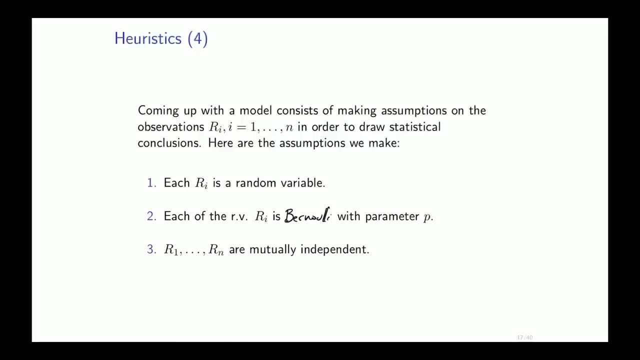 with each other, then I'm in trouble. There's nothing I can actually get, And then I'm going to assume that those guys are mutually independent, And most of the time they will just say independent, meaning that it's not like all these guys called each other. 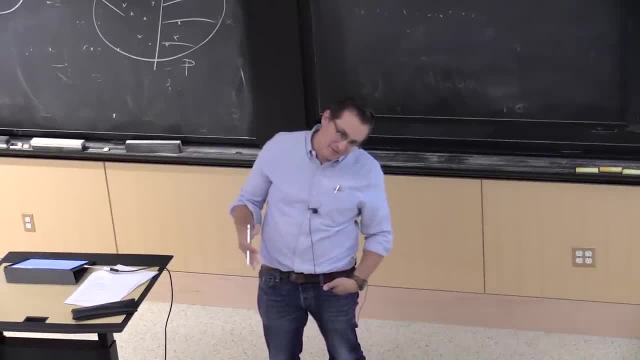 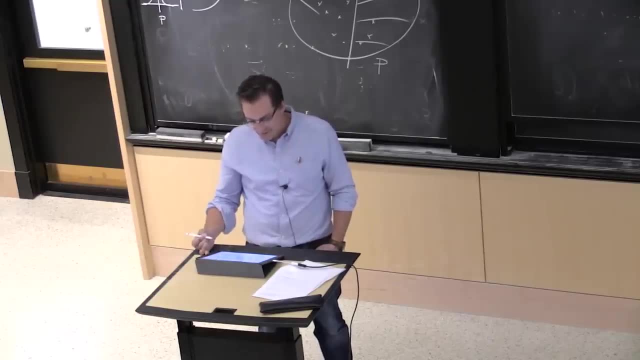 and it's actually a flash mob, And they were like: let's all turn our heads to the left, And then this is definitely not going to give you a valid conclusion. OK, so again, randomness is a way of modeling lack of information. 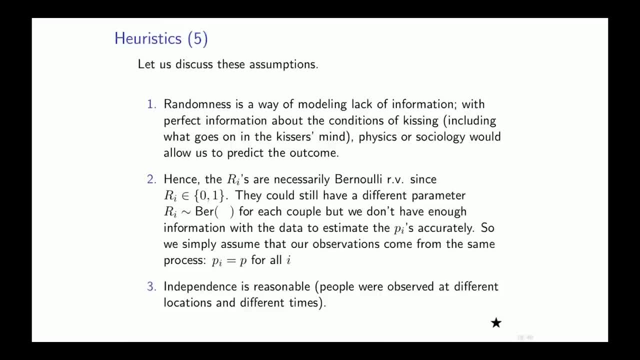 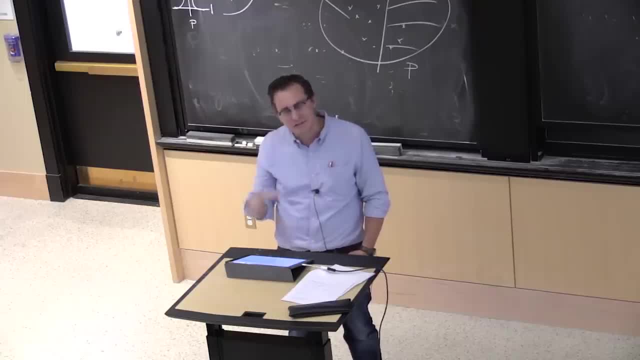 Here there is a way to figure it out. Maybe I could have followed all those guys and know exactly what they were. Maybe I could have looked at pictures of them in the womb and guess how they were turning. Oh, by the way, that's one of the conclusions. They're guessing that we turn our head to the right because our head is mostly turned to the right in the womb, So we don't know what goes on in the kissers' minds. And there's physics, sociology. There's a lot of things that could help us. 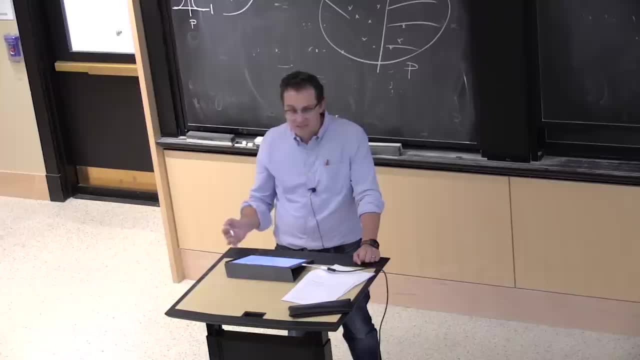 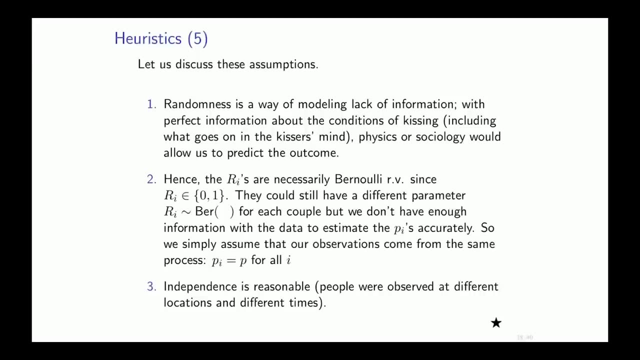 but it's just too complicated to keep track of or too expensive for many instances. Now again, the nicest part of this modeling was the fact that the RIs take only two values, which mean that this conclusion that they were Bernoulli. 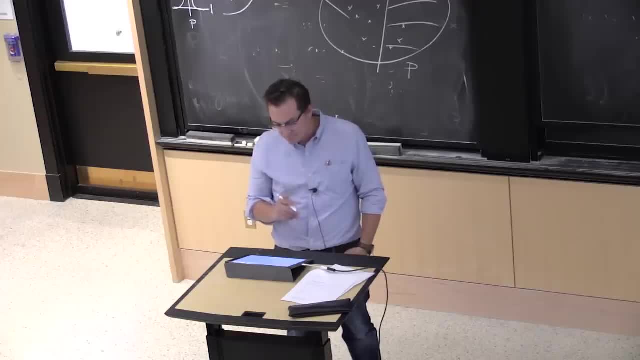 because our head is mostly turned to the right in the womb, So we don't know what goes on in the kissers' minds. And there's physics, sociology. There's a lot of things that could help us, but it's just too complicated to keep track of. 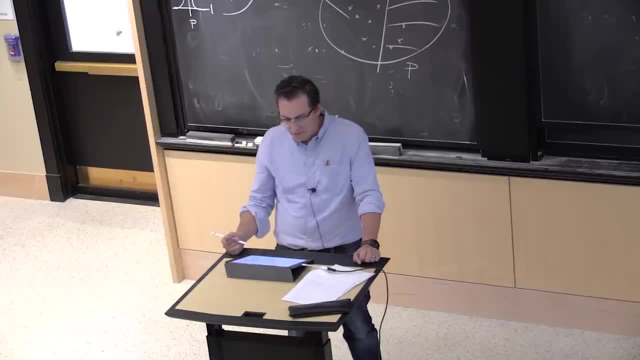 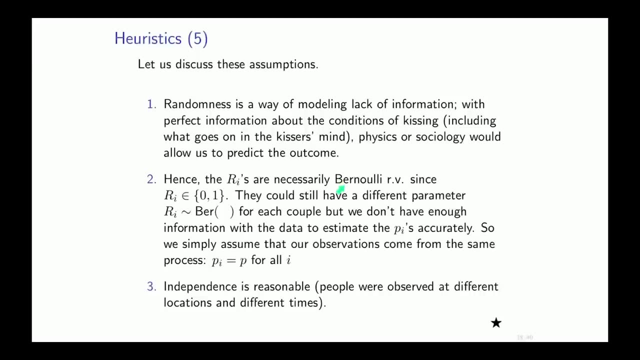 or too expensive for many instances. Now again, the nicest part of this modeling was the fact that the RIs take only two values, which mean that this conclusion that they were Bernoulli was totally free for us. Once we know it's random variable, it's a Bernoulli. 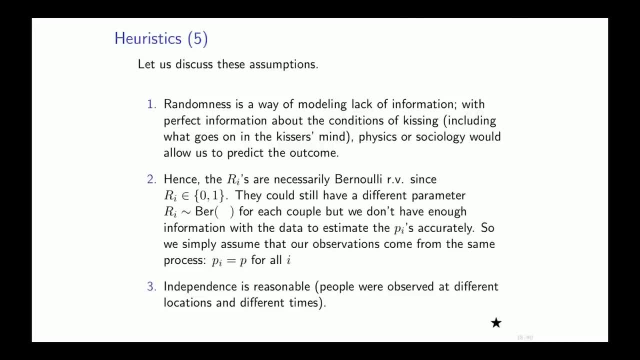 Now they could have been as we said. they could have been a Bernoulli with parameter pi For each i. I could have put a different parameter, But I just don't have enough information, right? What would I say? 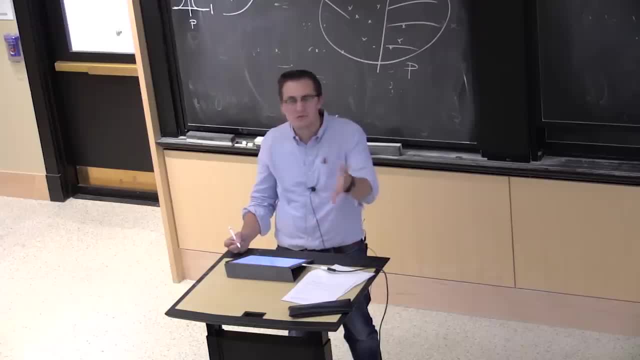 I would say: well, the first couple turn to the right, pi. p1 has to be 1.. That's my best guess. right, The second couple kiss to the left. Well, p2 should be 0.. That's my best guess. 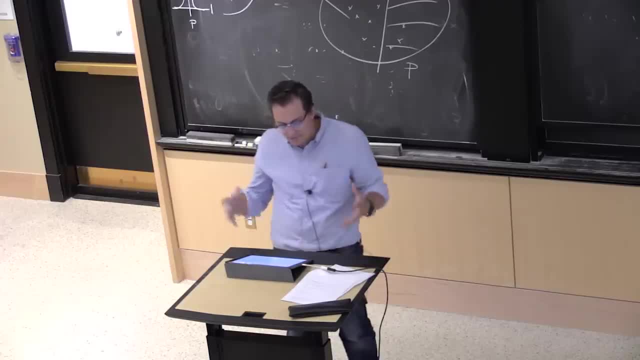 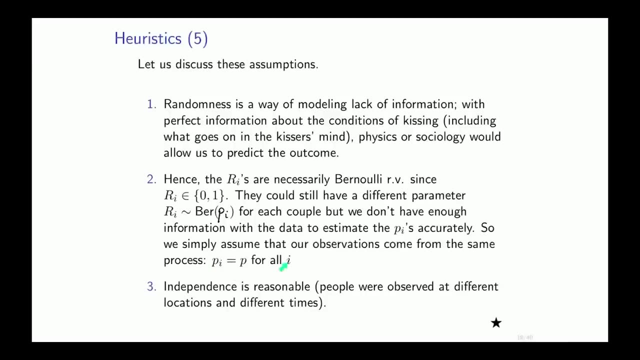 And so, basically, I need to have to be able to average my information, And the way I do it is by coupling all these guys pi's to be the same p for all i. Does it make sense Here? what I'm assuming is that my population is homogeneous. 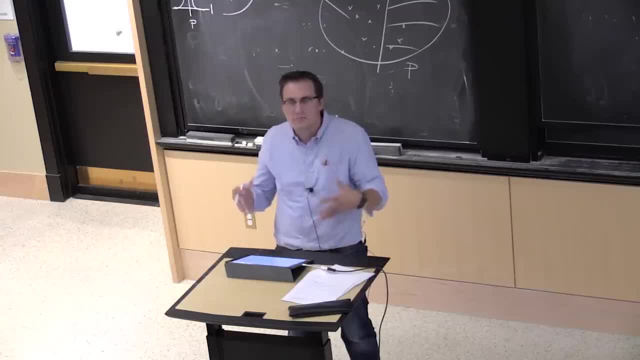 OK, Maybe it's not, Maybe I could actually look at a finer grain, But I'm basically making a statement about a population, And so maybe you kiss to the left And then I'm not making a statement about a person individually. I'm making a statement about the overall population. 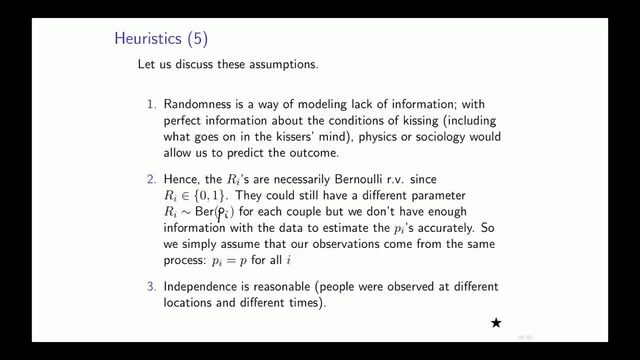 Now independence is probably reasonable, right? This person just went And you can seriously hope that this couple did not communicate with each other or that you know they did not text that. we should all turn our head to the left now. 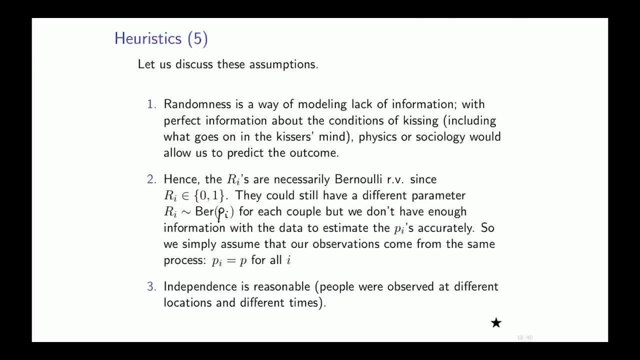 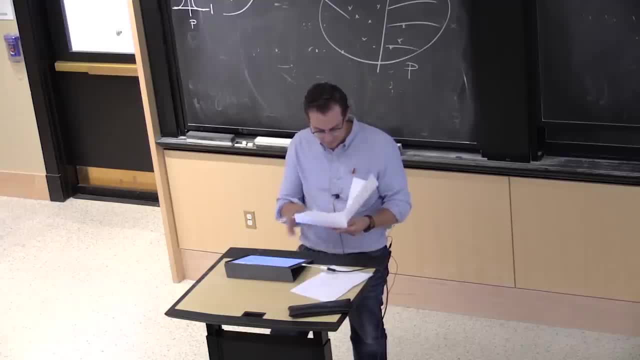 And there's no external stimulus that forces people to do something different. OK, so sorry about that. Since we have about less than 10 minutes, let's do a little bit of exercises, Is that OK with you? So I just have some exercises, so we. 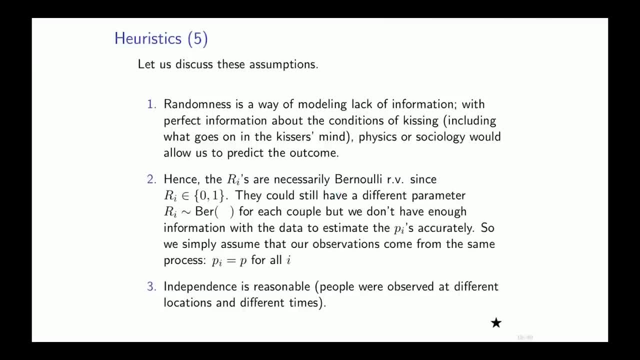 was totally free for us. Once we know it's a random variable, it's a Bernoulli. Now they could have been as we said. they could have been a Bernoulli with parameter pi. for each i I could have put a different parameter. 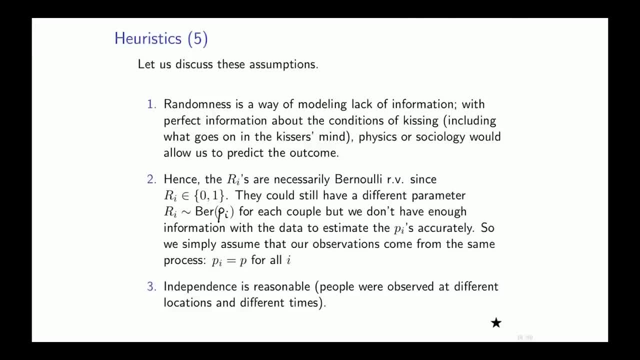 but I just don't have enough information right. What would I have said? I would say, well, the first one is that the first couple turn to the right, pi p1 has to be 1. That's my best guess, right. 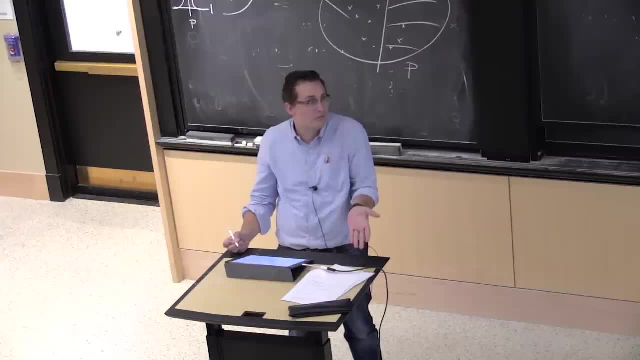 The second couple kiss to the left. Well, p2 should be 0. That's my best guess, And so, basically, I need to have to be able to average my information, And the way I do it is by coupling all these guys pi's. 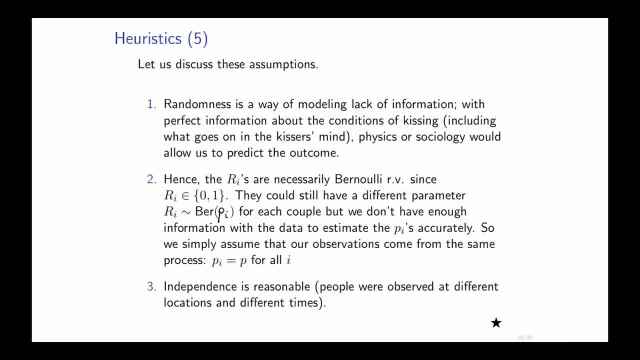 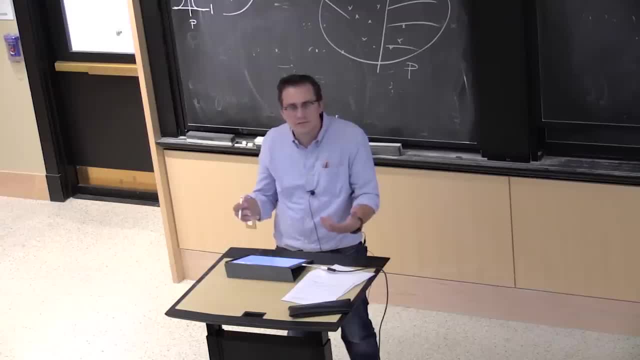 to be the same p for all i. Does it make sense Here? what I'm assuming is that my population is homogeneous. Maybe it's not. Maybe I could actually look at a finer grain, But I'm basically making a statement about a population. 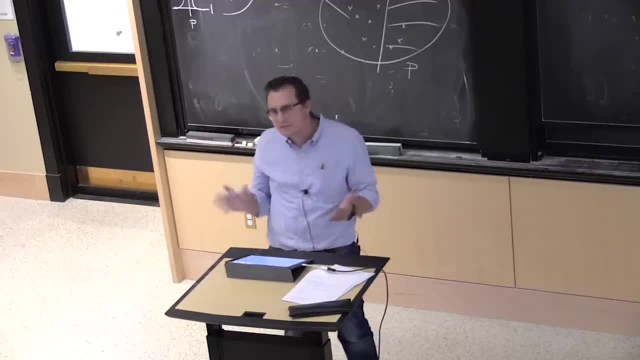 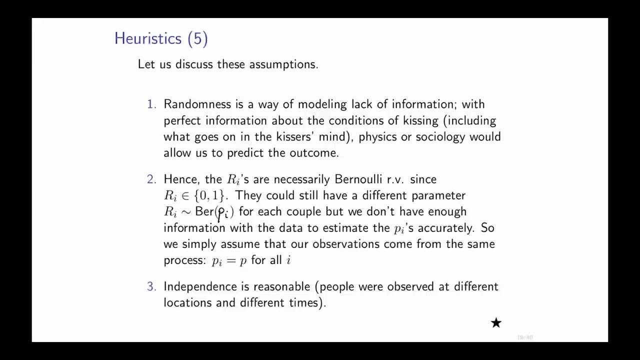 And so maybe you kiss to the left And then I'm not making a statement about a person individually. I'm making a statement about the overall population. Now, independence is probably reasonable, right? This person just went and you can seriously hope that this couple did not communicate with each other. 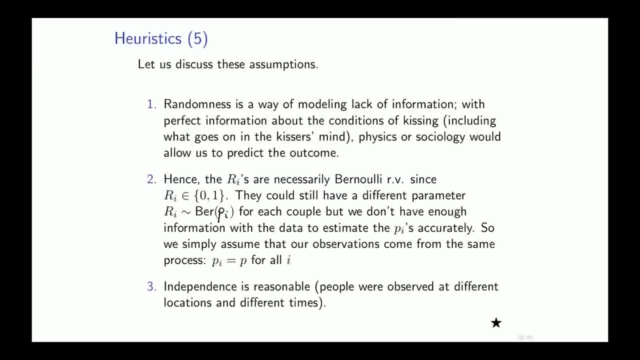 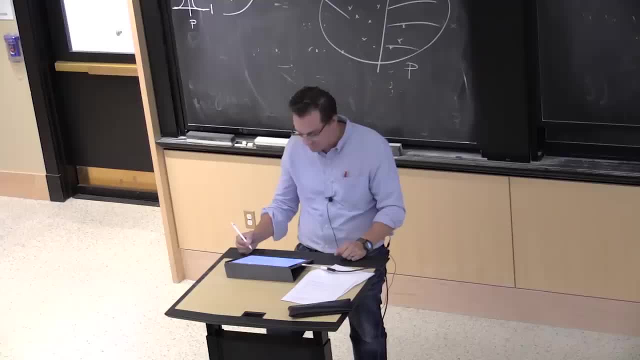 or that Kanye did not text That we should all turn our head to the left now And there's no external stimulus that forces people to do something different. OK, so sorry about that. Since we have about less than 10 minutes, let's do a little bit of exercises. 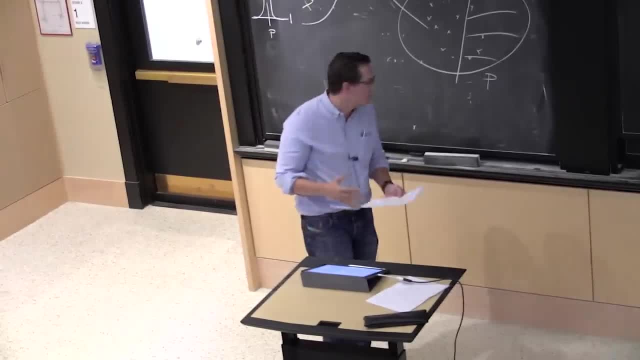 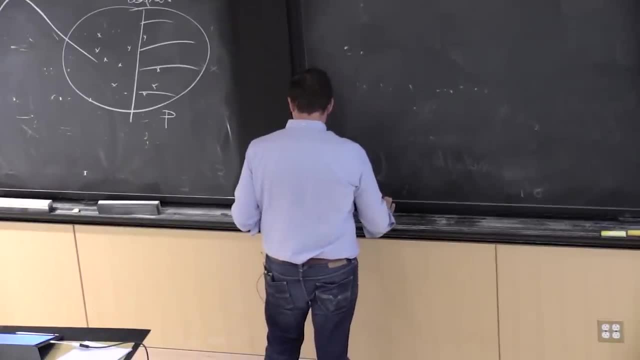 Is that OK with you? So I just have some exercises so we can see what an exercise is going to look like. This is, you know, sort of similar, Similar to the exercise you will see, but maybe we should do it together, OK. 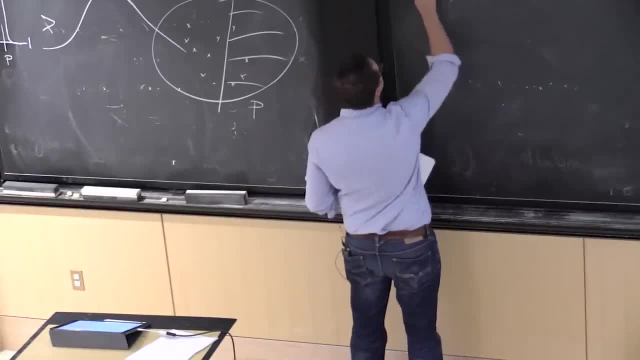 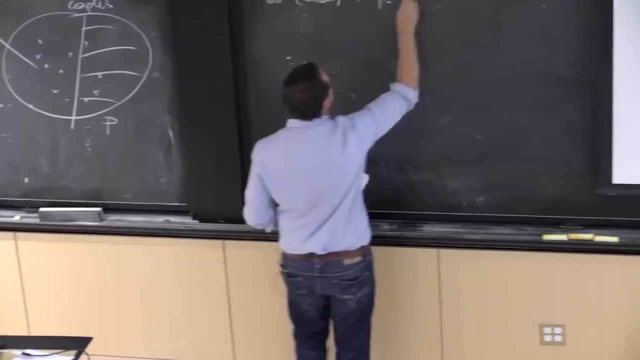 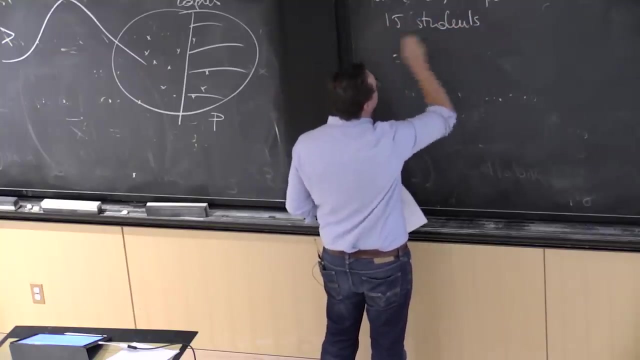 So now we're going to have- I have a test, OK, So that's an exam. say all right, in probability, OK, And I'm going to have 15 students in this test And hopefully this should be 15 grades. 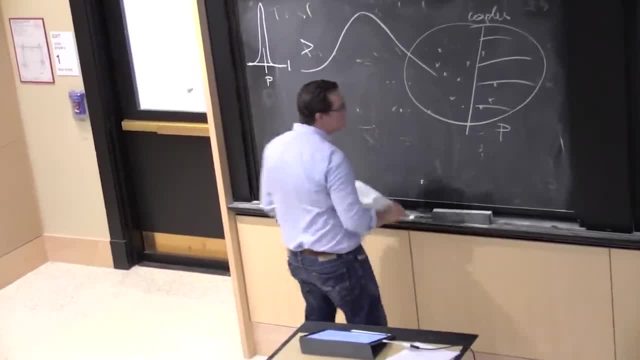 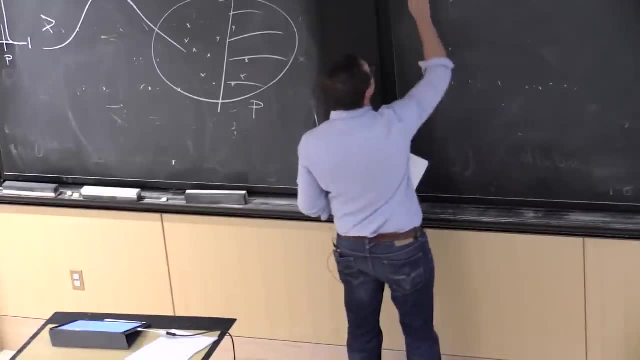 can see what an exercise is going to look like. This is, you know, Sort of similar to the exercise you will see, But maybe we should do it together, OK. So now we're going to have- I have a test, OK. 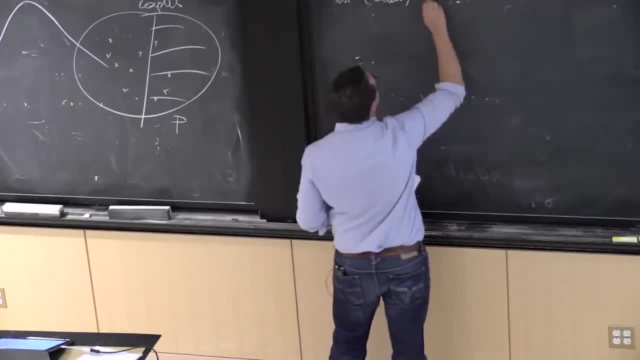 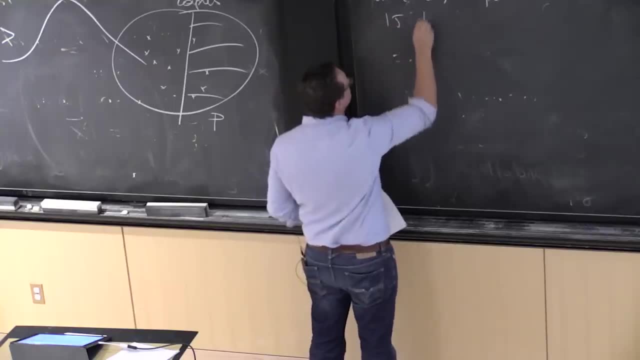 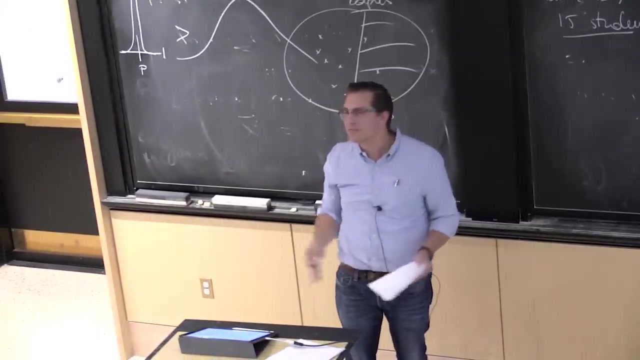 So that's an exam. say all right in probability, OK, And I'm going to have 15 students in this test And hopefully this should be 15 grades that are representative of the grades of all a large class, right? 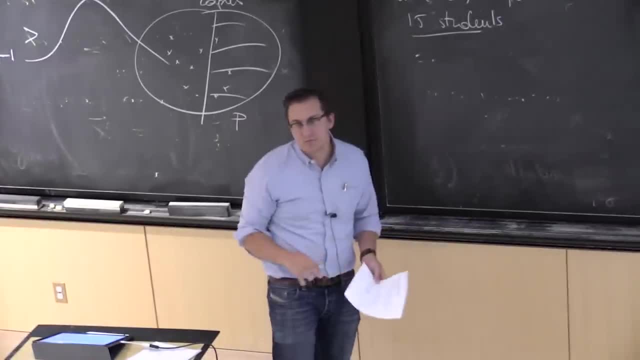 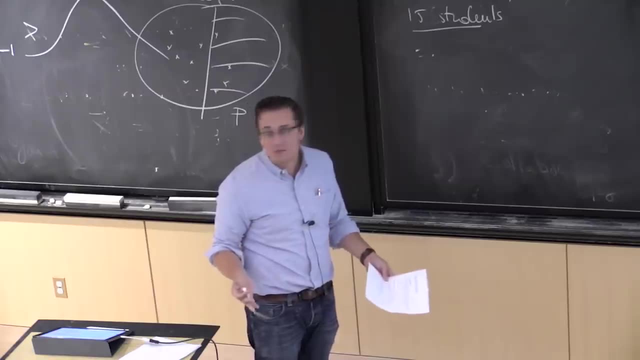 So if you took, you know 18600, it's a large class. There's definitely more than 15 students And maybe just by sampling 50 students at random, I want to have an idea of what my grade distribution will look like. OK, 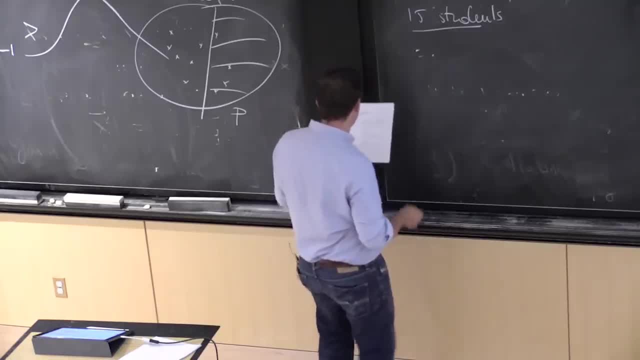 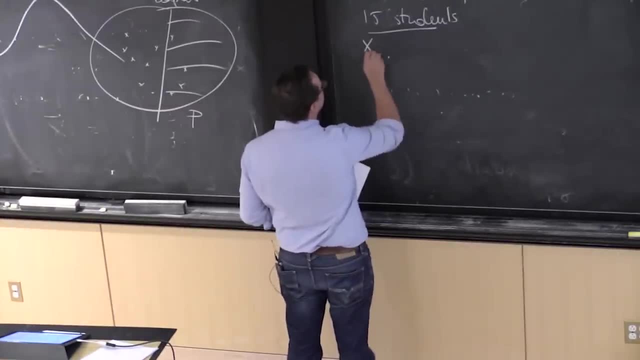 I'm grading them. I want to make an educated guess, OK, So I'm going to make some modeling assumption for those guys. OK, And so here so 15 students, and the grades are x1 to x15, right, Just like we had r1, r2, all the way to r124. 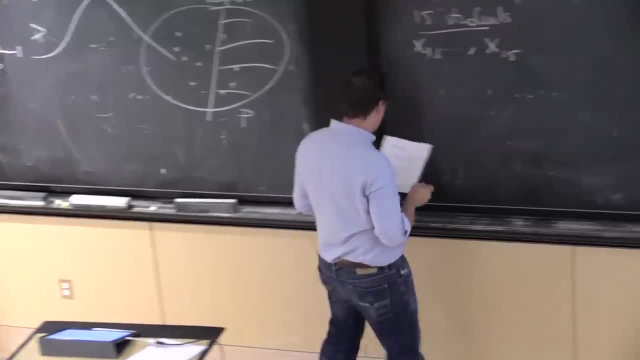 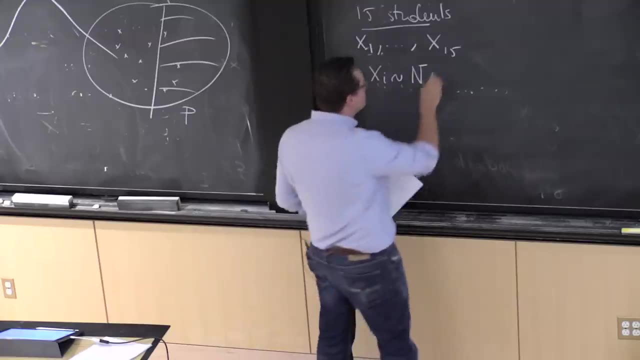 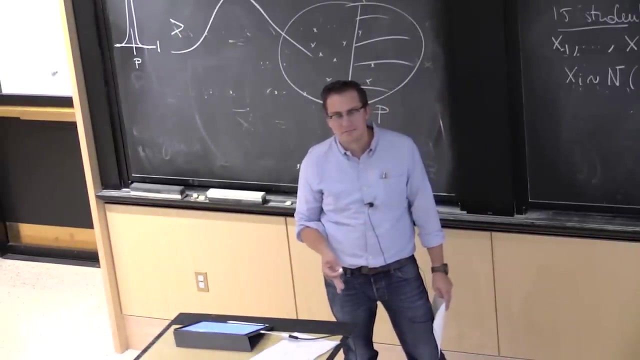 Those were my ri's, And so now I have my xi's, And I'm going to assume that xi follows a Gaussian or normal distribution with mean mu and variance sigma squared. Now this is modeling right. Nobody told me There's no physical process that makes this happen. 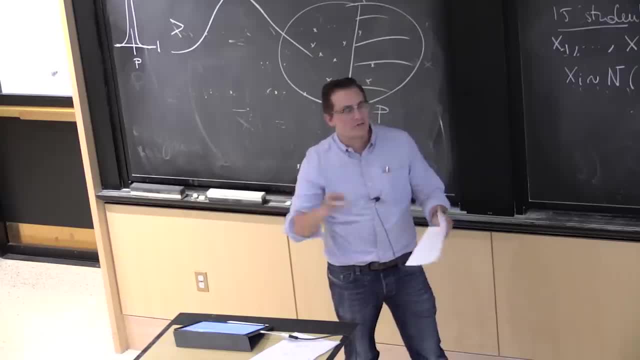 We know that there's something called the central limit theorem in the background. that says that you know, things tend to be Gaussian, But this is really a matter of convenience. Actually, this is, if you think about it, this is terrible. 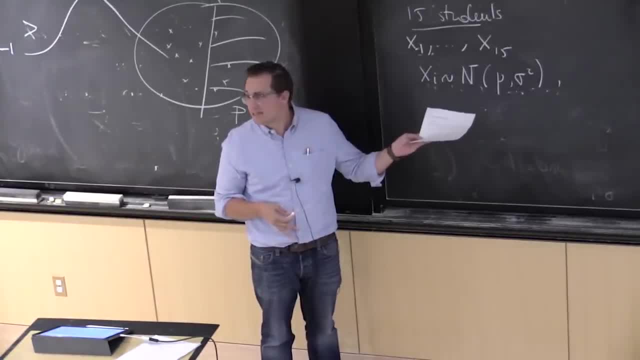 Because this puts non-zero probability on negative scores. I'm definitely not going to get a negative score, But you know it's good enough because I know the probability is non-zero, but it's probably, you know, 10 to the minus 12.. 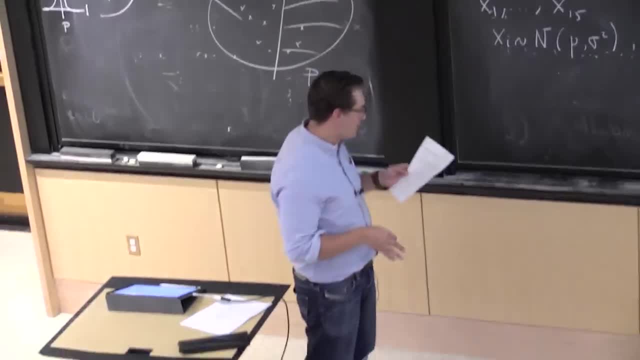 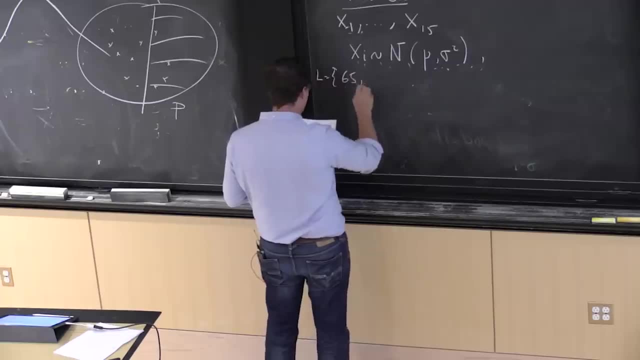 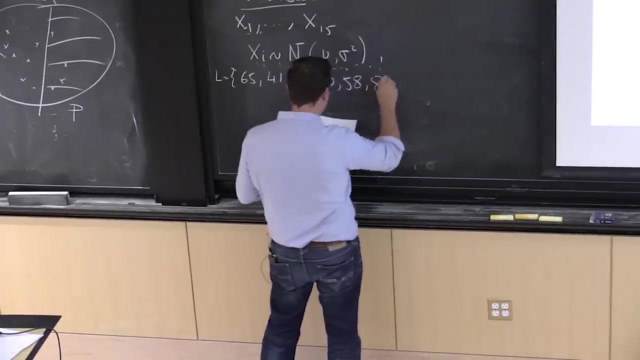 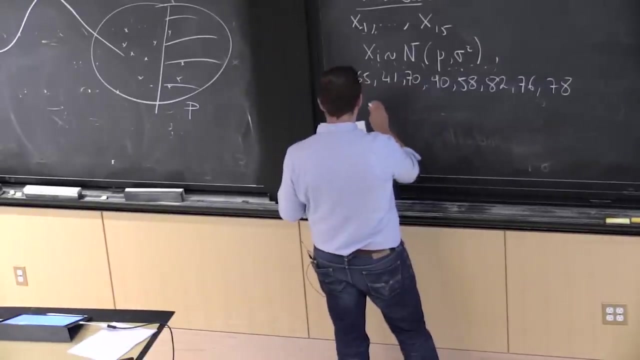 So I would be very unlucky to see a negative score. So here is the list of grades. So I have 65,, 41,, 70,, 90,, 58,, 82,, 76,, 78. Maybe I should have done it with 8.. 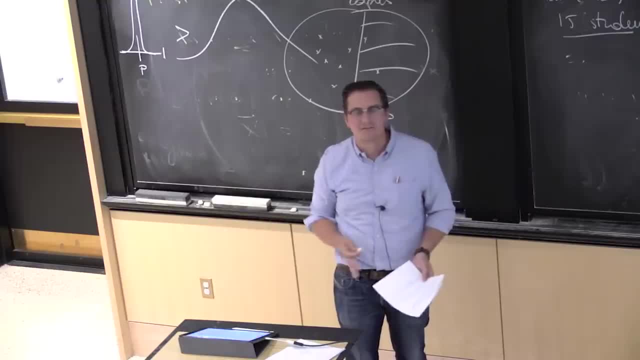 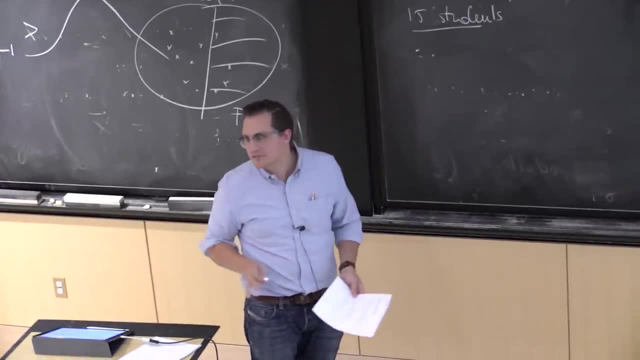 that are representative of the grades of all a large class, right? So if you took a, you know 18600 is a large class. There's definitely more than 15 students And maybe just by sampling 50 students at random. 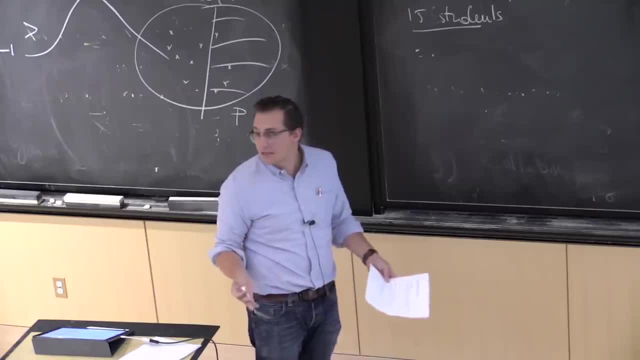 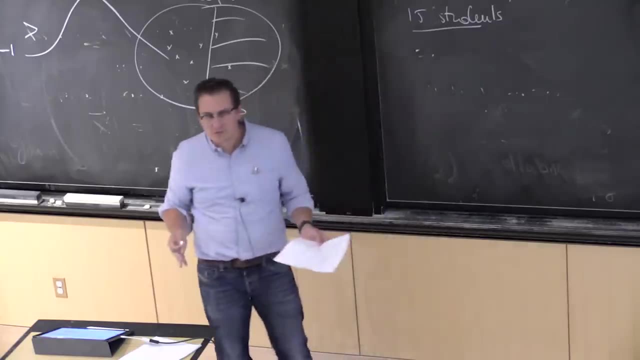 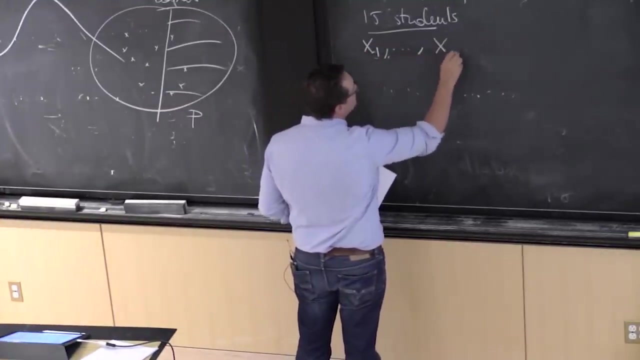 I want to have an idea of what my grade distribution will look like. OK, I'm grading them. I want to make an educated guess. OK, So I'm going to make some modeling assumption for those guys. OK, And so here. so 15 students and the grades are x1 to x15,. 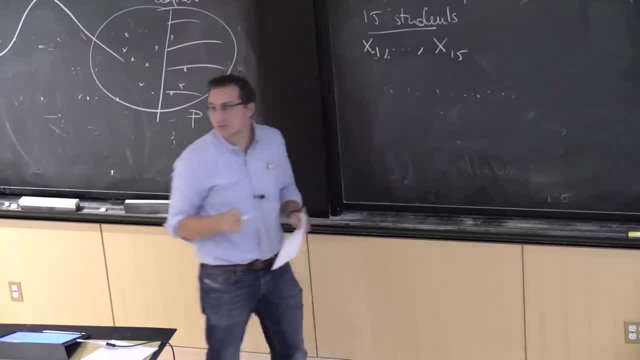 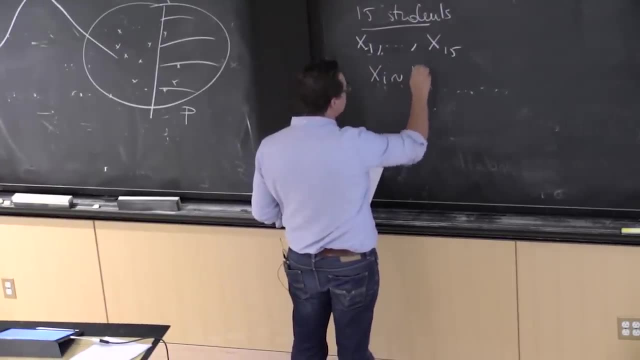 right, just like we had r1,, r2, all the way to r124.. Those were my ri's, And so now I have my xi's, And I'm going to assume that xi follows a Gaussian or normal distribution with mean mu. 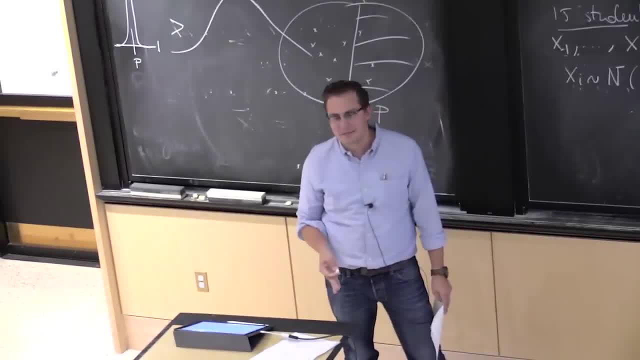 and variance sigma squared. Now this is modeling right. Nobody told me There's no physical process that makes this happen. We know that there's something called the central limit theorem in the background that says that. you know, things tend to be Gaussian. 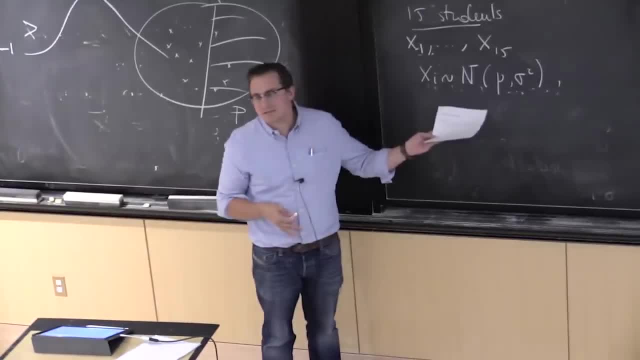 But this is really a matter of convenience. Actually, this is, if you think about it, this is terrible Because this puts non-zero probability on negative scores. I'm definitely not going to get a negative score, But you know it's good enough because I 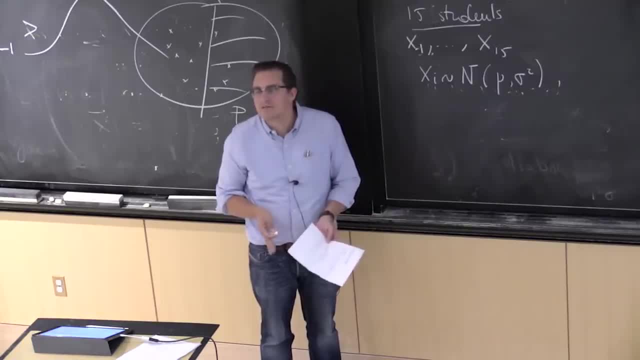 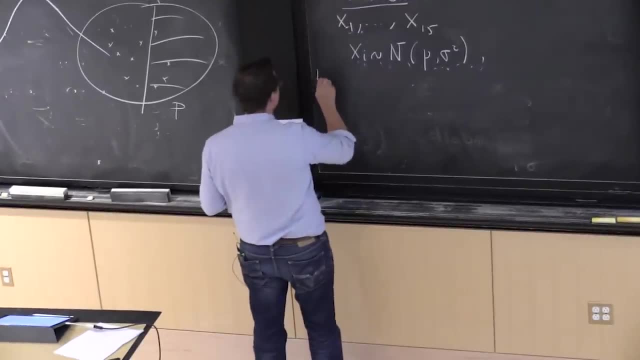 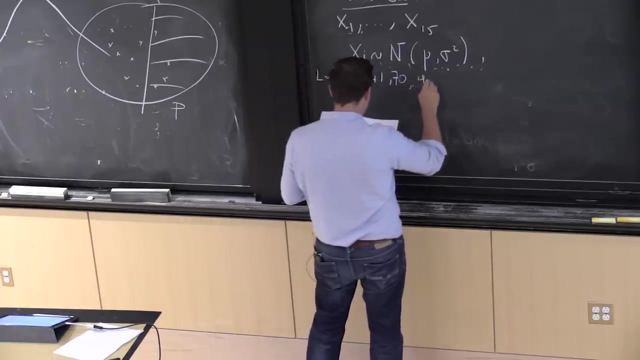 know, the probability is non-zero, But it's probably, you know, 10 to the minus 12.. So I would be very unlucky to see a negative score. So here's the list of grades. So I have 65,, 41,, 70,, 90,, 58,, 82,, 76,, 78.. 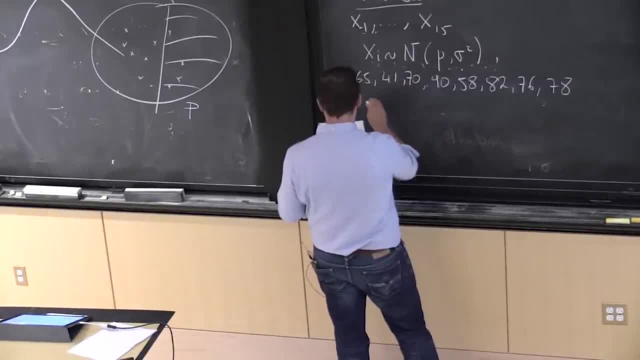 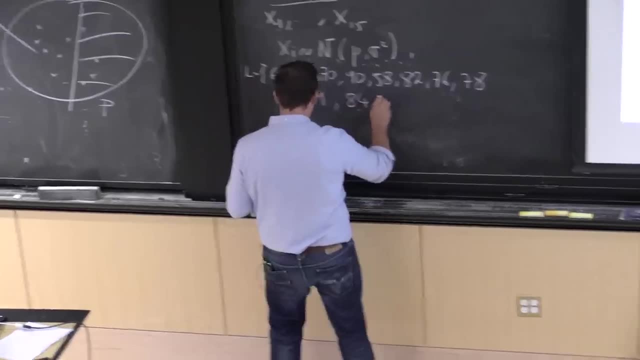 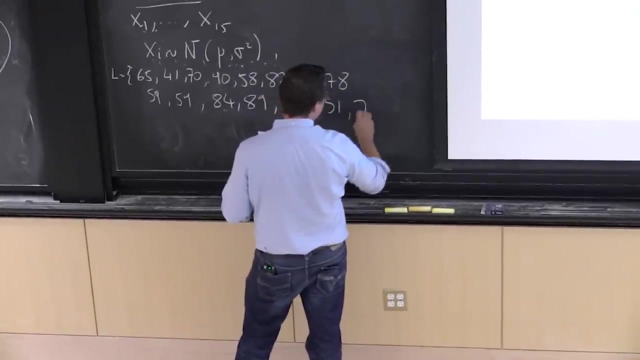 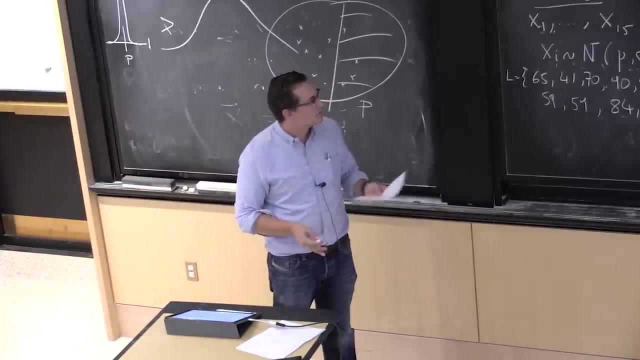 Maybe I should have done it with 8.. 59,, 59, sitting next to each other, 84,, 89,, 134,, 51, and 72.. OK, so those are the scores that I got. They were clearly some bonus points over there. 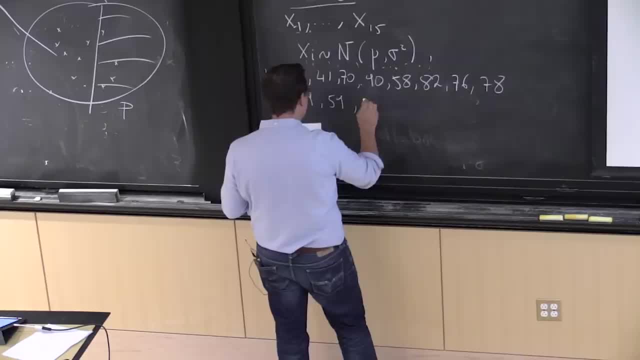 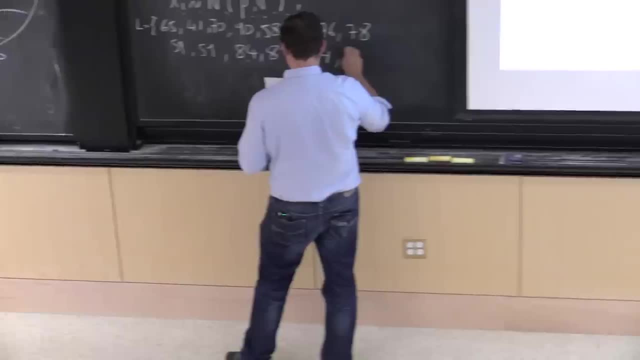 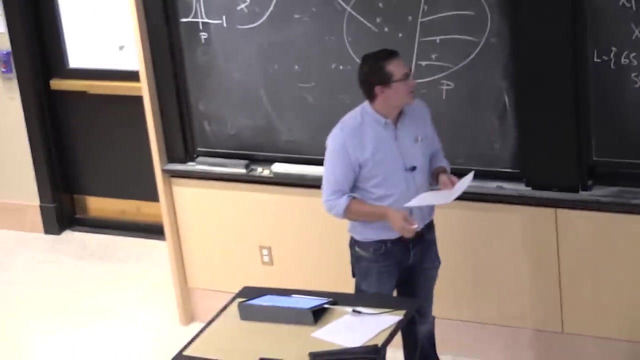 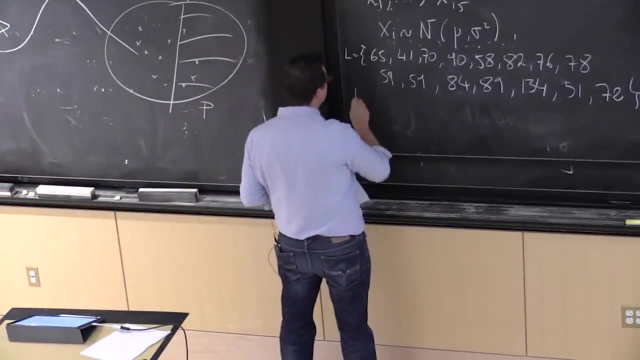 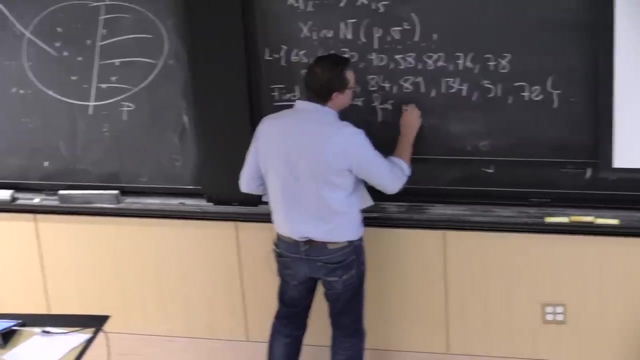 59,, 59, sitting next to each other, 84,, 89,, 134,, 51, and 72.. So those are the scores that I got. There were clearly some bonus points over there And the question is: find estimator for mu. 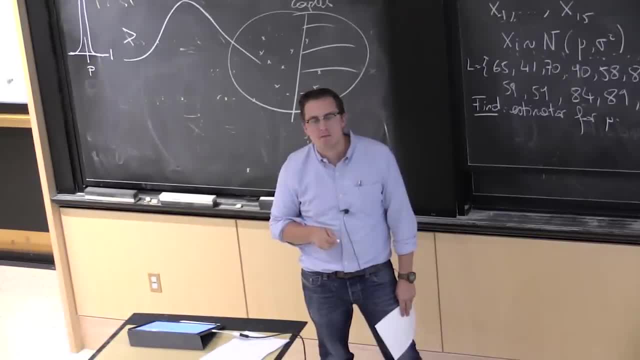 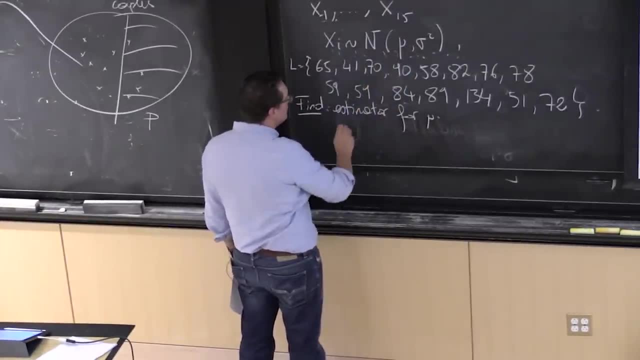 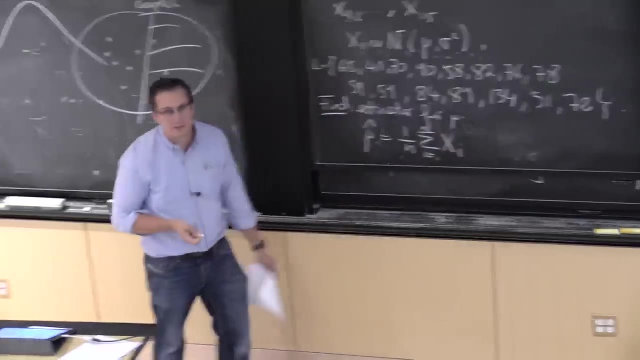 What is my estimator for mu? Well, estimator again, is something that depends on the random variable. So mu is the expectation. So a good estimator is definitely the average score, just like we had the average of the RI. Now the xi's no longer need to be 0's and 1's. 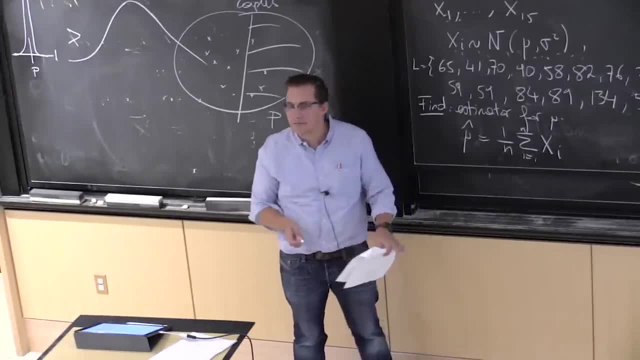 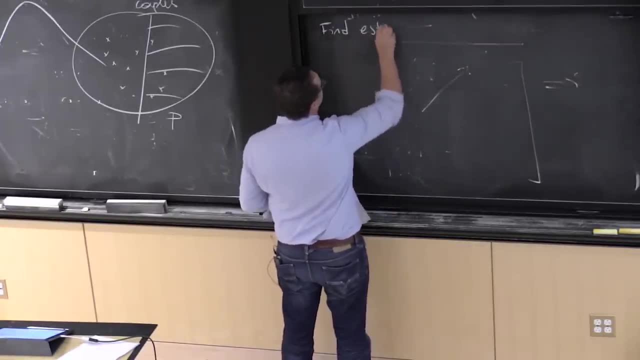 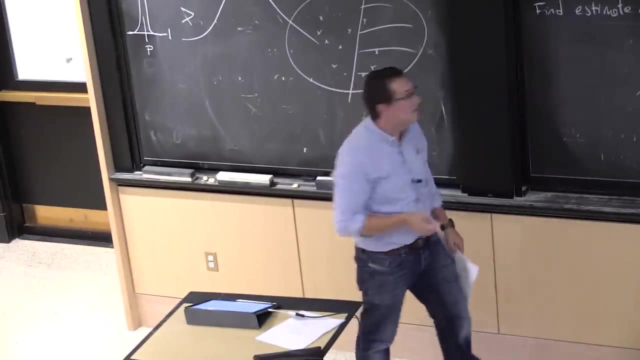 So it's not going to boil down to being a number of 1's divided by the total numbers. Now, if I'm looking for an estimate, well, I need to actually sum those numbers and divide them by 15.. So my estimate is going to be 1 over 15.. 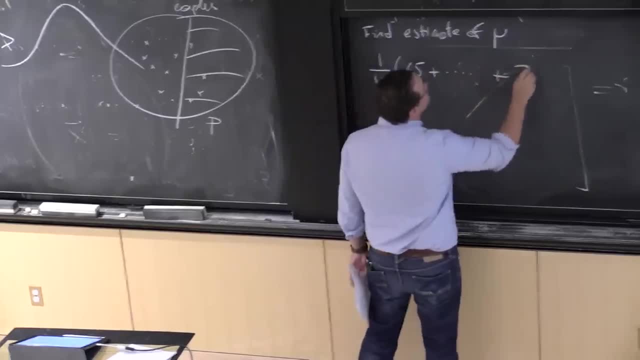 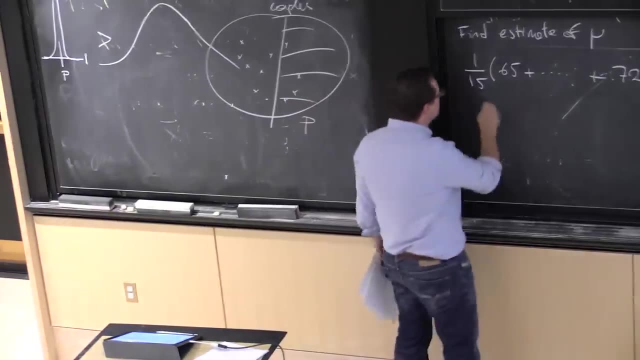 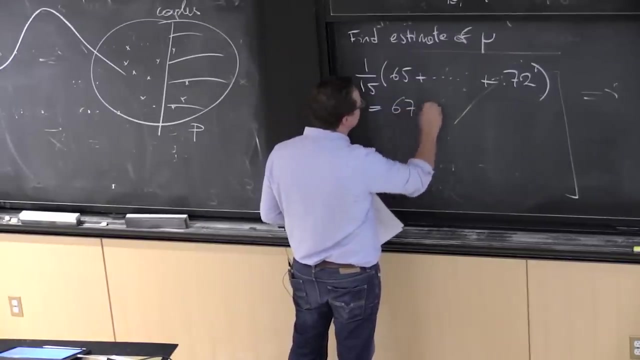 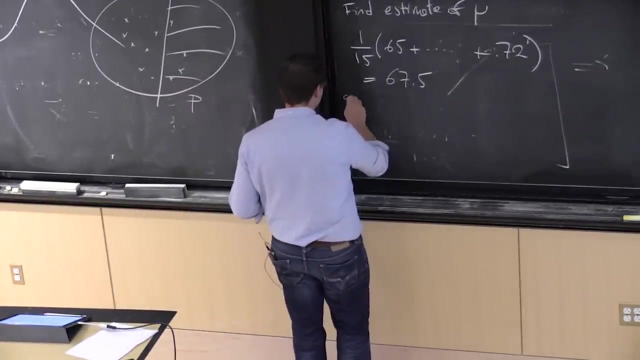 And then I'm going to start summing those numbers: 65 plus 72.. OK, And I can do it, and it's 67.5.. So this is my estimate. Now, if I want to compute a standard deviation, 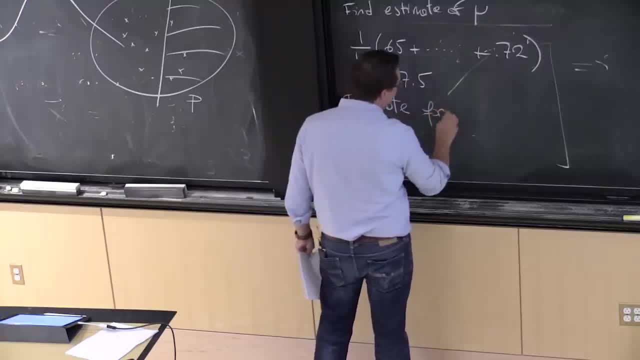 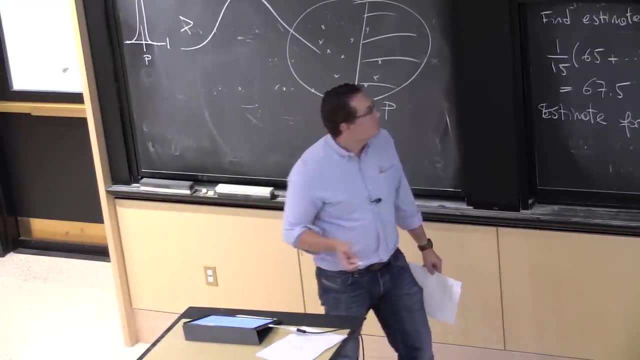 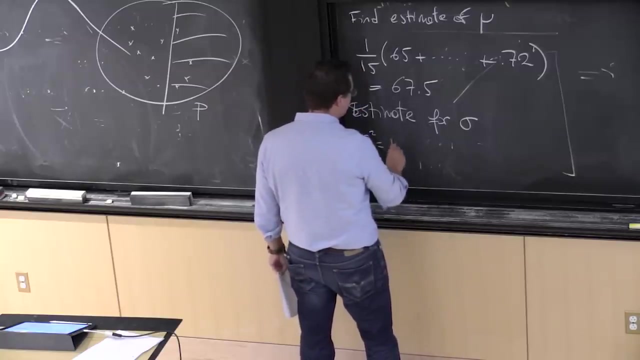 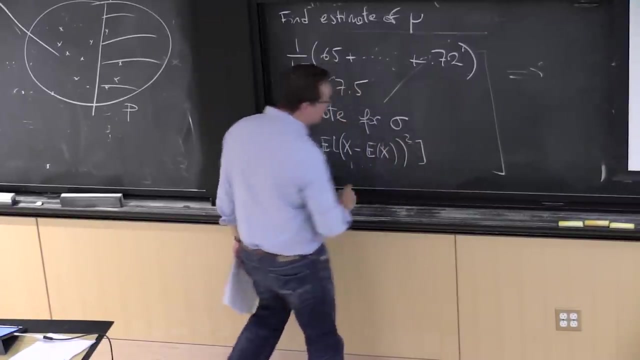 so let's say: estimate for sigma. you've seen that before, right, An estimate for sigma is what An estimate for sigma, and we'll see methods to do this. but sigma squared is the variance, so it's the expectation of x minus expectation of x squared. 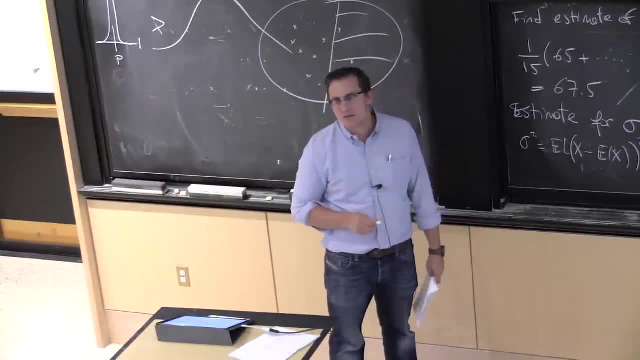 And the problem is that I don't know what those expectations are, And so I'm going to do what 99.9% of statistics is. What is statistics about? That's my motto. Statistics is about replacing expectations. It's about replacing expectations with averages. 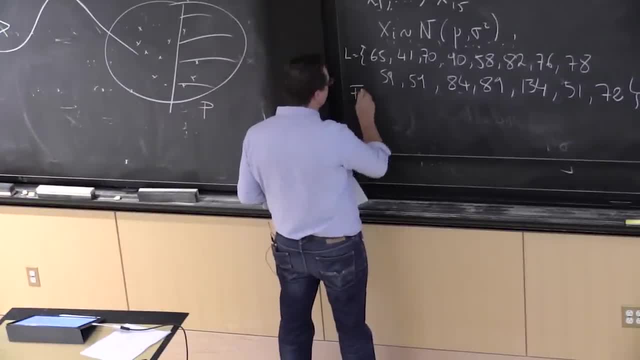 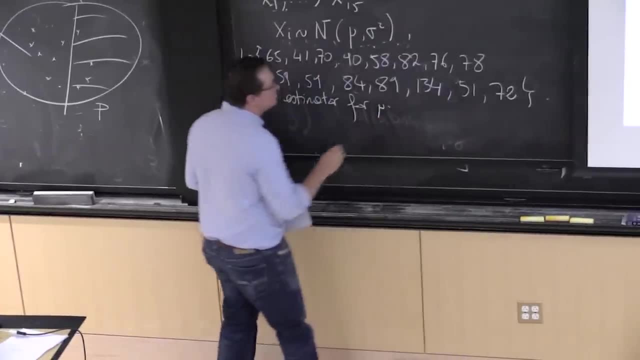 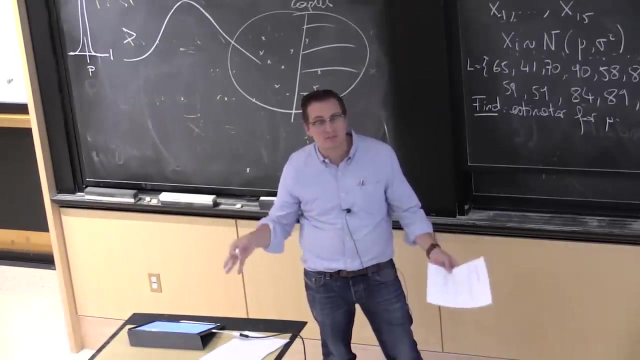 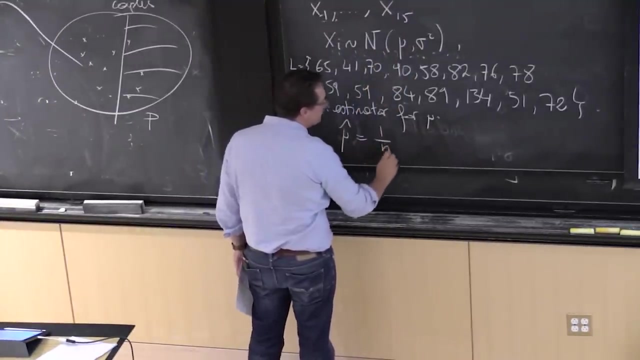 And the question is: find, Find an estimator for mu. What is my estimator for mu? Well, an estimator, again, is something that depends on the random variable. So mu is the expectation, right? So a good estimator is definitely the average score. 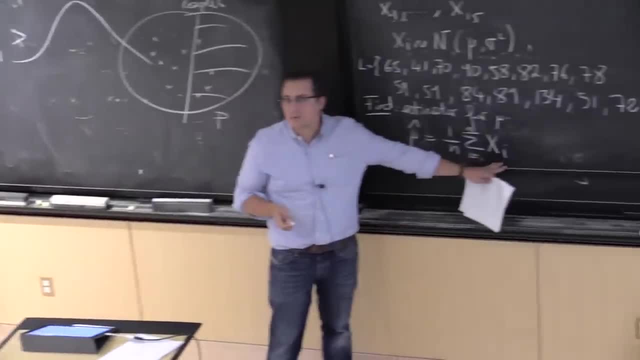 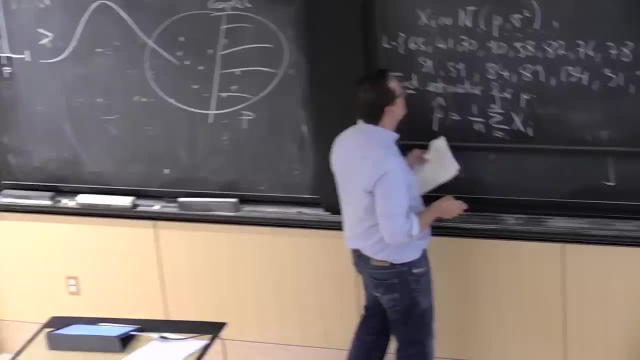 just like we had the average of the RIs, Now the Xi's no longer need to be 0s and 1s, So it's not going to boil down to being a number of 1s divided by the total numbers. 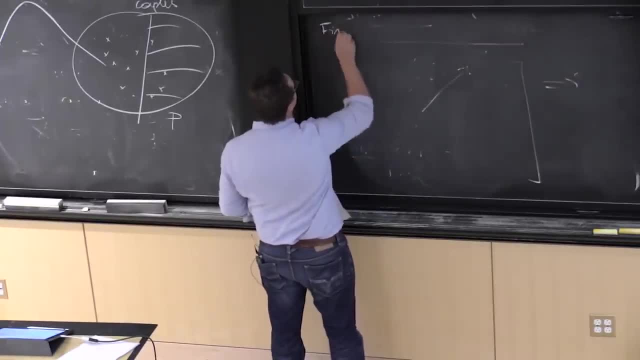 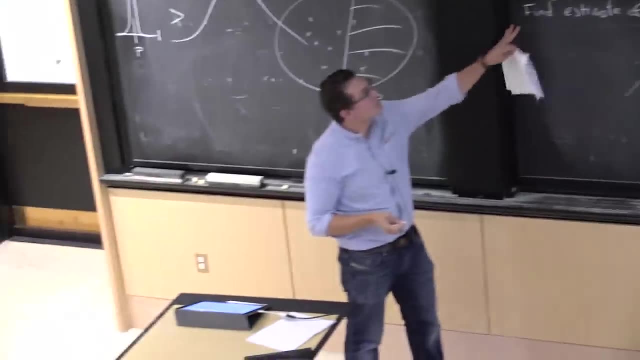 Now, if I'm looking for an estimate, well, I need to actually sum those numbers and divide them by 15, right? So my estimate is going to be 1 over 15.. And then I'm going to start summing those numbers: 65. 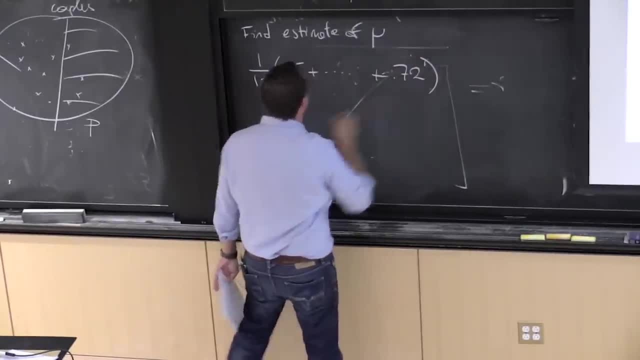 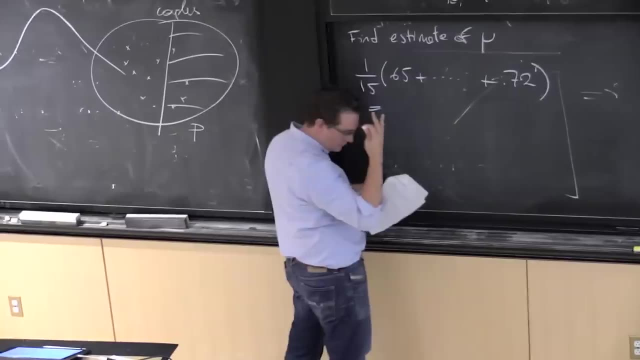 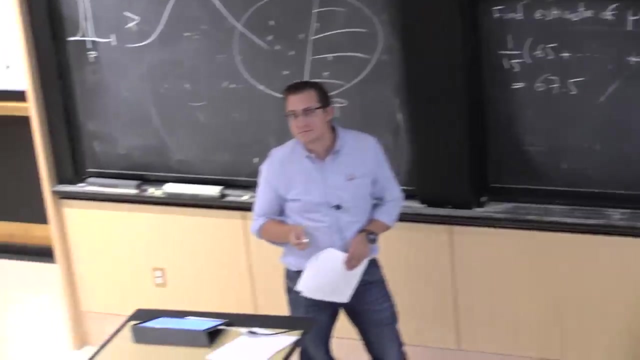 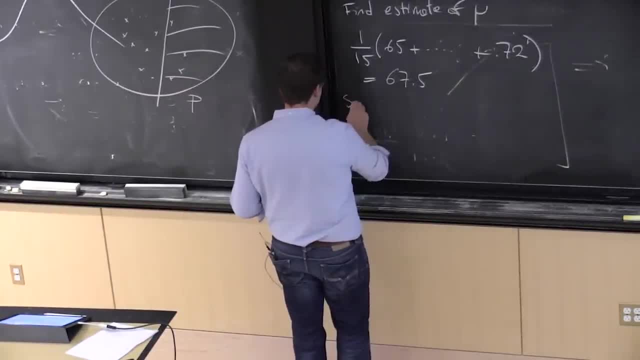 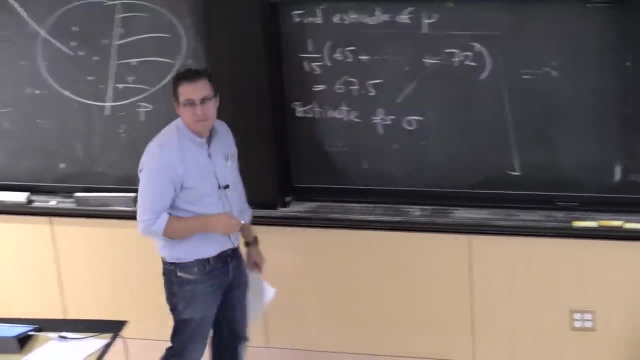 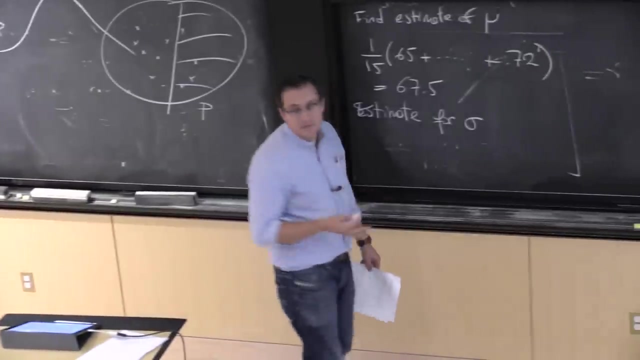 Now if I want to compute a standard deviation. so let's say estimate for sigma. you've seen that before. right, An estimate for sigma is what An estimate for sigma, and we'll see methods to do this. but sigma squared is the variance. 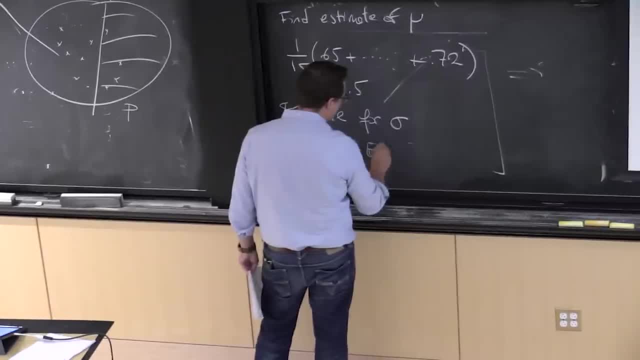 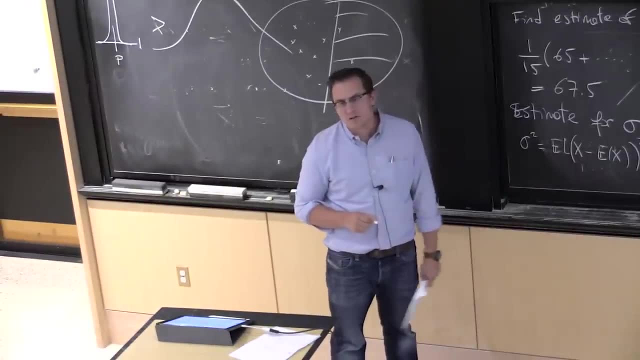 so it's the expectation of x minus expectation of x squared, And the problem is that I don't know what those expectations are, and so I'm going to do what 99.9% of statistics is. What is statistics about? That's my motto. 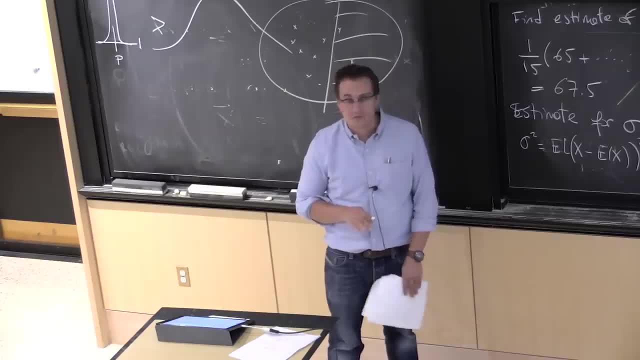 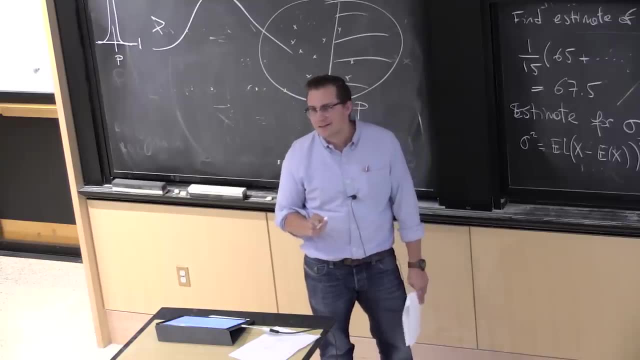 Statistics is about replacing expectations with averages. That's what all of statistics is about. There's 300 pages in a purple book called All of Statistics that tell you this, And then you do something fancy. Maybe you minimize something after you replace the expectation. 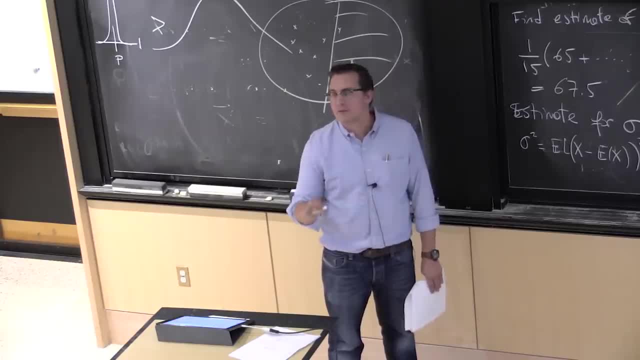 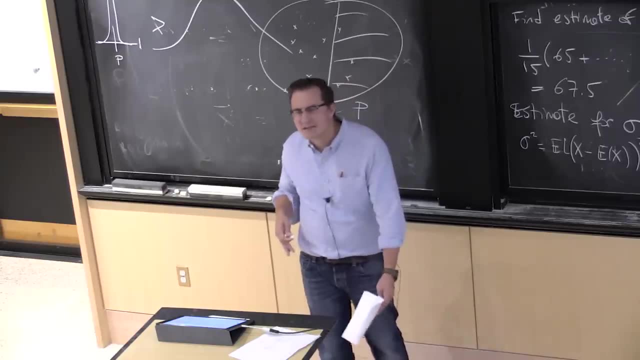 That's what all of statistics is about. There's 300 pages in a purple book called All of Statistics that tell you this, And then you do something fancy. Maybe you minimize something after you replace the expectation. Maybe you need to plug in all this stuff. 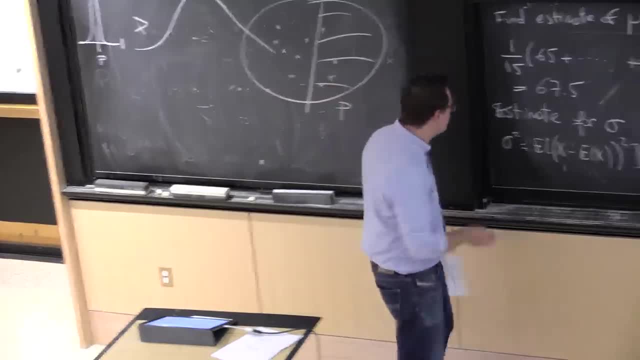 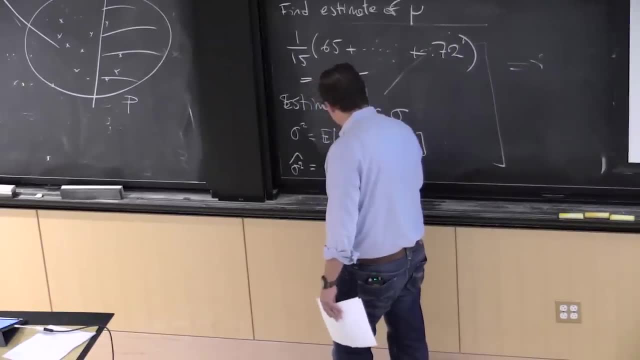 But really, every time you see an expectation, you replace it by an average. OK, let's do this. So sigma squared hat will be what It's going to be. 1 over n, sum from i equal 1 to n of xi. 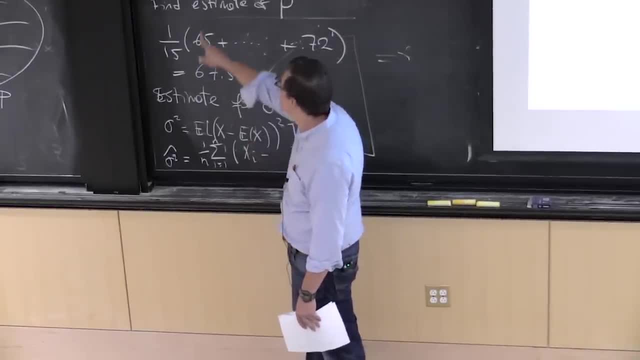 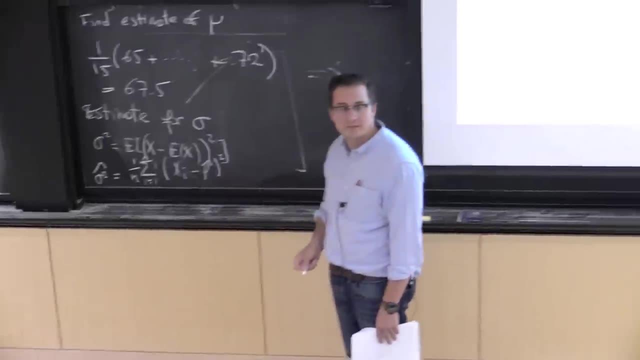 minus. well, here I need to replace my expectation by an average, which is really this average. So I'm going to call it nu hat squared. There you go. I've replaced my expectation with average. OK, so the golden thing is: take your expectation. 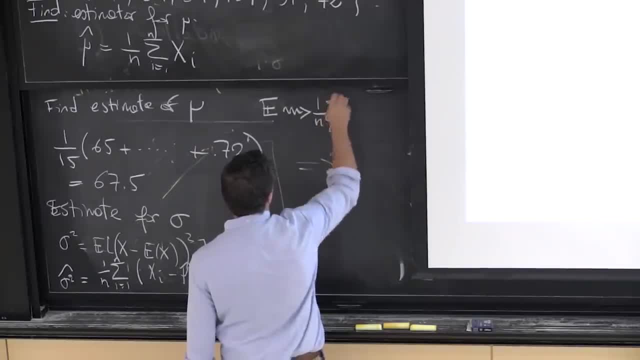 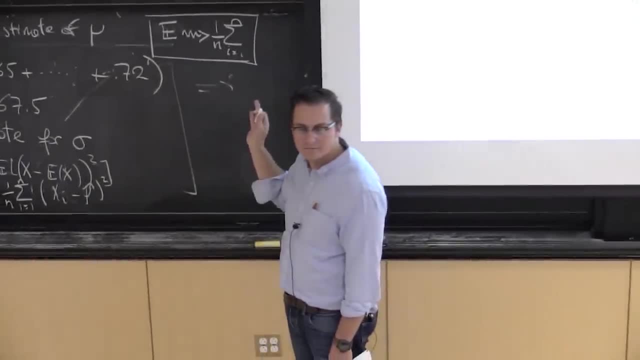 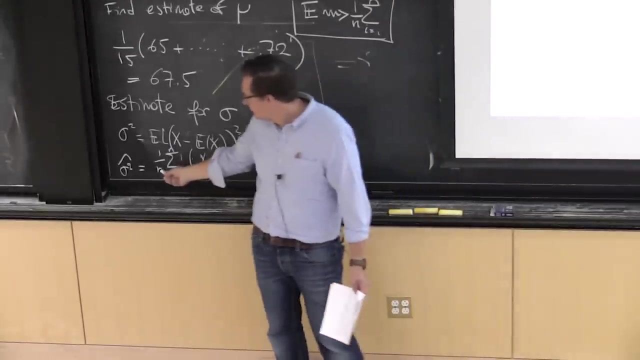 and replace it with this Frame, it Get a tattoo. I don't care, but that's what it is. If you remember one thing from this class, that's what it is. So now you can be fancy. If you look at your calculator, it's going to put an n minus 1. 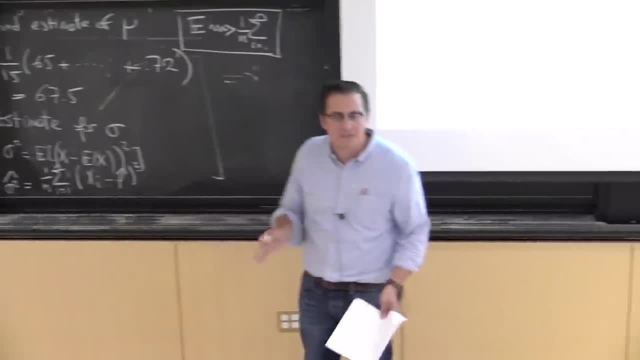 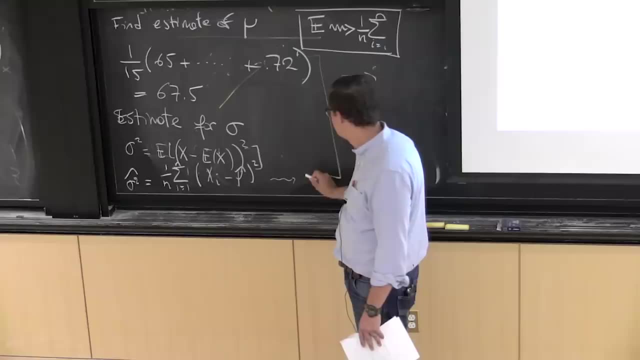 here because it wants to be unbiased, And those are things we're going to come to. But let's say right now we stick to this And then, when I plug in my numbers, I'm going to get an estimate for sigma which: 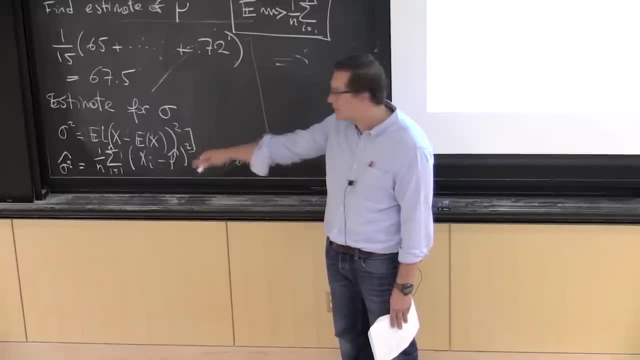 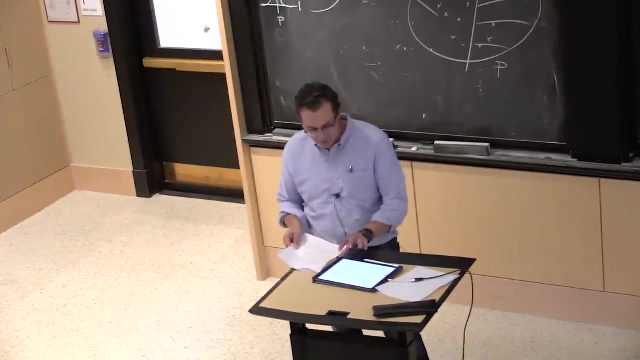 is the square root of the estimator. once I plug in the numbers And you can check that, the number you will get will be 18.. OK, So those are basic things And if you've taken any AP stats, this should be completely standard to you. 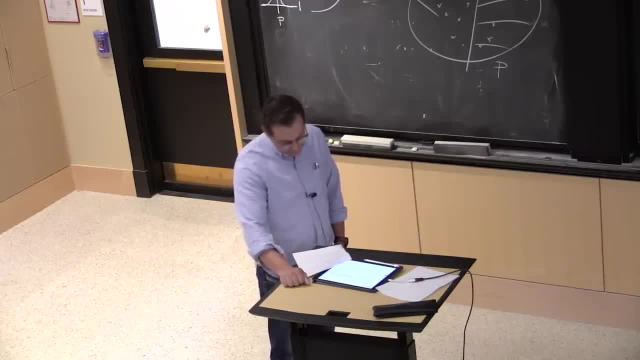 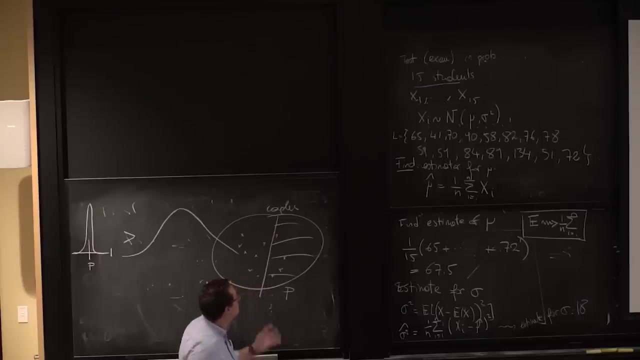 Now I have another list And I don't have time to see it. It doesn't really matter. OK, we'll do that next time. This is fine. We'll see another list of numbers and see We're going to think about modeling assumptions. 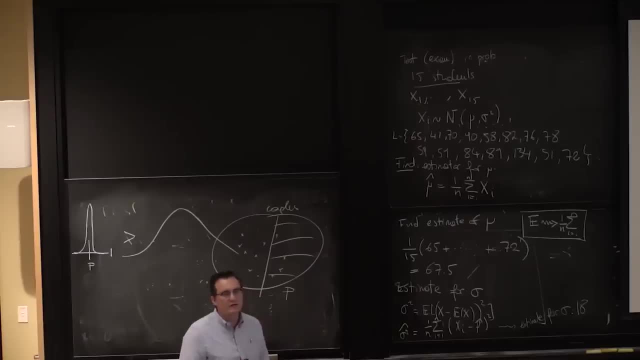 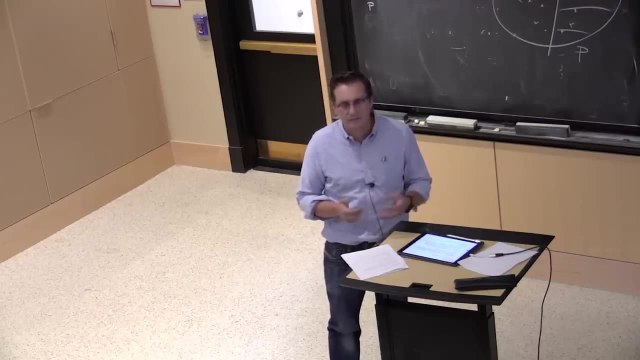 The goal of this exercise is not to compute those things. It's really to think about modeling assumptions. Is it reasonable to think that things are iid? Is it reasonable to think that they have all the same parameters, that they're independent, et cetera? 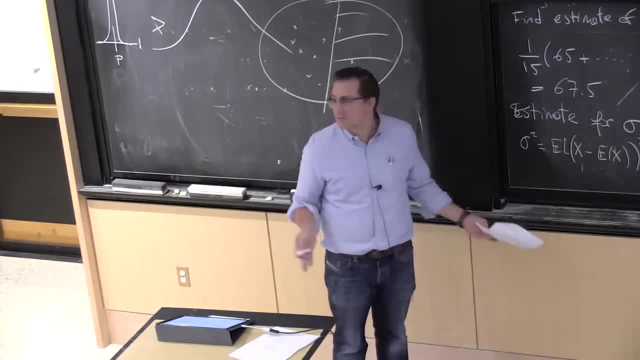 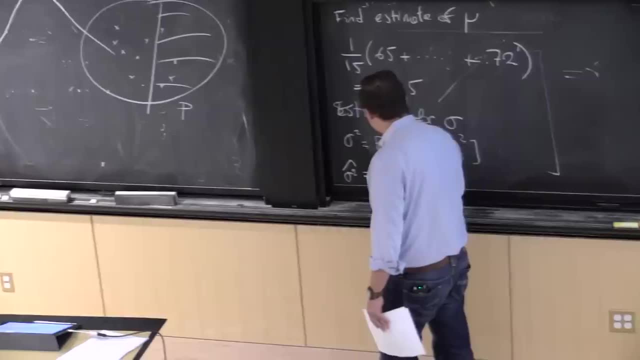 Maybe you need to plug in all this stuff, But really, every time you see an expectation, you replace it by an average. OK, let's do this. So sigma squared hat will be what It's going to be. 1 over n. sum from i equal 1 to n of xi minus. 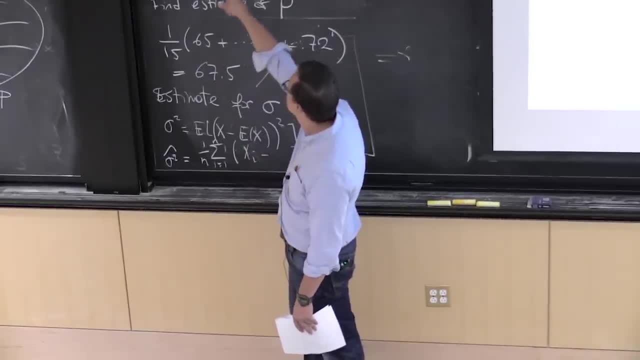 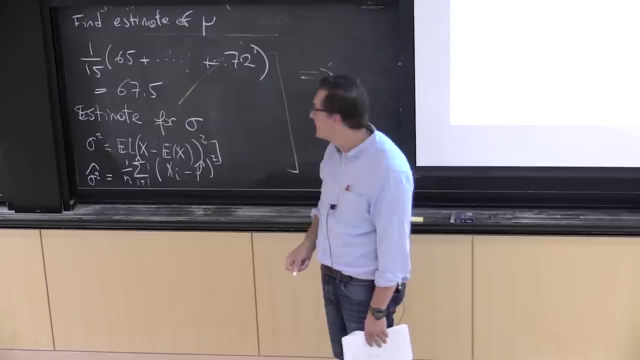 well, here I need to replace my expectation by an average, which is really this average. So I'm going to call it mu hat squared. There you go. I've replaced my expectation with average. OK, so the golden thing is: take your expectation. 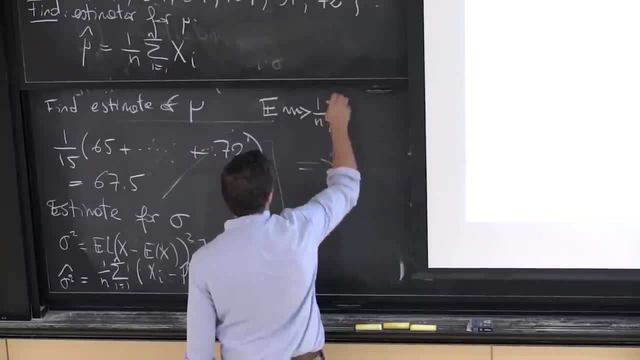 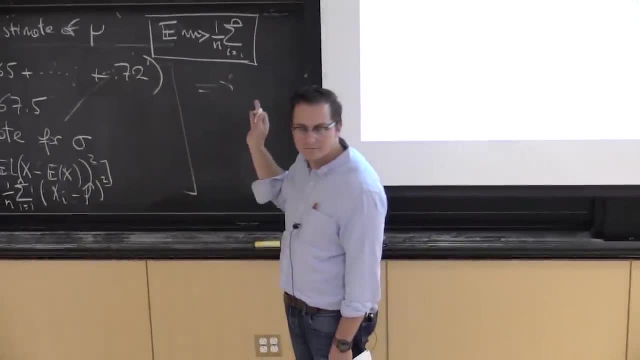 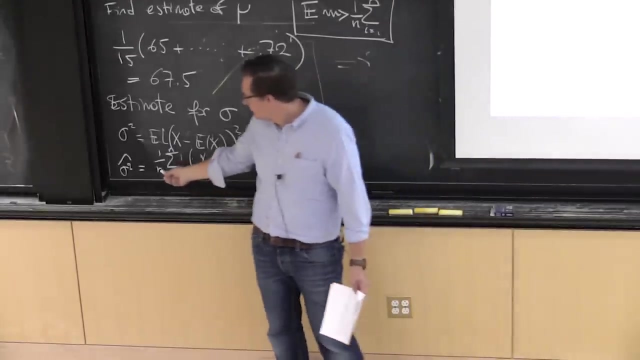 and replace it with this Frame, it Get a tattoo. I don't care, but that's what it is. If you remember one thing from this class, that's what it is. Now you can be fancy If you look at your calculator: it's. 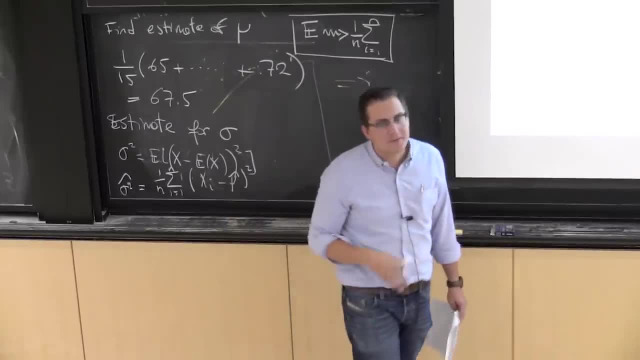 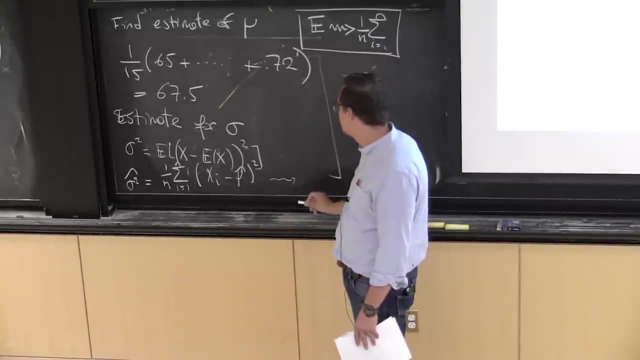 going to put an n minus 1 here because it wants it to be unbiased, And those are things we're going to come to. But let's say right now, we stick to this And then, when I plug in my numbers, I'm going to get an estimate for sigma which. 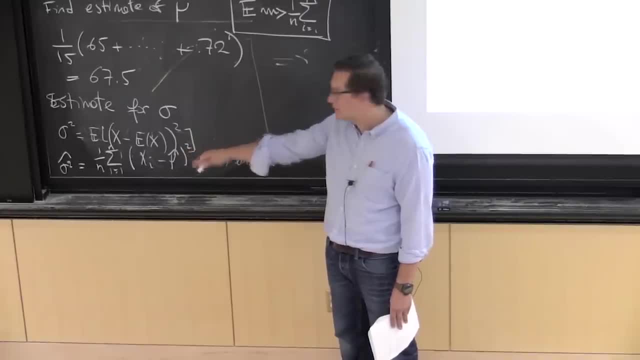 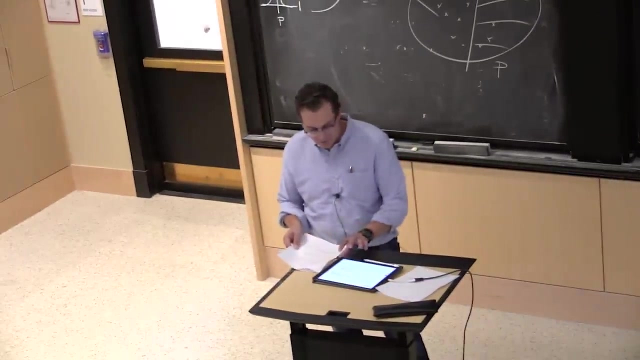 is the square root of the estimator. once I plug in the numbers And you can check that, the number you will get will be 18.. OK, So those are basic things And if you've taken any AP stats, this should be completely standard to you. 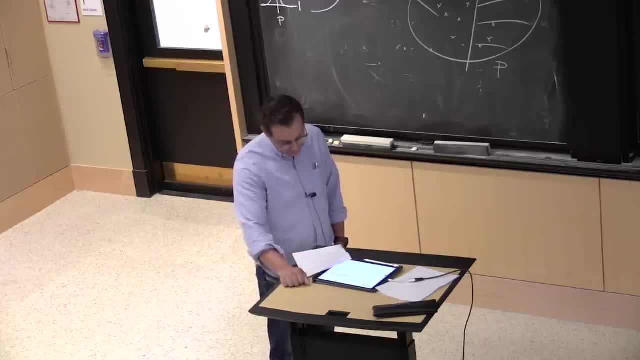 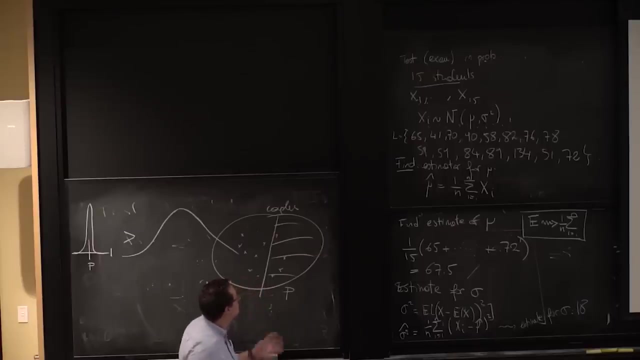 Now I have another list And I don't have time to see it. It doesn't really matter. OK, we'll do that next time. This is fine. We'll see another list of numbers and see We're going to think about modeling. 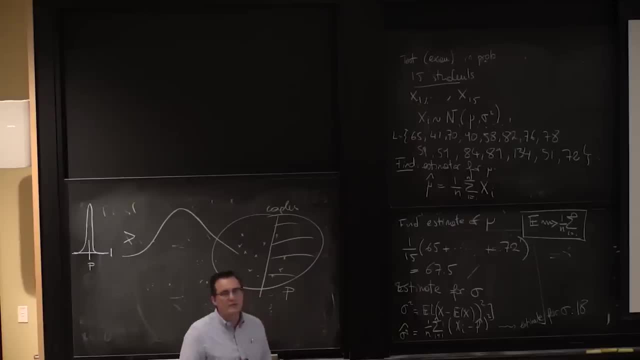 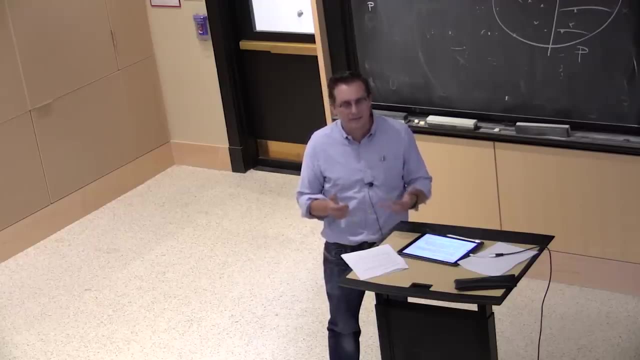 Assumption. the goal of this exercise is not to compute those things. It's really to think about modeling assumptions. Is it reasonable to think that things are iid? Is it reasonable to think that they have all the same parameters, that they're independent? 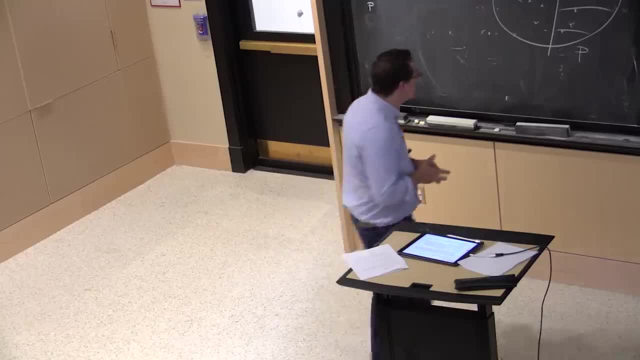 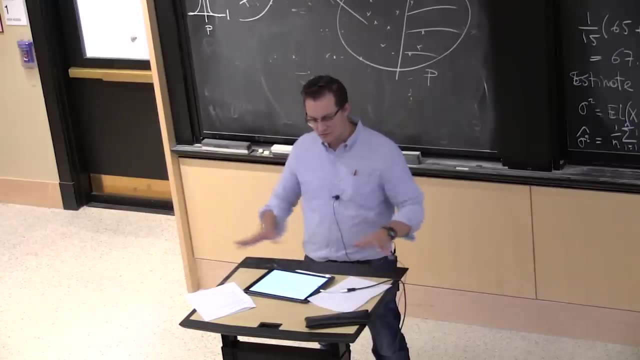 et cetera. OK, so one thing that I wanted to add is probably by tonight, so I will try to use- in the spirit of you- I don't know what's starting to happen- In the spirit of using my iPad and fancy things. I will.